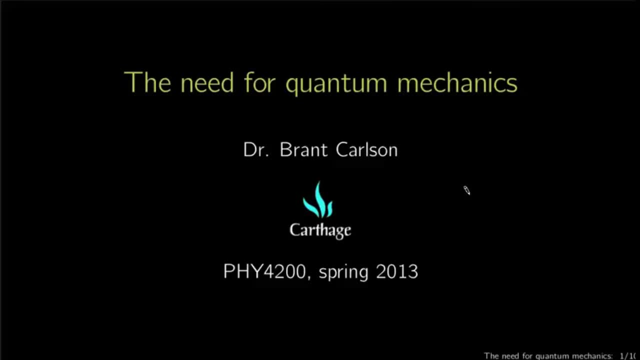 and second of all, to put it in historical context. Well, I'll show one of the most famous photographs in all of physics. that really gives you a feel for the brain power that went into the construction of this theory And hopefully we'll put it in some historical context as well. 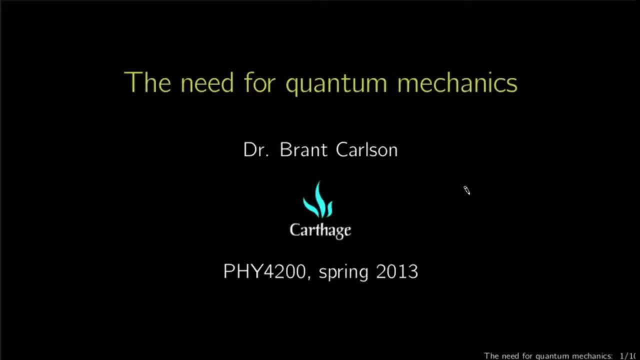 so you can understand where it fits in the broader philosophy of science. But the main goal of this lecture is about the need for Quantum Mechanics, which I really ought to just have called. Why Do We Need Quantum Mechanics? This subject has a reputation for being a little bit annoying. 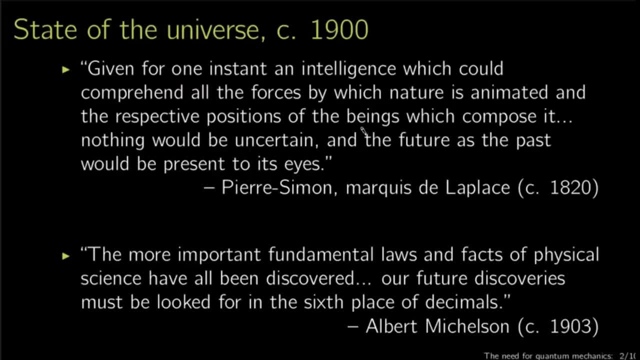 so why do we bother with it? Well, first off, for some historical context, imagine yourself back in 1900., Turn of the century. Science has really advanced a lot. We have electricity, We have all this fabulous stuff that electricity can do. 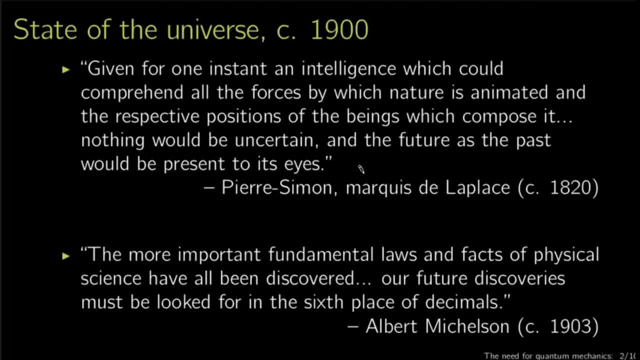 And even almost a hundred years before that, physicists thought they had things figured out. There's a famous quote from Laplace: Given for one instant an intelligence which could comprehend all the forces by which nature is animated and the respective position of the beings which compose it. 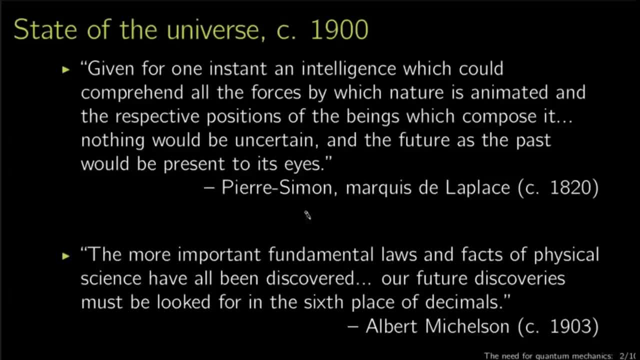 nothing would be uncertain and the future as the past would be present to its eyes. Now, maybe you think intelligence which can comprehend all the forces of nature is a bit of a stretch, And maybe such a being which can know all the respective positions of everything in the universe? 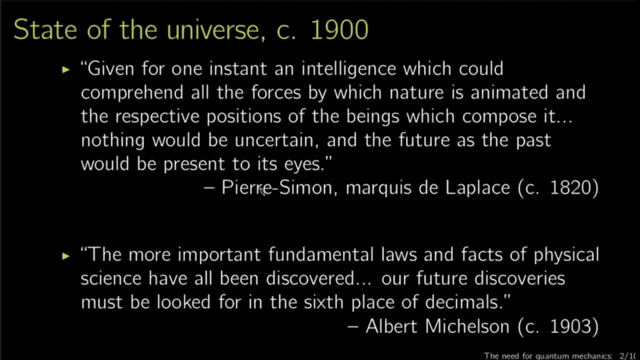 is a bit of a stretch as well. The feeling at the time was that if you could do that, you would know everything. If you had perfect knowledge of the present, you could predict the future And, of course, you can infer what happened in the past. 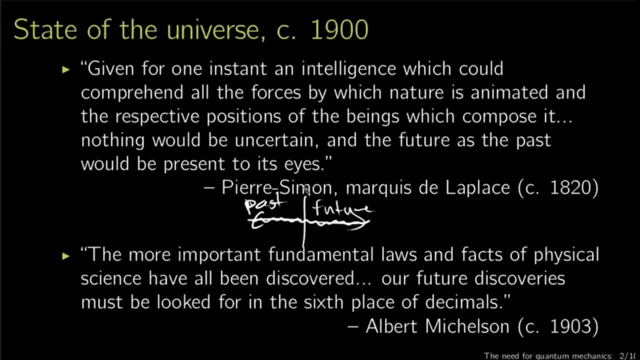 And everything is connected by one unbroken chain of causality. Now, in 1903, Albert Michelson- another famous quote from that time period- said: The more important fundamental laws and facts of physical science have all been discovered. Our future discoveries must be looked for. 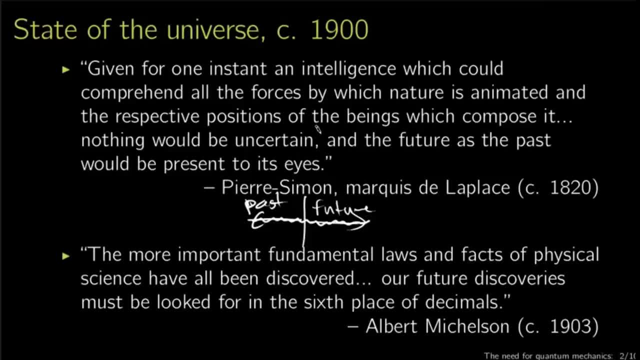 in the sixth place of decimals. Now this sounds rather audacious. This is 1903, and he thought that the only thing that we had left to nail down was the part-in-a-million level precision. Well, to be fair to him, he wasn't talking about. 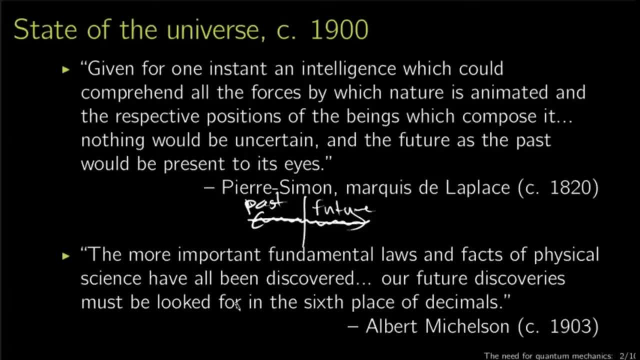 never discovering new fundamental laws of physics. He was talking about really astonishing discoveries, like the discovery of Uranus on the basis of orbital perturbations of Neptune. Never having seen the planet Uranus before, they figured out that it had to exist just by looking at things that they had seen. 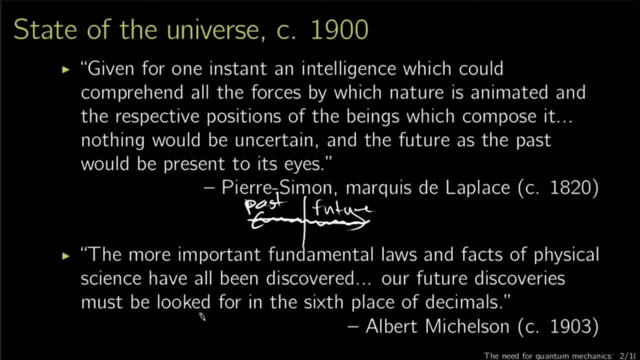 That's pretty impressive And Michelson was really on to something. Precision measurements are really really useful, especially today, But back in 1903, it wasn't quite so simple and Michelson probably regretted that remark for the rest of his life. 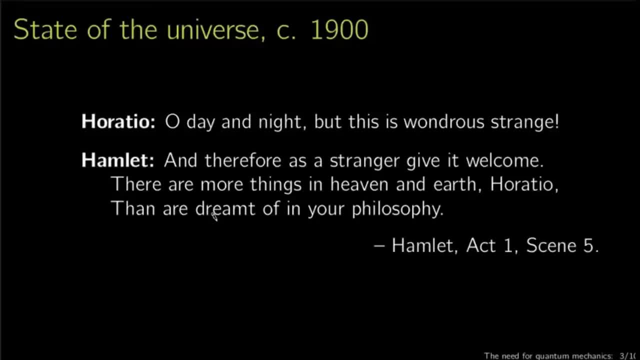 The attitude that I want you guys to take when you approach quantum mechanics, though, is not this sort of 1900s notion that everything is predicted. It comes from Shakespeare. Horatio says So. that's the attitude I want you guys to take. 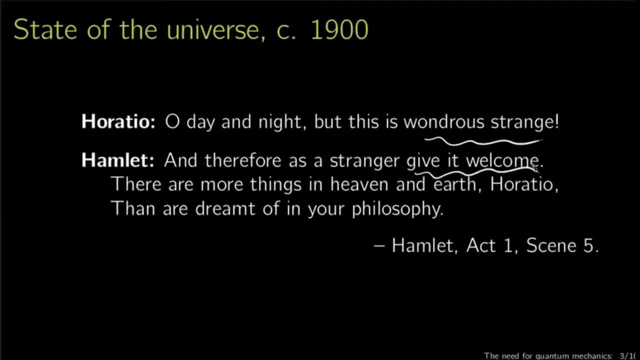 when you approach quantum mechanics, It is wondrous, strange and we should give it welcome. There are some things in quantum mechanics that are deeply non-intuitive, but if you approach them with an open mind, quantum mechanics is a fascinating subject. There's a lot of really fun stuff. that goes on. 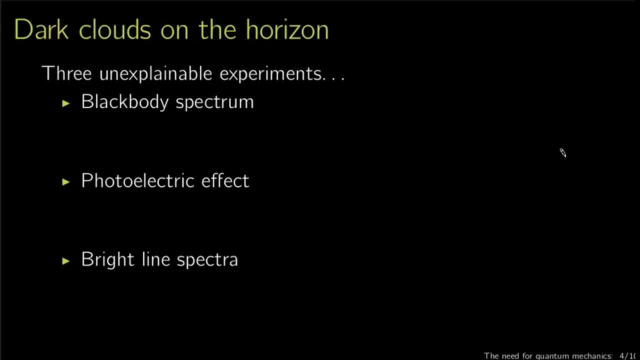 Now to move on to the necessity for quantum mechanics. there were some dark clouds on the horizon even at the early 20th century. Michelson wasn't quite having a big enough picture in his mind when he said that everything was down to the sixth place of decimals. 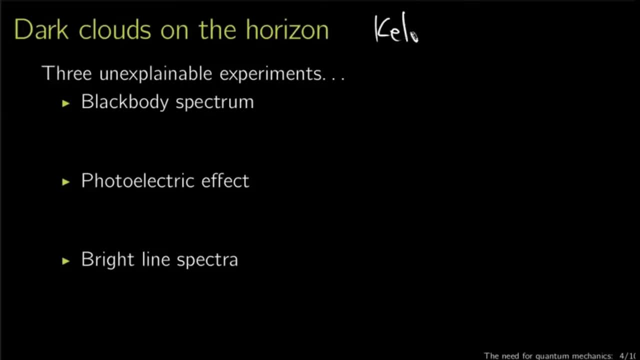 The dark clouds on the horizon, at least according to Kelvin. here were a couple of unexplainable experiments. One, the black body spectrum. Now a black body you can just think of as a hot object, And a hot object like, for example, 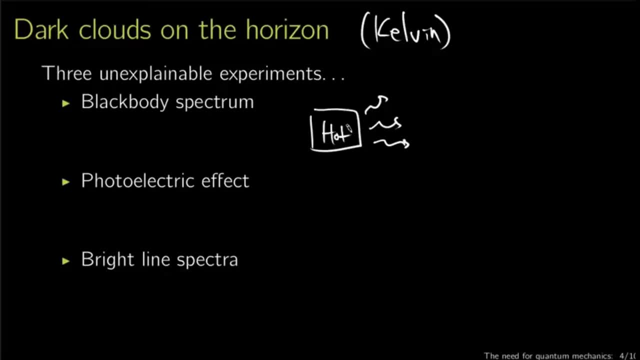 the coils on an electrical stove when they get hot will glow, And the question is: what color do they glow? Do they glow red? Do they glow blue? What is the distribution of radiation that is emitted by a hot object? Another difficult to explain experiment. 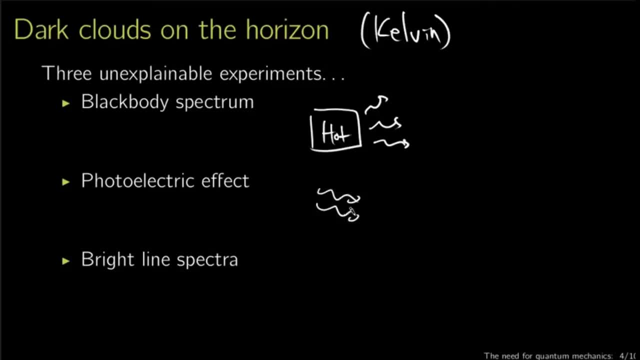 is the photoelectric effect. If you have some light and it strikes a material, electrons will be ejected from the surface And, as we'll discuss in a minute, the properties of this experiment do not fit what we think we know about, or at least what physicists thought they knew. 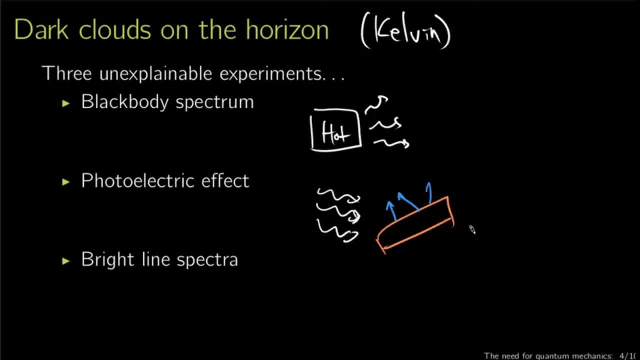 about the physics of light and the physics of electrons at the turn of the 20th century. The final difficult experiment to explain is bright line spectra. For example, if I have a flame coming from, say, a Bunsen burner, and I put a chunk of something, 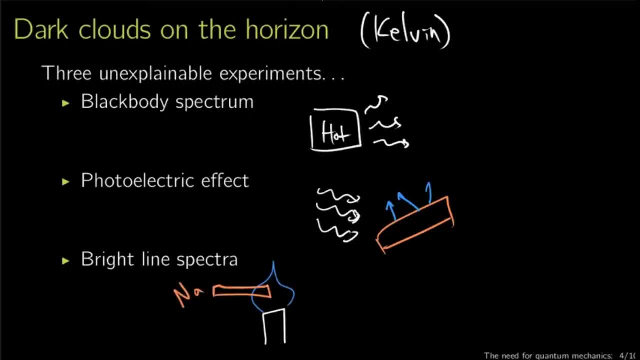 perhaps sodium in that flame it will emit a very particular set of frequencies that looks absolutely nothing like a black body. We'll talk about all of these experiments in general or in a little bit more detail in a minute or two. but just looking at these experiments now. 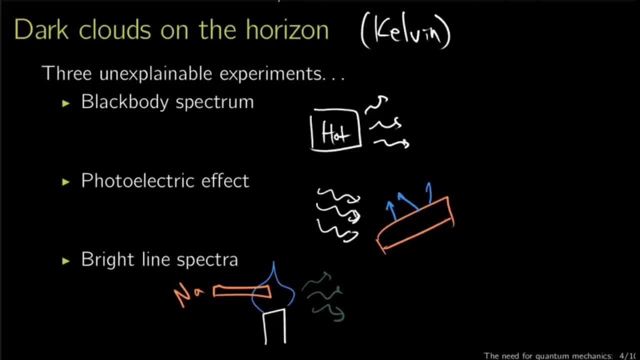 these are all experiments that are very difficult to explain, knowing what we knew at the turn of the 20th century about classical physics, And they're also experiments that involve light and matter, So we're really getting down to the details of what stuff is really made of. 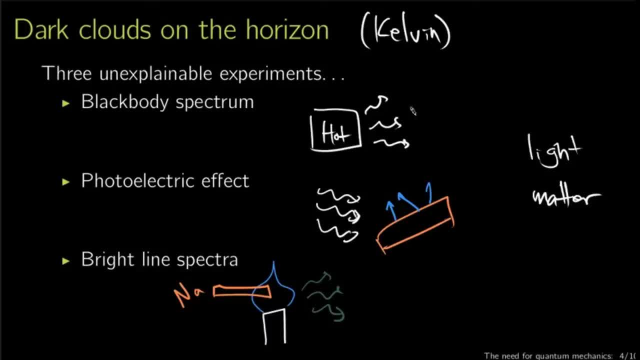 and how it interacts with the things around it. So these are some pretty fundamental notions and that's where quantum mechanics really got its start. So let's pick apart these experiments in a little more detail. The black body spectrum, as I mentioned. 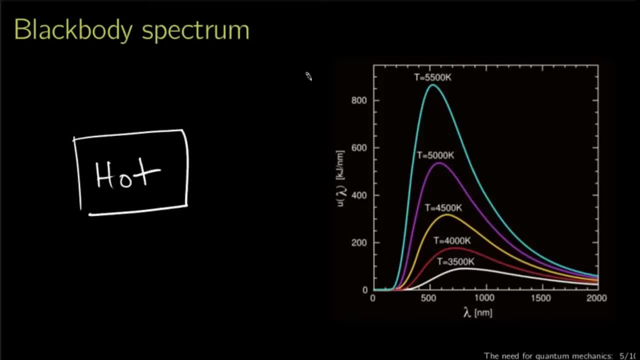 you can think of as the light that's emitted just by a hot object. And while hot objects have some temperature associated with them, let's call that T. The plot here on the right is showing very qualitatively, I'll just call it. 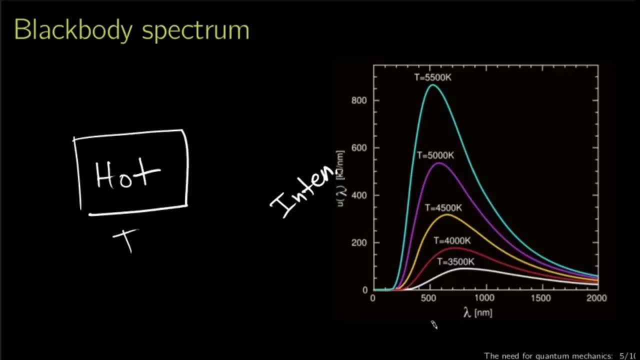 the intensity of the light emitted as a function of the wavelength of that light. So short wavelengths- high energy, long wavelengths- low energy. Now if you look at, T equals 3500 Kelvin. curve here. it has a long tail to long wavelengths. 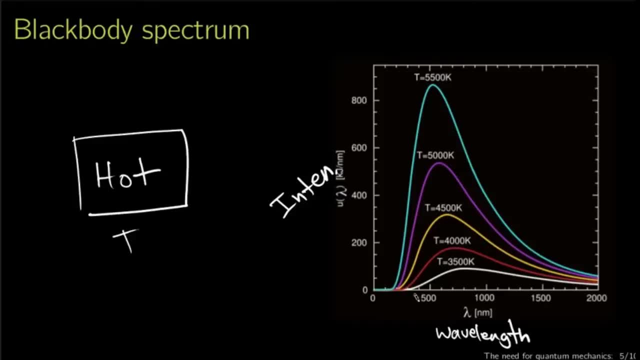 and it cuts off pretty quickly as you go to short wavelengths, So it doesn't emit very much high energy light, Whereas if you have a much hotter object- 5500 Kelvin- it emits a lot more high energy light. The red curve here is much higher than the black curve. 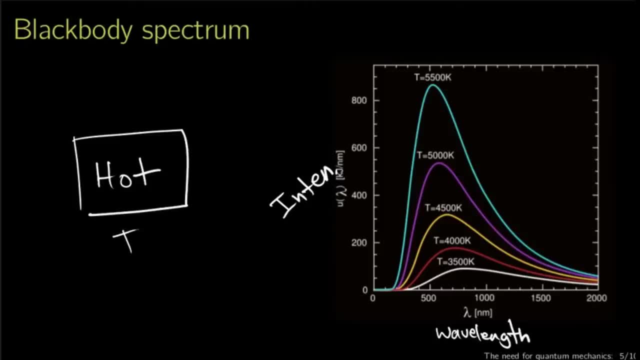 Now, if you try to explain this, knowing what early 20th century physicists knew about radiation and about electrons and about atoms and how they could possibly emit light, you get a prediction And it works wonderfully well up until about here, at which point it blows up to infinity. 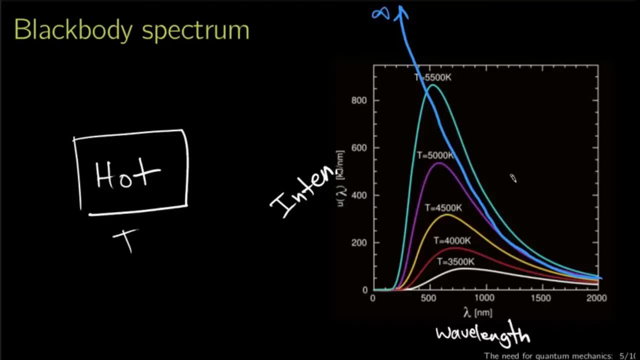 Infinities are bad in physics. This is the Rayleigh-Jeans law, and it works wonderfully well for long wavelengths, but does not work at all for short wavelengths. That's called the ultraviolet catastrophe, if you've heard that term. 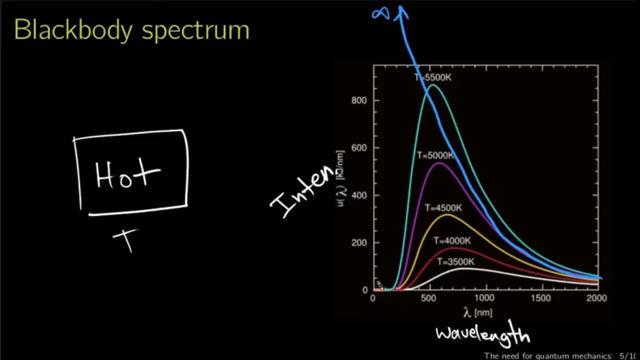 On the other end of things, if you look at what happens down here, well, it's not so much a prediction but an observation. but there's a nice formula that fits here. So on one side we have a prediction that works well on one end, but doesn't work on the other. 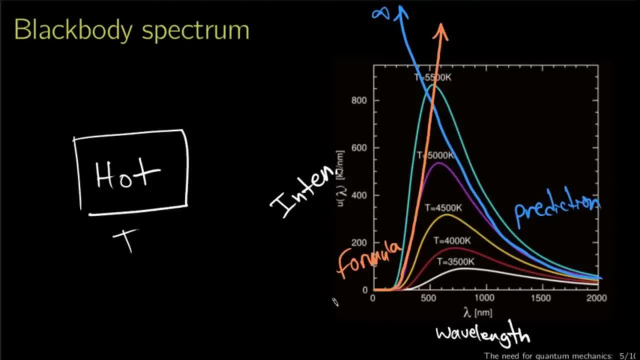 And on the other hand we have a sort of empirical formula called Wien's law that works really well at the short wavelengths, but well also blows up to infinity at the long wavelengths. Both of these blowing up things are a problem, and the question is: how do you get something? 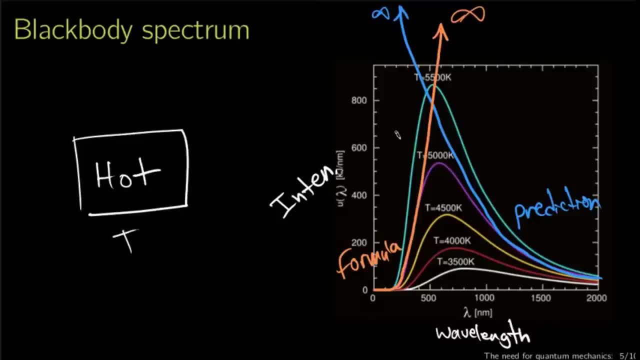 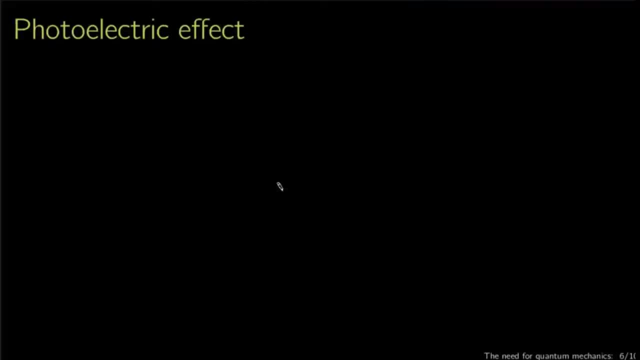 that explains both of them. This is the essence of the blackbody spectrum and how it was difficult to interpret in the context of classical physics. The next experiment I mentioned is the photoelectric effect. This is sort of the opposite problem. It's not how a material emits light. 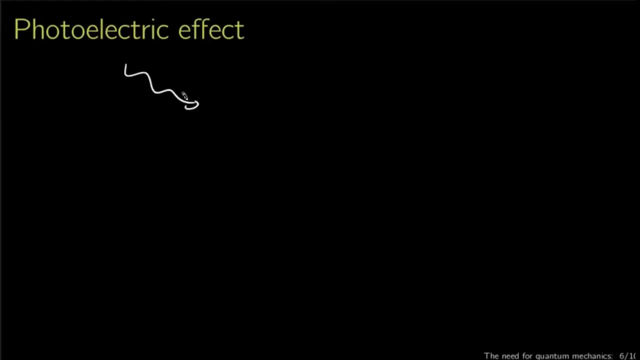 it's how light interacts with the material. So you have light coming in and the experiment is usually done like this: You have your chunk of material, typically a metal, and when light hits it, electrons are ejected from the surface, hence the electric part of the photoelectric effect. 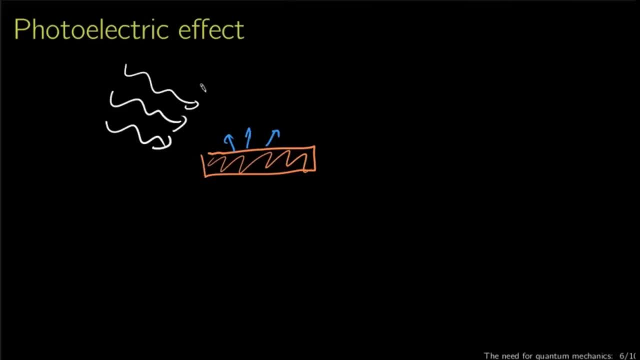 And you do all this in a vacuum and the electrons are then allowed to go across a gap to some other material, another chunk of metal. where they strike this metal- And the experiment is usually done like this- You connect it up to a battery. 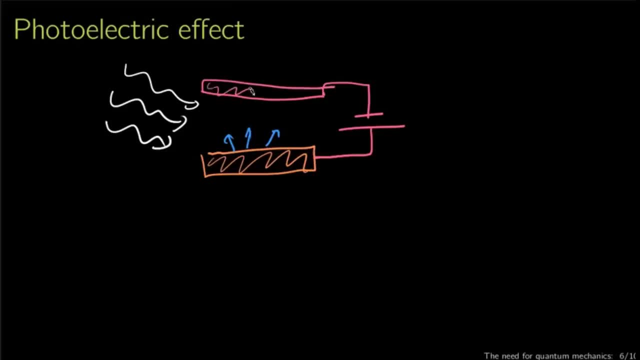 So you have your material on one side and your material on the other and you have light hitting one of these materials and ejecting electrons, And you tune the voltage on this battery such that your electrons, when they're ejected, never quite make it. 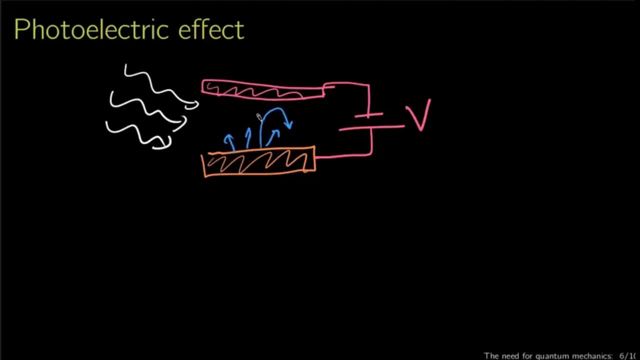 So the electric field produced by this voltage is opposing the motion of the electrons. When that voltage is just high enough to stop the motion of the electrons, keep them from completely making it all the way across. we'll call that the stopping voltage. Now it turns out. 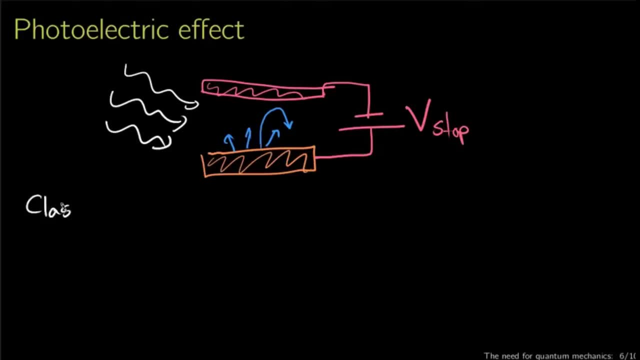 that what classical E&M predicts, as I mentioned, doesn't match what actually happens in reality. But let's think about what does classical E&M predict here. Well, classical electricity and magnetism says that electromagnetic waves here have electric fields and magnetic fields associated with them. 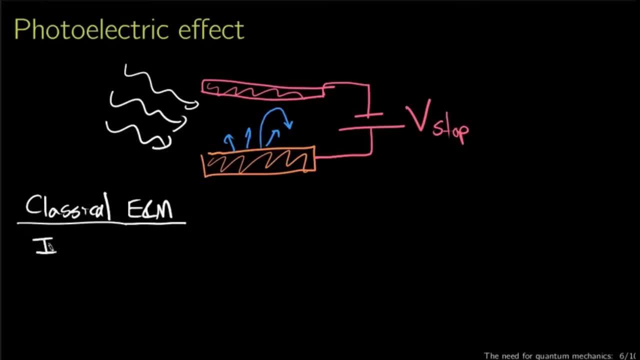 And these are propagating waves. If I increase the intensity of the electromagnetic wave, that means the magnitude of the electric field involved in the electromagnetic wave is going to increase. And if I'm an electron sitting in that electric field, the energy I acquire is going to increase. 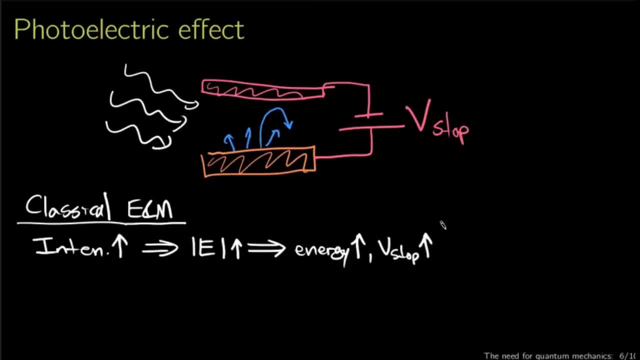 That means the stop is going to increase Because I'll have to have more voltage to stop a higher energy electron, as would be produced by a higher intensity beam of light. The other parameter of this incoming light is its frequency, So we can think about varying the frequency. 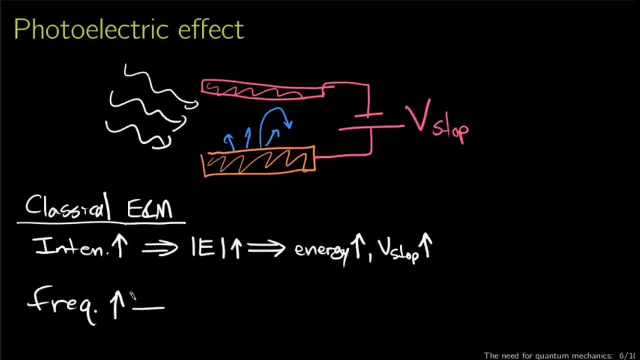 If I increase the frequency I have more intense light. Now that doesn't say anything about the string, sorry. if I increase the frequency I don't necessarily have more intense light. The electric field magnitude is going to be the same. 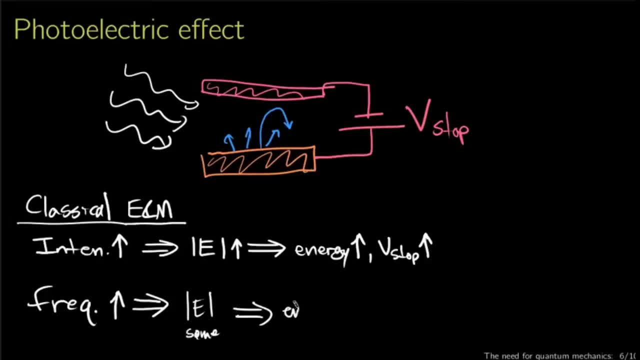 Which means the energy and the stopping voltage will also be the same. Now it turns out what actually happens in reality does not match this at all. In reality, when the intensity increases, the energy- which I should really write as V- stop. 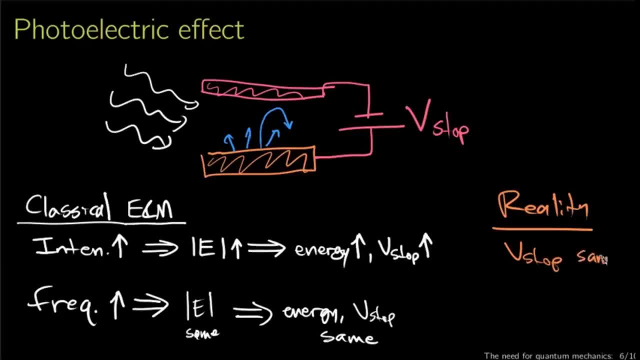 the stopping voltage necessary doesn't change, And when I increase the frequency, the voltage necessary to stop those electrons increases. So this is sort of exactly the opposite. What's going on here? That's the puzzle in explaining the photoelectric effect. 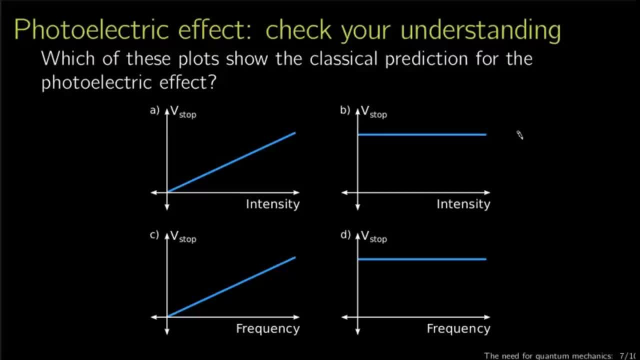 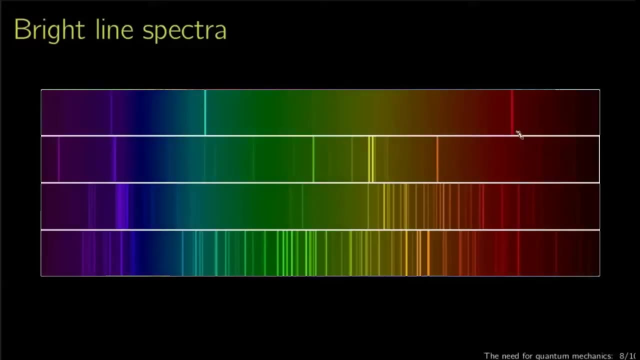 Just to briefly check your understanding, consider these plots of stopping voltage as a function of the parameters of the incident light and check off, which you think shows the classical prediction for the photoelectric effect. The third experiment that I mentioned is bright line spectra. 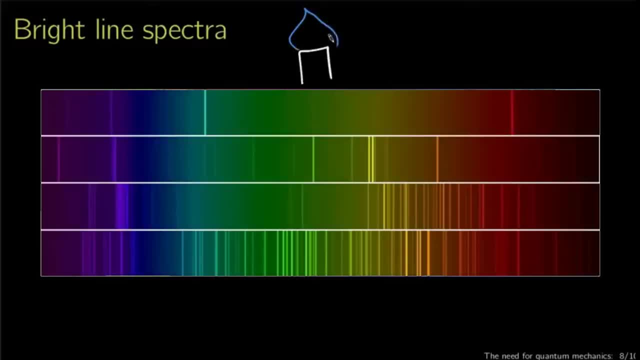 And, as I mentioned, this is what happens. if you take a flame or some other means of heating a material like the bar of sodium I mentioned earlier, This will emit light and, in this case, the spectrum of light from red to blue. 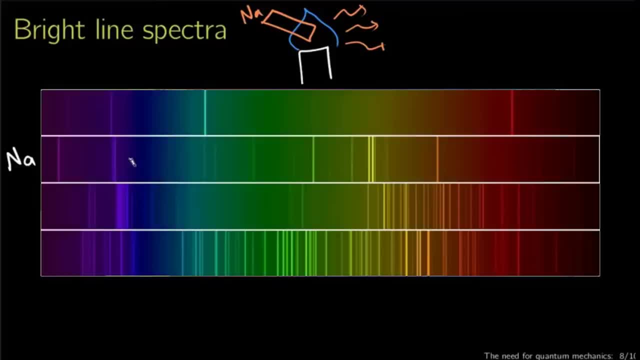 of sodium looks like this. Actually, I'm sorry, that's not sodium, that's mercury. These are four different elements: hydrogen, mercury, neon and xenon- And instead of getting a broad, continuous distribution, like you would from a black body, 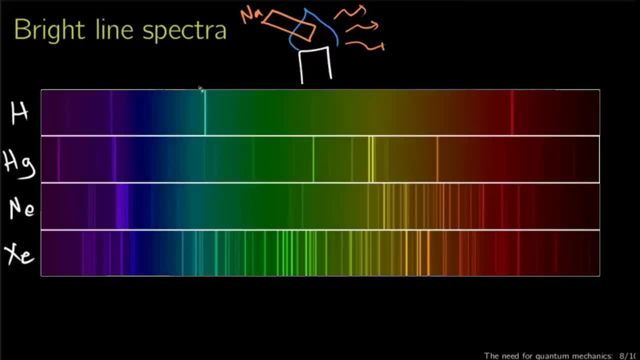 under these circumstances, where you're talking about gases, you get these very bright regions. It's the spectrum and instead of looking like a smooth curve like this, it looks like spikes. Those bright lines are extraordinarily difficult to explain with classical physics. 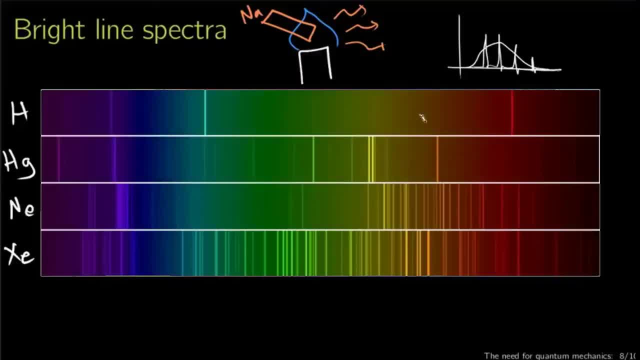 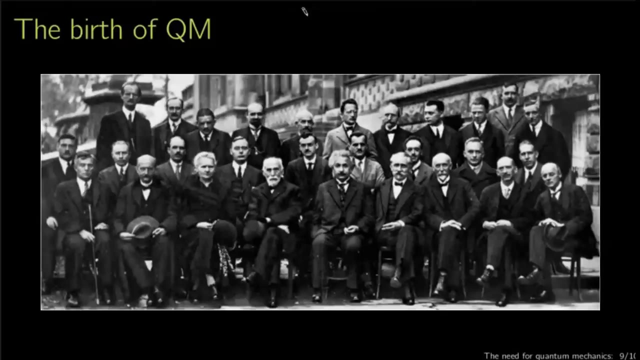 And this is really the straw that broke the camel's back, broke classical physics' back. that really kicked off quantum mechanics. How do you explain this? This is that famous photograph that I mentioned. This is really the group of people who first built quantum mechanics. 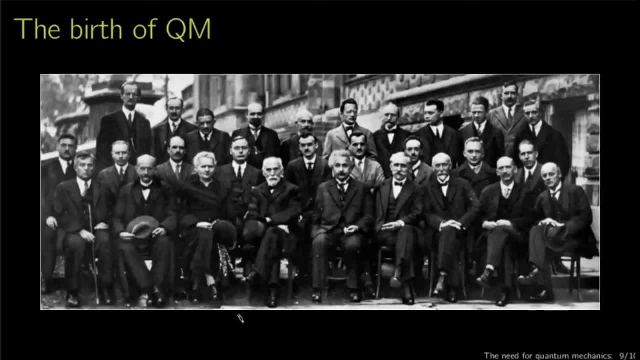 Now I mentioned three key experiments: The black body spectrum: this guy figured that out. This is Planck. The photoelectric effect: this guy- who I hope needs no introduction, this is Einstein- figured that out. This is the paper that won Einstein the Nobel Prize. 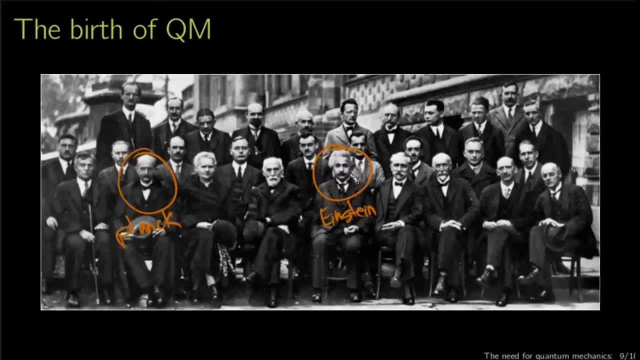 And as far as the bright line spectra of atoms. it took a much longer time to figure out how all of that fit together And it took a much larger group of people, But they all happen to be present in this photograph. There's this guy. 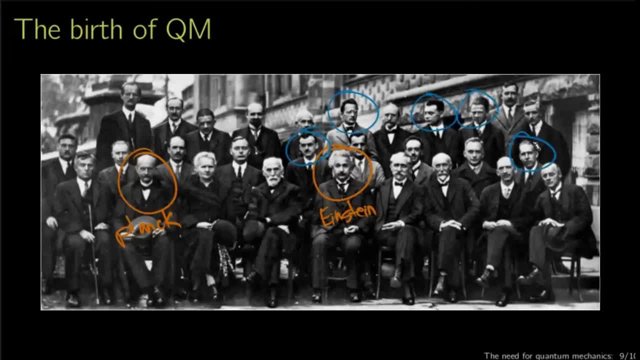 and this guy, and these two guys and this guy. This photograph is famous because these guys worked out quantum mechanics, But that's not the only. these aren't the only famous people in this photograph. You know this lady as well. This is Marie Curie. 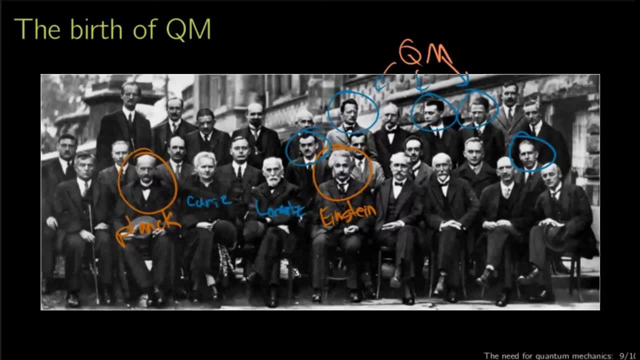 This is Lorentz, Which, if you studied special relativity, you know Einstein used the Lorentz transformations. Pretty much everyone in this photograph is a name that you know. I went through and looked up who these people were. These were all of the names that I recognized. 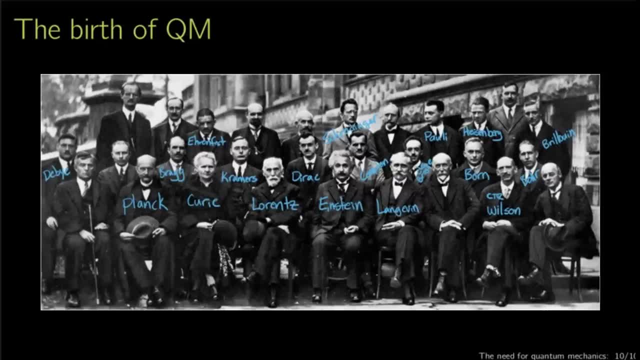 which doesn't mean that the people whose names I didn't recognize weren't also excellent scientists, For example, CTR Wilson here, One of my personal favorites- Inventor of the cloud chamber. This is the brain trust that gave birth to quantum mechanics. 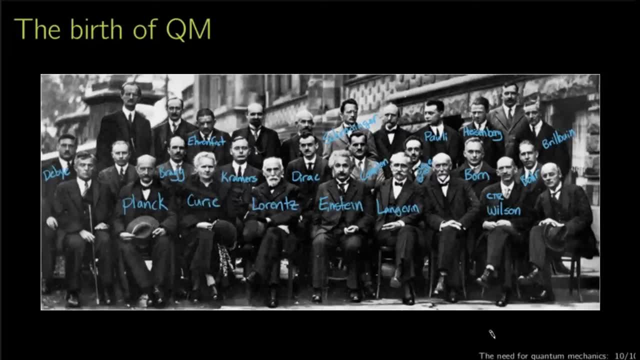 And it was quite a brain trust. You had some of the most brilliant minds of the century working on some of the most difficult problems of the century, And what's astonishing is they didn't really like what they found. They discovered explanations that made astonishingly accurate predictions. 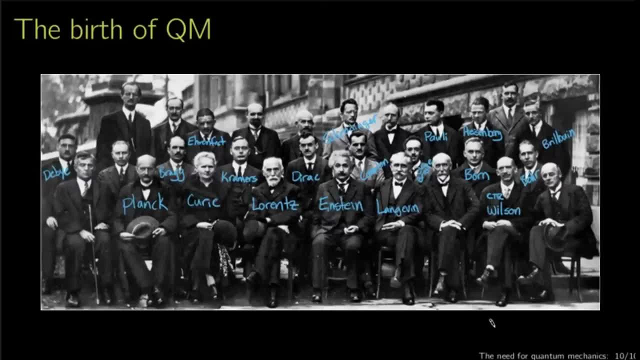 But throughout the history you keep seeing them disagreeing Like no, that can't possibly be right. Not necessarily because the predictions were wrong or they thought there was a mistake somewhere, but because they just disliked the nature of what they were doing. 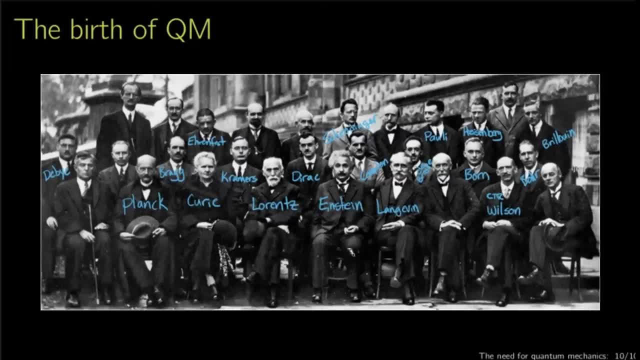 They were upending their view of reality. Einstein, in particular, really disliked quantum mechanics to the day that he died, Just because it was so counterintuitive. So with that introduction to a counterintuitive subject, I'd like to remind you again: 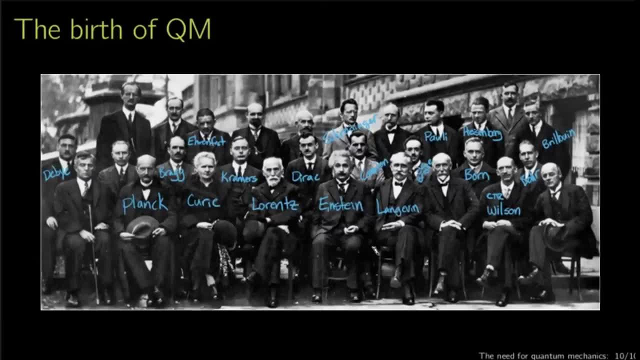 of that Shakespeare quote: There are more things in heaven and earth, Horatio, than are dreamt of in your philosophy. Try to keep an open mind and hopefully we'll have some fun at this, Knowing that quantum mechanics has something to do with explaining. 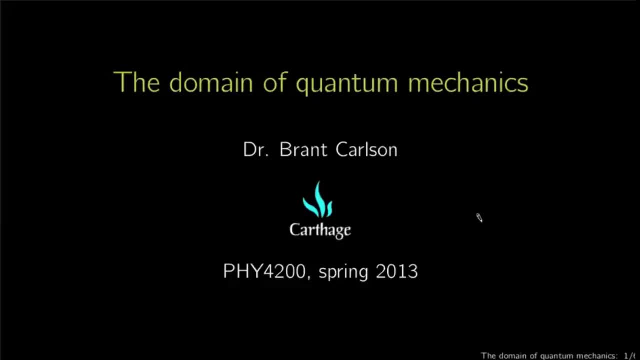 the interactions of light and matter, For instance in the context of the photoelectric effect or the black body radiation or bright line spectra of atoms and molecules, one might be led to the question of when is quantum mechanics actually relevant? The domain of quantum mechanics? 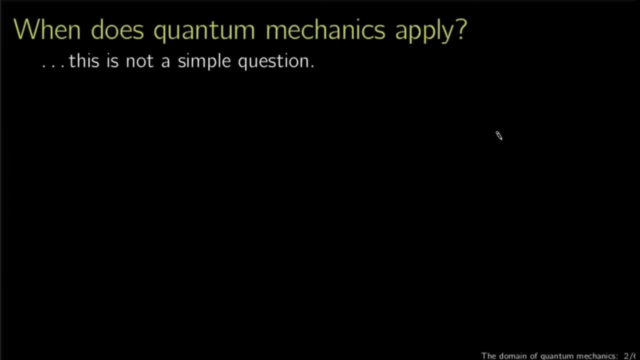 is unfortunately not a particularly simple question. When does it apply? Well, on the one hand, you have classical physics And on the other hand, you have quantum physics, And the boundary between them is not really all that clear On the classical side. 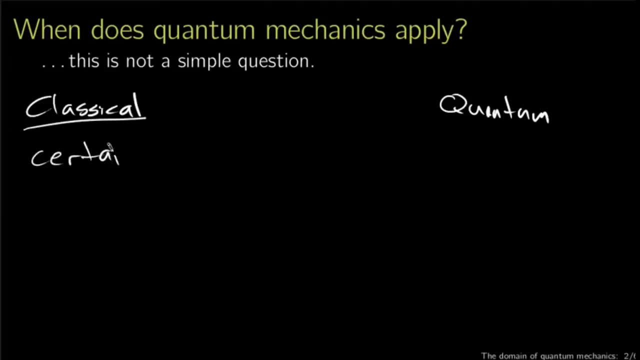 you have things that are certain, Whereas on the quantum side you have things that are uncertain. What that means in the context of physics is that on the classical side, things are predictable. They may be chaotic and difficult to predict, but in principle they can be predicted. 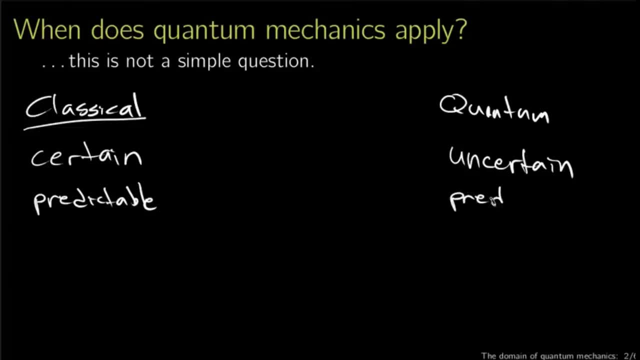 While on the quantum side, things are predictable too, But with a caveat, In the classical side you determine everything. Basically, every property of the system can be known with perfect precision, Whereas in quantum mechanics, what you predict are probabilities And learning to work with probabilities. 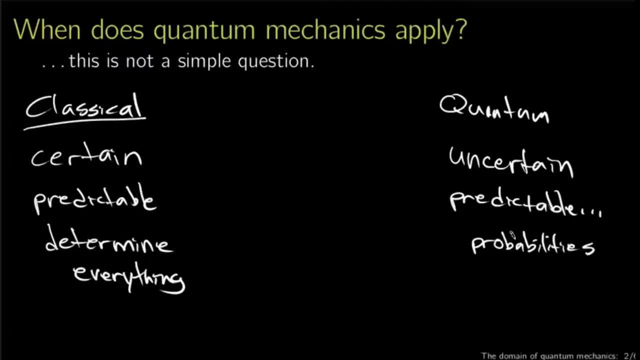 is going to be the first step to getting comfortable with quantum mechanics. The boundary between these two realms, when the uncertain and probabilistic effects of quantum mechanics start to become relevant, is really a dividing line between things that are large and things that are small. 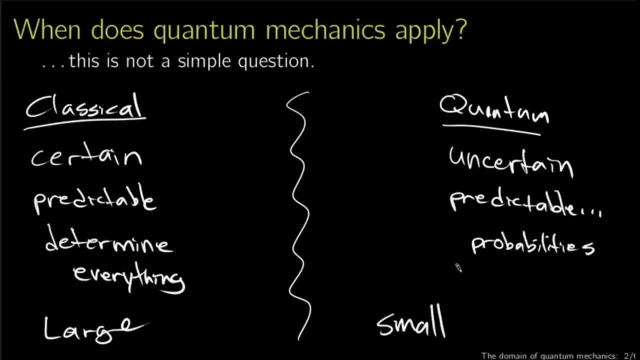 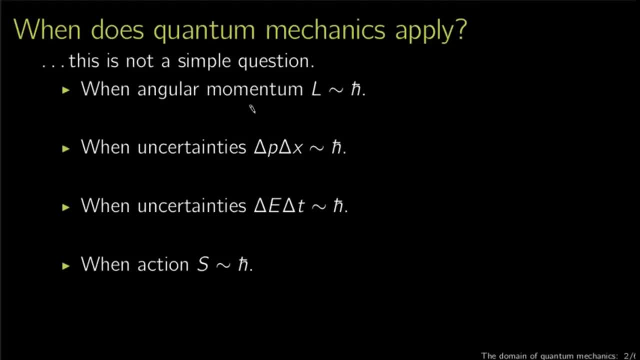 And that's not a particularly precise way of stating things, Doing things more mathematically. quantum mechanics applies, for instance, when angular momentum L is on the scale of Planck's constant or the reduced Planck's constant h-bar. 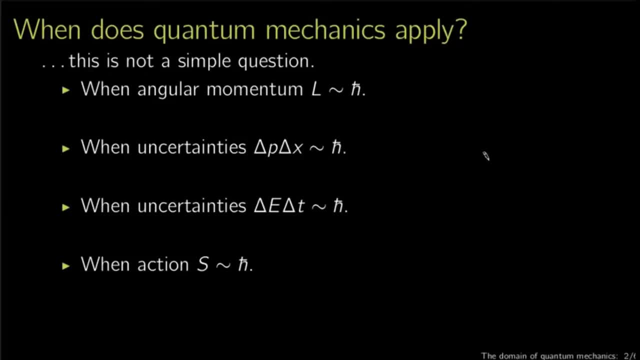 Now, h-bar is the fundamental scale of quantum mechanics And it appears not only in the context of angular momentum. Planck's constant has units of angular momentum, So if your angular momentum is of order Planck's constant or smaller, you're in the domain of quantum mechanics. 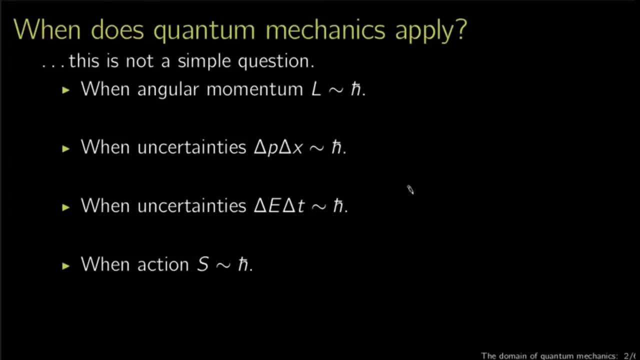 We'll learn more about uncertainty principles later as well. Uncertainties in this context have to do with products of uncertainties, For instance the uncertainty in the momentum of a particle times, the uncertainty in the position of the particle- This if it's comparable to Planck's constant. 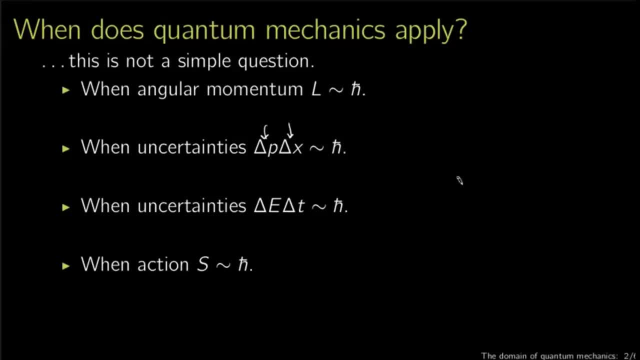 is also going to give you the realm of quantum mechanics. Energy and time also have an uncertainty relation, again approximately equal to Planck's constant. Most fundamentally, the classical action. When you get into more advanced studies of classical mechanics you'll learn about a quantity called the action. 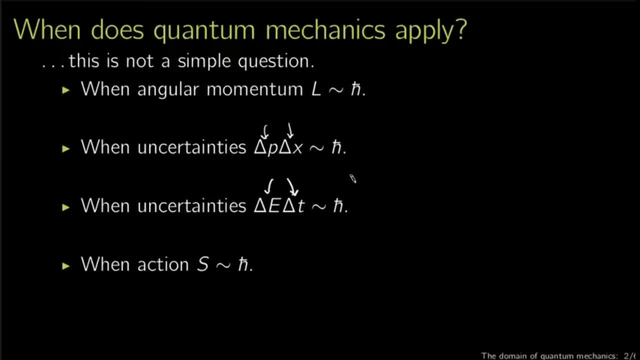 which has to do with the path a system takes as it evolves in space and time. If the action of the system is of order Planck's constant, then you're in the quantum mechanical domain. Now, Planck's constant is a really small number. 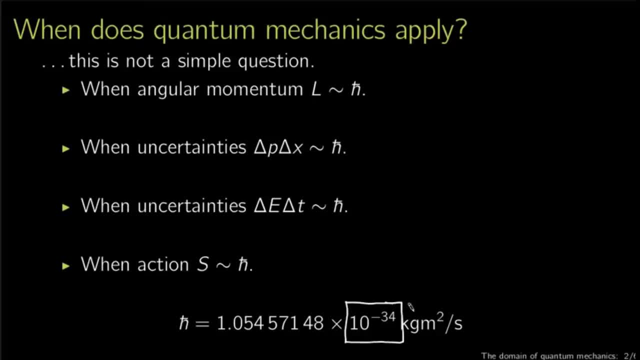 It's 1.05 times 10 to the negative 34 kilogram meters squared per second. Times 10 to the negative 34 is a small number. So if we have really small numbers, then we're in the domain of quantum mechanics. 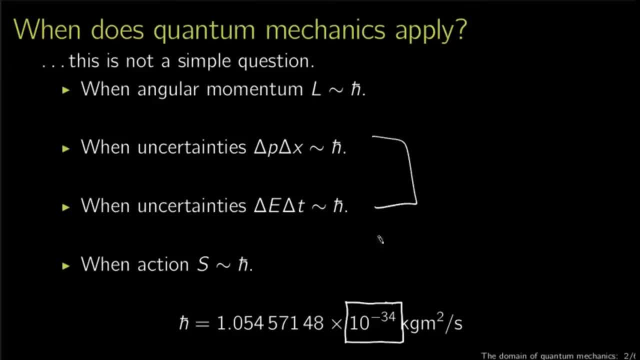 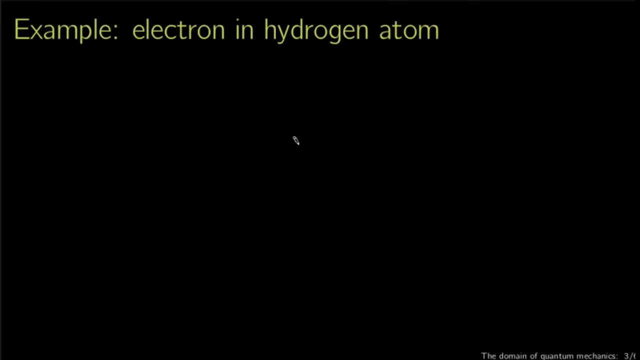 In practice, these guys are the most useful, whereas this is the most fundamental. But we're more interested in useful things than we are in fundamental things. after all, For example, the electron in the hydrogen atom. Now, you know from looking at the bright line spectra. 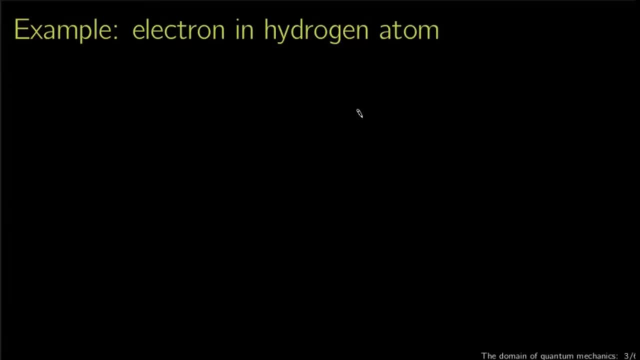 that this should be in the domain of quantum mechanics. But how can we tell? Well, to use one of the uncertainty principles as a calculation. consider the energy. The energy of an electron in a hydrogen atom is you know? let's say: 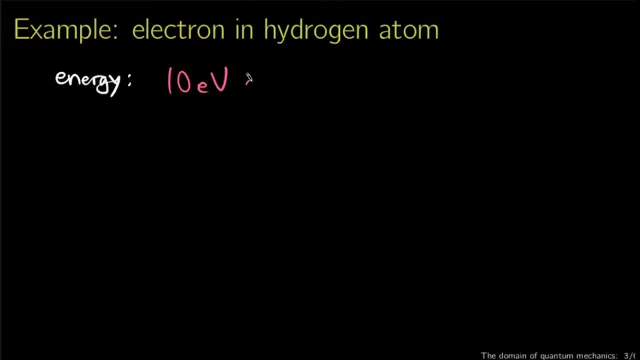 about 10 electron volts. If we say that's p squared over 2m, using the classical kinetic energy relation between momentum and kinetic energy, that tells us that the momentum p is going to be about 1.7 times 10 to the minus 24th. 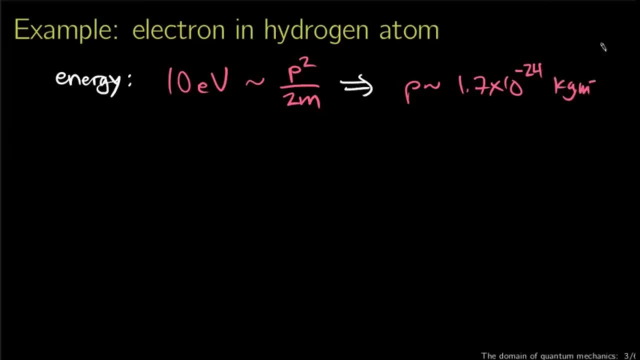 kilogram meters- sorry, kilogram, where'd it go? where's my eraser? Kilogram meters per second? Now, this suggests that the momentum of the electron is, you know, non-zero. But if the hydrogen atom itself is not moving, 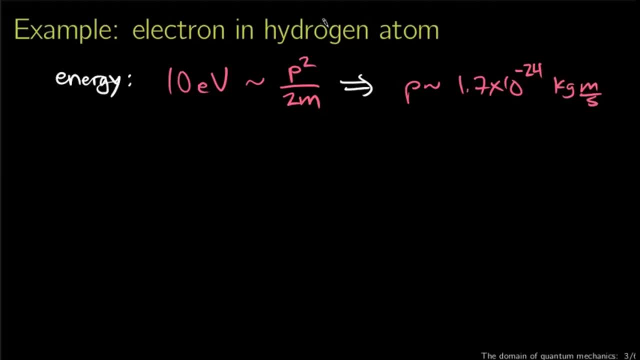 we know, the average momentum of the electron is zero. So if the momentum of the electron is going to be zero, with still some momentum being given to the electron, this is more the uncertainty in the electron momentum than the electron momentum itself. The next quantity, if we're looking at the electron. 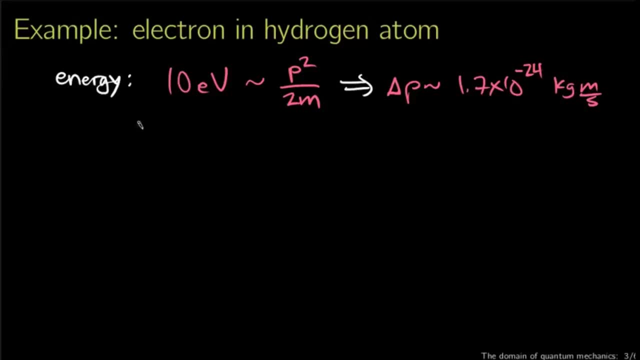 if we're looking at the uncertainty relation between momentum and position, is we need to know the size of, or the uncertainty in the position of the electron, which has to do with the size of the atom. Now, the size of the atom. 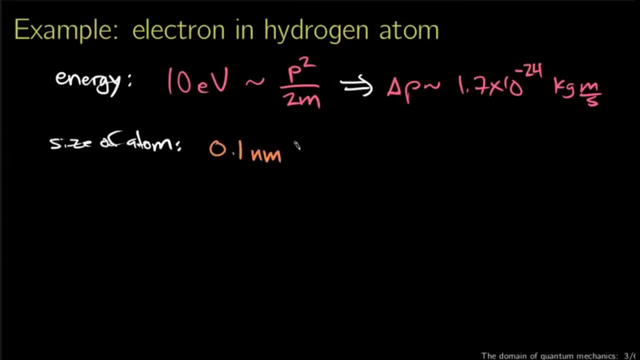 that's about 0.1 nanometers, which, if you don't remember, the conversion from nanometers is 10 to the minus 10th meters. So let's treat this as delta x: our uncertainty in position, Because we don't really know where the electron is within the atom. 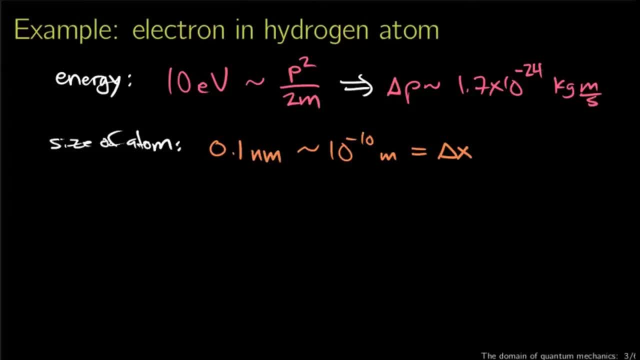 so this is a reasonable guess at the uncertainty. Now, if we calculate these two things together, delta p, delta x, you get something- and I should say this is approximate, because this is very approximate- 1.7 times 10- to the negative 34th. 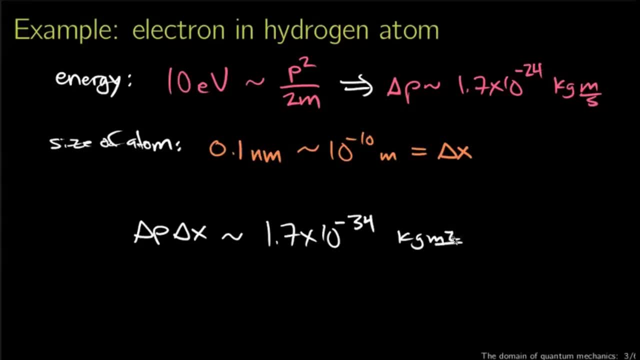 And if you plug through the units, it's kilogram meters squared per second. This is about equal to h-bar. So this tells us that quantum mechanics is definitely important here. We have to do some quantum in order to understand this system. As an example of another small object: 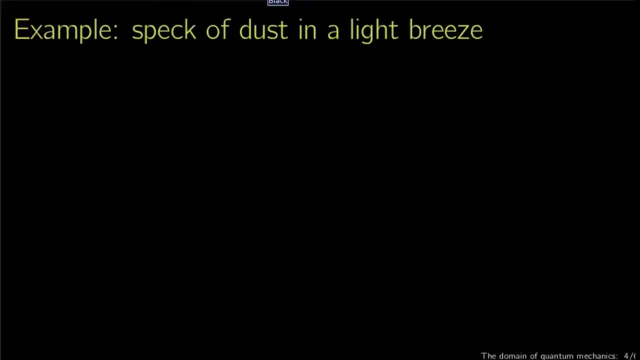 that might have quantum mechanics relevant to it. this is one that we would actually have to do a calculation. I don't know intuitively whether a speck of dust in a light breeze is in the realm of quantum mechanics or classical physics. Now I went online and looked up some numbers. 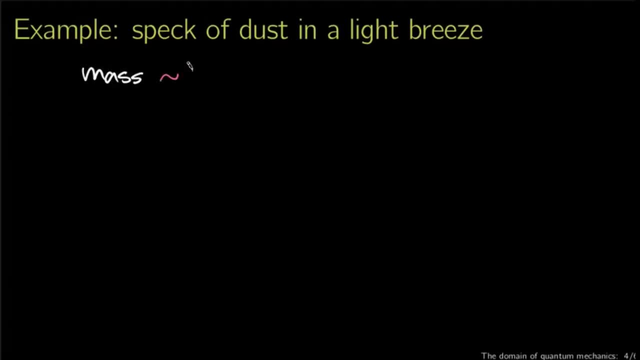 For a speck of dust, let's say the mass is about 10 to the minus 6th kilograms. a microgram. It has a velocity in this light breeze of, let's say, 1 meter per second, And let me make myself some more space here. 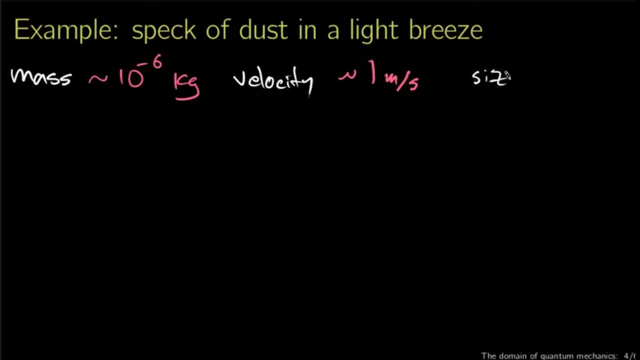 The size of this speck of dust is going to be about 10 to the minus 5 meters. So these are the basic parameters of this speck of dust in a light breeze. Now we can do some calculations with this, For instance momentum. 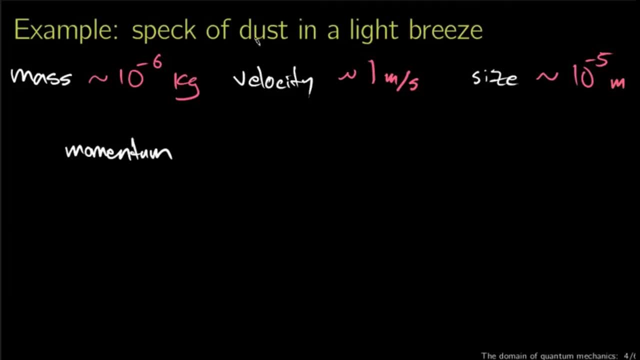 Well, the momentum is just the mass times, the velocity. So p is going to be about equal to, equal to 10 to the minus 9 kilogram meters per second. Better make that 10 to the minus 6th kilogram meters per second. 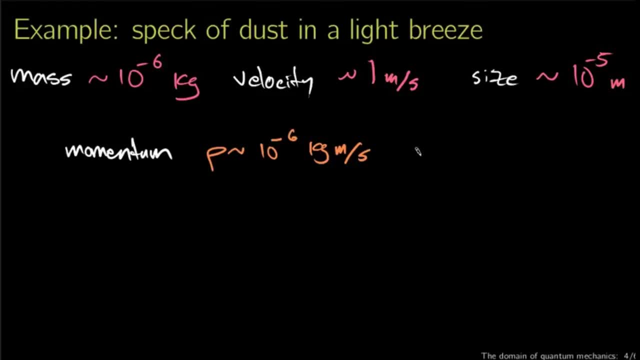 My notes are backwards here. The uncertainty in the momentum, then, is we could say it's 10 to the minus 6th kilograms meters per second, but let's say it's a little smaller than 10 to the minus 6th kilograms meters per second. 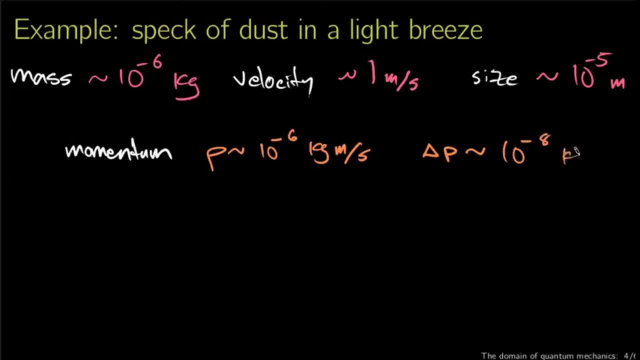 Let's say 10 to the minus 8 kilogram meters per second. Now the position uncertainty. that's going to be a function of the size of the object. If we know the size of the object, the position uncertainty is probably not all that much. 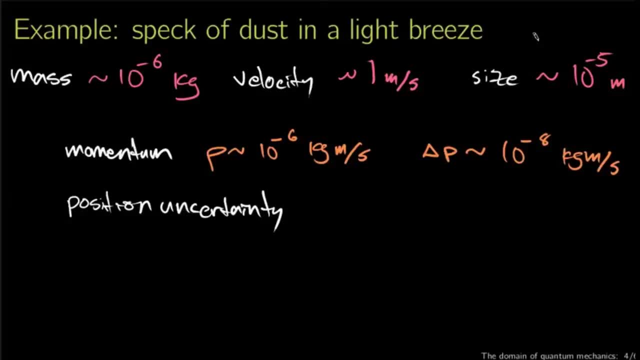 larger than the size of the object. In fact it's probably smaller. We can measure where a speck of dust is to better than the diameter of the speck of dust just by putting it in a microscope, for example. So let's say the position uncertainty here. 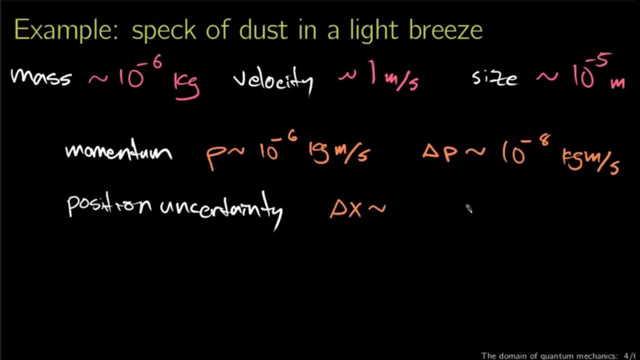 is going to be about 10 to the minus 6th meters. Now, if we run that calculation, delta P, delta X comes out to be 10 to the 6th times 10 to the minus 8th, which is 10 to the minus 14th kilogram meters squared per second. 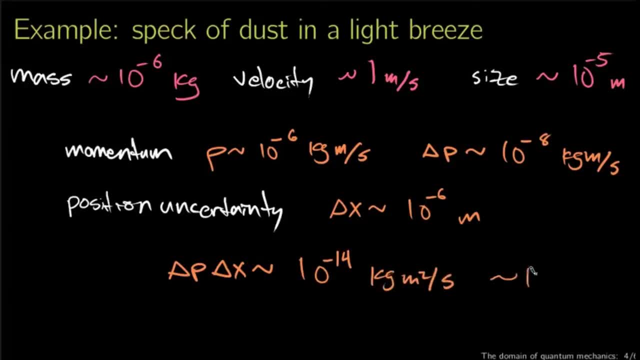 This is a good factor of 10 to the 20th, larger than h-bar. So this is solidly in the realm of classical physics. So even something really small like a speck of dust in a light breeze is still going to be classical. 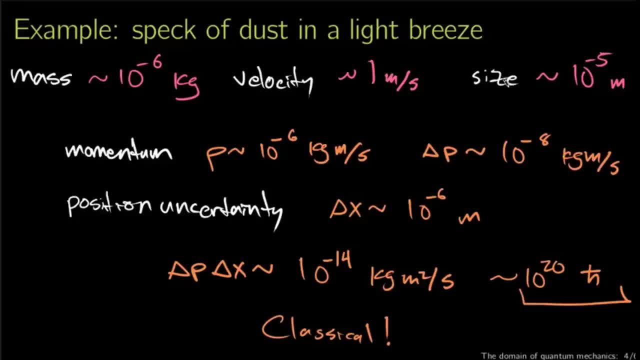 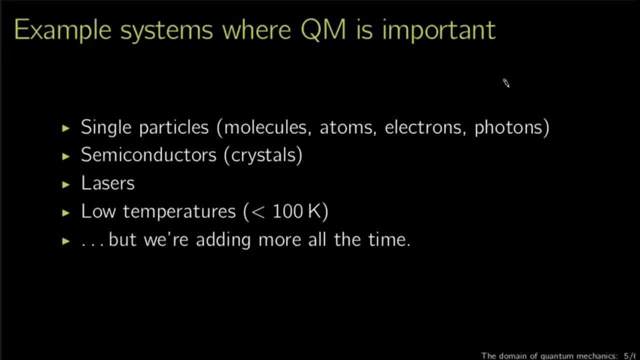 So the size of something here, the smallness of it, is something that you might have to calculate until you start getting a feel for it. Just some basic examples. to put things in context a little further, Quantum mechanics is most likely going to be important. 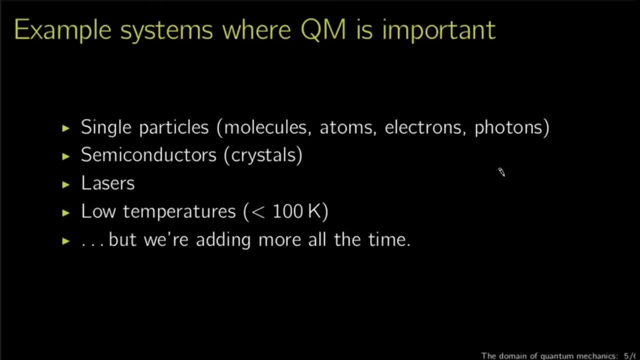 if you're dealing with single particles, atoms, molecules, single electrons, single photons, small systems of electrons and photons. It's also going to be very, very relevant if you're talking about semiconductors: The quantum mechanical properties of semiconductors. 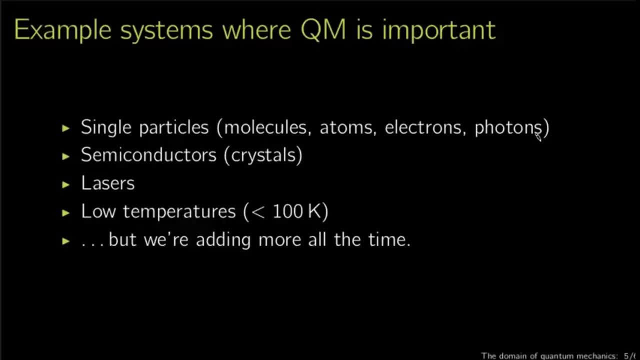 are what makes them into such spectacularly useful electronic devices. Lasers are another situation where quantum mechanics is crucially important. Without quantum mechanics, there would be no lasers. And finally, if you're talking about very low temperature, physics temperatures less than about 100 Kelvin. 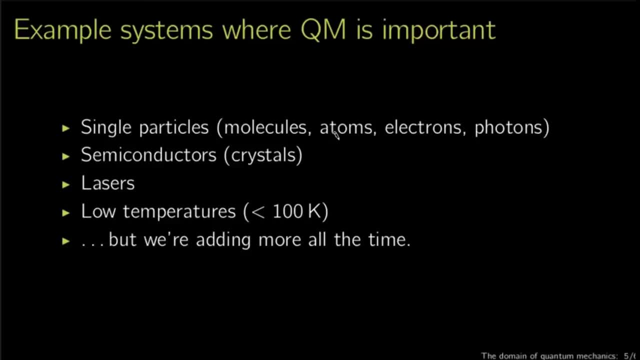 well, those are going to be quantum mechanical as well. So single particles, weird materials, crystals, lasers, low temperatures- they're kind of an exotic set of phenomena, but we're adding more all the time. Quantum mechanics allows us to do things that we wouldn't be able to do. 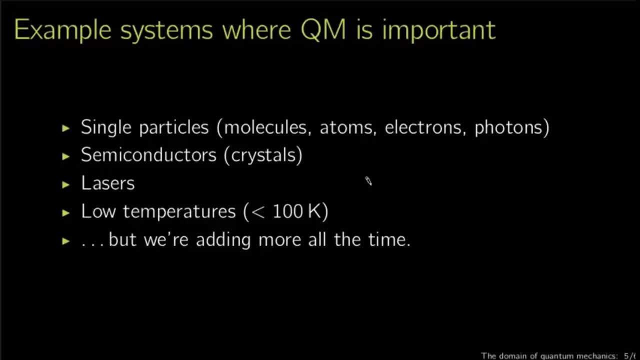 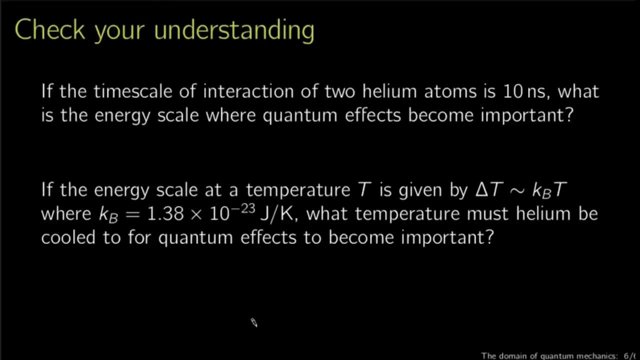 in the classical world. Consequently, it's in our best interest to try and push quantum mechanics as far as we can take it. So to check your understanding, this is a short question about the uncertainty in the relevant parameters of interaction between two helium atoms. 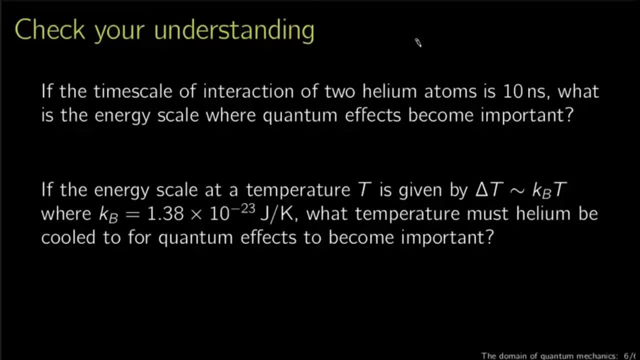 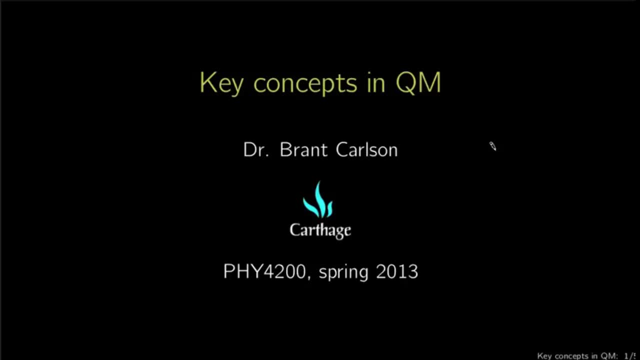 and what temperature scale these interactions become important or become quantum mechanical at. In order to understand quantum mechanics, there's some basic vocabulary that I need to go over, So let's talk about the key concepts in quantum mechanics. Thankfully, there are only a few. 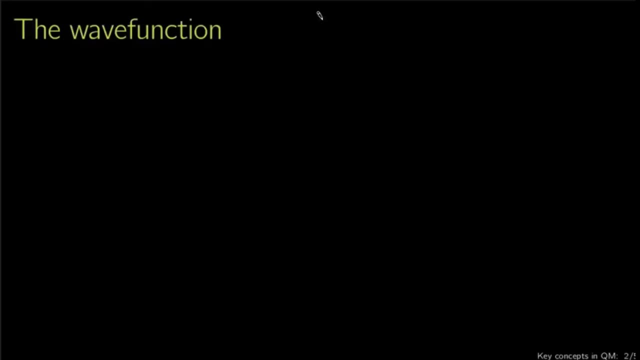 There's really only three, And the first is the wave function. The wave function is, and always has been, written as psi, the Greek letter. My handwriting gets a little lazy sometimes and it'll end up just looking like this, but technically it's supposed to look something like that. 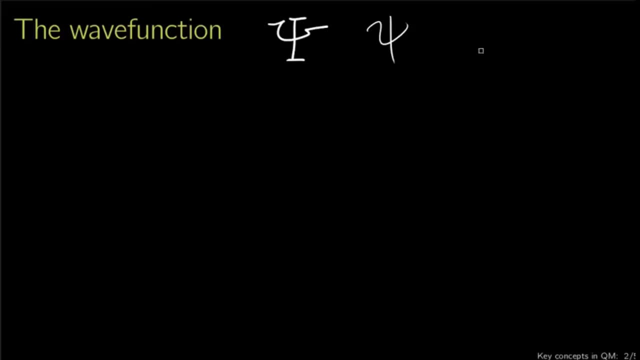 Details are important, provided you recognize the symbol. Psi is a function of position, potentially in three dimensions: x, y and z, and time, And the key facts here is that psi is a complex function, which means that while x, y, z and t here are real numbers, 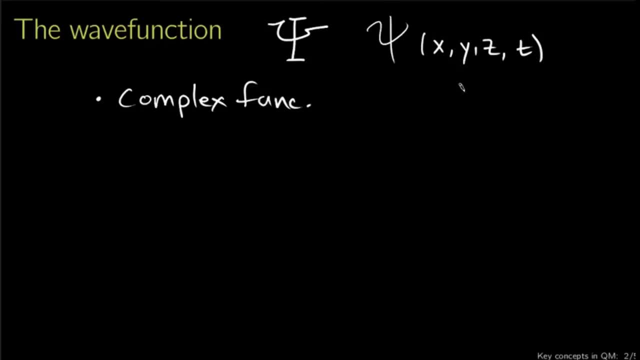 psi, evaluated at a particular point in space, will potentially be a complex number, with both real and imaginary part. What is subtle about the wave function- and we'll talk about this in great detail later- is that, while it represents the state of the system, 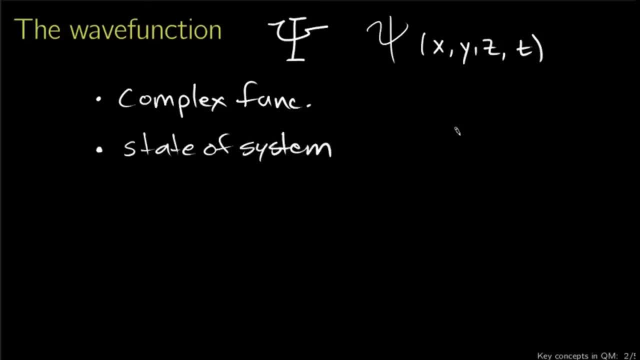 it doesn't tell you with any certainty what the observable properties of the system are. It really only gives you probabilities. So, for instance, if I have a coordinate system something like this, where, say, this is position in this direction? 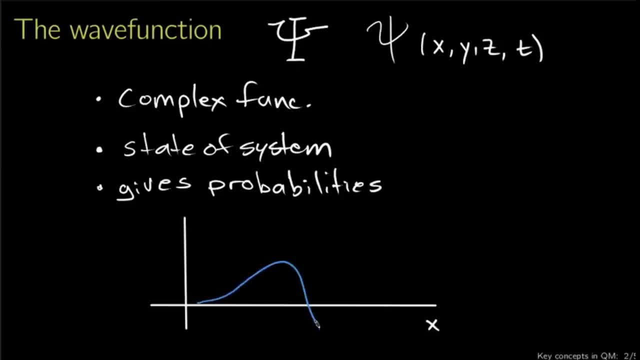 psi, with both real and imaginary parts, might look something like this: This could be the real part of psi and this could be, say, the complex or the imaginary part of psi. What is physically meaningful is the squared magnitude of psi. 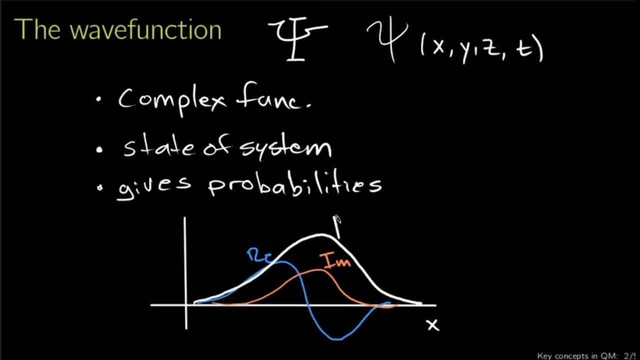 which might look something like this in this particular case, And that is related to the probability of finding the particle at a particular point in space. As I said, we'll talk about this later, but the key facts that you need to know about the wave function is that it's complex. 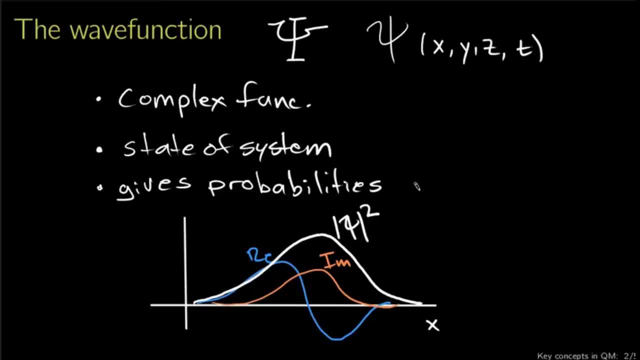 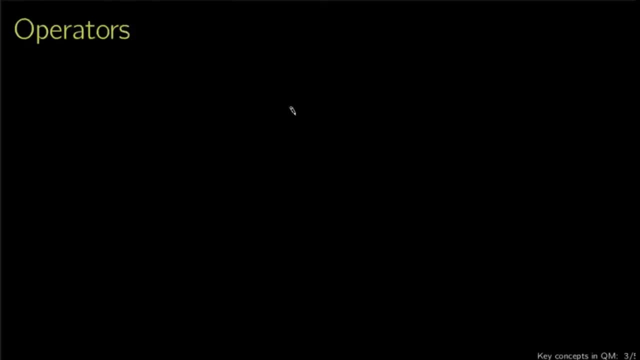 and it describes the state of the system, but not with certainty. The next key concept in quantum mechanics is that of an operator. Now, operators are what connect psi to observable quantities. That is one thing operators can do. Just a bit of notation. 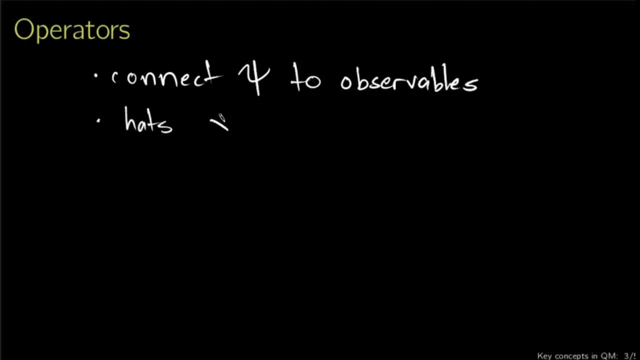 usually we use hats for operators. For instance, x-hat or p-hat are operators that you'll encounter shortly. Operators act on psi, So if you want to apply, for instance, the x-hat operator to psi, you would write x-hat, psi. 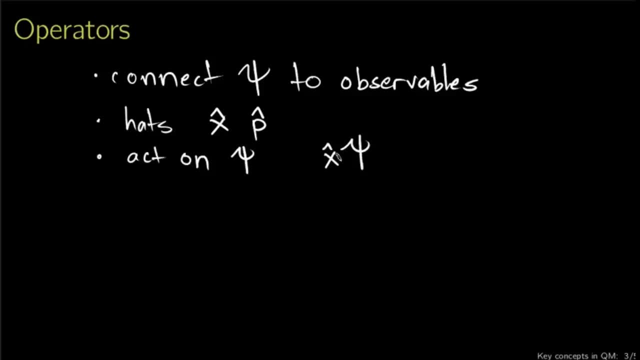 As it appears on the left of psi. the assumption is that x acts on psi. If I write psi x-hat, it doesn't necessarily mean that x-hat acts on psi. You assume operators act on whatever lies to the right. Likewise, of course, p-hat psi. 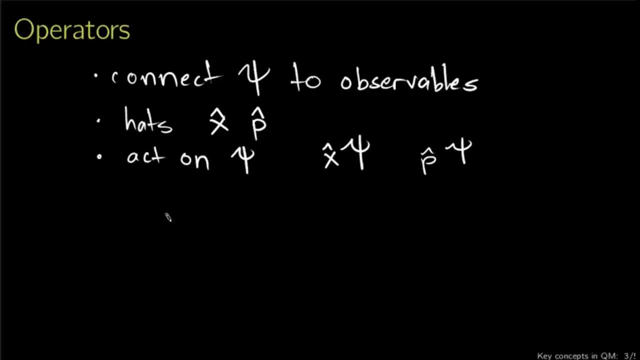 Now we'll talk about this in more detail later- but x-hat the operator can be thought of as just multiplying by x. So if I have psi as a function of x, x-hat psi is just going to be x times psi of x. 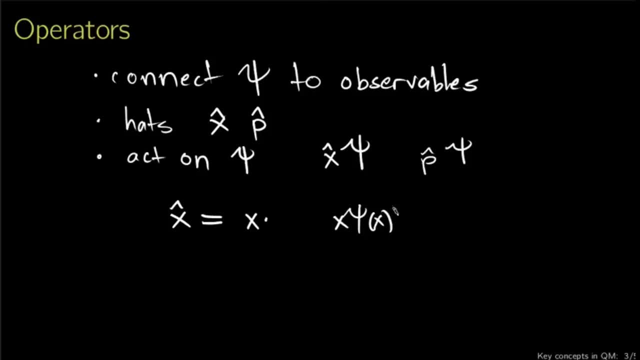 So if psi was a polynomial, you could multiply x by that polynomial. The p-operator, p-hat, is another example. It's a little bit more complicated. This is just an example now and technically this is the momentum operator, but we'll talk more about that later. 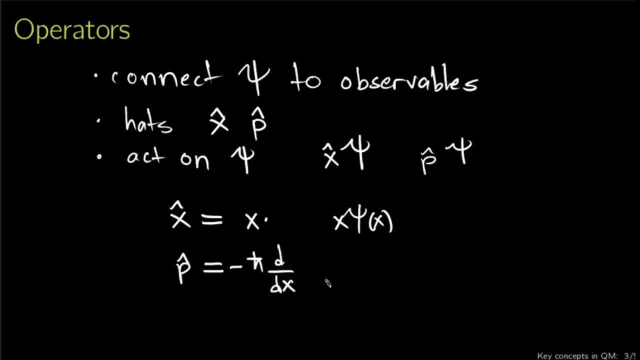 So p-bar times the derivative with respect to x. So this is again something that needs a function, needs the wave function to actually give you anything meaningful. Now, the important thing to note about the operators is that they don't give you the observable quantities either. 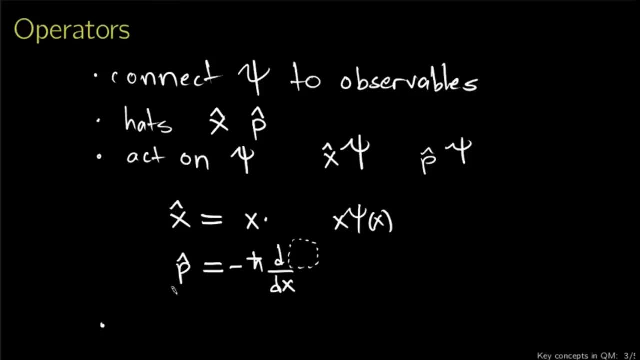 But in quantum mechanics you can't really say the momentum of the wave function, For instance, p-hat psi is not- and I'll put this in quotes because you won't hear this phrase very often- the momentum of psi. It's the momentum operator acting on psi. 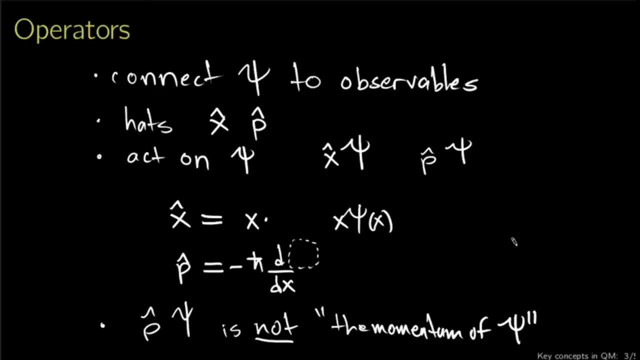 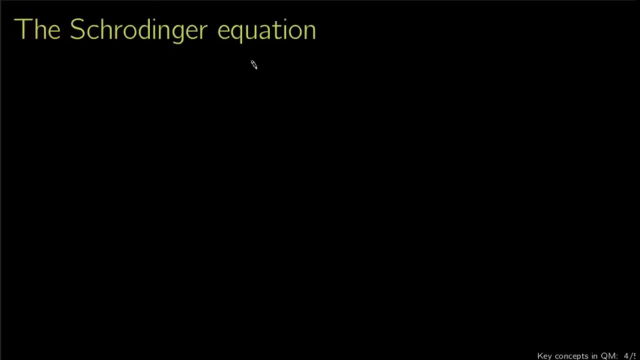 and that's not the same thing as the momentum of psi. The final key concept in quantum mechanics is the Schrodinger equation, And this is really the big equation, So I'll write it big. I h-bar partial derivative of psi with respect to time. 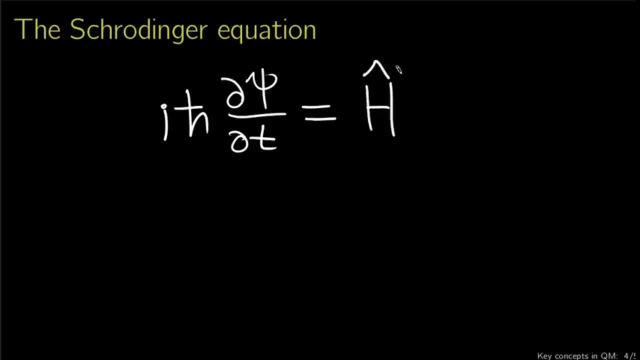 is equal to h-hat, that's an operator acting on psi. Now h-hat here is the Hamiltonian, which you can think of as the energy operator. So the property of the physical system that h is associated with is the energy of the system. 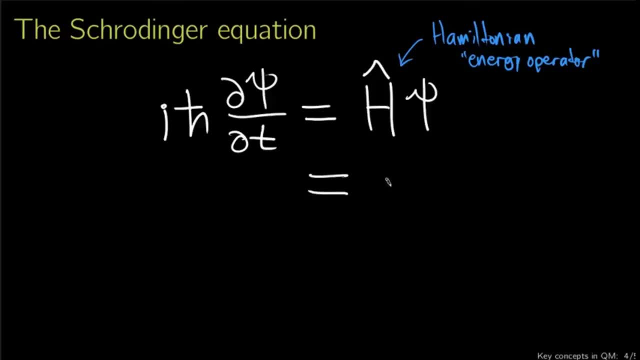 And the energy of the system can be thought of as a kinetic energy. So we can write a kinetic energy operator plus a potential energy operator together acting on psi, And it turns out the kinetic energy operator can be written down. This is going to end up looking like: 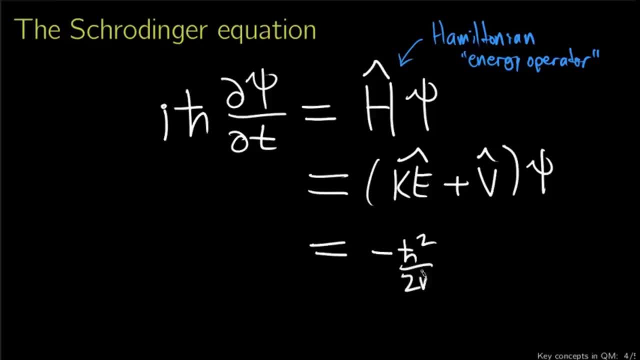 minus h-bar, squared over 2m. partial derivative of psi with respect to- sorry. second partial derivative of psi with respect to position Plus. and then the potential energy operator is going to look like the potential energy is a function of position, just multiplied by psi. 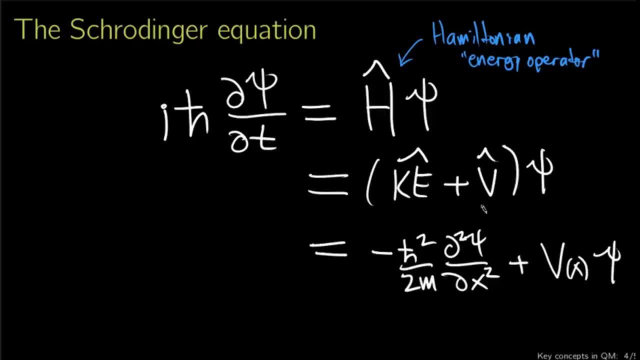 So this is the Schrodinger equation. Typically you'll be working with it in this form. So i: h-bar times. the partial derivative with respect to time is related to the partial derivative with respect to space and then multiplied by some function, The basic quantum mechanics. 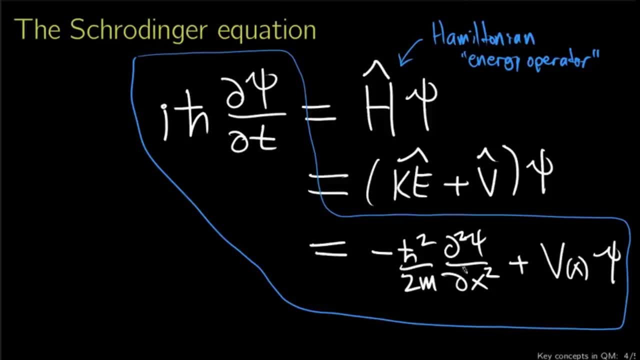 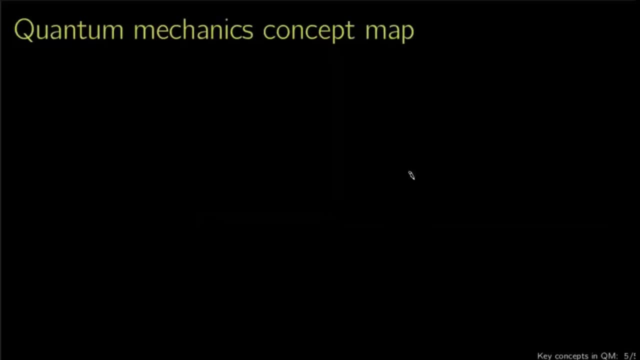 that we're going to learn in this course mostly revolves around solving this function and interpreting the results. So to put these in a bit of a road map, we have operators, We have the Schrodinger equation and we have the wave function. 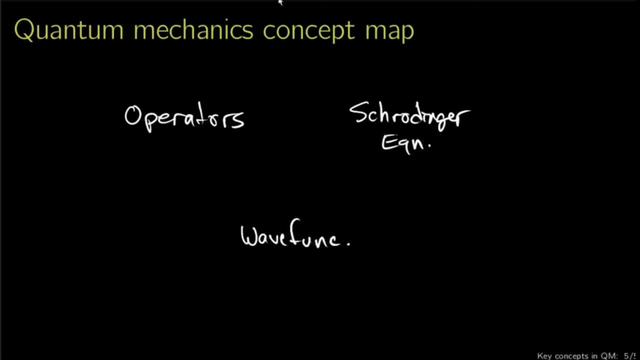 Now operators act on the wave function and operators are used in the Schrodinger equation. Now the wave function that actually describes the state of the system is going to be the solution. It's going to be the solution to the Schrodinger equation. 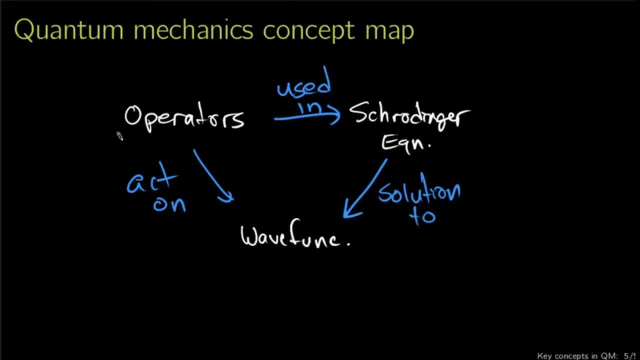 Now I mentioned operators acting on the wave function. What they give you when they act on the wave function is some property of the system, Some observable perhaps. And the other key fact that I mentioned so far is that the wave function doesn't describe the system perfectly. 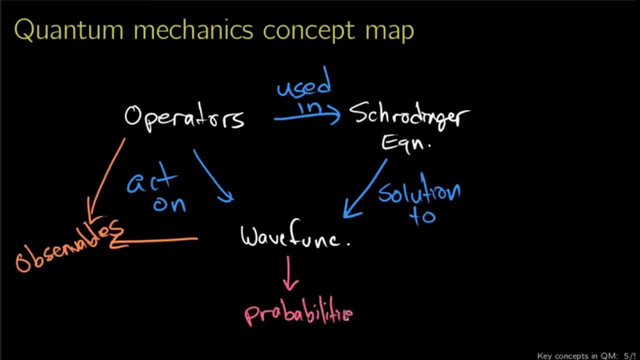 It only gives you probabilities. So that's our overall concept map. To put this in the context of the course outline, the probabilities are really the key feature of quantum mechanics And we're going to start this course with a discussion of probabilities. We'll talk about the wave function after that. 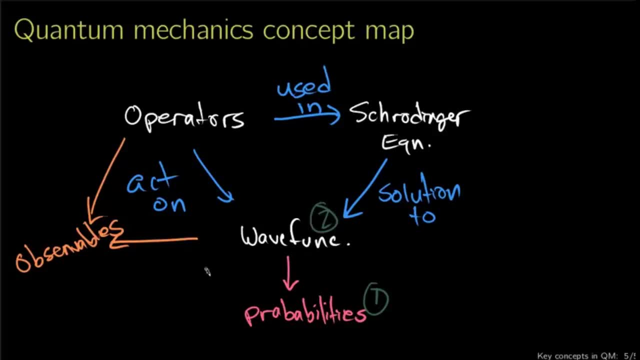 and how the wave function is related to those probabilities. And we'll end up talking about operators and how those operators and the wave functions together give you probabilities associated with observable quantities. That will lead us into a discussion of the Schrodinger equation, which will be most of the course really. 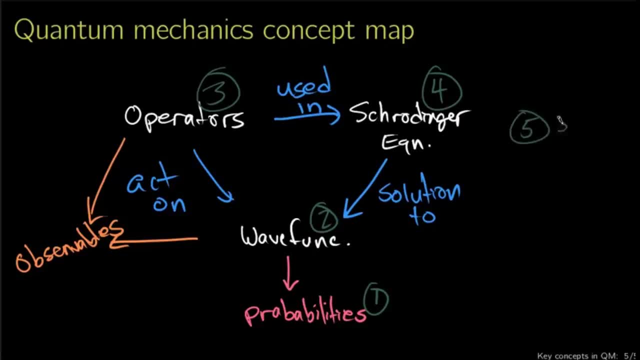 The bulk of the material before the first exam will be concerned with various examples Solution to the Schrodinger equation under various circumstances. This is really the main meat of quantum mechanics in the beginning. After that we'll do some formalism, And what that means is we'll learn. 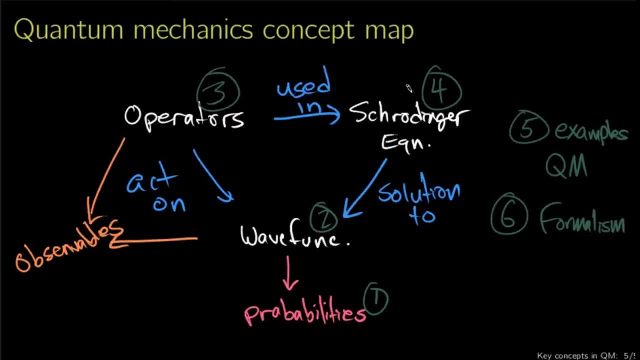 about some advanced formulas and advanced mathematical tools that make keeping track of all the details of how all of this fits together a lot more straightforward, And then we'll finish up the course by doing some applications. So those are our key concepts and a general roadmap through the course. 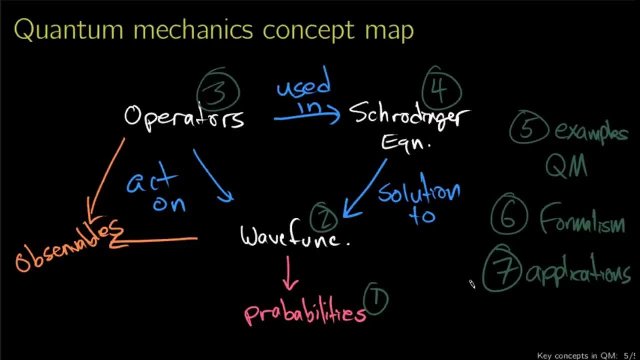 Hopefully now you have the basic vocabulary necessary to understand phrases like the momentum operator acts on the wave function or the solution to the Schrodinger equation describes the state of the system and that sort of thing. Don't worry too much if these concepts haven't quite clicked. 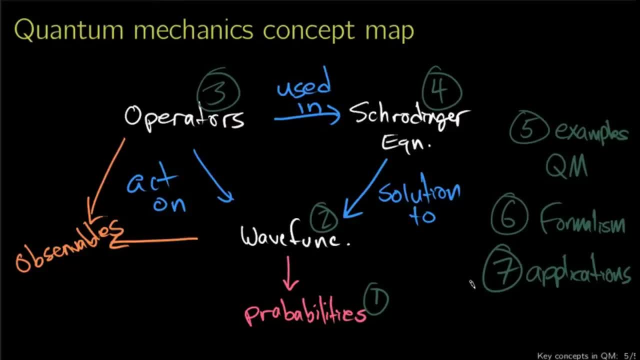 In order to really understand quantum mechanics, you have to get experience with them. These are not things that you really have any intuition for based on anything you've seen in physics so far. So bear with me and this will all make sense in the end, I promise. 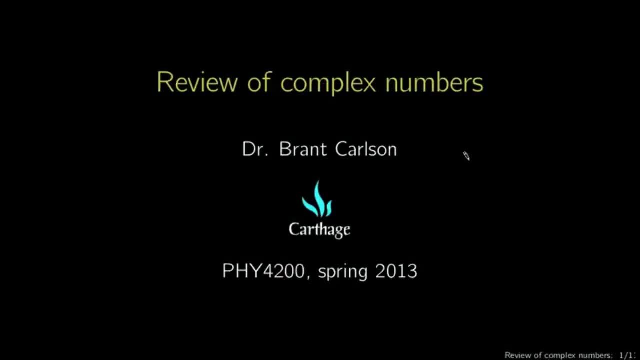 Complex numbers or numbers involving conceptually- you can think about it as the square root of negative 1, i are essential to understanding quantum mechanics, Since some of the most fundamental concepts in quantum mechanics, for instance the wave function, are expressed in terms of complex numbers. 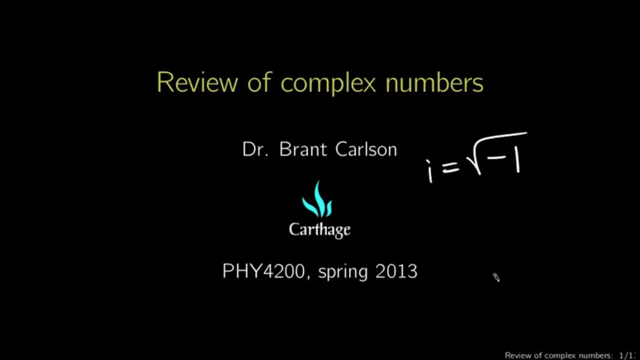 Complex analysis is also one of the most beautiful subjects in all of mathematics, but unfortunately in this course I don't have the time to go into the details. Lucky you, perhaps. Here's what I think you absolutely need to know to understand quantum mechanics from the perspective of complex analysis. 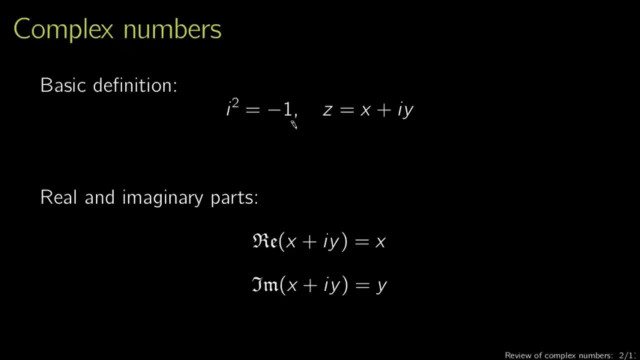 First of all, there's basic definition: i squared is equal to negative 1, which you can think of also as i equals the square root of negative 1.. In general, a complex number, z, then, can be written as the sum of: 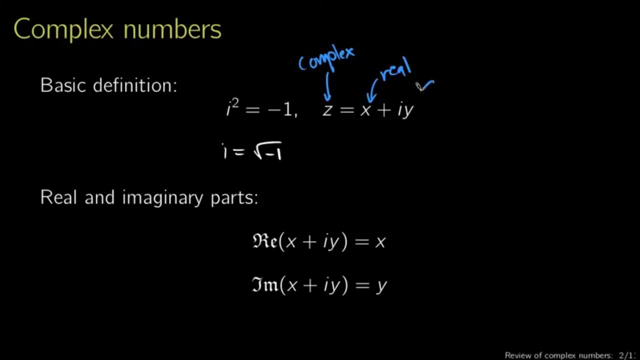 a purely real part, x, and a purely imaginary part. i times y. Note in this expression z is complex, x and y are real. where i times, y is purely imaginary. The terms purely real or purely imaginary in the context of this expression like this: 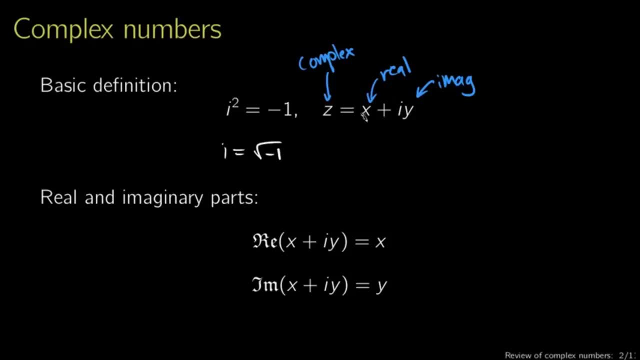 x plus i y. something is purely real if y is 0,. something is purely imaginary if x is 0.. As far as some notation for extracting the real and imaginary parts, typically mathematicians will use this funny calligraphic font to indicate the real part of x plus i y. 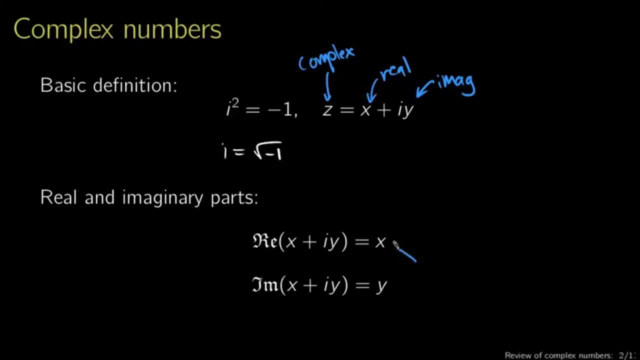 or the imaginary part of x plus i, y, and that just pulls out x and y. Note that both of these are real numbers. When you pull out the imaginary part, you get x and y. You don't get i, y, for instance. 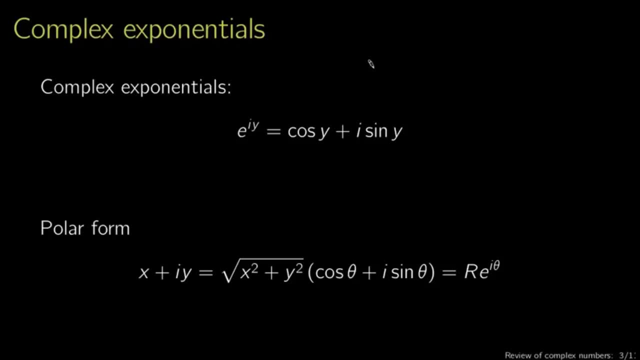 Another one of the most beautiful results in mathematics is e to the i. pi plus 1 equals 0. This formula kind of astonished me when I first encountered it, but it is a logical extension of this more general formula that e raised to a purely imaginary power, i y. 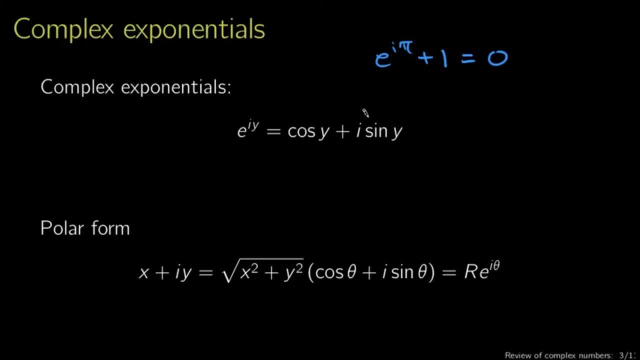 is equal to the cosine of y plus i times the sine of y. This can be shown in a variety of ways, in particular involving the Taylor series, If you know, the Taylor series for the exponential, the Taylor series for cosine of y and the Taylor series for sine of y. 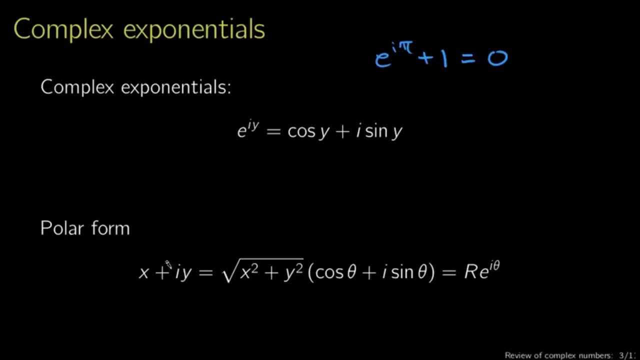 you can show quite readily that the Taylor series for complex exponential is the Taylor series of cosine plus the Taylor series of sine, And while that might not necessarily constitute a rigorous proof, it's really quite fun if you get the chance to go through it. 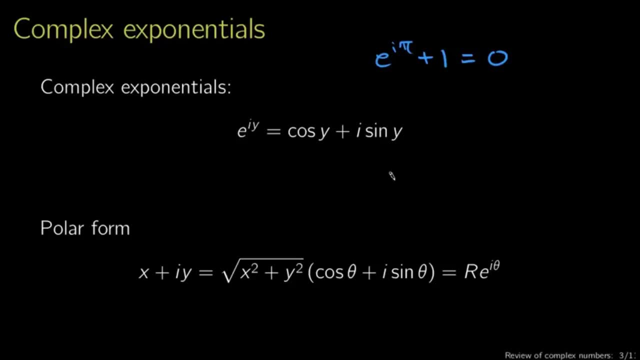 At any rate, the trigonometric functions, here cosine and sine, should be suggestive, and there is a geometric interpretation of complex numbers that we'll come back to in a minute. But for now, know that while we have rectangular forms like this: 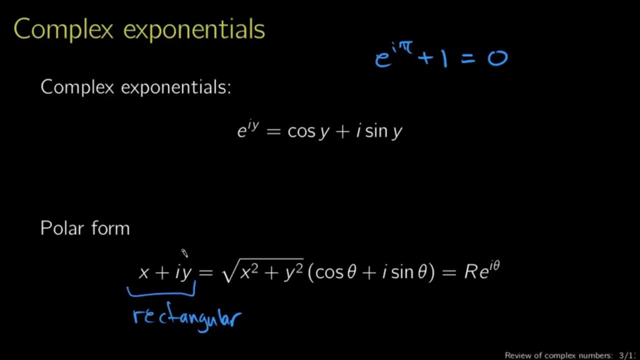 x plus i, y, where x and y- the nomenclature there- is chosen on purpose. you can also express this in terms of r? e to the i theta, where you have now a radius and an angle- The angle here, by the way. 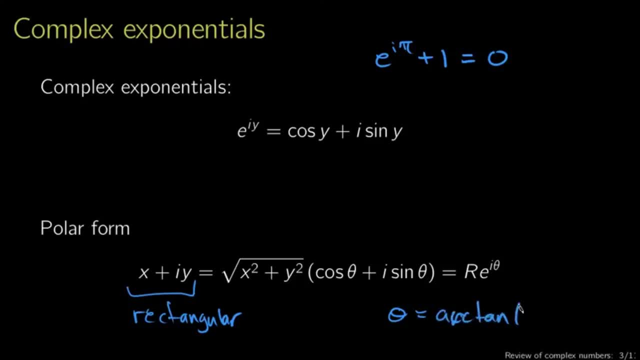 is going to be the arc tangent of y over x, And we'll see why that is in a moment when we talk about the geometric interpretation. But given these rectangular and polar forms of complex numbers, what do the basic operations look like? How do we manipulate these things? 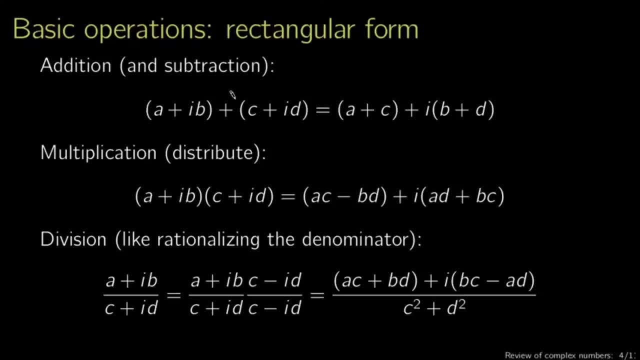 Well, addition and subtraction in rectangular form is straightforward. If we have two complex numbers- a plus i, b plus- and we want to add to that this complex number c plus i, d, we just add the real parts a and c. 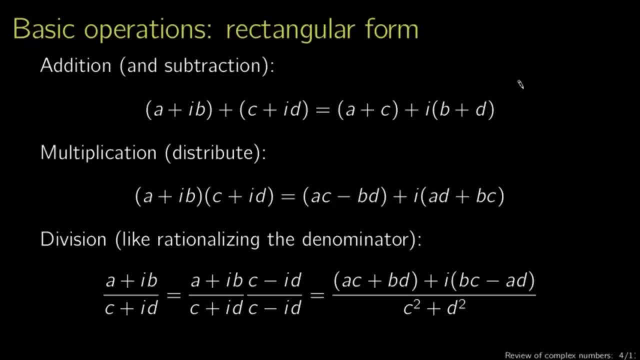 and we add the imaginary parts b and d. This is just like adding in any other sort of algebraic expression. Multiplication is a little bit more complicated. You have to distribute, and you distribute in the usual sort of draw a smiley face kind of way. 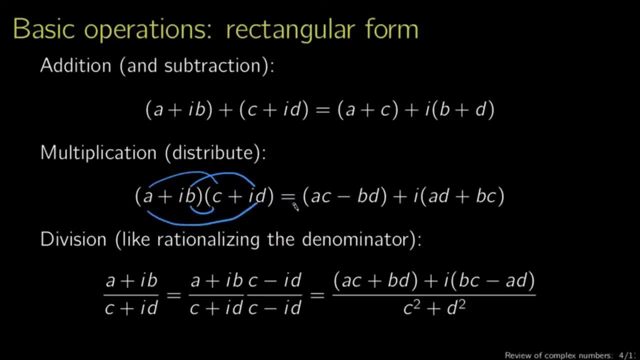 a times c and b times d are going to end up together in the real part, And the reason for that is well, a times c, a and c both being real numbers. a times c will be real, Whereas i, b times i d. 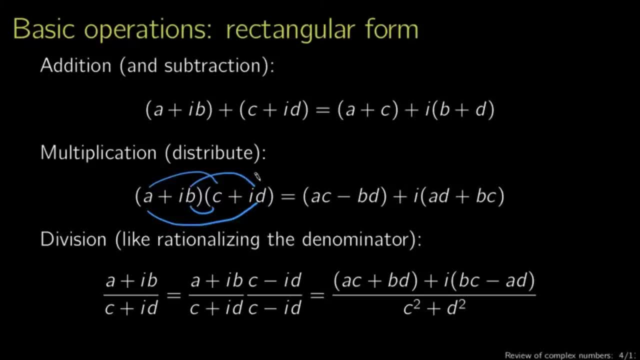 both being purely complex numbers, you'll end up with b times d times i squared, and i squared is minus 1.. So you just end up with minus bd, which is what we see here. Otherwise, the complex part is perhaps a little more easy to understand. 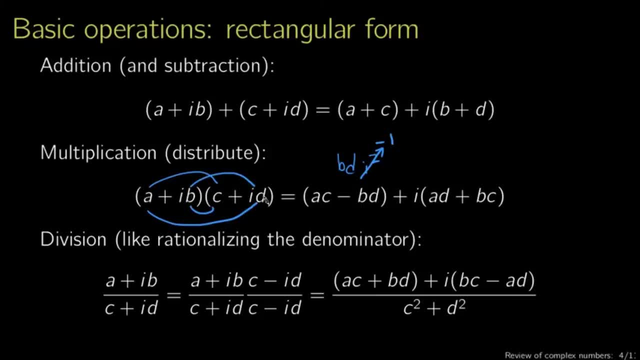 You have i times b times c, and you have a times i times d, both of which end up with plus signs in the complex part. Division in this case is like rationalizing the denominator, except instead of involving radicals, you have complex numbers. 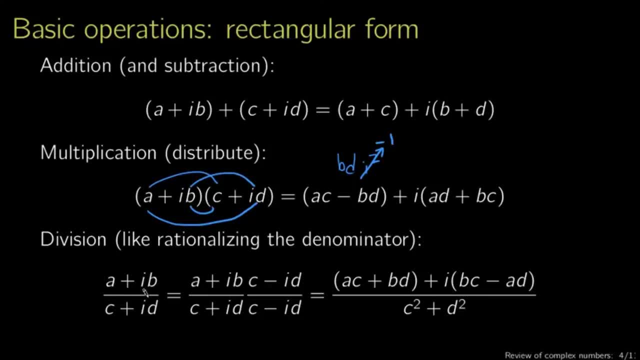 If I have some number, a plus i b- divided by c plus i d, I can simplify this by both multiplying and dividing by c minus i d. Note the sign change in the denominator here. c plus i d is then prompting me to multiply by c minus i d over c minus i d. 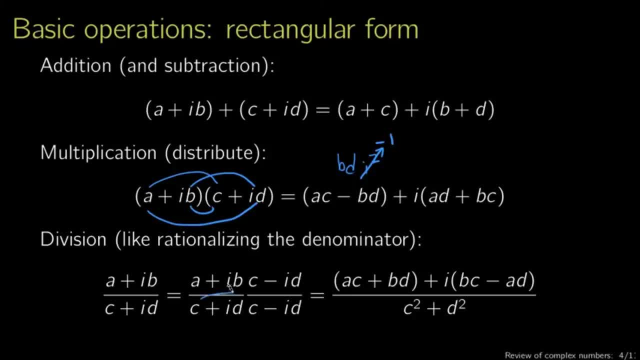 Now, when you do the distribution there, for instance, let's just do it in the denominator c plus i d times c minus i d. my top eyebrows here of the smiley face: c squared minus sorry, c squared times i d. 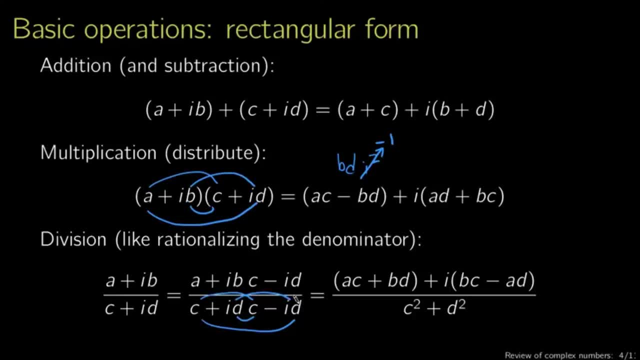 c squared plus now i d times minus i d, which is. well, I'll just write it out: i times minus i d, which is going to be d squared times i times minus i. so i squared times minus 1,. 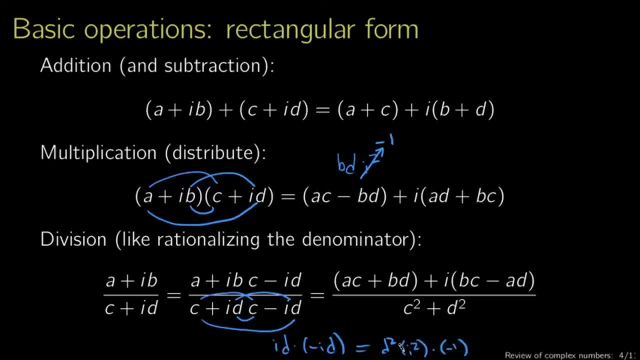 and i squared is minus 1.. So I have minus 1 times minus 1,, which is just 1, so I can ignore that. I've just got d squared. So what I end up with in the denominator is just c squared plus d squared. 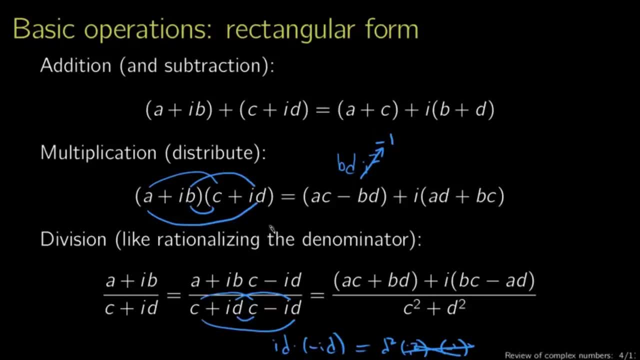 What I end up with in the numerator. well, that's the same sort of multiplication thing that we just discussed. So the simplified form of this has no complex part in the denominator, which helps keep things simple. It's always a little simple and a little easier to interpret. 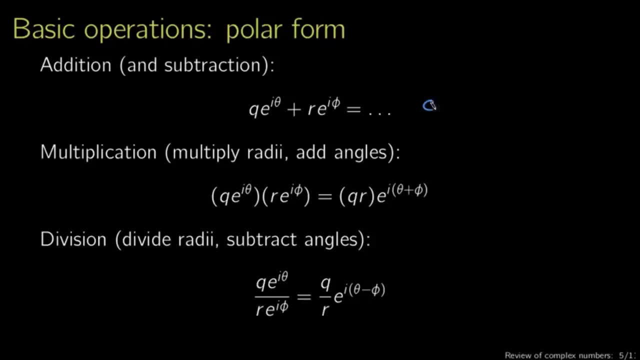 Now in polar form: addition and subtraction. well, they're complicated Under most circumstances. if you have two complex numbers given in polar form, it's easiest just to convert to rectangular form and add them together there- Multiplication and division, though. 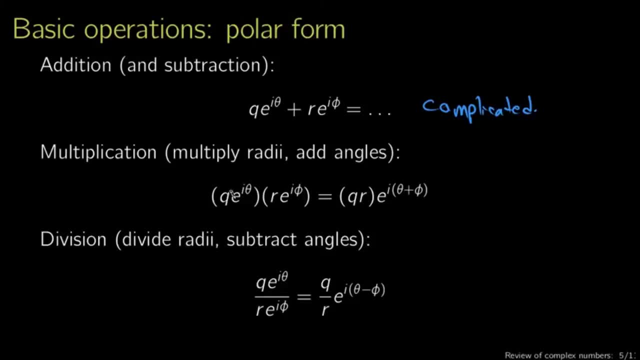 in polar form have very nice expressions: q? e to the i theta times, r e to the i phi. well, these are just all real numbers multiplying together, and then I can use the rules regarding multiplication of exponentials. meaning, if I have two things, 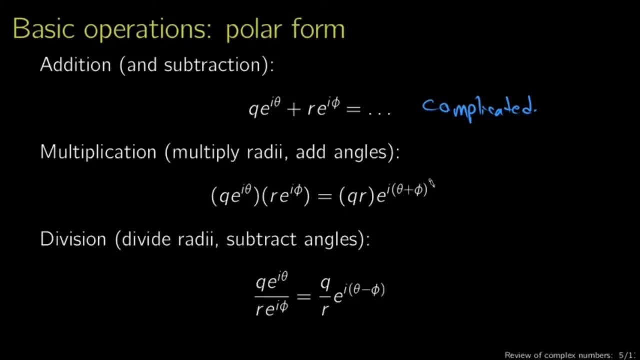 like e to the i theta and e to the i phi. I can just add the exponents together. It's like taking x squared times x to the fourth and getting x to the sixth, But q? r e to the i theta plus phi. 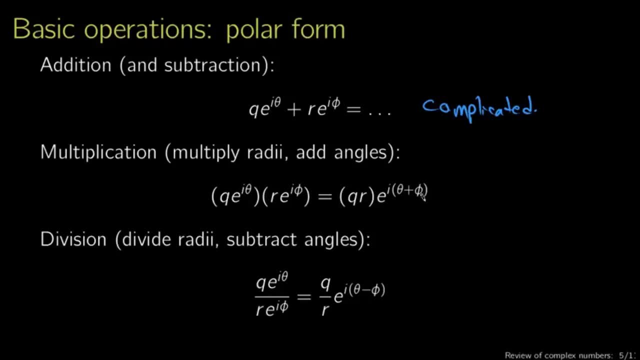 So that was easy. We didn't have to do any distribution at all. The key fact here is that you add the angles together. In the case of division, it's also quite easy. You simply divide the radii q over r. 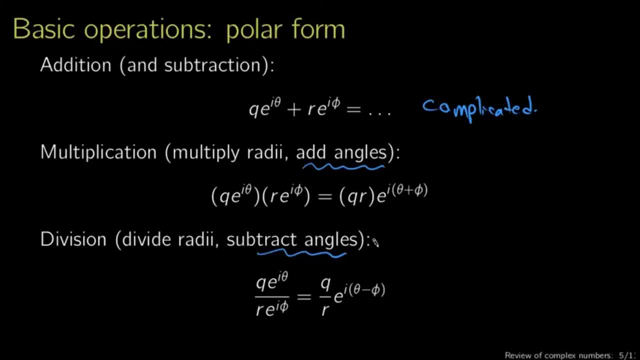 and instead of adding, you subtract the angles. So complex numbers expressed in polar form are much easier to manipulate in multiplication and division, while complex numbers represented in rectangular form are much easier to manipulate for addition and subtraction. Taking the magnitude of a complex number, 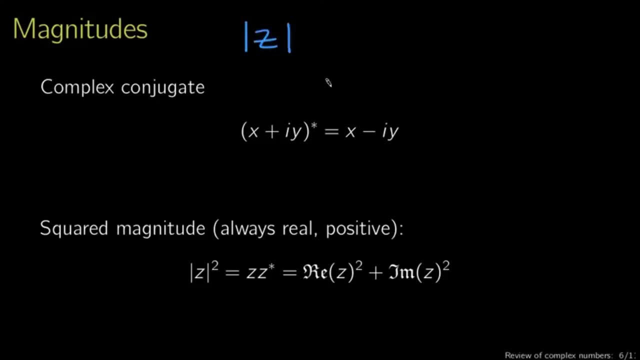 usually we'll write that as something like z. if z is a complex number, just using the same notation for absolute value of a real number usually is expressed in terms of the complex conjugate. The complex conjugate, notationally speaking, is usually written by whatever complex number you have. 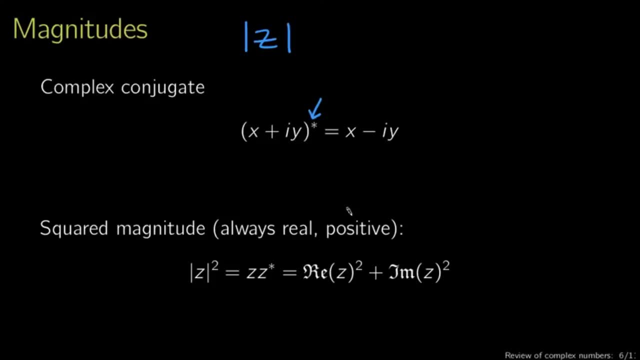 here, in this case, x plus i y, with a star after it, And what that signifies is you flip the sign on the complex part, on the imaginary part. x plus i y becomes x minus i y. The squared magnitude, then, which is always going to be a real and positive number. 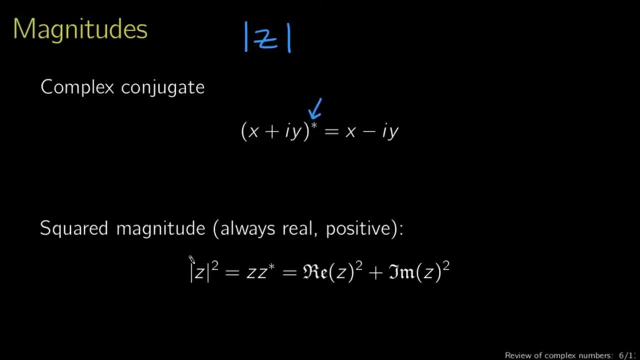 this absolute value squared notation is what you get from multiplying a number by its complex conjugate, And that's what we saw earlier with c plus i d. Say I take the complex conjugate of c plus i d and multiply it by c plus i d. 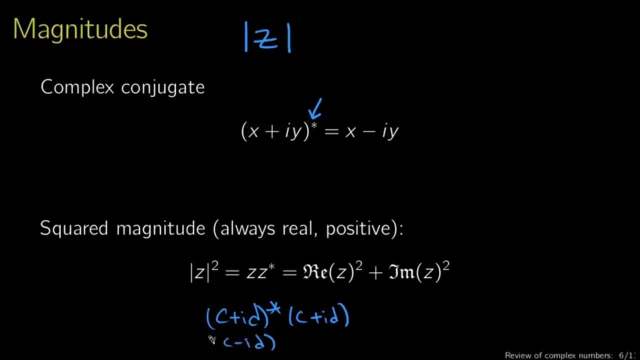 Well, the complex conjugate of c plus i d is c minus i d, times c plus i d. And doing the distribution like we did when we calculated the denominator, when we were simplifying the division of complex numbers in rectangular form, just gave us c squared plus d squared. 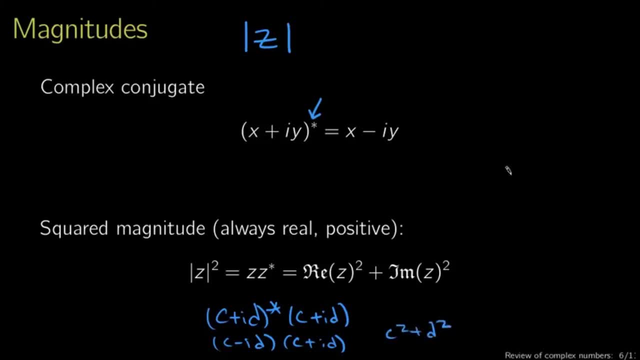 This should be suggestive. if you have something like x plus i- y, that's really messy- x plus i- y- and I want to know the squared absolute magnitude. Thinking about this as a position in Cartesian space should make this formula c squared plus d squared, in this case. 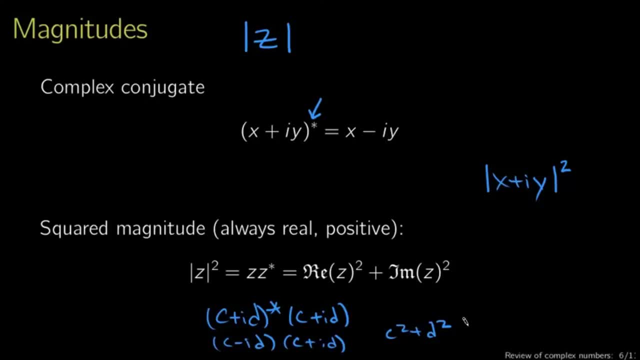 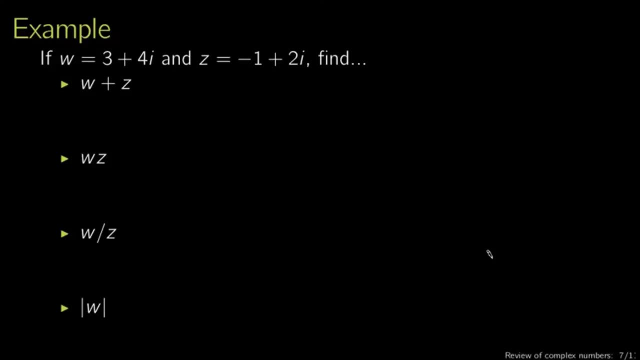 just make a little more sense. You can also, of course, write that in terms of real and imaginary parts, But let's do an example: If w is 3 plus 4i and z is minus 1 plus 2i, 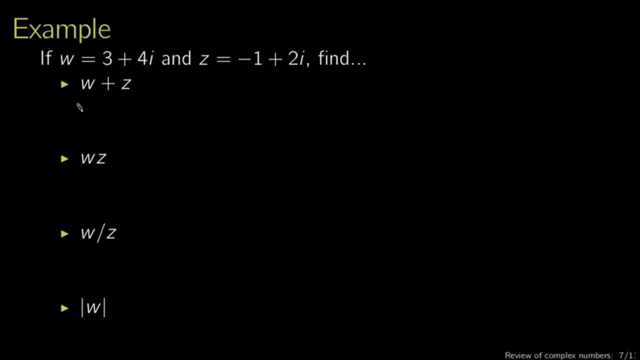 first of all, let's find w plus z. Well, w plus z is 3 plus 4i plus minus 1 plus 2i. That's straightforward. If you can keep track of your terms, 3 minus 1 is going to be our real part. 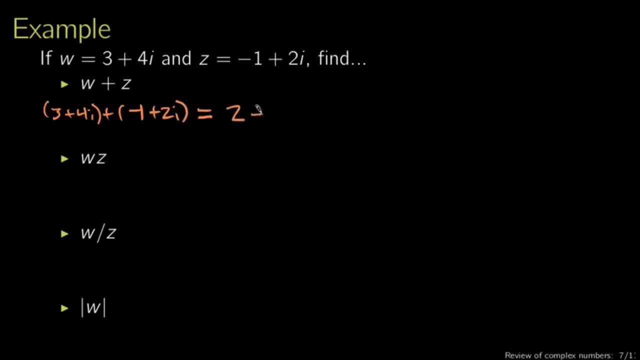 so that's 2. And 4i plus 2i, which is plus 6i, is going to be our complex part, Sorry, our imaginary part. Now, w times z, 3 plus 4i times minus 1 plus 2i. 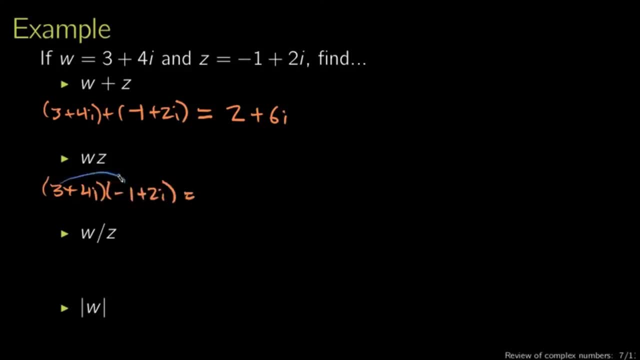 For this we have to distribute w times 2i, Like usual. So from our top eyebrow terms here we've got 3 times minus 1, which is minus 3, and 4i times 2i, Both positive. 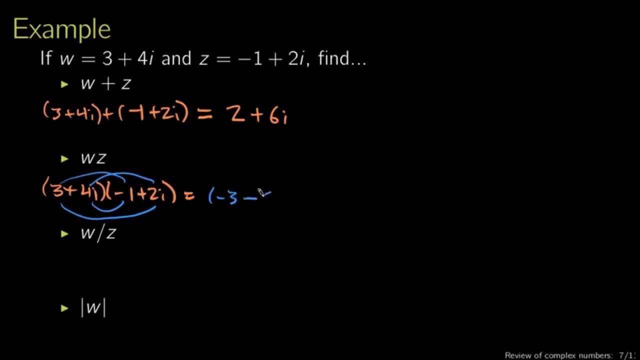 So I have 4 times 2,, which is 8,, and i times i, which is minus 1. Minus 8.. Then for my imaginary part, I guess the mouth and the chin, if you want to think about it that way. 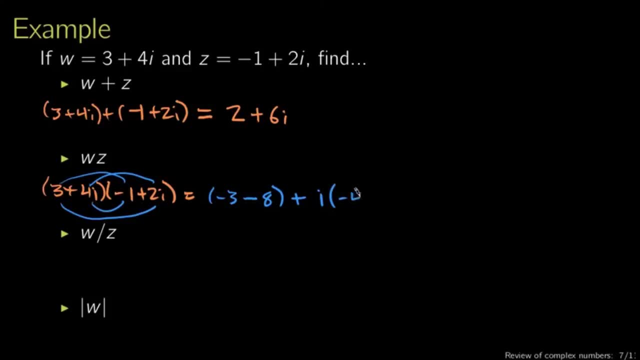 I have 4i times minus 1, minus 4, with the i out front will just be minus 4 inside the parentheses here- and 3 times 2i is going to give me 6i plus 6 inside. 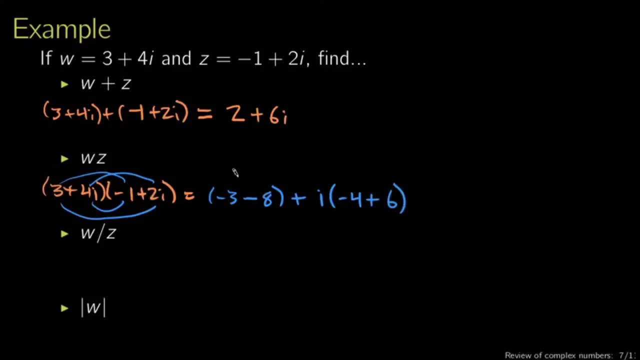 And the end result you get here is minus 8, minus 3 is minus 11, and minus 4 plus 6 is going to be is going to be 2.. So I get minus 11 plus 2i for my multiplication here. 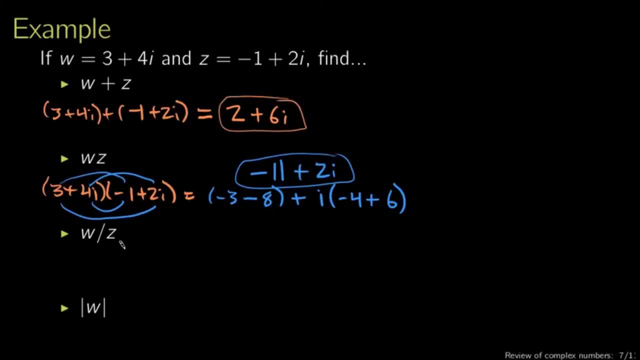 I guess if I'm going to circle that answer, I should circle this answer as well. Now, slightly more complicatedly: w over z. w is 3 plus 4i and z is minus 1 plus 2i. And you know when you want to simplify. 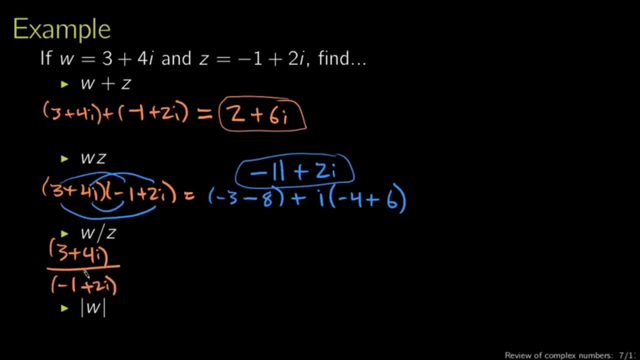 an expression like this: you multiply by the complex conjugate of the denominator, divided by the complex conjugate of the denominator. So minus 1 minus 2i divided by minus 1 minus 2i. And if we continue the same sort of distribution, 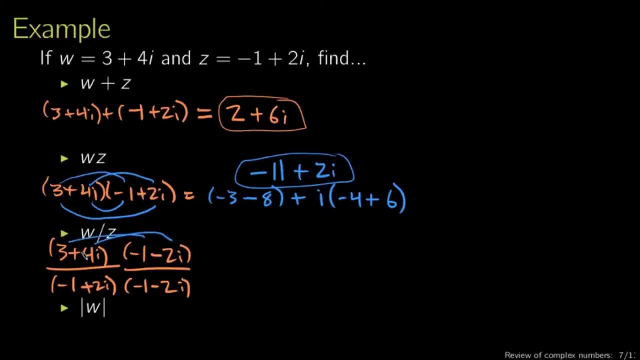 I'll do the numerator first, Same sort of multiplication we just did here, only the signs will be flipped a little bit. We'll end up with minus 3 plus 8, instead of minus 3 minus 8.. And for the complex: 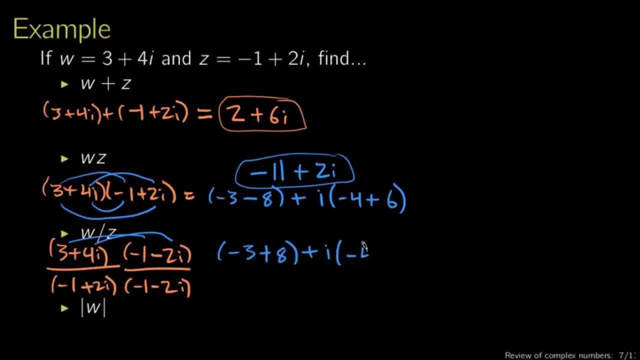 sorry for the imaginary part. we'll end up with minus 4 minus 6, instead of minus 4 plus 6. And you can work out the details of that distribution on your own if you want. The denominator is not terribly complicated. 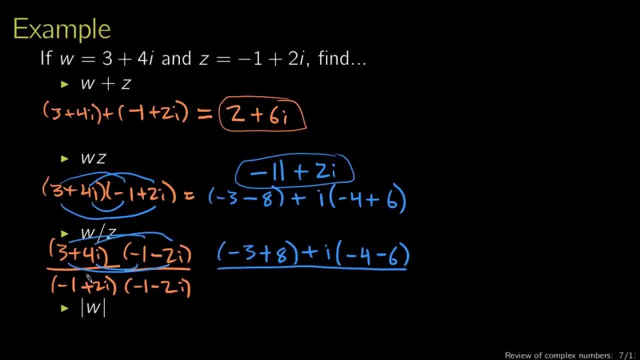 Since we know we're taking the absolute magnitude of a complex number by multiplying a complex number by its complex conjugate, we can just write this out as the square of the real part 1,, plus the square of the imaginary part minus 2,. 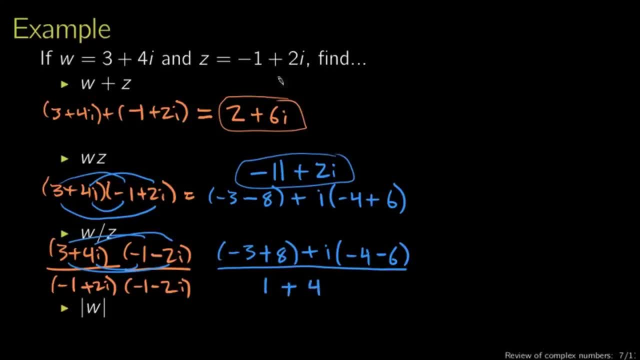 which squared is 4.. So, if I continue this final step, this is going to be 5, this is going to be minus 10i, and our denominator here is just going to be 5.. So, in the end, what I'll end up with is going to be 1 minus 2i. 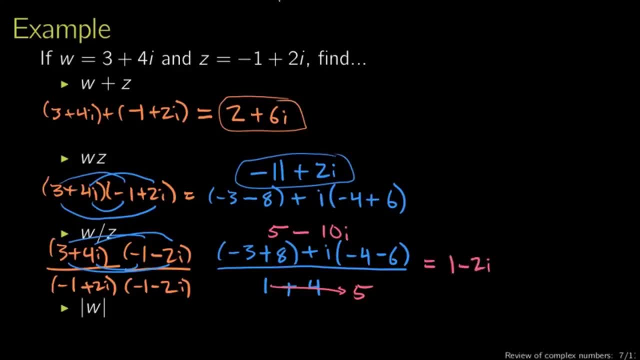 So it actually ended up being pretty simple in this case. Now for the absolute magnitude of w 3 plus 4i. You can think of this as w times w star square root. You can think of this as the square root of. 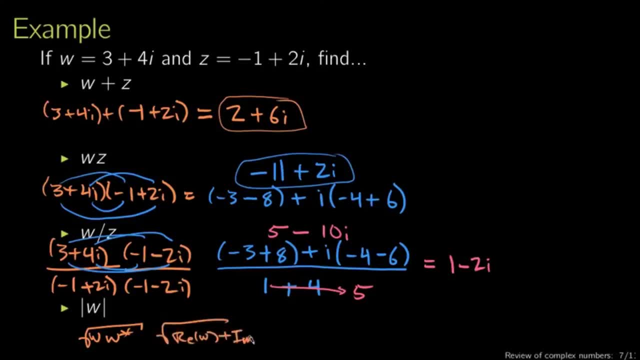 the real part of w plus the imaginary part of w. Sorry, square root of the square root of the real part plus the square of the imaginary part, Which is perhaps a little easier to work with in this case, so you don't have to distribute out complex numbers in that way. 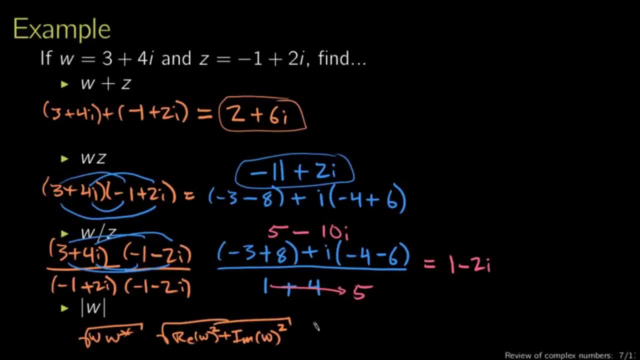 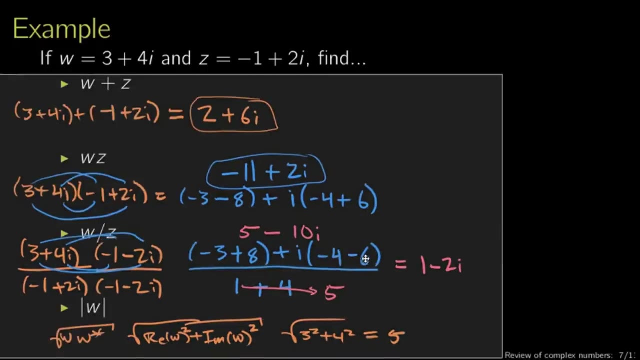 Real part is 3, imaginary part is 4, so we end up with the square root of 3 squared plus 4 squared, which is 5.. Now, this was all in rectangular form. Let me move this stuff out of the way a little bit. 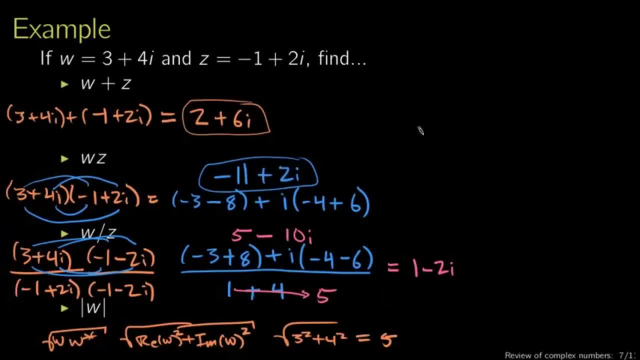 And let's do it again, at least a subset of it in polar form. In polar form: w 3 plus 4i- we know the magnitude of w, that's 5.. So that's going to be our radius. 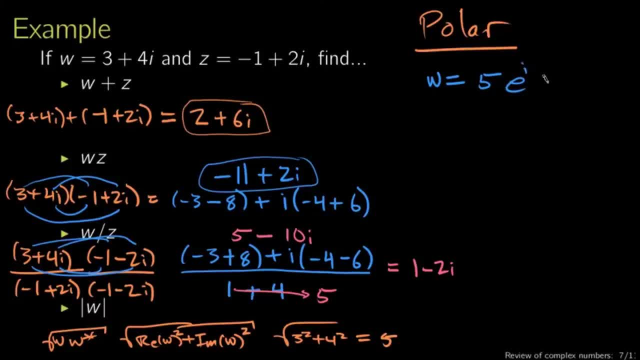 5, and our e to the i theta, where theta is, like I said, the arctan of, in this case not 4 fourths, 4 thirds. So that's the polar form of the complex number w. 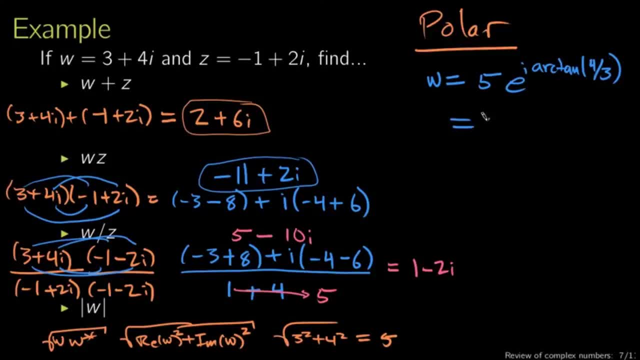 Now, if you plug this into your calculator to figure out what the arctan of 4 thirds is, you'll get 5e to the i 0.927.. If you do the same thing for z, you'll end up with the square root of 5. 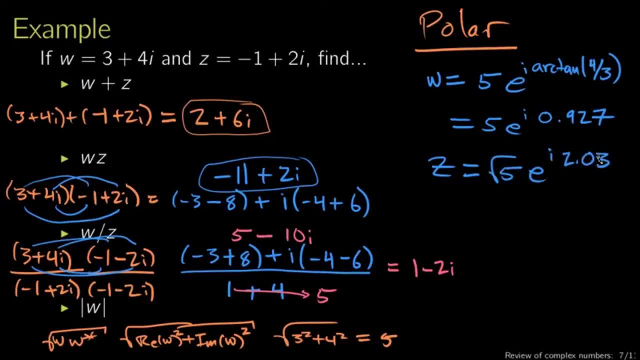 times e to the i, 2.03.. And, for instance, if I wanted to calculate w over z, I would just have, well, the radius associated with w divided by the radius associated with z times e to the i difference of the angles. 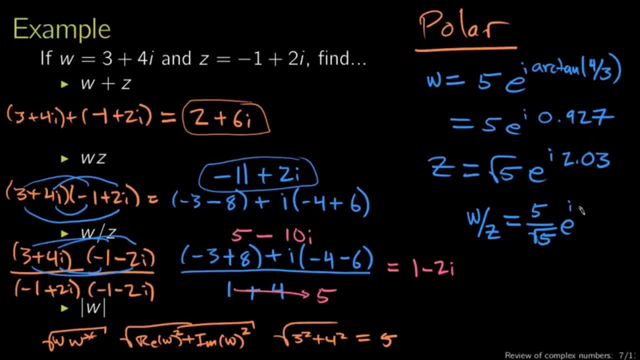 And if you take 0.927 and subtract 2.03, you end up with minus 1.1, give or take, And if you actually go through and check, you will find out that these two numbers are equal to each other. 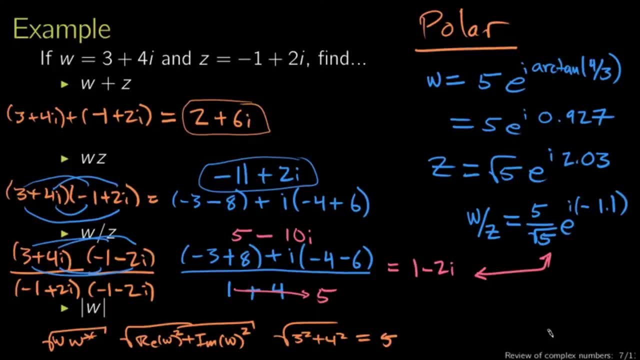 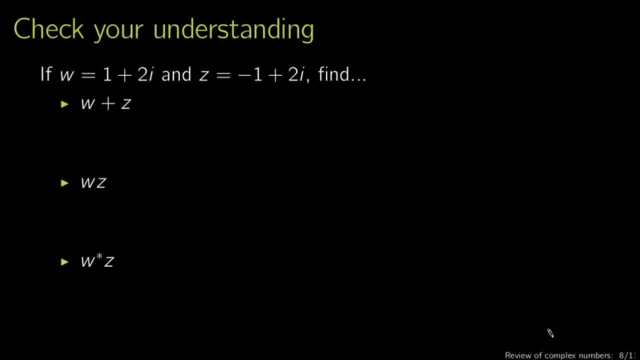 So that's an example of manipulating complex numbers just in a very simple way. In order to check your understanding, here's another example for you to work through on your own. Now, the geometric interpretation I've been alluding to is whoops. I wanted to do this in black. 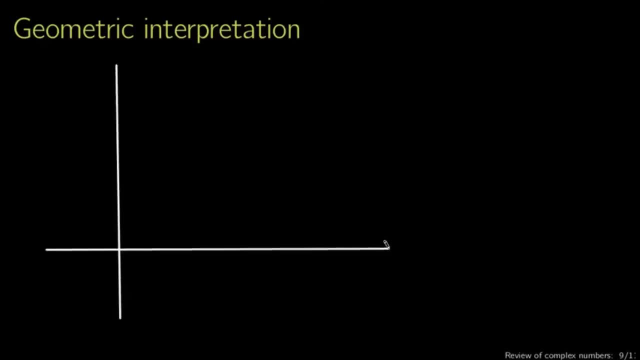 is in two dimensions, hopefully not too surprising. I kept mentioning the rectangular form and the polar form. Well, instead of the rectangular form being rectangular coordinates x and y, we're going to talk about the rectangular form being the real and imaginary parts of a complex number. 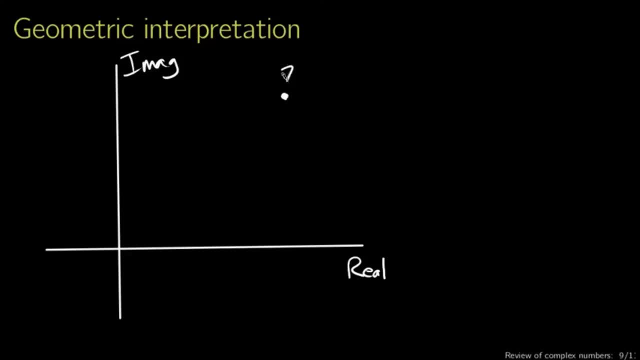 So if we have some complex number here, let's call it z. we can think of that as being composed of some real part of z and some imaginary part of z. That's the rectangular form of complex number z, If you want to think about. 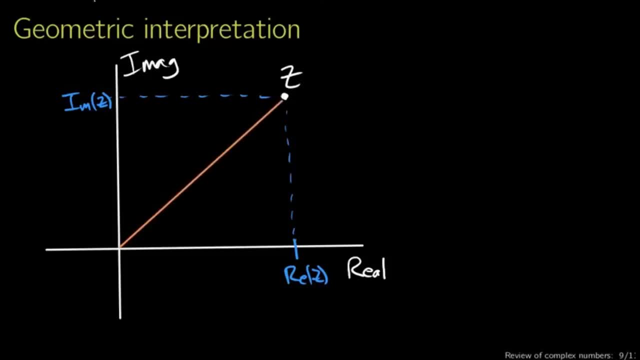 the polar form of z. well, this would be the radius associated with that and this would be the angle. So if I want to say z equals r, e to the i theta, this is the distance I'm talking about for r and this is the angle I'm talking about for theta. 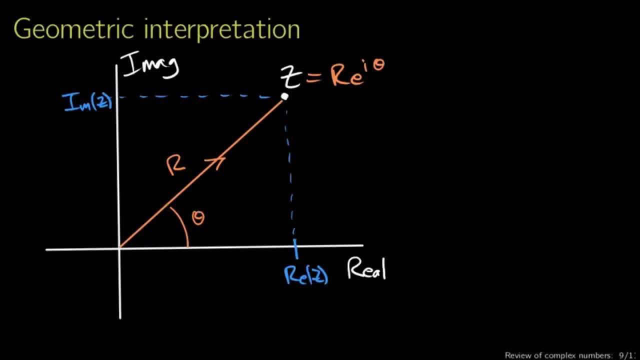 Now, in the geometric interpretation, addition and multiplication do pretty much what you would expect. Sorry, addition and subtraction do pretty much what you would expect. If I have a complex number here, say w, and another complex number here, say z. 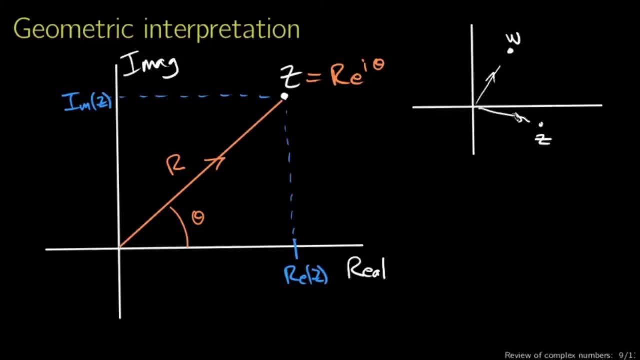 I can treat these as vectors and just add them tip to tail. So one vector is going in this direction, one vector is going in this direction. the vector sum will just put me out here w plus z. Same thing for subtraction, but with the sine flip. 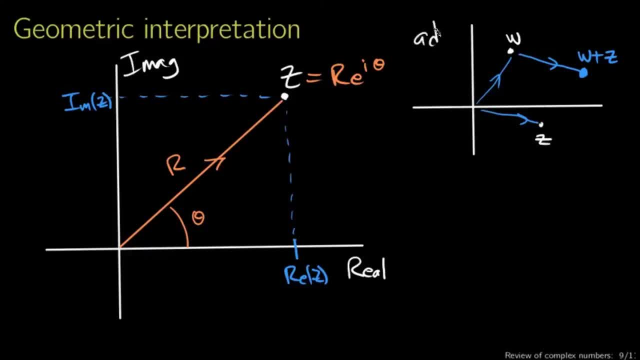 on whatever is being subtracted. This is for addition. When I multiply, the multiplication rule or the geometric interpretation also has a nice way of treating multiplication. If I have some complex number, again say w, some complex number, say z. 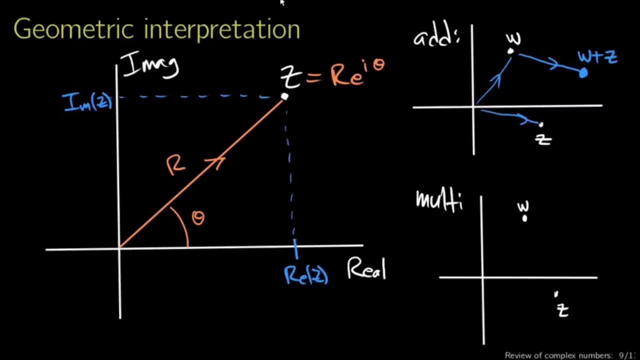 the best way of thinking about this is in polar form, where I have, say, a vector with one angle- here I'll call that theta, let's call it theta1, and another vector here with an angle- theta2.. Sorry for the small font. 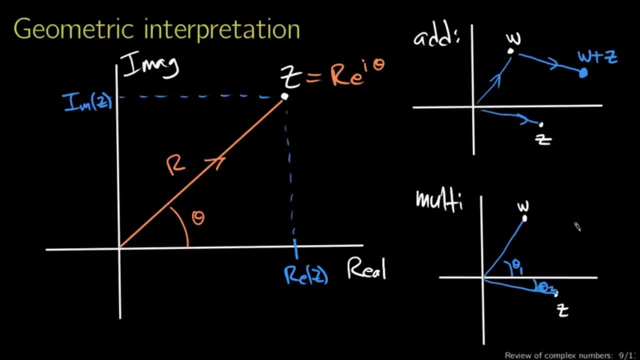 I hope this is legible. When you multiply these two complex numbers together, you know you have to multiply the radii- maybe that will put you out somewhere at large radii- and you have to add the angles together. In this case, theta1 is going. 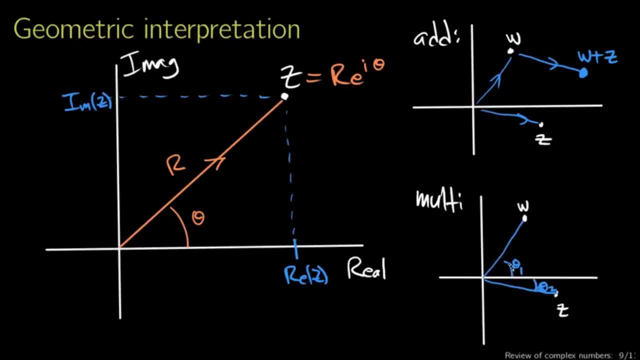 upwards, theta2 is going downwards. So if I go up theta1, and then add going back down theta2, I'll end up somewhere out here, say, where the distance I've gone is the magnitude of w times the magnitude of z. 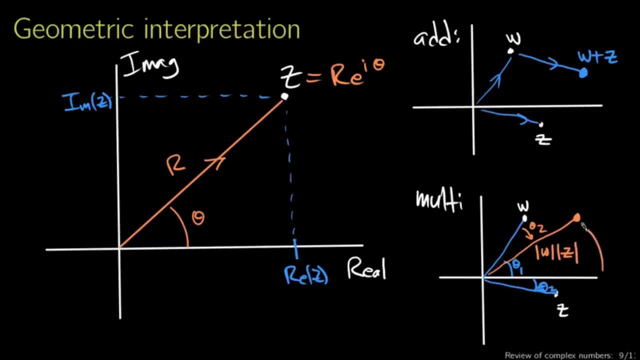 and the angle I'm at now here is theta1 plus theta2, where theta2 is negative. So addition and multiplication are nice geometric interpretations as well. Especially useful in visualizing multiplication is this notion of rotating your complex vector. I have effectively rotated. 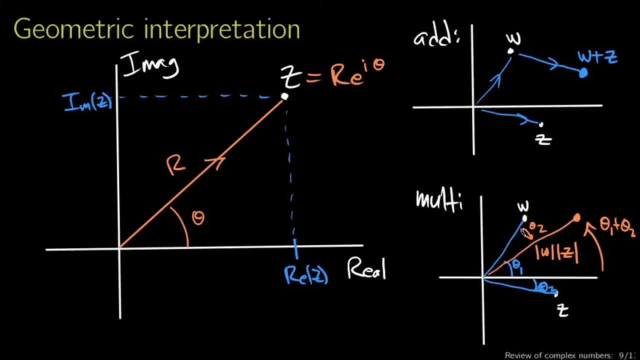 down theta2 from the vector to w in order to get in the direction from the origin towards the product w times z. So hopefully that's reasonably clear. The geometric interpretation can help a lot when it comes to visualizing what actually happens with complex numbers, especially. 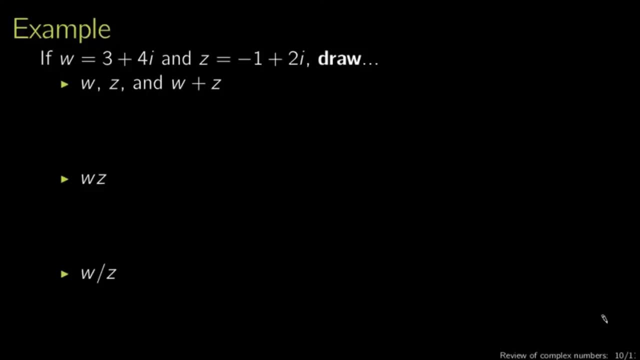 in the context of quantum mechanics, when you're dealing with complex functions. At any rate, here's another example where I'm going to draw out what these things actually look like. So I have two complex numbers: 3 plus 4i and minus 1 plus 2i. 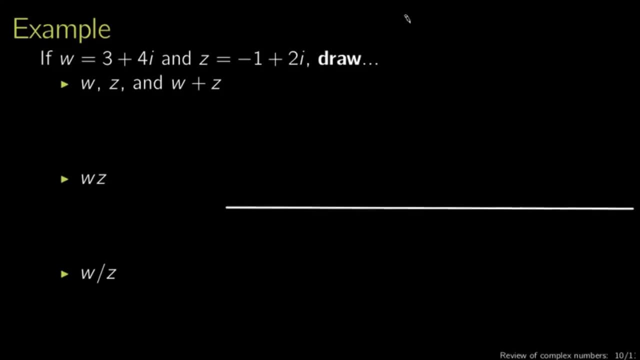 Let me draw myself a nice big coordinate system here And I'll put some tickmarks on it: 1, 2, 3, 4,, 5,, 6,, 7, 8.. 1,, 2,, 3, 4,. 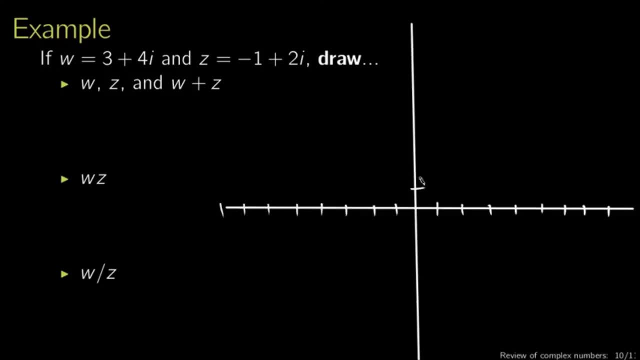 5,, 6,, 7,, 8.. 1,, 2,, 3,, 4,, 5,, 6,, 7,, 8.. And 1,, 2,, 3,, 4,, 5,, 6,, 7,, 8.. 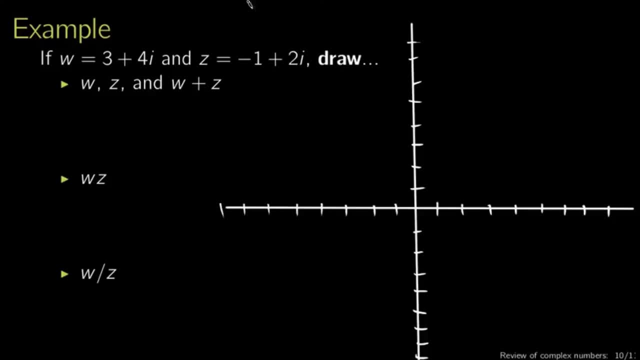 More or less. Now, first of all draw w z, and w plus z is 3 plus 4i. So my real part is 3, 1,, 2, 3.. My imaginary part is 4, so I go 1,, 2,. 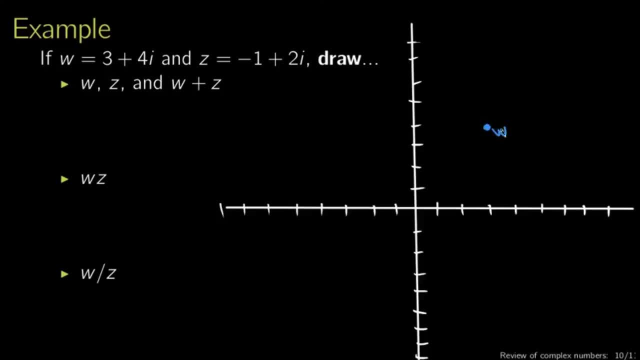 3, 4.. So I am up here. That's where w would be. Now. z is minus 1 plus 2i. So minus 1 plus 2i is z. So z is going to be there Now, if I treat these both as. 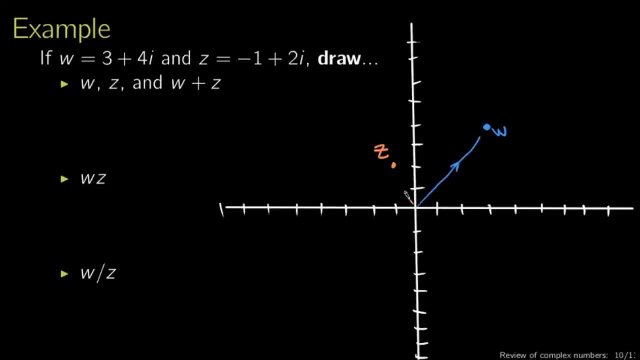 vectors. I have a vector to w and I have a vector to z and I add the vectors the way I would normally add vectors: tip to tail. I'll end up here at w plus z. Now it's easy to see this in Cartesian coordinates as well. If I'm adding w and 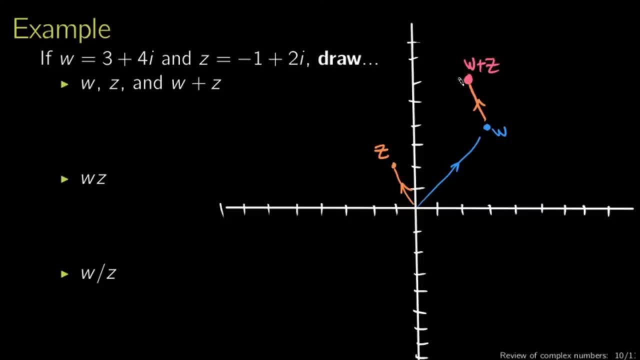 z. I'm going to end up with 3 minus 1, or 2 up here and 4i plus 2i or 6i, 1,2,12,3,4,5,6 for the 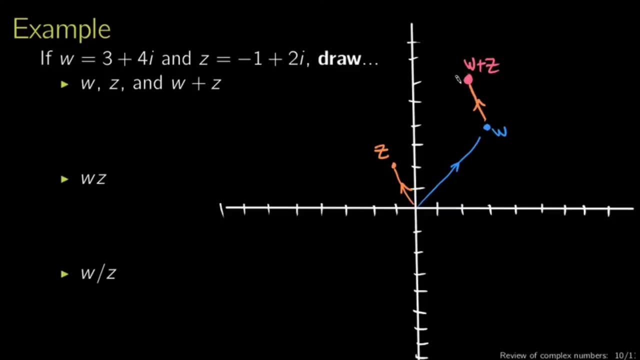 imaginary part. Let's see what that means. now, It's not relative, it's two-棊 very similar. Was that sort of a J away fromầ×우 erschHe's same imaginary part? Now W times Z, If you actually go through and work out what W. 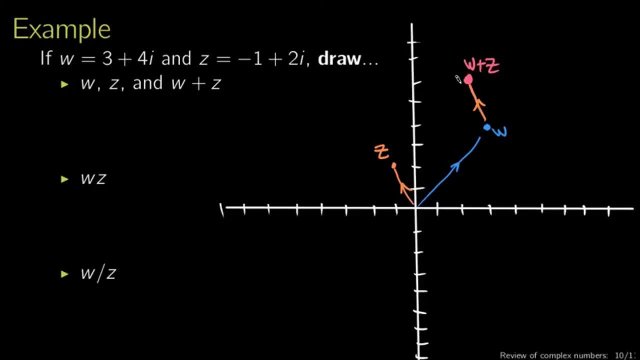 times Z is, you'll find out, it has quite a large magnitude. It has a magnitude a little bit larger than 11, 11 point something. But what I really want to emphasize here is the geometric interpretation, and in that case you need. 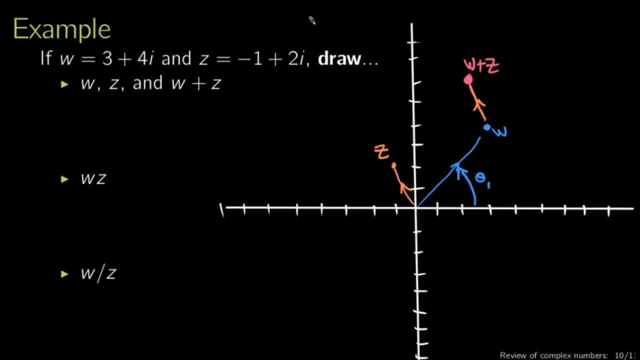 to know the angles involved. So I have an angle here, theta 1, and I have an angle here, theta 2.. And it turns out if I add these two angles together, say going up theta 1 and then going over theta 2, I end up somewhere along this in this. 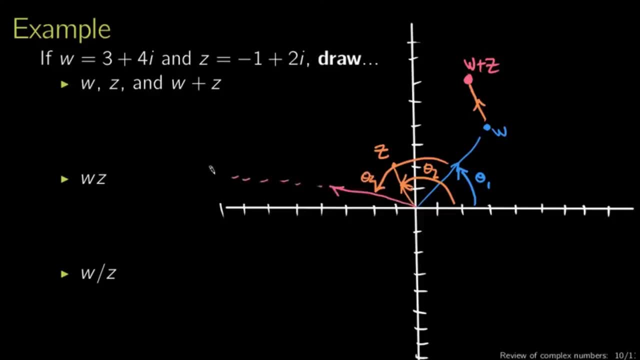 direction And you actually have to go out quite a ways. You have to go all the way to minus 11 plus what was it? plus 2i? I think Yes. minus 11 plus 2i is the answer for W times Z. And if you just look at the, 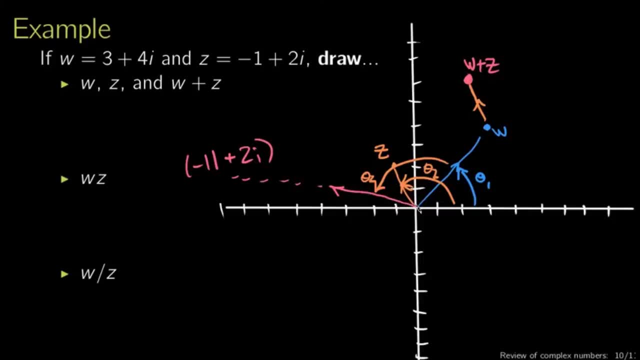 angles here. you'll notice that I have a little bit of a slope here, So I can here adding theta1, and theta2 is going to point you in that direction. so you know it's going to have a negative real part and a positive imaginary part, but perhaps a small positive. 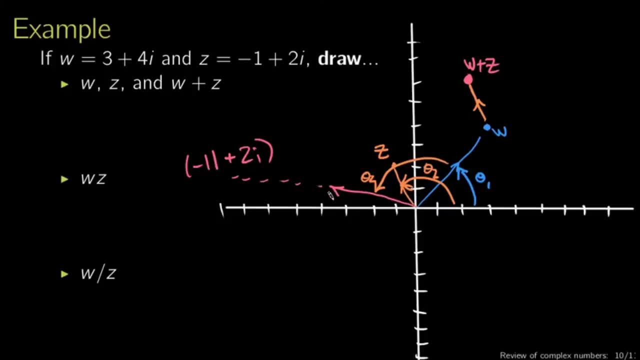 imaginary part, just by eyeballing the angles, which is not really all that bad. W divided by z is the same sort of situation, except now, instead of adding theta2 to theta1,, you're going to subtract theta2 from theta1, so I'm going to go up theta1 and then back. 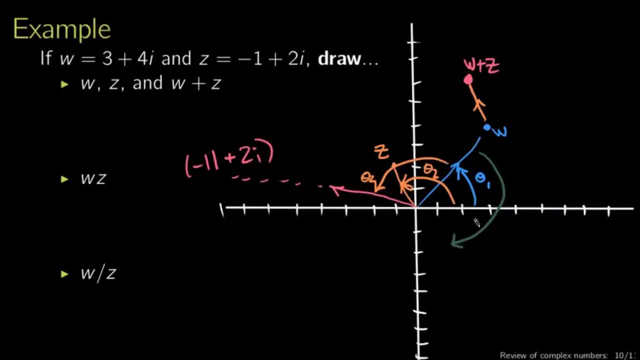 down theta2, and where you end up is actually here at 1 minus 2i. But just by eyeballing the angles you can get a good feel for what part of the complex plane you're in, where typically this is the real axis of the complex plane and this is 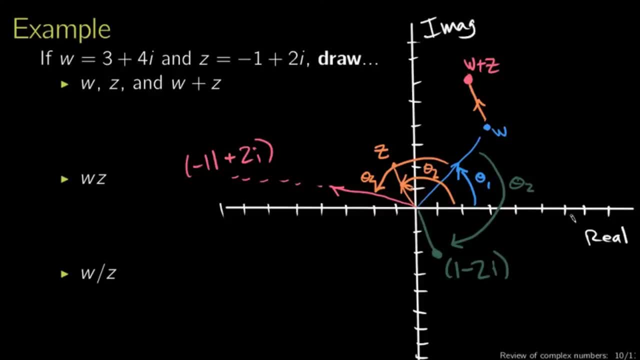 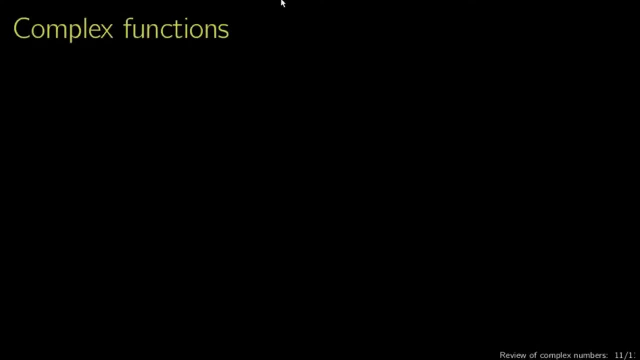 the imaginary axis, In Cartesian coordinates, you have two degrees of freedom: x and y. In the complex plane, you have two degrees of freedom: the real part and the imaginary part. The last thing that I need you to understand about complex numbers from the perspective. 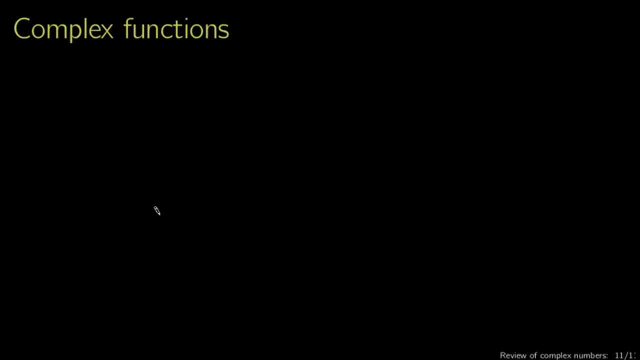 of quantum mechanics is complex functions. Now, the theory of complex functions is a lot of fun, but beyond the scope of a quantum course, To give you an idea for how complex these things can be, f of z is a complex function. Now z as a complex number. sorry, f of z, if f is a complex function, is going to be. 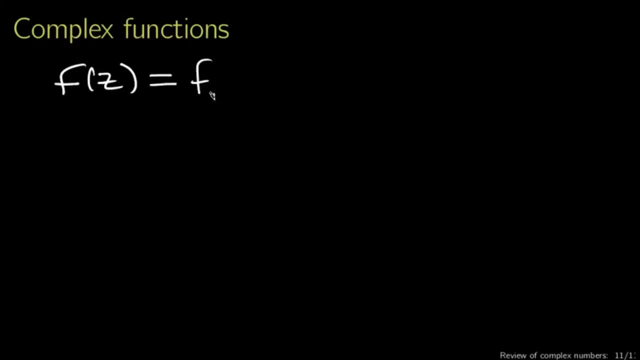 complex meaning. I can think about this as some real part function plus some imaginary part function times. i So my one function of a complex variable can actually be a complex function of a complex variable, can actually be thought of as two separate functions, Separate real functions, mind you. 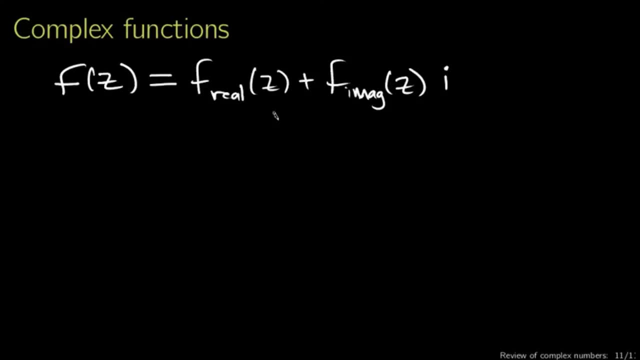 So this is a slightly simpler way of thinking about things. But you have a real part and an imaginary part. Now, in the case of true complex functions like f of z, z itself has two degrees of freedom. So you can think of this as f- real of the real part of z, and then the imaginary part. 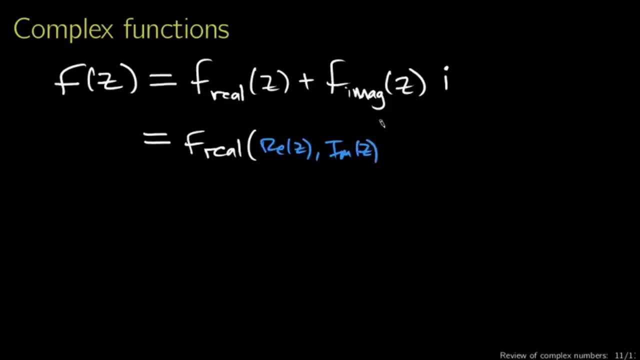 of z As two separate arguments To that function, And then plus i times f, imaginary times the same thing, The real part of z and the imaginary part of z. So we have, instead of one function of one variable, we have two functions of two variables. 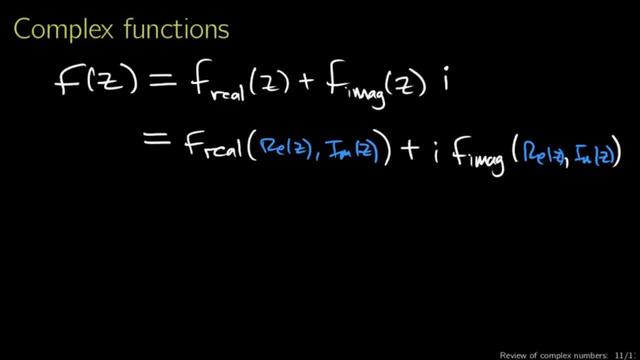 And that makes things very difficult to visualize. Thankfully, in quantum mechanics, What we're typically working with Is the wave function, psi, And psi, for a lot of the problems that we're going to be thinking about, is only a function of one coordinate. 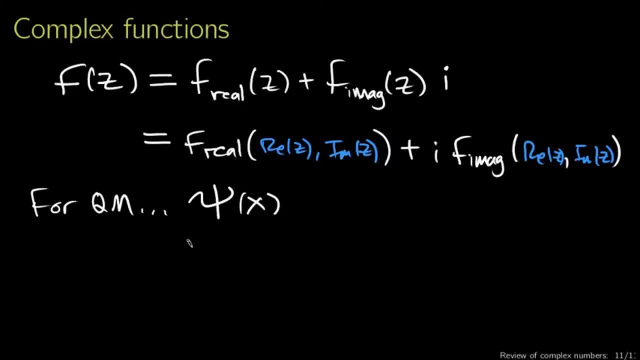 So you can think about this as psi of x, where x is a coordinate, So psi, while psi of x is complex, X is real. So while we have to think about The real and imaginary parts of x, parts of psi, we don't have to worry about the real and imaginary parts of X. 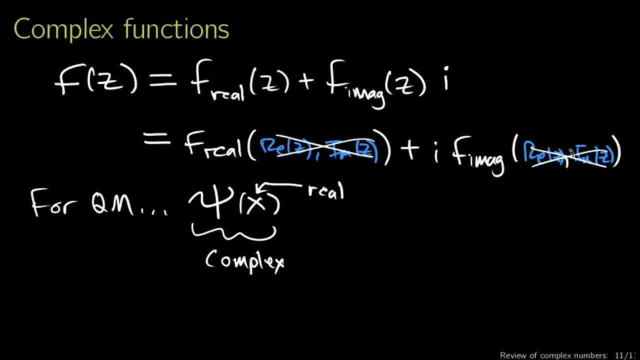 We can just think about this as X, a single argument In terms of how to visualize complex functions like this. you can think about plotting both the real and imaginary parts of this function as a function of whatever you're working with. In this case, let's say, we have to deal with psi of X, so this is going to be the x-axis. 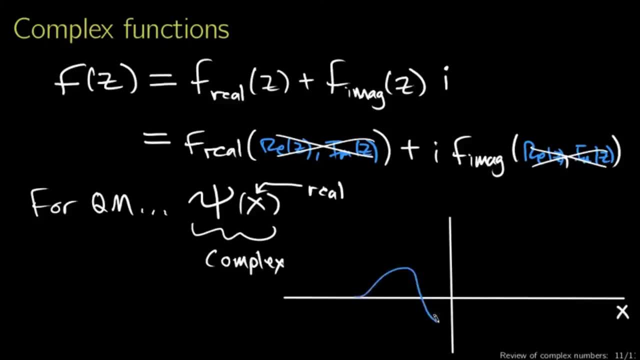 and we'll have something. maybe it looks like this for the real part of psi, of X, and something maybe it looks like this for the imaginary part of psi. So think about plotting two separate functions, the real and imaginary parts of this effective function of psi. 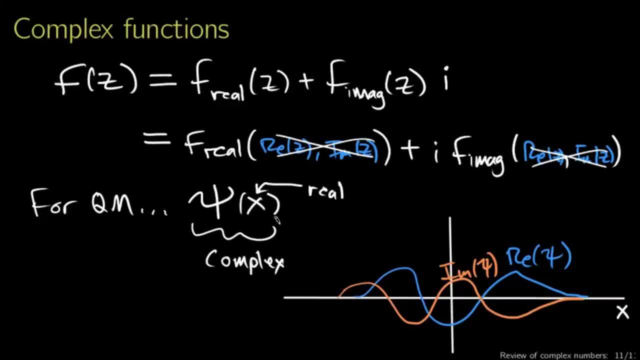 It's effectively a single function, as a function of- in the case of this, X, It's rather simple to visualize. Now I have some more advanced visualizations that use color to represent the angle in the polar interpretation of psi as a complex function and they get a little bit psychedelic and you start hallucinating. 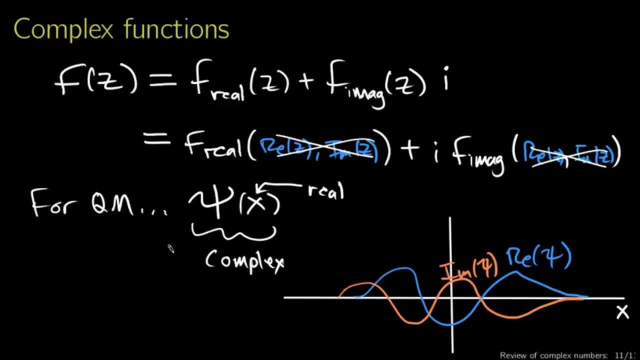 after a while if you look at them too much. But for now try to keep in mind that complex numbers have real and imaginary parts and can be interpreted both as X and Y in the complex plan, The real part and the imaginary part in a two-dimensional Cartesian plane or a. 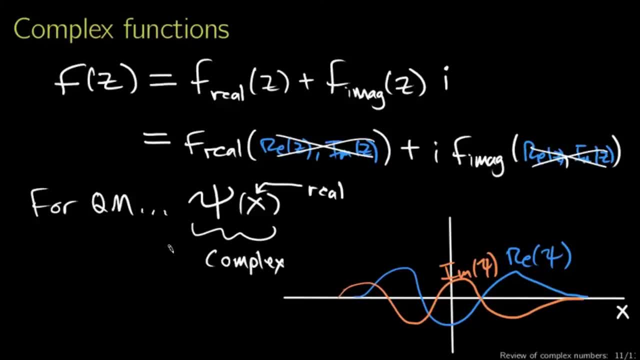 radius and an angle in a polar representation of the same two-dimensional complex plane. That's about it for quantum mechanics. Like I said, that's about it for complex analysis as needed for quantum mechanics. Like I said, complex analysis is a very deep, very beautiful topic and I encourage you to. 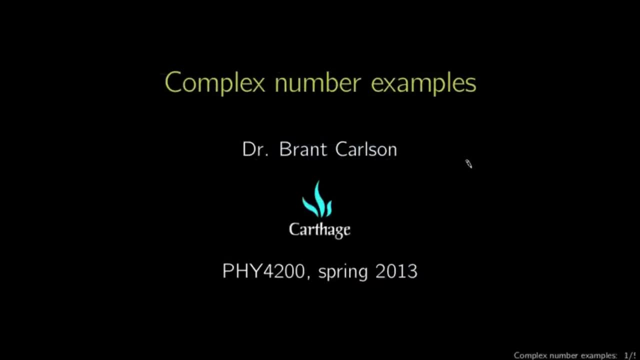 study it further in the future, but for now, I think that's all you need to know. Since complex numbers are so important to quantum mechanics, let's do a few more examples. In this case, I'm going to demonstrate how to manipulate complex numbers in a more general way, not so much just doing. 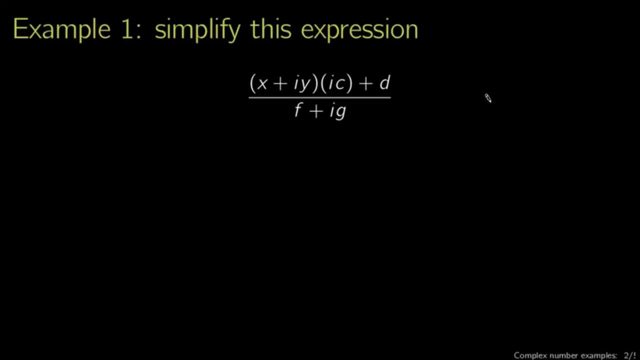 examples with numbers. First example: simplify this expression. You have two complex numbers multiplied in the numerator and then a division. First of all, the first thing to simplify is this multiplication: You have X plus IY times IC. This is pretty easy. It's a simple sort of distribution. We're 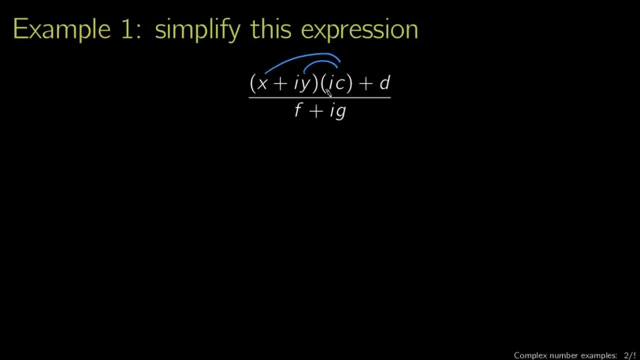 going to have X times IC. That's going to be a complex part, so I'm going to write that down a little bit: to the right: I X C, And then we're going to have IY times IC, which is going to be minus YC. That's going to be real. We also have a real 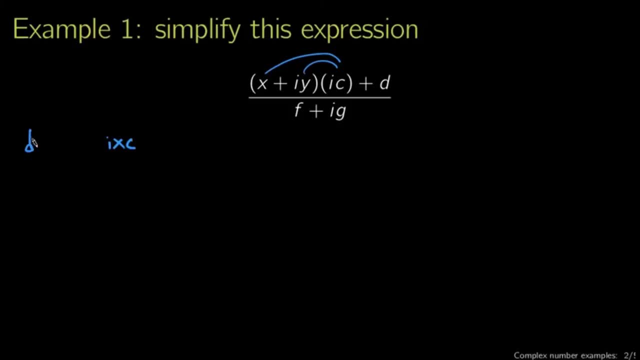 part in the numerator from the D here. so I'm going to write this as D minus YC plus IC. That's the result of multiplying this out. That's then going to be divided by F plus IG. Now, in order to simplify this, 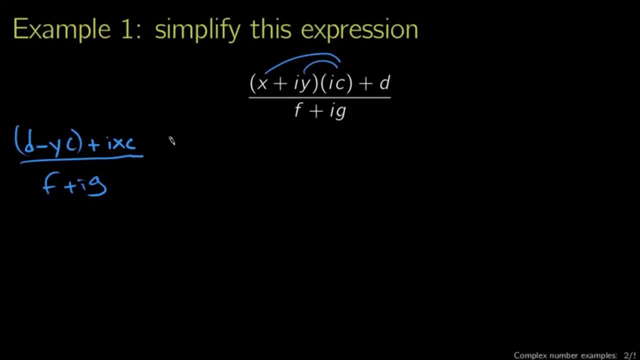 we have a complex number in the denominator. You know you need to multiply by the complex conjugate and divide by the complex conjugate. So F minus IG divided by F minus IG. Now expanding this out is a little bit messier, But fundamentally you've seen this sort of thing before. You have real part, real 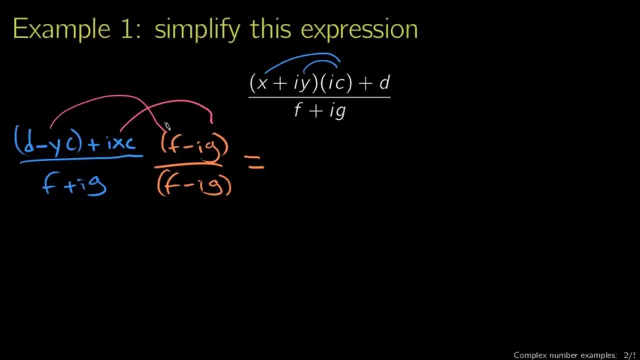 part and imaginary part, imaginary part in the numerator And then you're going to have imaginary part, real part and real part, imaginary part, And what you're going to end up with from this first term you get F times D minus YC From. 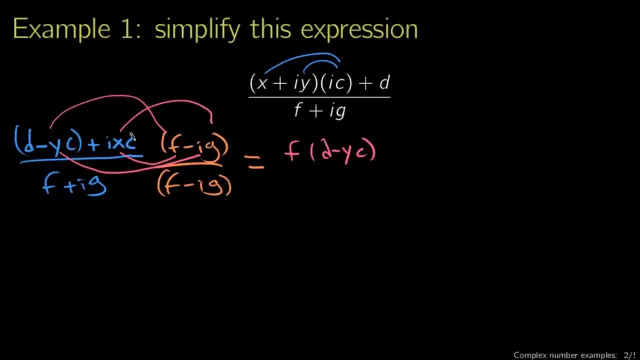 the second term. you have minus IG times IXC, which is going to give you XC G. You have a minus I times an I, which is going to give us a plus. Incidentally, if you're having trouble figuring out something like minus I times, I think 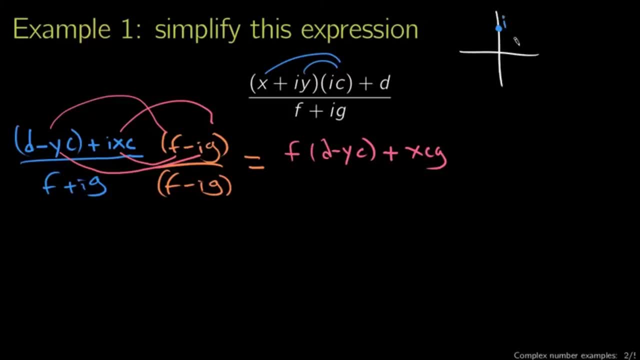 about it in the geometric interpretation. This is I in the complex plane, This is minus I in the complex plane, So I have one angle going up, one angle going down. If I'm multiplying them together, I'm adding the angles together, So I 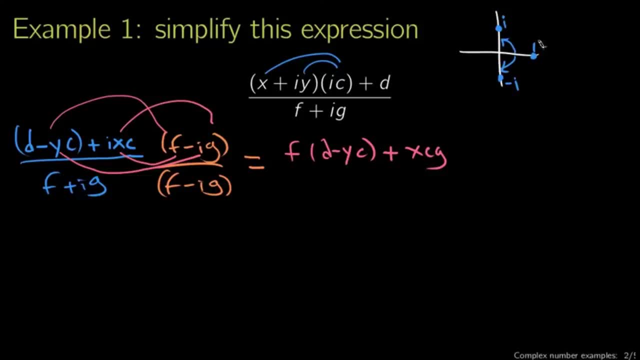 essentially go up and back down and I just end up with one equals I times minus I. Otherwise you can keep track of I squared equals minus ones and just count up your minus signs. This, then, is the real part. I suppose I should write that in green lest my fonts get too confusing, Excuse me. So that's the. 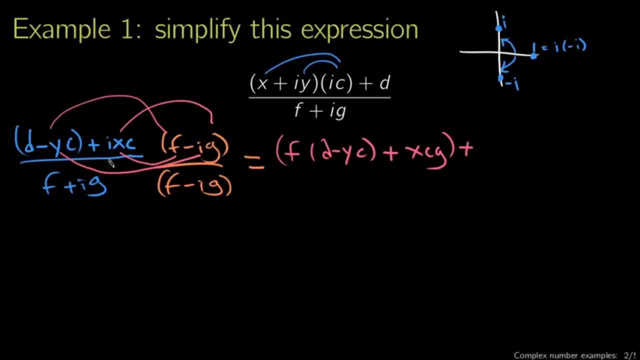 real part. The imaginary part, then, is what you get from these terms. here I'm going to write an I out front, and now we have XC times F, So XCF with an I from here, and then we have D minus YC times, IG, which 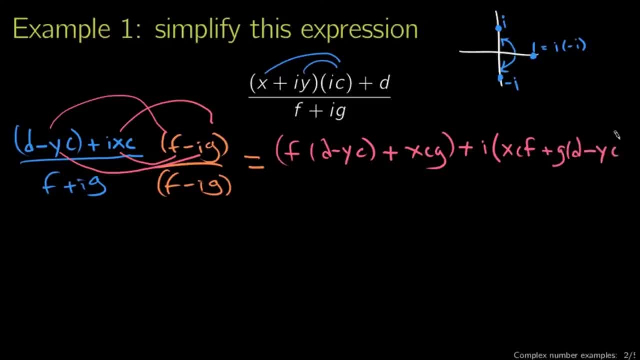 I'll just write as G D minus YC In the denominator. we're now multiplying a number by its complex conjugate. You know what to do there: F squared plus G squared. This is just the magnitude of this complex number, Sorry. 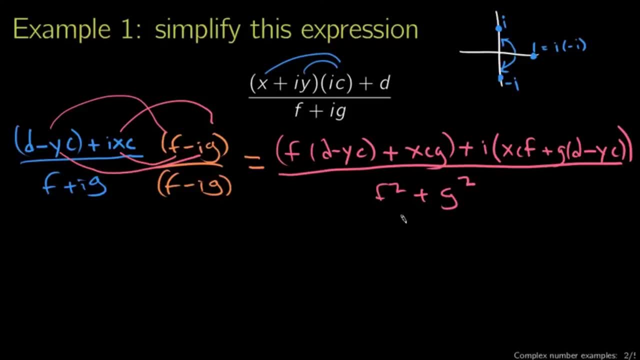 square root of YC. Now this doesn't necessarily look more simple than what we started with, but this is effectively fully simplified. You could further distribute this and distribute this, but it's not really going to help you very much. The thing to notice about: 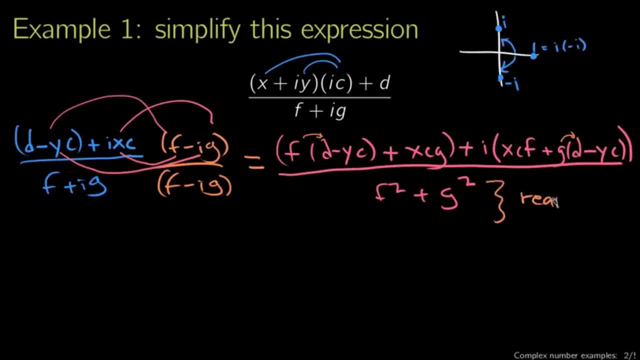 this is that the denominator is purely real. We've also separated out the real part of the numerator and the imaginary part of the numerator. My handwriting is getting messier as I go. Imaginary part of the numerator. So we can look at this numerator now and say, ah, this is the complex number. real part, imaginary. 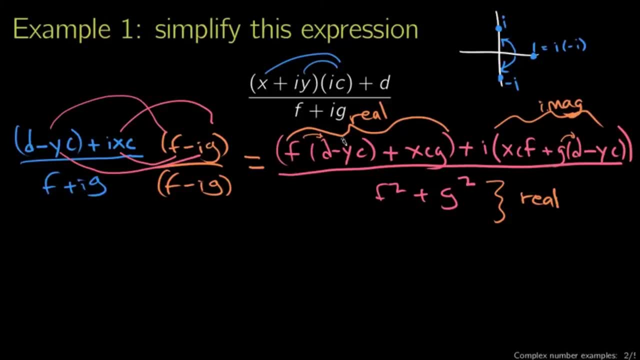 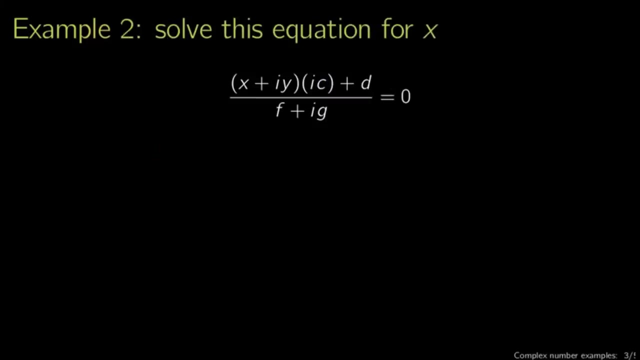 part, and then it's just divided by this real number, which effectively is just a scaling. It's a relatively simple thing to do: to divide by a real number. As a second example, consider solving this equation for X. Now, this is the same expression that we had in the last problem. 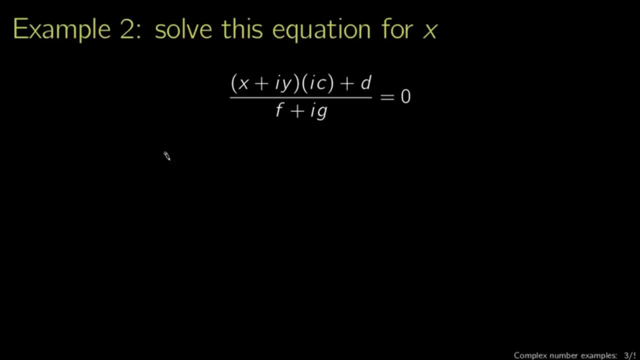 Only now we're solving it for it equal to zero. So from the last page I'm going to borrow that first simplification step we did. distributing this through, We had D minus YC for the real part plus IXC for the imaginary part and that was divided by F plus IG. 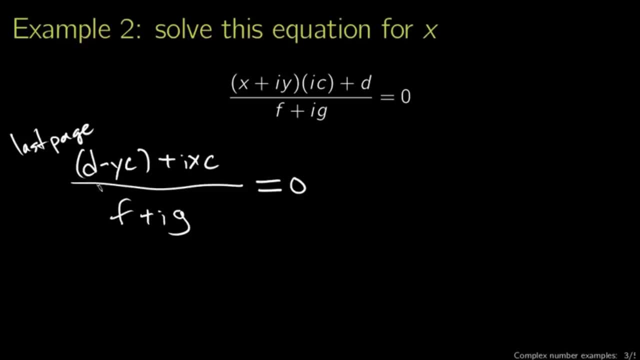 If we're setting this equal to zero. the nice part about dealing with complex expressions like this is that zero, treated as a complex number, is zero plus zero I. It has a real part and an imaginary part as well. it's just kind of trivial, And in order for this complex 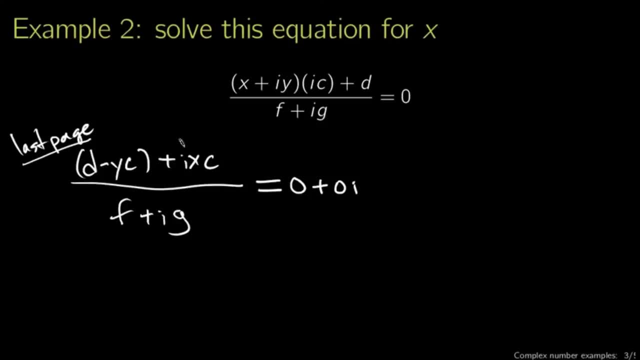 number to be equal to zero. the real part must be zero and the imaginary part must be zero. So we can think of this as D minus YC plus IXC. This has to equal zero and this has to equal zero separately. So we effectively have two equations. 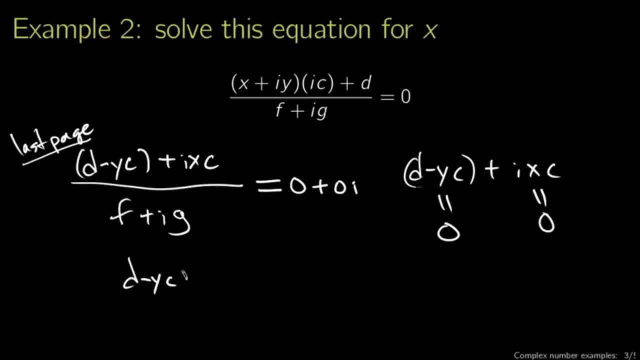 Not just one, which is nice. We have D minus YC equals zero and XC equals zero, Which, unless C equals zero, just means X equals zero. That's, the only way that this equation can hold is if X equals zero. The key fact here is to keep in mind that, in order for 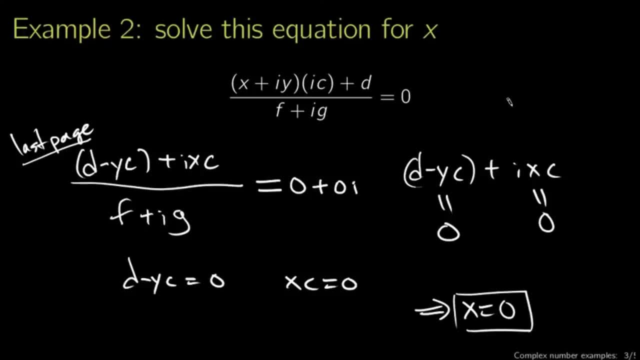 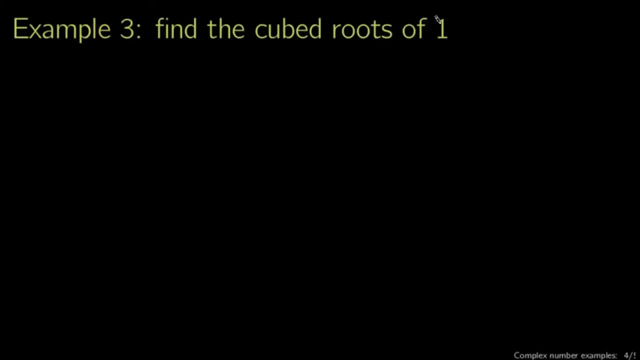 two complex numbers to be equal, both the real parts and the imaginary parts have to be equal. As a slightly more involved example, consider finding the cubed roots of one. Now you know, one cubed is one. that's a good place to start. We'll see that fall out of the algebra pretty. 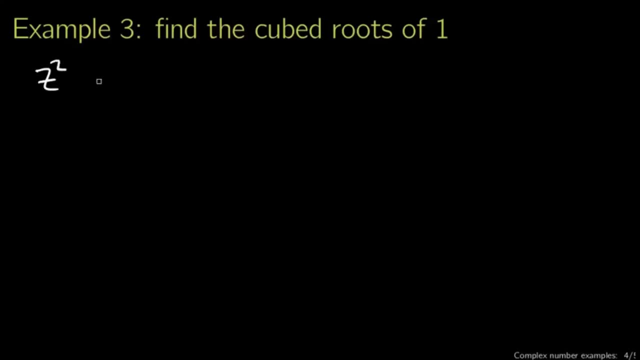 quickly. What we're trying to do is solve the equation Z cubed equals one, which you can think of as X plus IY, where X and Y are real numbers: cubed equals one. Now if we expand out this cubic, you get X cubed plus 3X squared times IY plus 3X times IY squared. 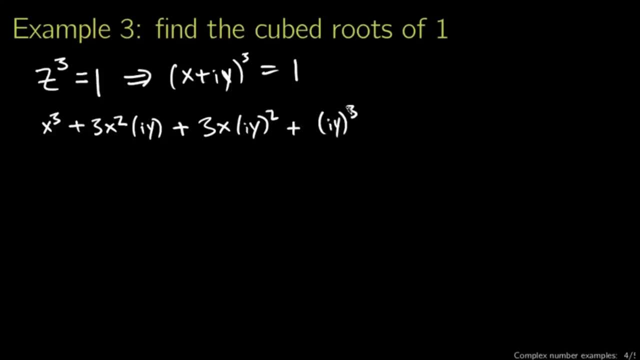 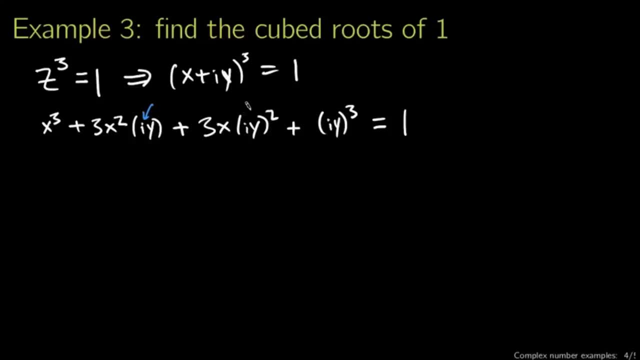 here we have an IY squared. This is going to give me an I squared, which is going to be a minus sign. And here I have an IY cubed. This is going to give me an I cubed, which is going to be minus I. So I have two complex parts and two real parts, So I'm going to 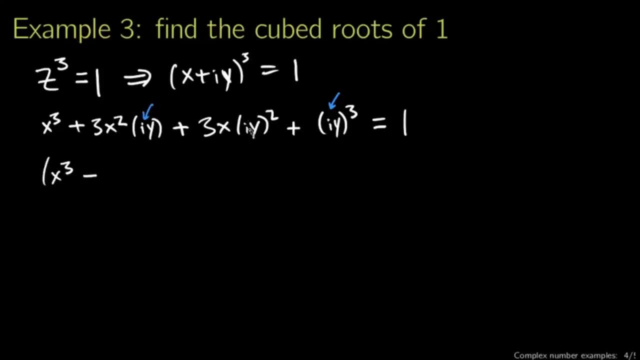 rewrite that X cubed, and then now a minus sign from the I squared 3XY squared, plus pulling an I out front. The imaginary part, then, is going to come from this 3X squared Y and this Y cubed. So I've. 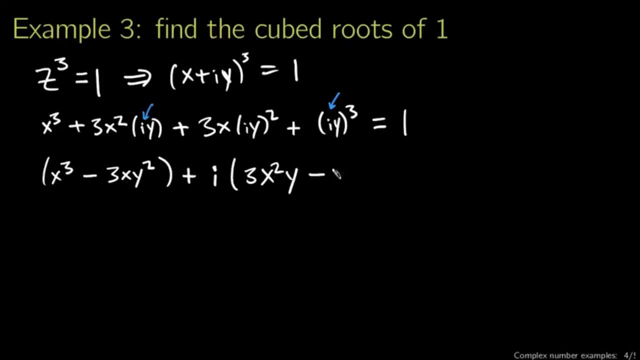 got a 3X squared Y here And then a minus Y, cubed Minus, coming from the I squared, And this is also going to have to equal one. Now, in order for this complex number to equal this complex number, both the real parts and the imaginary parts have to be equal. So let's. 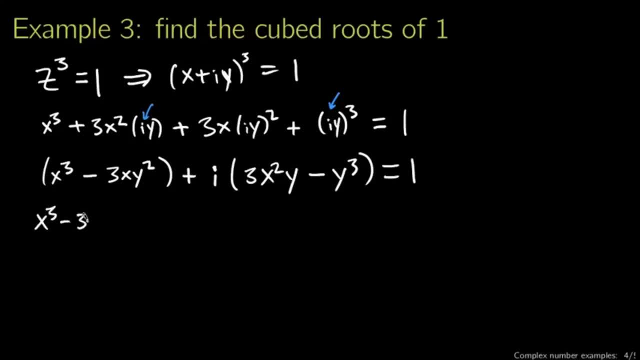 write those two separate equations: x cubed minus 3xy squared equals the real part of this is the real part of the left-hand side has to equal the real part of the right-hand side, 1. And the imaginary part of the left-hand side: 3x squared, y minus. 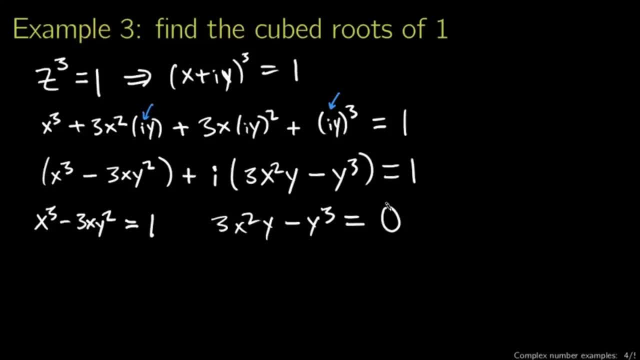 y cubed has to equal the imaginary part of the right-hand side, 0.. So those are our two equations. This one in particular is pretty easy to work with. We can simplify this. This is: we can factor a y out. This is y times 3x squared minus y. 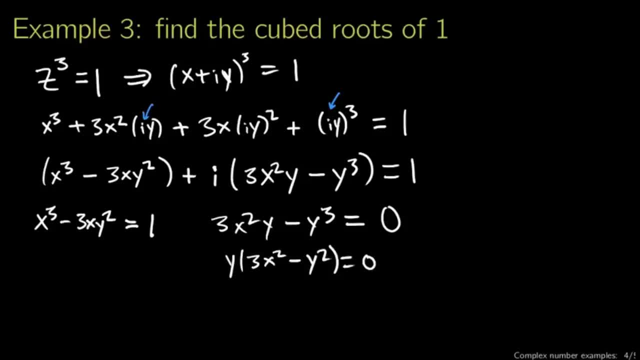 squared equals 0.. One possible solution, then, is going to come from this. You know, you have a product like this that equals 0. Either this is equal to 0, or this is equal to 0. And saying y equals to 0 is rather straightforward, So let's say y. 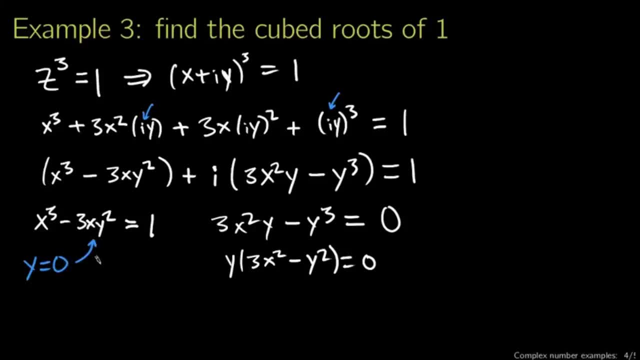 equals 0, and let's substitute that into this expression. So let's say: y equals 0, and let's substitute that into this expression. So let's say y equals 0, and let's substitute that into this expression. That's going to give us x cubed equals 1, which might look a lot like the. 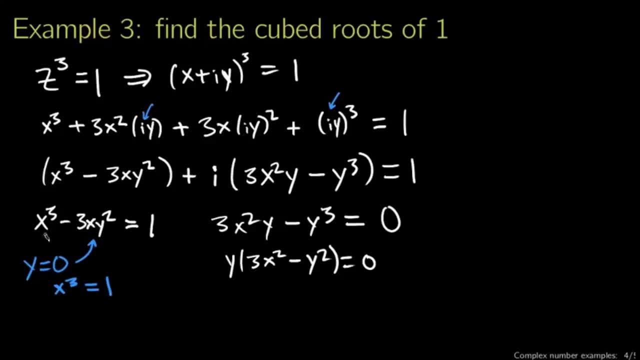 equation we started with: z cubed equals 1, but it's subtly different because z is a general, complex number, Whereas our assumption in starting the problem this way is that x is a purely real number. So a purely real number which, when cubed, 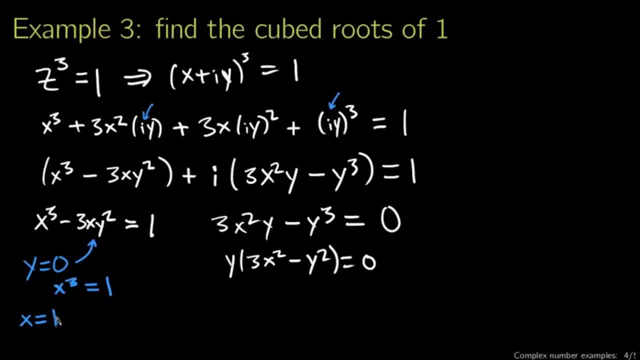 gives you 1, that means x equals 1.. So x equals 1,, y equals 0.. That's one of our solutions: z cubed equals 1.. Now we could have told me that right off the bat: z cubed equals 1.. Well, one possible. 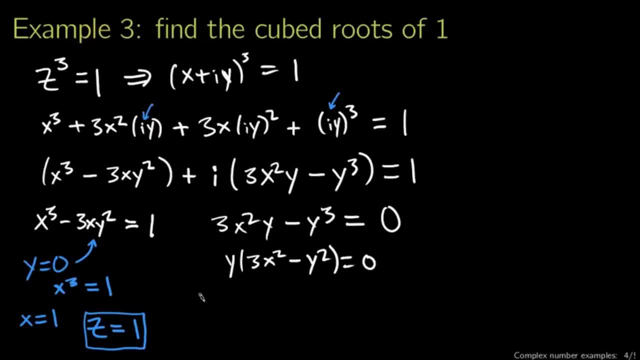 solution is that z equals 1, since 1 cubed is 1.. The other thing we can do here is we can say: 3x squared minus y squared is equal to 0. This means that I'll just cheat a little. 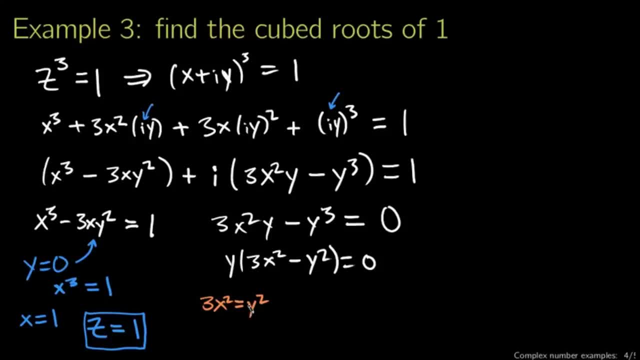 bit and simplify this: 3x squared equals y squared. Now I can substitute this in this y squared into this expression as well, And what you end up with is x cubed minus 3x, and then y squared was equal to 3x squared. 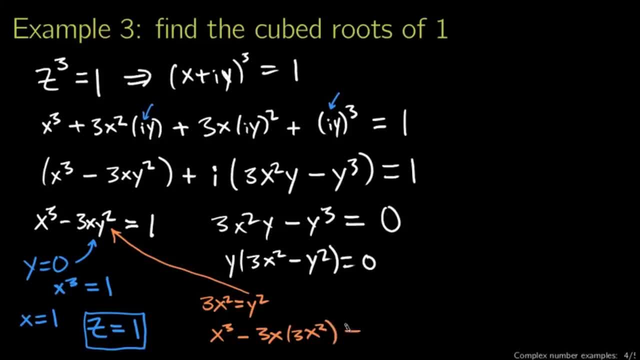 So 3x squared is going to go in there. That has to equal 1.. Let's move up here. What does that leave us with? That says x cubed minus 9x cubed equals 1.. So minus 8x cubed equals 1.. 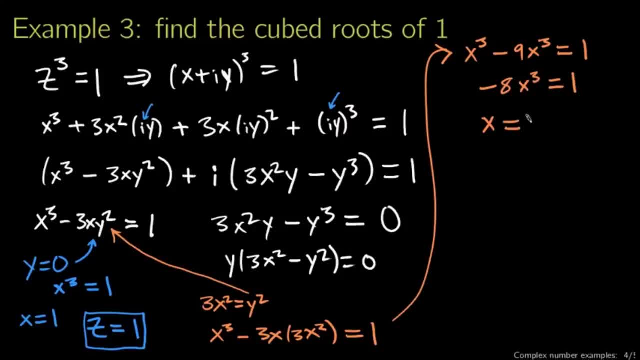 This means x, again being a purely real number, is equal to minus 1 half, Minus 1 half times minus 1, half times minus 1, half times 8 times minus 1 is equal to 1.. You can check that pretty easily. 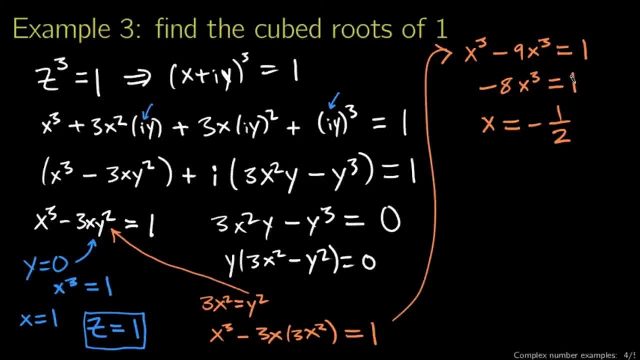 Now, where does that leave us? Where did I go? That leaves us substituting this back in to this expression which tells us that 3x squared equals y squared. x equals minus 1 half. so 3 minus 1 half squared equals y squared, which. 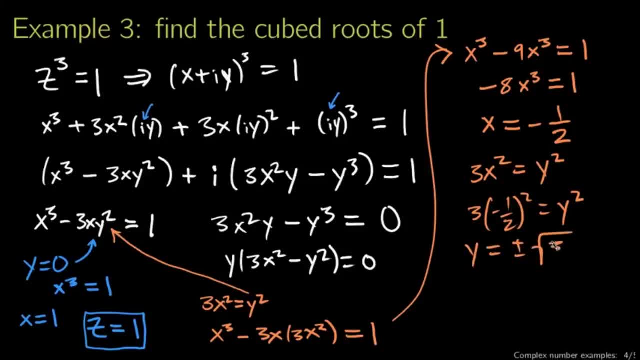 tells you that y equals plus or minus the square root of 3 fourths if you finish your solution. So now we have two solutions for y here coming from one value for x, and that gives us our other two solutions to this cubic. 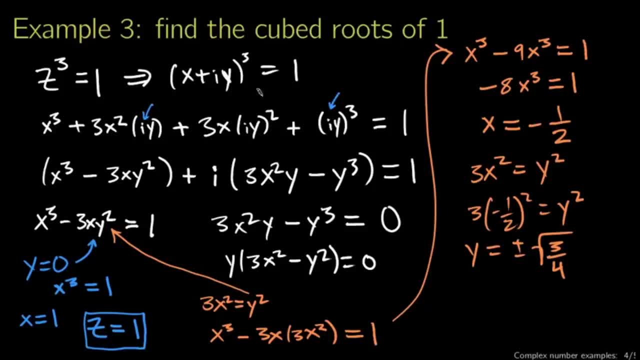 We have a cubic equation, we would expect there to be three solutions, especially when we're working with complex numbers like this. This is our other solution: Z equals minus 1, half plus or minus the square root of 3 fourths i. 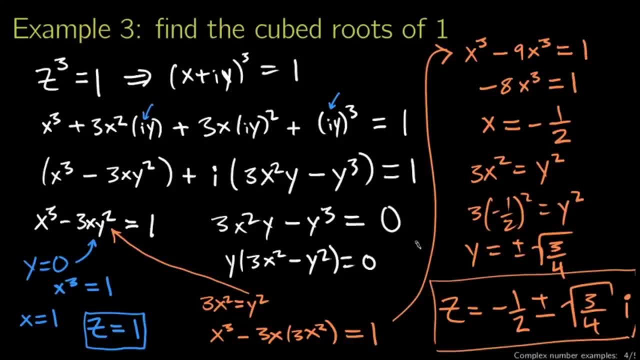 So those are our three solutions. Now, finding the cubed roots of 1 to be these complex numbers is not necessarily particularly instructive. However, there's a nice geometric interpretation: The cubed roots of unity. like this: the nth roots of unity doesn't have to be a cubed. 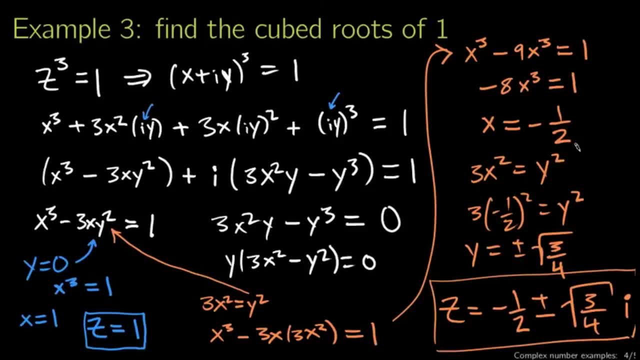 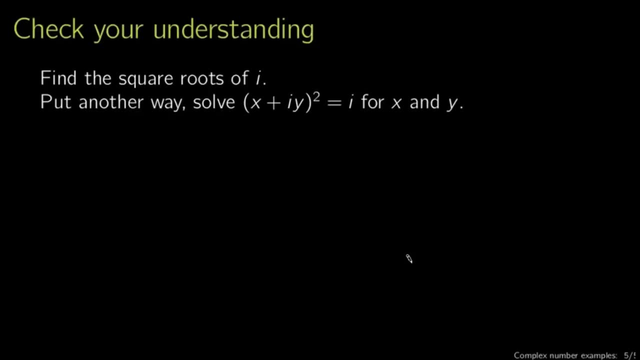 root all lie on a circle of radius 1 in the complex plane And if you check the complex magnitude of this number and the complex magnitude of this number, you will find that it is indeed unity. To check your understanding of this. a slightly simpler problem is to find the square roots. 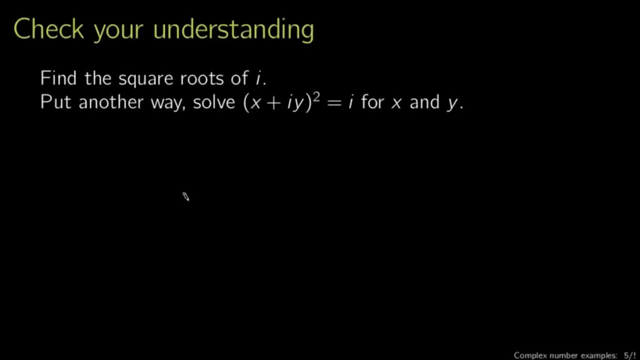 of i, Z equals minus 1 half. Put another way, you've got z, some generic complex number here. equals to x plus i, y Quantity squared. if that's going to equal y will expand this out. solve for x and y. 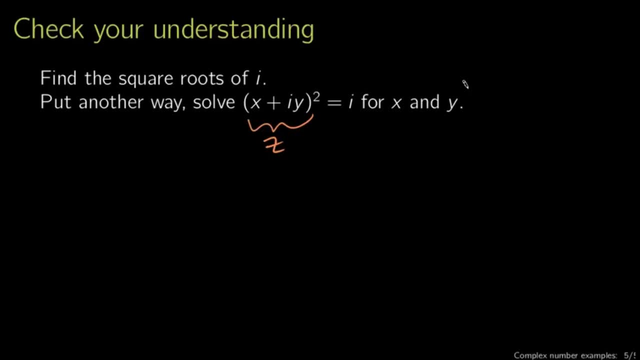 in the two equations. that will result from setting real and imaginary parts equal to each other And same. as with the cubed roots of 1, the square roots of i will also fall on a circle of radius 1 in the complex plane. So those are a few examples of how complex numbers can actually be manipulated in particular. 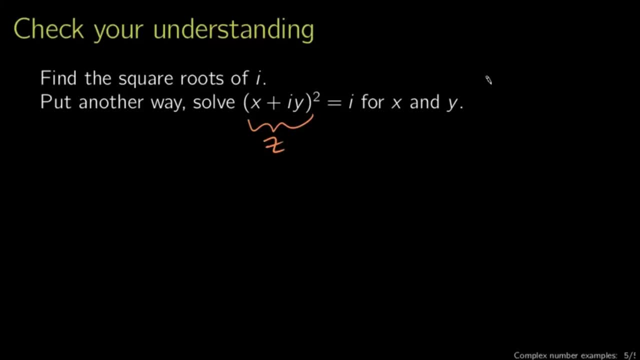 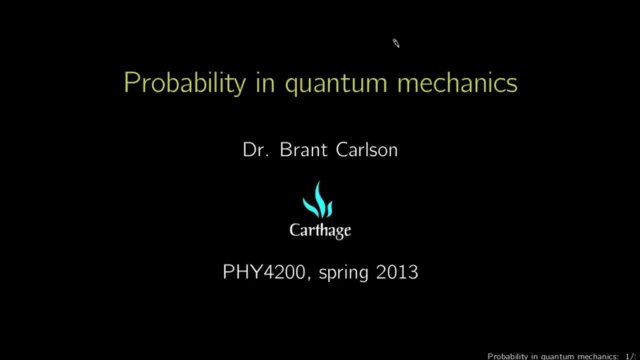 finding the roots of unity. There are better formulas for that than the approach that we took here, but I feel this was hopefully instructive. If probability is at the heart of quantum mechanics, what does that actually mean? Well, the fundamental source of probability in quantum mechanics is the wave function. 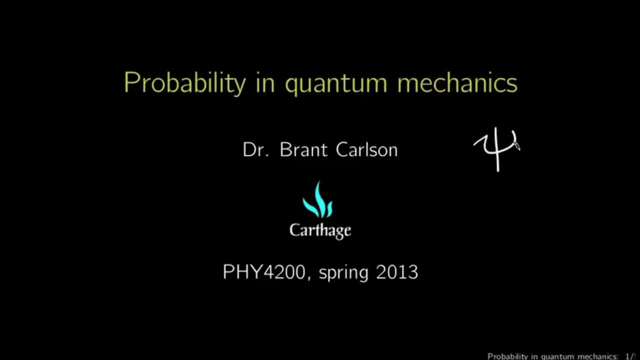 psi. Psi tells you everything that you can, in principle, know about the state of the system, But it doesn't tell you everything with perfect precision. How that actually gives rise to probability distributions in observable quantities like position or energy or momentum, is something that we'll talk more about later. but from 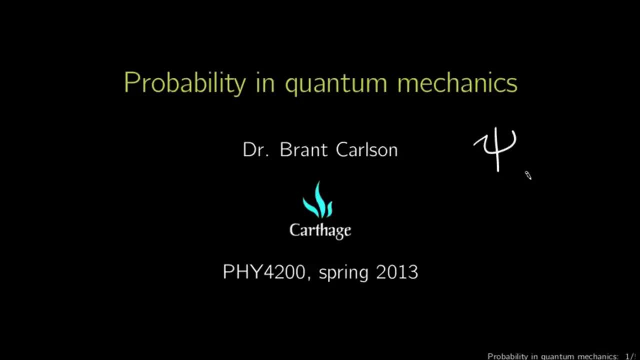 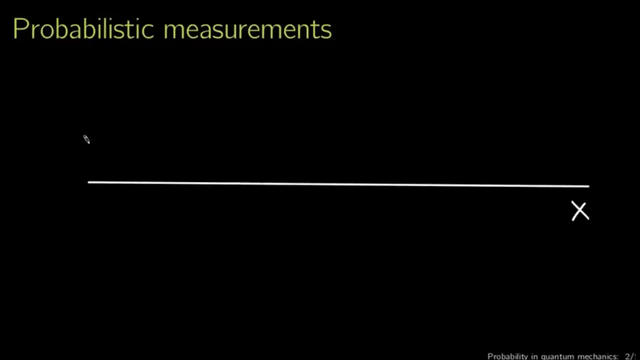 the most basic perspective, psi can be thought of as related to a probability distribution. But let's take a step back and talk about probabilistic measurements in general first. If I have some space, Let's say it's position space. Let's say: this is the floor of a lab and I have a ball that is somewhere on the floor. 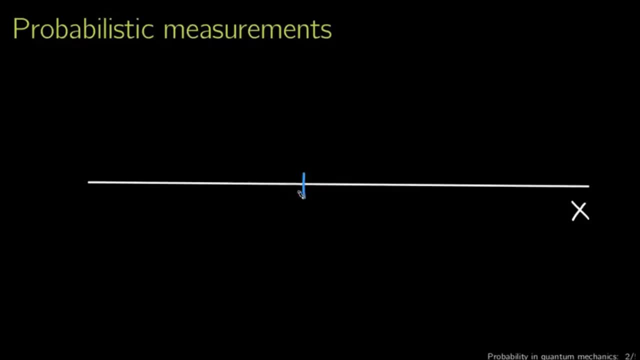 I can measure the position of that ball. Maybe I measure the ball to be there on the floor If I prepare the experiment in exactly the same way, attempting to put the ball in the same position on the floor and measure the position of the ball again. I won't always. 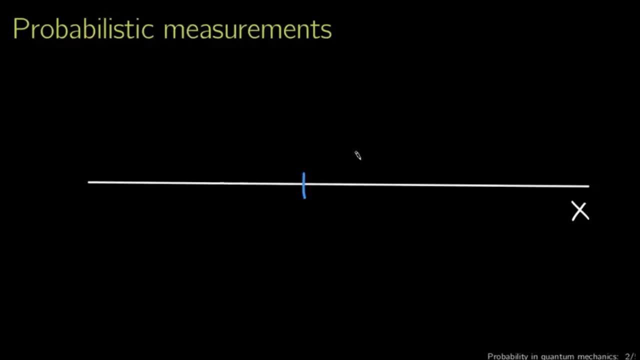 get the same answer. Because of perhaps some imprecision in my measurements. I can measure the position of the ball again. Maybe I have some precision in my measurements or some imprecision in how I'm reproducing the system, So I might make a second measurement there or a third measurement there. 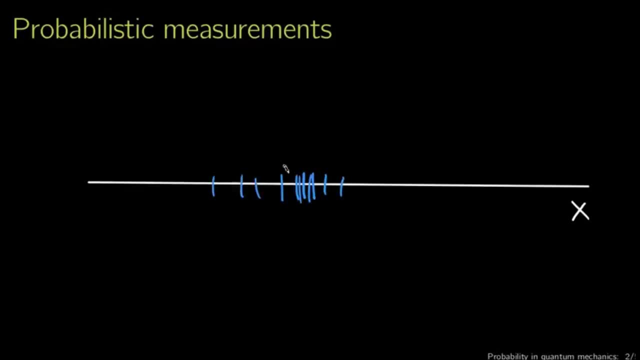 If I repeat this experiment many times I'll get a variety of measurements at a variety of locations And maybe they cluster in certain regions or maybe they're very unlikely in other regions. But this distribution of measurements, we can describe that mathematically with the: 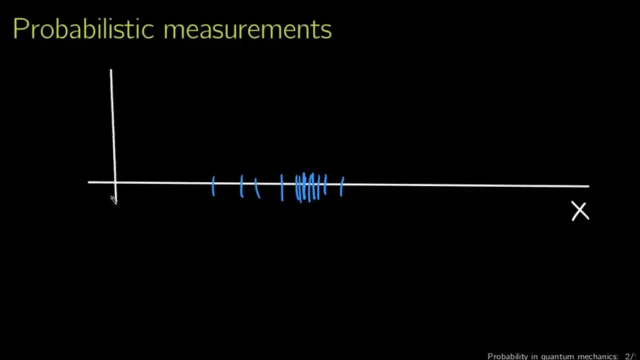 probability distribution. A probability distribution, for instance. I could plot p of x here and p of x tells you roughly how many or how likely you are to make a measurement. So I would expect p of x as a function to be larger here, where there's a lot of measurements. 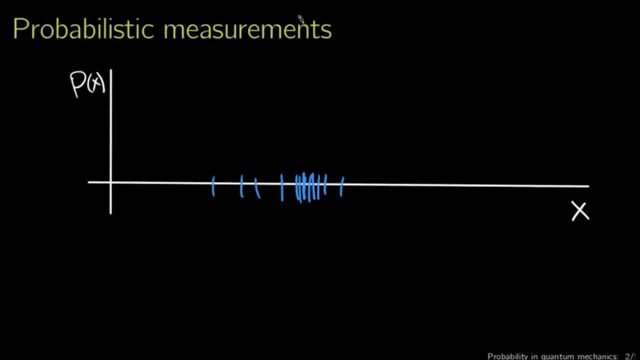 and zero here where there's no measurements, and relatively small here where there's few measurements. So p of x might look something like this: So the height of p of x here tells us how likely we are. So the height of p of x here tells us how likely we are to make a measurement in a given. 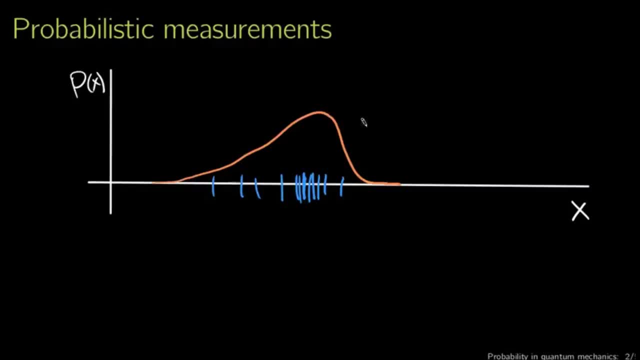 location. This concept of a probability distribution is intimately related to the wave function. So the most simple way that you can think of probability in quantum mechanics is to think of the wave function. psi of x. Now, psi of x, you know, is a complex function. 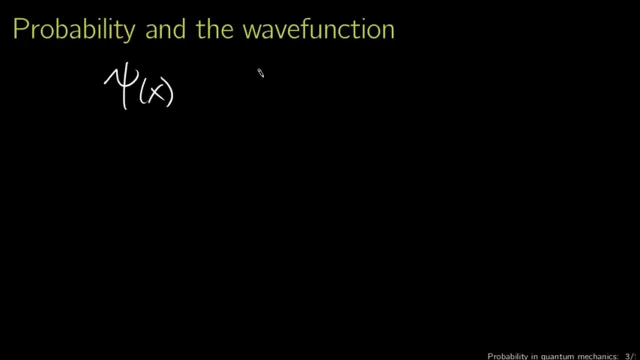 And a complex number can never really be observable. What would it mean, for example, to measure a position of, say, 2 plus 3i meters? This isn't something that's going to occur in the physical universe, But the fundamental interpretation of quantum mechanics, that most that your book this. 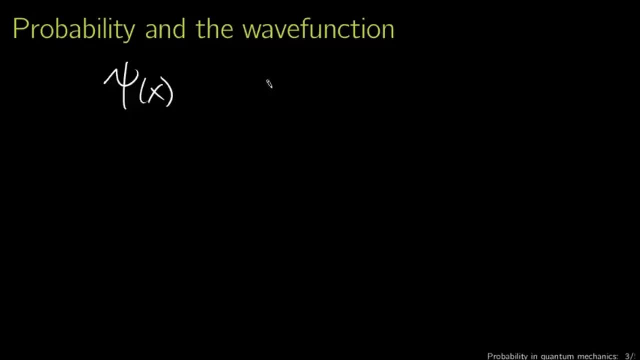 book in particular that most physicists think of is the interpretation that psi in the context of a probability distribution. the absolute magnitude of psi squared is related to the probability of finding the probability distribution of psi squared, And the absolute magnitude of psi squared is related to the probability of finding the 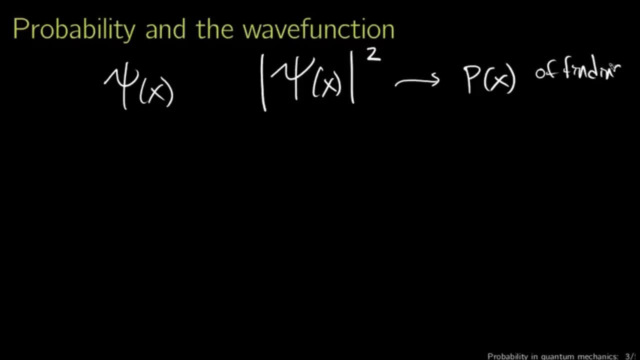 particle described by psi. So if the squared magnitude of psi is large at a particular location, that means it is likely that the particle will be found at that location. Now, the squared magnitude here means that we're not that we have to. well, we have. 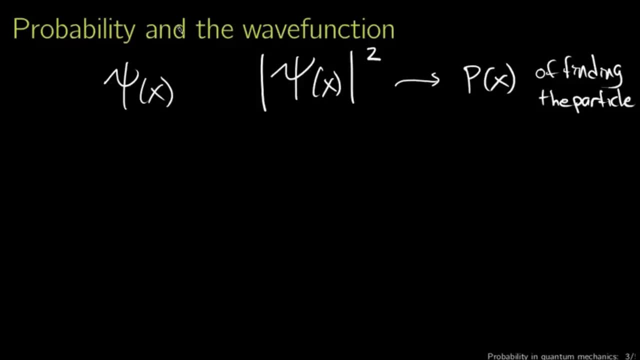 to take the squared magnitude of psi. We can't just take psi itself. So, for instance, in the context of the plot that I just made on the last page, if this is x and our y axis here is psi, psi has real and imaginary parts. 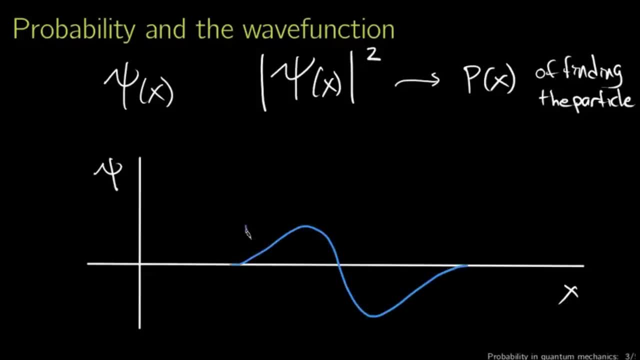 So the real part of psi might look something like this, and the imaginary part might look something like this, And the squared magnitude would look something like: Well, what you can imagine the squared magnitude of that function looking like. You can think of the squared magnitude of psi as the probability distribution. 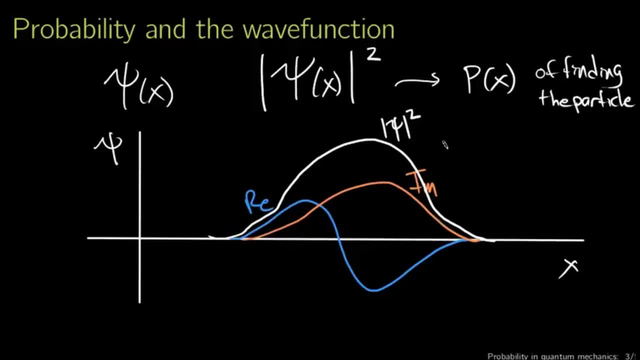 Let me move this up a little bit, get myself some more space. The squared magnitude of psi, then, can be thought of as a probability distribution in the likelihood of finding the particle at a particular location, like I said. Now, what does that mean mathematically? 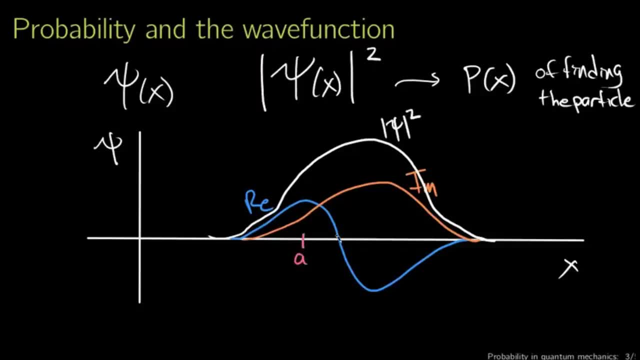 Mathematically. suppose you had two positions, a and b, and you wanted to know what the probability of finding the particle between a and b was. Given a probability distribution, you can find that by integrating the probability distribution. So the probability that the particle is between a and b 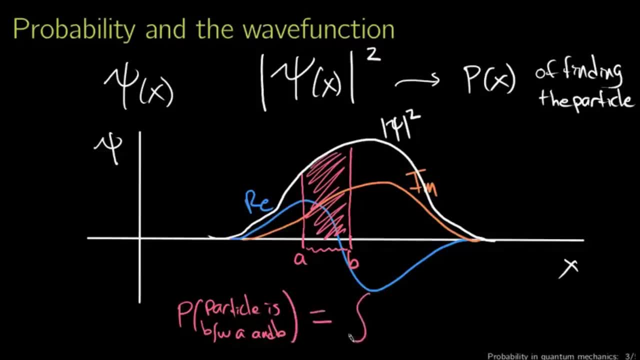 is the probability that the particle is between a and b. So the probability that the particle is between a and b is given by the integral from a to b of the squared absolute magnitude of psi dx. You can think of this as a definition. 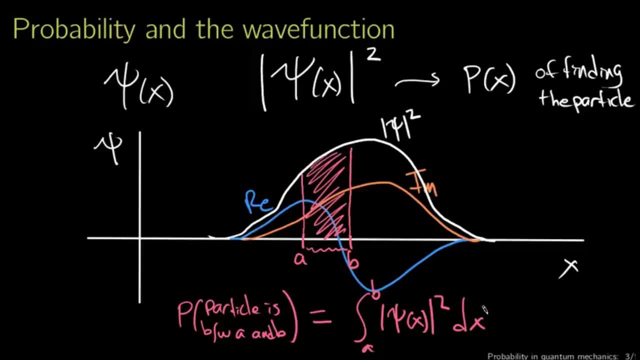 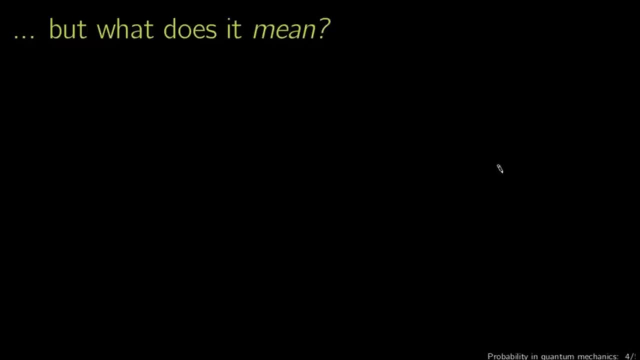 You can think of this as an interpretation, But fundamentally, this is what the physical meaning of the wave function is. It is related to the probability distribution of position associated with this particular state of the system. Now, what does that actually mean? And that's a bit of a complicated question. 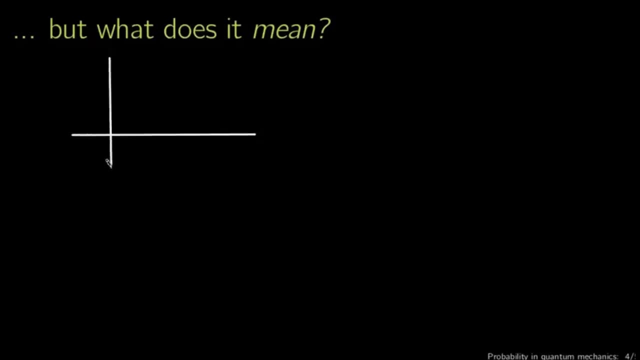 It's very difficult to answer. Suppose I have a wave function which I'm just going to write as the squared magnitude of psi. now Suppose it looks something like this: Now that means I'm perhaps likely to measure the position of the particle somewhere in the middle here. 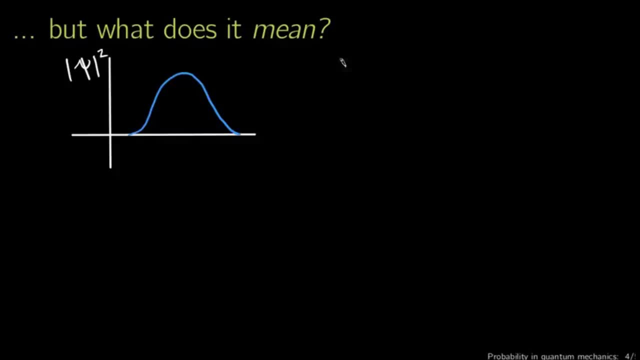 So suppose I measure the position of the particle here. So I've made a measurement. now Messy handwriting: I've made a measurement and I've observed the particle to be here. What does that mean in the context of the wave function? 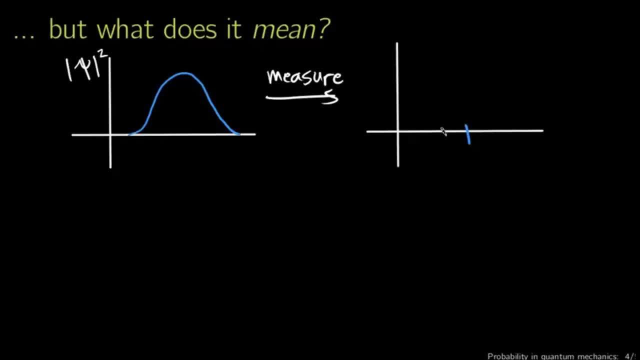 Now, everything that I can possibly know about the particle has to be encapsulated. Everything that I can possibly know about the particle has to be encapsulated. So after the measurement, when I know the particle is here, you can think of the wave function as looking something like this: 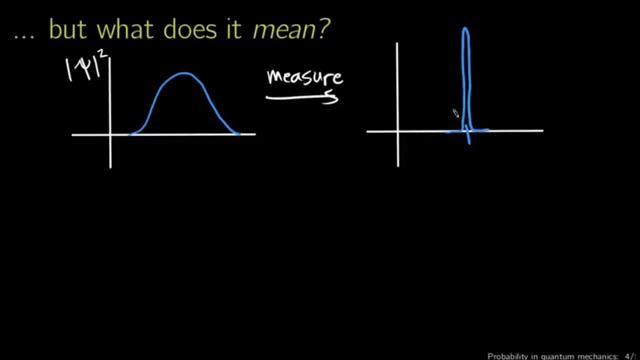 It's not going to be infinitely narrow because there might be some uncertainty. The width of this is related to the precision of the measurement, But the wave function before the measurement was broad like this and the wave function after the measurement is narrow. 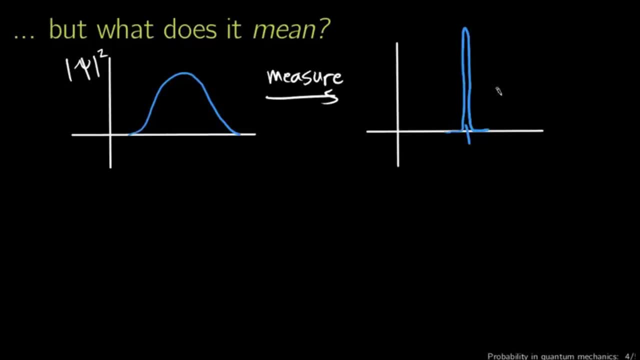 What actually happened here? What about the measurement caused this to happen? This is one of the deep issues In quantum mechanics that is quite difficult to interpret. So what do we make of this? Well, one thing that you could think just intuitively is that well, 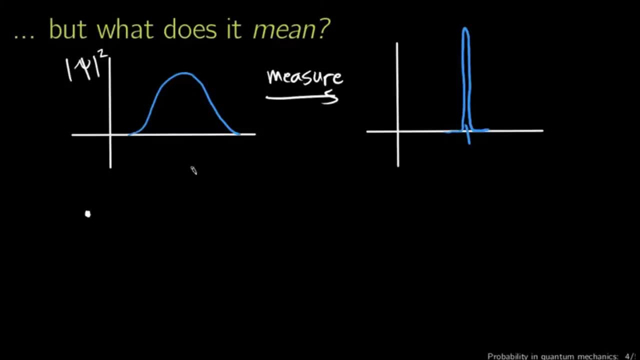 this probability distribution wasn't really all the information that was there Really. the particle was there. Let's say this is point C. One interpretation is that the particle really was at C all along. That means that this distribution reflects ignorance on our part as physicists. 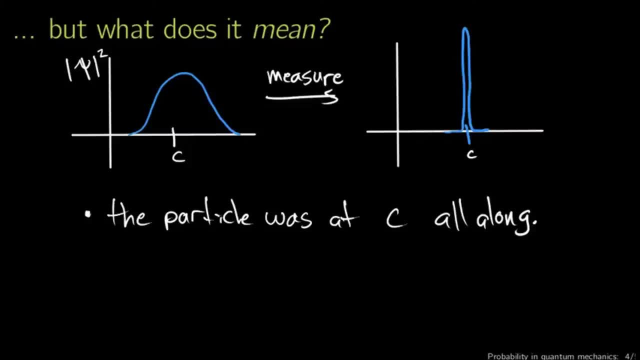 not fundamental uncertainty in the physical system. This turns out to not be true And you can show mathematically and in experiments that this is not the case. The main interpretation that physicists use is to say: let's say that this wave function, psi- here also shown here- collapses. 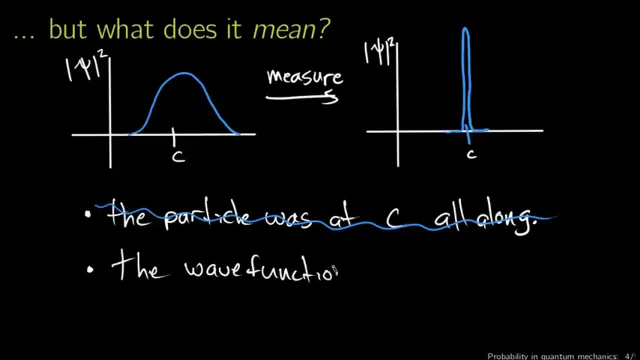 Now, that's a strange term- Collapses- But it's hard to think of it any other way. Suppose you were concerned with the wave function's value here: Before the measurement it's non-zero, Whereas after the measurement it's zero. 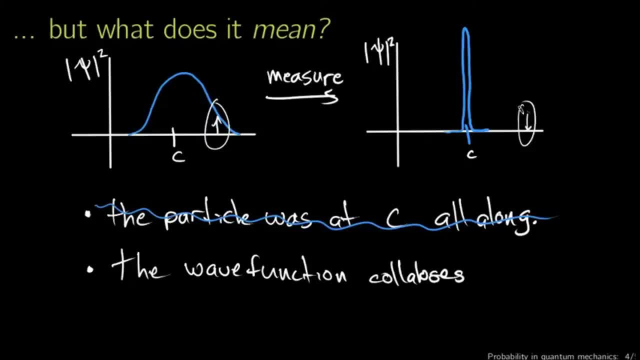 So this decrease in the wave function out here is a reasonable to call that a collapse. What that wave function collapse means is subject to some debate, And there are other interpretations. One interpretation that I'll mention very briefly but we won't really discuss very. 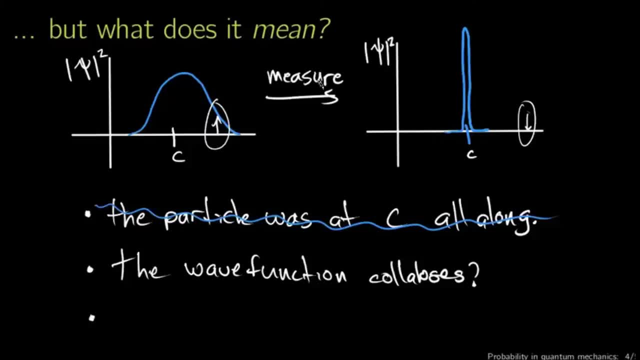 much is the many-worlds interpretation, And that's that when you make a measurement like this, the universe splits. So it's not that the wave function collapses, It's not that the wave function all of a sudden decreases here. It's that for us, in our tiny little chunk of the universe, the wave function is now this: 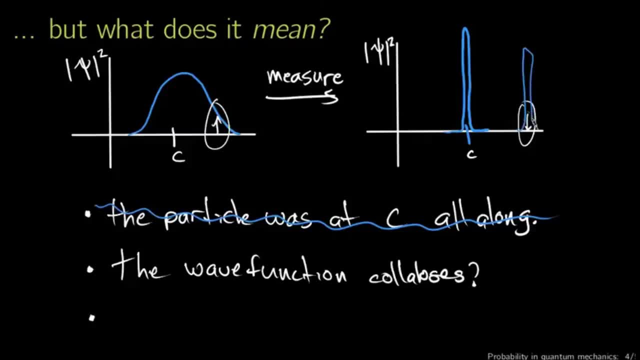 And there's another universe somewhere else, where the wave function is this, because the particle is observed to be here. Don't worry too much about that, but the interpretation issues in quantum mechanics are really fascinating. once you start to get into them, You can think about this as the universe splitting. 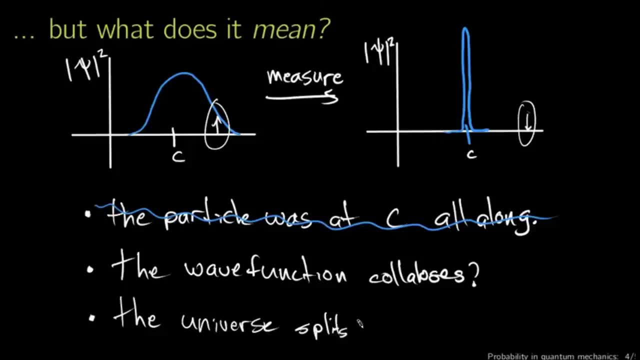 You can think about this as the universe splitting into many little sub-universes where the particle is observed at a variety of locations- One location per universe. really. This question of how measurements take place is really fundamental, but hopefully this explains a little bit of where probability comes from in quantum mechanics. 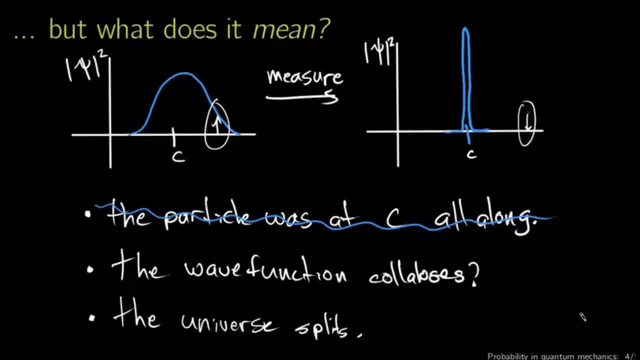 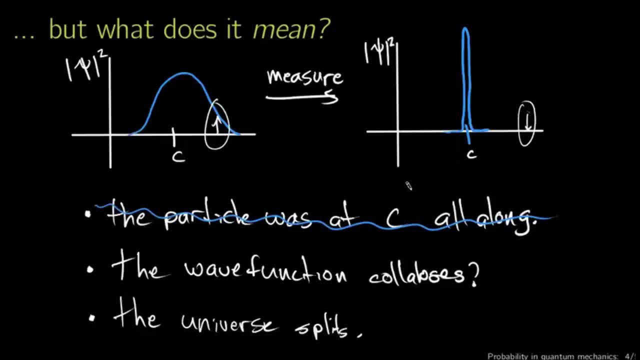 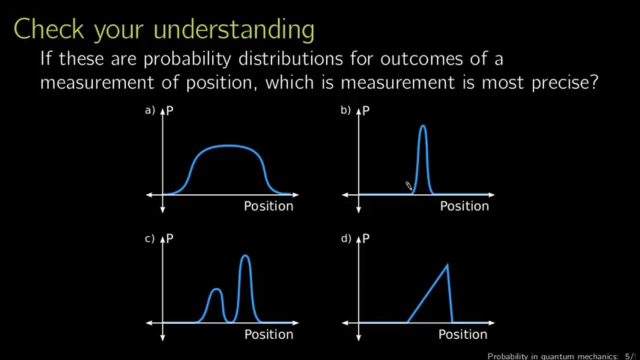 It can be thought of as a probability distribution for position measurements And unfortunately the measurement process is not something that is particularly easy to understand, But that's the fundamental origin of probability in quantum mechanics. To check your understanding, here is a simple question about probability distributions and how to interpret them. 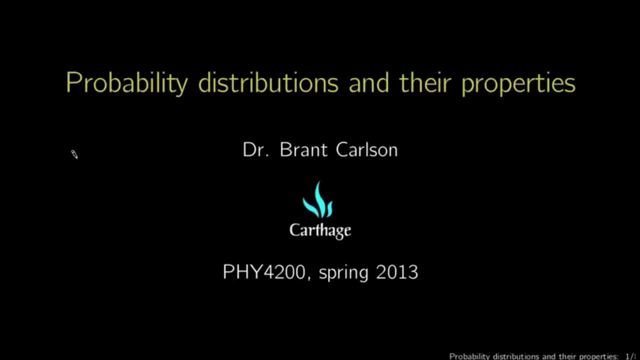 Since probability is so essential to quantum mechanics, it's good to go back and review it. go back and review to make sure we're all on the same page as far as probability. The fundamental concepts of probability, aside from probability itself, are probability distributions and what their properties are. So let's 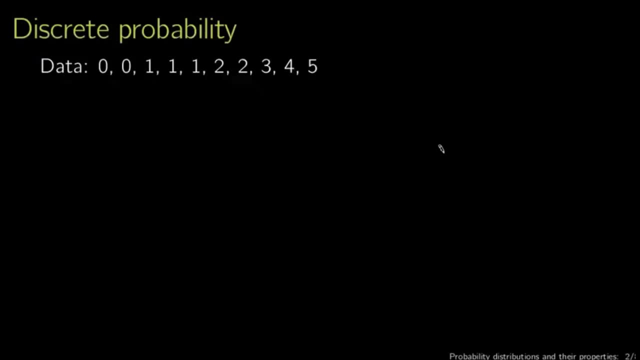 review probability. There are two main kinds of probability: discrete and continuous. Discrete probability is what you get if you have only a specific set of outcomes, hence the word discrete. You have a discrete set of outcomes, and these outcomes can be anything. They can be the outcomes of a 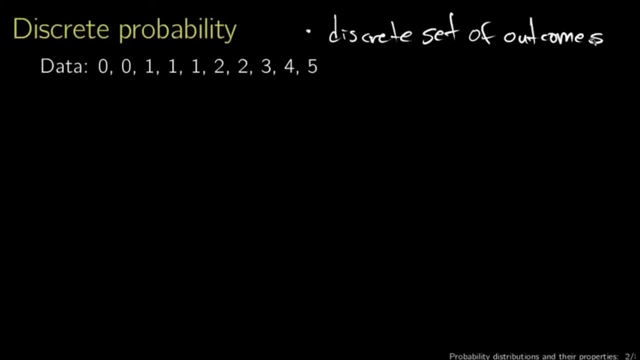 measurement. they can be responses in a survey. they can be any sort of data set. For example, if this is your data set: 0, 0, 1, 1, 1, 2, 2, 3, 4, 5.. Two zeros, three ones, two twos and one. 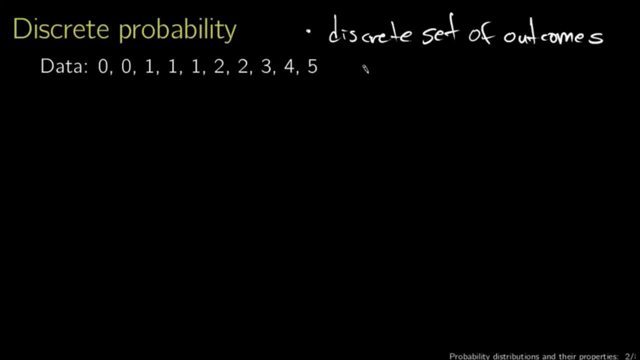 each of 3,, 4, and 5.. For instance, suppose you go out and you ask ten members of the general public how many sexual partners they've had. You might get a data set, something like this: The way to think of this in the context of a 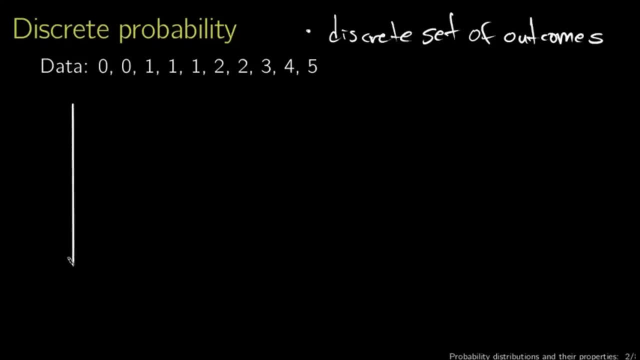 probability distribution. well, I like to plot things, So let's make a plot of this probability distribution. We have our outcomes: 0,, 1,, 2,, 3,, 4, and 5.. I've done my axis a little there. We have 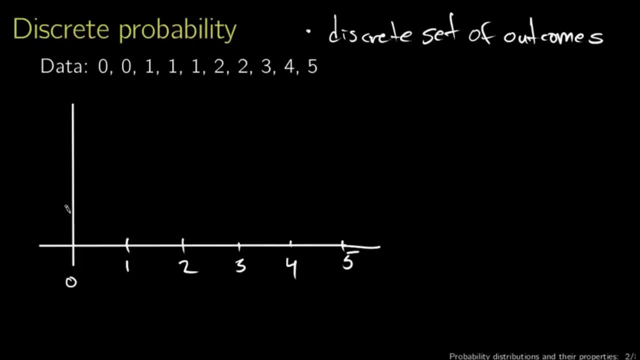 two people who answered 0, so if we make a y-axis here- 1,, 2,- I can put a bar here at 0 that goes up to 2.. There were three people that answered 1, so I should make. 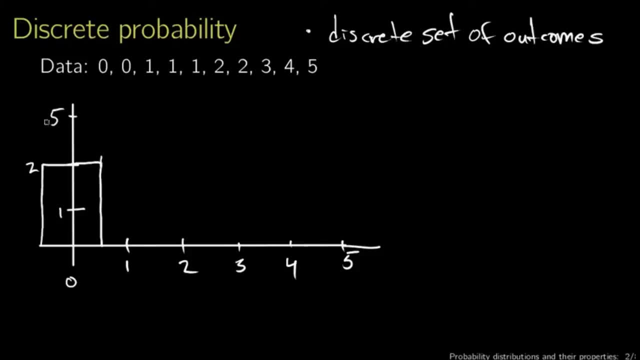 a bar that goes up to 3 above the 1,, 5, 3 above the 1.. Likewise for 2,. there were two answers for 2, and there were one each for 3,, 4, and 5.. 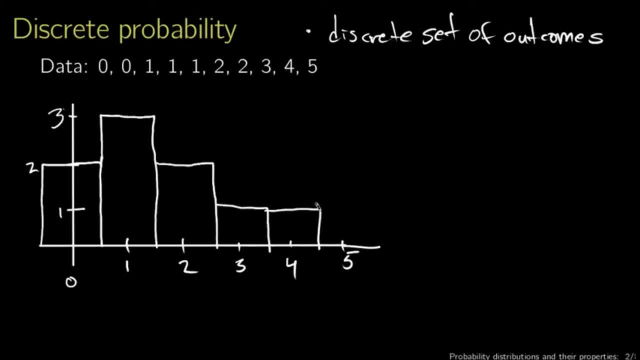 One there, one there and one there. Now our probability distribution looks like this when you plot it. What are we actually plotting? here We're plotting the number of people who responded for each particular answer here. We can make a table, then, of the probabilities. 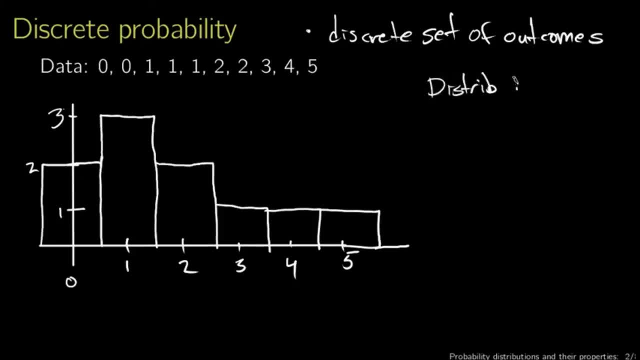 Either we have: on the left we have the value, and on the right we have the probability. Now, what is the probability under these circumstances? We have a discrete set of outcomes, six different numbers- 0 through 5, and the probability. 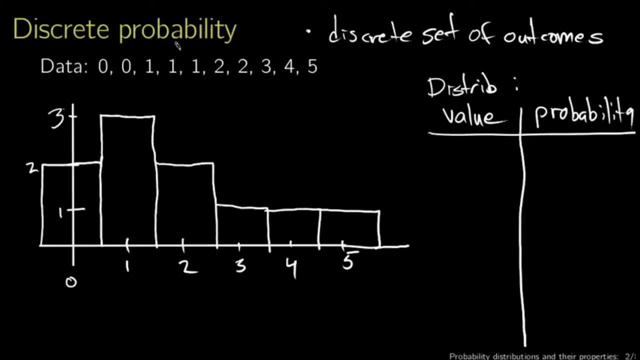 of, say, 3, is just the number of threes that appear in this data set divided by the total number of entries in the data set. So, for instance, if I want to know the probability of the value 1, well, there were two, sorry, let's start. 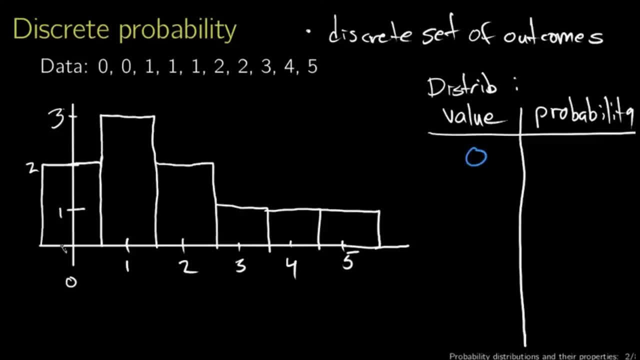 with 0.. If I want to know the probability of the value 0, there were two respondents, so that would be 2 divided by 10. Two people out of 10.. So if I chose one of these at random- not looking- 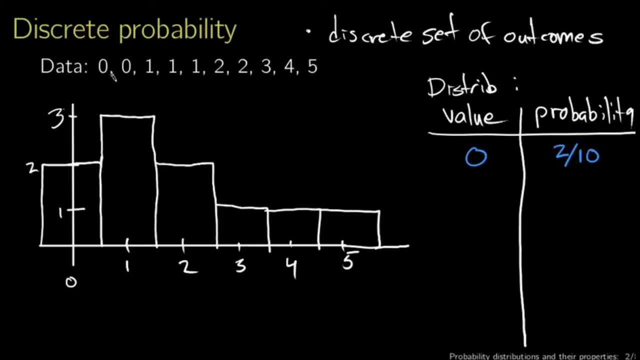 at the numbers, the likelihood that I would choose 0 is well, 2 out of 10.. Two times in 10, I would choose a 0 probability on average, And you can do the same thing for 1, 3. 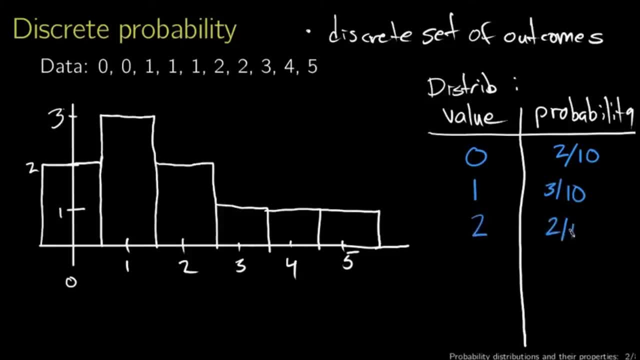 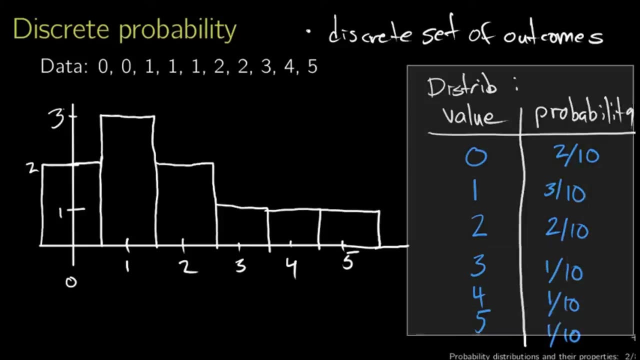 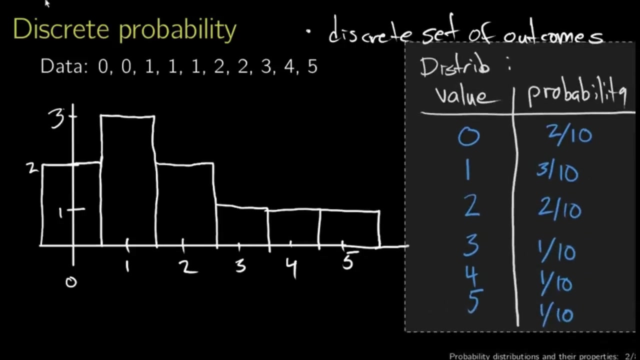 out of 10,, 2, 2 out of 10, again 3, 4, and 5, all 1 out of 10.. And some things you should notice about this. let me move it up slightly. move everything up the numbers. 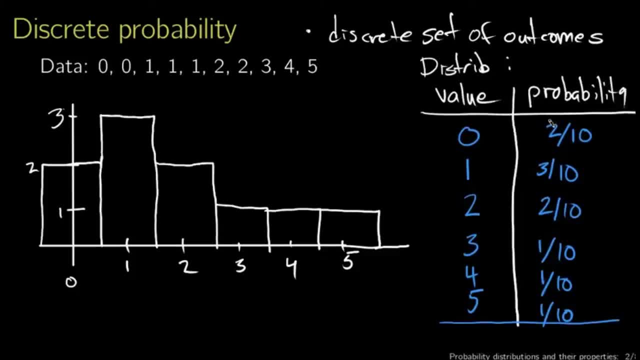 here. if I add these up- 2 plus 3 plus 2 plus 1 plus 1 plus 1, it adds up to 10 out of 10.. So the total probability of drawing any number is 1, and that is sort. 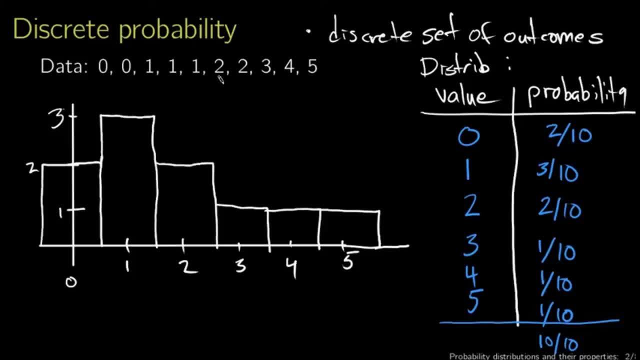 of a certainty: If you draw a number, you will draw a number. So if you only have a discrete set of outcomes, for instance the integers, like this, you're dealing with the discrete probability distribution and the sum of the probabilities in the discrete. 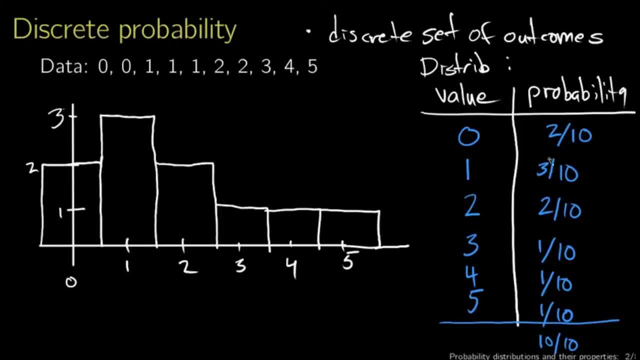 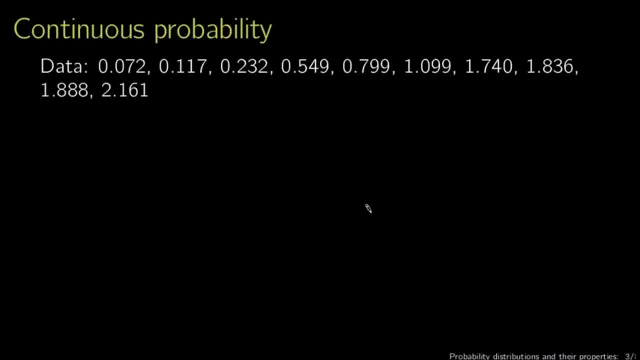 probability distribution: half the sum to 1, and it's a straight sum if I add up these numbers. The other class of probability distribution is a continuous probability distribution. Continuous probability distributions are what you work with when you have a range of values. a range of values, not a list of. 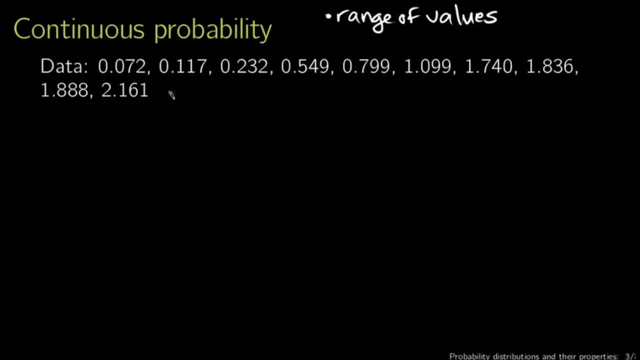 values. So, for instance, suppose you got this set of numbers, This might be what you would get if you talked to 10 people who had just gotten off the phone with Comcast tech support and asked them, for instance, how long did Comcast put you on hold, say in hours? 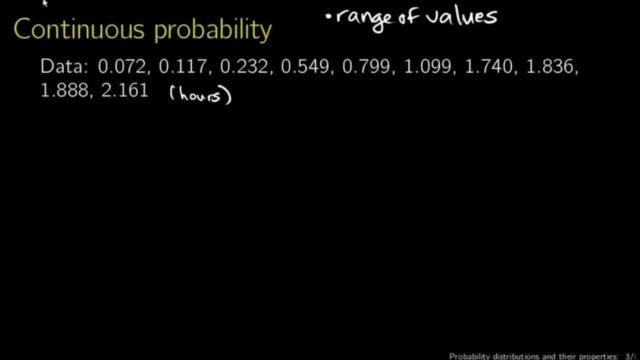 We can look at this probability distribution graphically as well, only it's slightly more complicated. Suppose the x-axis. now here is my time in hours and I have 1 and 2. Give a scale on my axis. Now, if I plot, 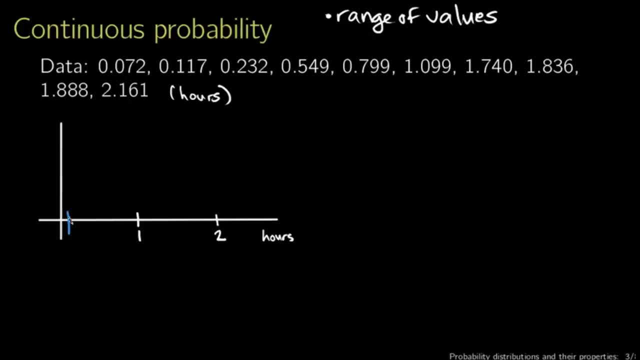 this data set. I've got one at like 0.7 or 0.07,, one at 0.11,, one at 0.23,, 0.55, 0.79,, 1.09,, 1.7, probably about there. 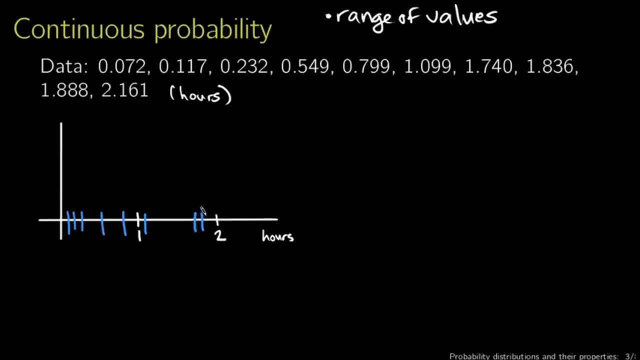 1.8,, 1.88, and 2.16, something like that. So these discrete answers: each answer here is only a specific number on this axis. So if I want to make a meaningful plot, I can either pretend that my 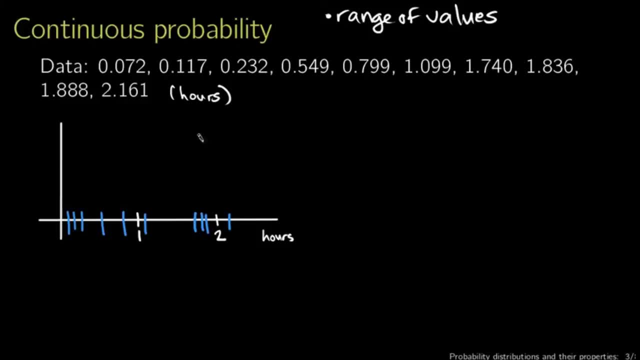 probability distribution is discrete, or I can attempt to guess at what the probability distribution looks like. Since I know what the answer is here, let's call this: row. of x is typically the name given to a continuous probability distribution, and it would look something like this in this case: 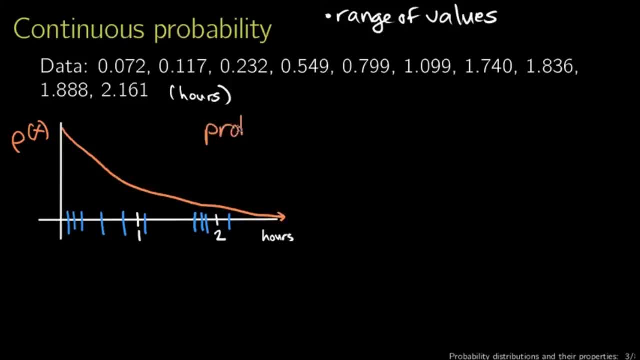 So we have what's called a probability density function, or just a probability density rho of x. Now the reason we have a probability density like this rho of x, is because x is a continuous variable. now It can be anything in this case, say, from 0 to infinity. 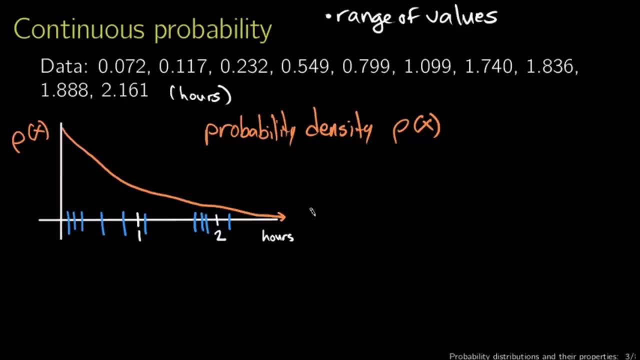 What does that mean? If I evaluate rho of x at say, x equals 1, you might think: well, okay, that's the probability of 1.. But one of the three fundamental facts of continuous probability distributions is that the probability that x is exactly equal to 1. 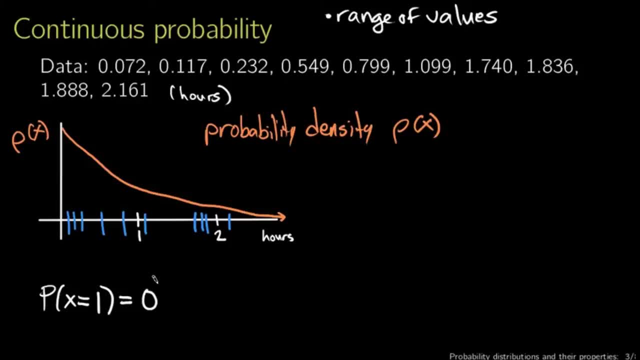 is going to be 0.. The example given in the text. the text is: suppose you walked up to a random person on the street and asked: is your age? 18 years, 3 months, 12 days, 18 minutes, 16 seconds, 52 microseconds, etc. 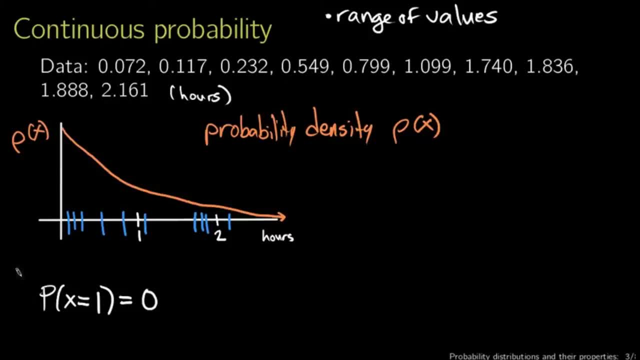 If you precisely specify the exact answer you want, the probability that you'll get that exact answer is going to be 0.. The only reason or the only way that makes sense for a continuous variable or continuous probability is for the probability to be specified between limits. 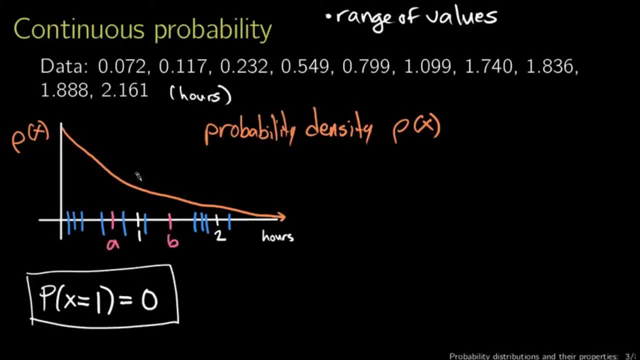 Suppose I had a and b and I want to know the probability that the number that you're drawing from this distribution or the random probability of the amount of time that you would like to have to spend on hold with Comcast between, say, 45 minutes and an hour and 45, or an hour and a half. 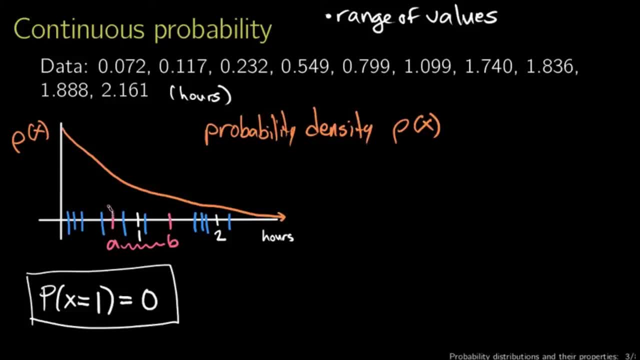 you could calculate that knowing this function. And the way you calculate it is by integrating, Put mathematically, the probability that say x is between a and b is the integral from a to b of rho, of x, dx. 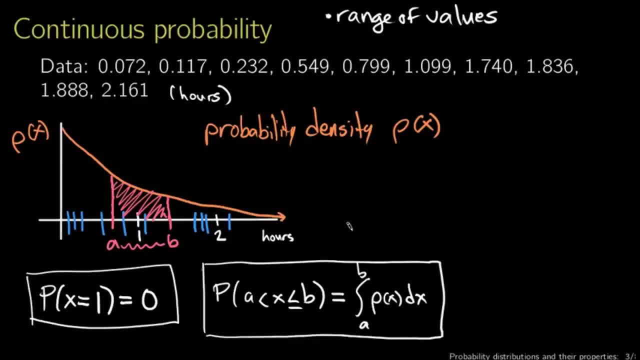 You can think of this more or less as the definition of the probability density function. If you have a way of calculating probabilities for x's and ranges, that is the probability density function. Probability density functions also have to sum to one, but instead of having a sum, 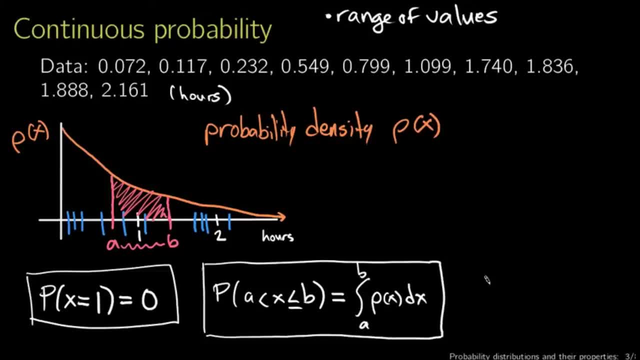 in the case of discrete probability distribution we have an integral. So the other property here is that the integral, from minus infinity to infinity, the entire possible range of values, rho of x, dx, has to equal, not zero, has to equal one. 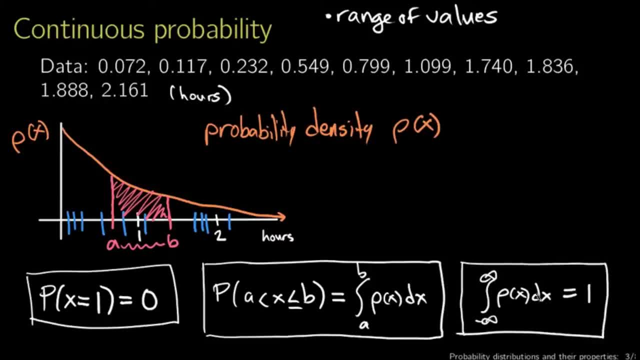 The answer, or the question that this equation here answers is: what is the probability of drawing a number in between negative infinity and positive infinity, And that had better be unity. This is the equivalent of the sum of the probabilities in a discrete probability, distribution being equal to one. 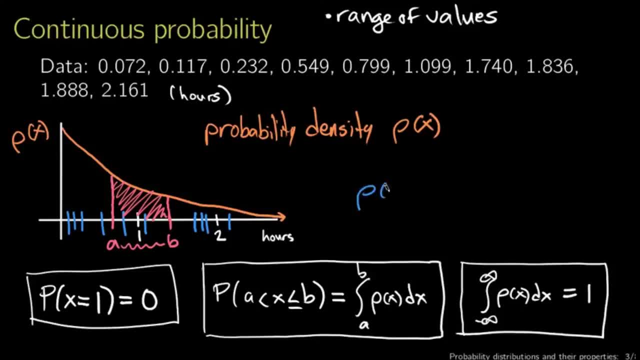 Now, in this case, the probability distribution, to give you a feel for what these things look like, rho of x, in this case, is zero. if x is less than zero and is equal to e to the minus one, e to the minus x, 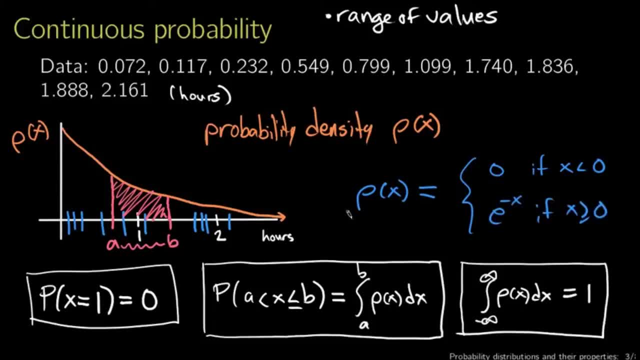 if x is greater than or equal to zero. So this is an example of a probability distribution function or probability density. That's actually the distribution I used when I drew these numbers. So that's continuous probability If you have a continuous range of outcomes. 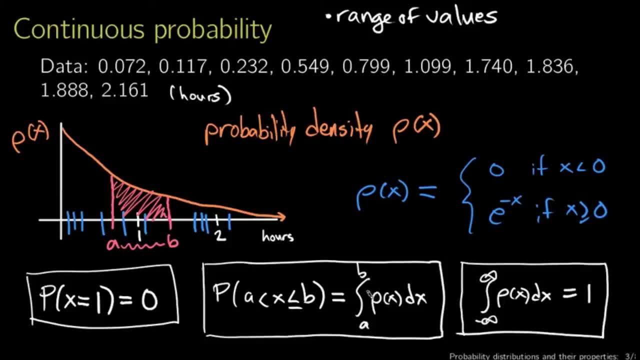 you have to deal with probability distributions and your probability density functions, and you have to do some integrals if you want to calculate properties. Now, what are those properties? Well, the most basic properties that you can think of is probably the most likely outcome. 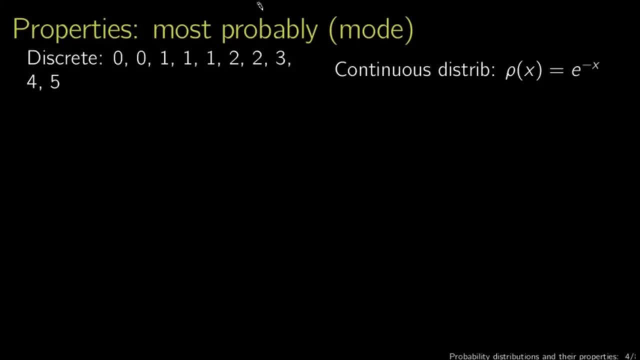 Now, in the case of a discrete probability distribution, this is just the most probable. What that means is that you've got the highest probability, And in this case, that means it's just the outcome that occurs the most times, In this case, one. 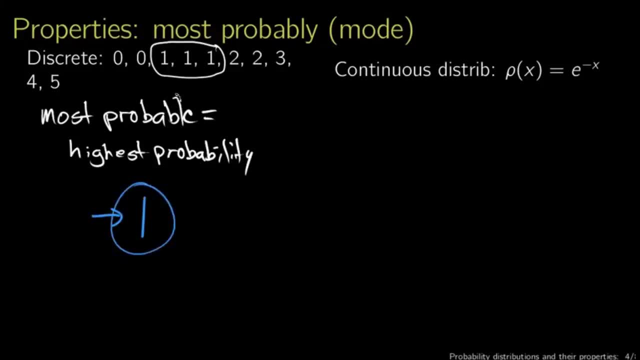 So our most probable outcome here is one: In the case of a continuous distribution, it's slightly more complicated If I plot the distribution function from before the exponential turn off the ruler. if I plot the probability distribution from before, it looks something like this: 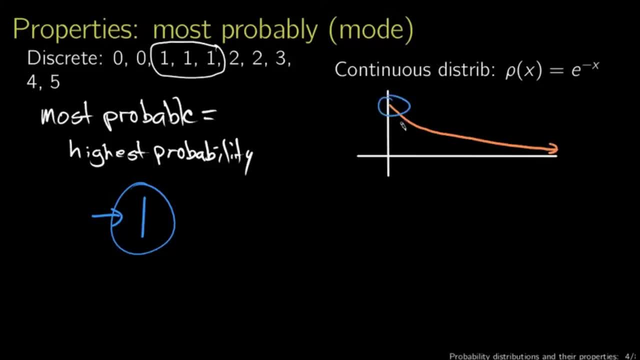 The most probable is actually going to be zero. Now you might think: what are the odds that Comcast puts me on hold for zero minutes? Well, zero. That's our rule: that the probability that x is exactly equal to zero is zero. It only makes sense to make a statement like the probability. 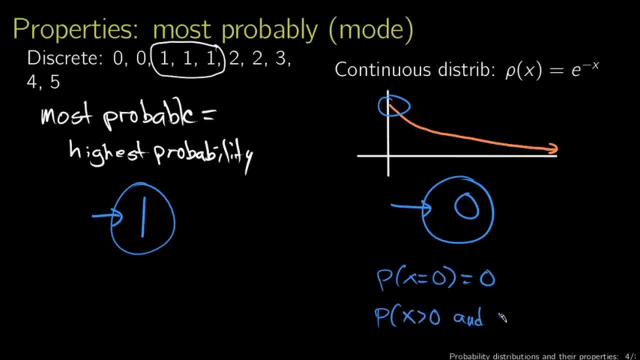 that, say, x is greater than zero and x is less than, say, five minutes, And that you can calculate with your integral, like on the last page. But in the case of the most probable value, the peak of the distribution is indeed zero. here 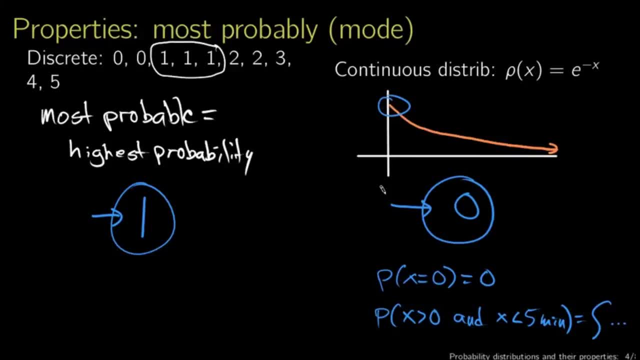 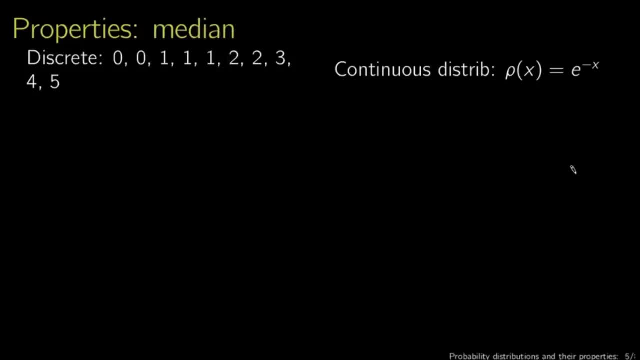 in spite of the fact that zero will effectively never happen. Any exact value will effectively never happen, but zero is the most likely. The next property is the median Median is not something that appears very often in physics, but it appears a lot in statistics. 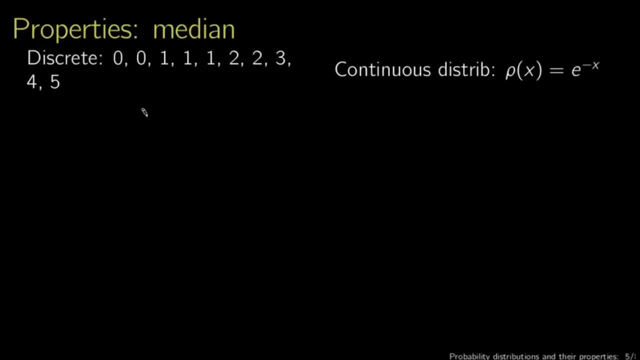 so we need to mention it. The median is essentially the middle of the data set. So you've got half are smaller and half are larger than the median. So here I have ten numbers. The median is going to be something that falls in between one and two. 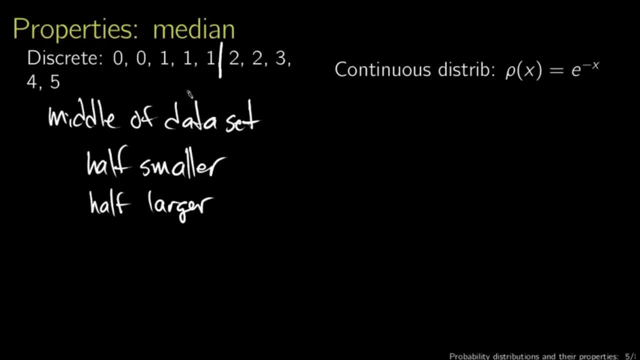 Half the data set, 00111, is smaller and 22345 are all larger. Typically, what statisticians do when they define the median here, when there's no exact number, that is the median, is to just put it halfway between the numbers. 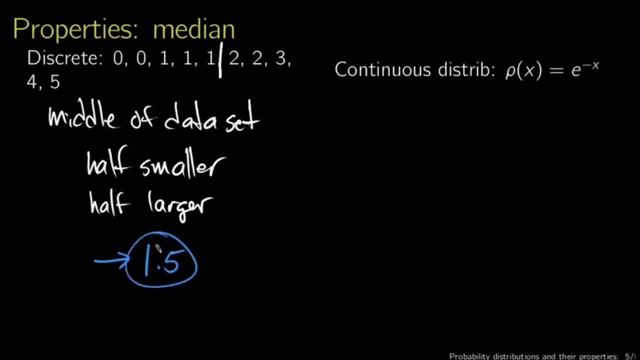 So in this case the median would be 1.5. In the context of a continuous probability distribution, the median is the number such that your probability adds up to a half. So if I integrate from minus infinity the lower possible limit that you could possibly, 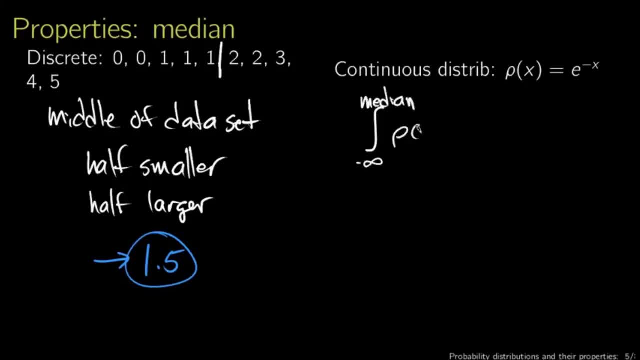 have up to the median rho of x- dx, I would get 0.5.. So in the case of this probability distribution function, e to the minus x, I can write that out. This integral from 0 to, I'll just call the median m. now. 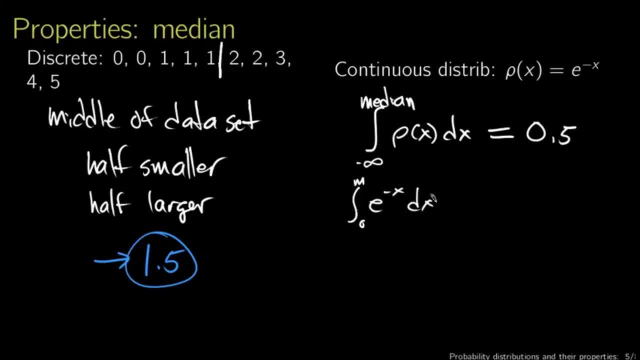 e to the minus x is rho of x- dx. Now I constructed this integral from 0 to m instead of from minus infinity to m, because this probability distribution is 0 for x less than 0, just to make sure that it's clear why I used 0 here. 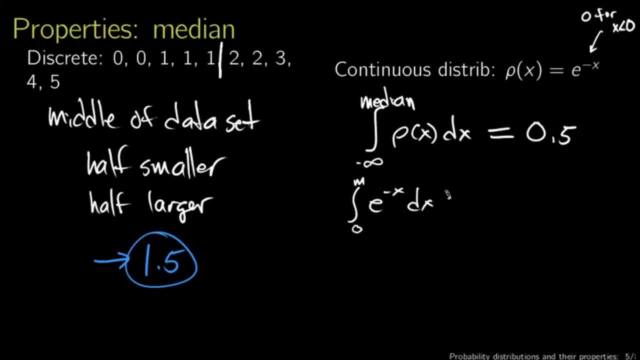 That's not actually a 6,, that's a 0. So if you do this integral, you know the integral of e to the minus x is minus e to the minus x. Hopefully. if you don't, you need to review some calculus. 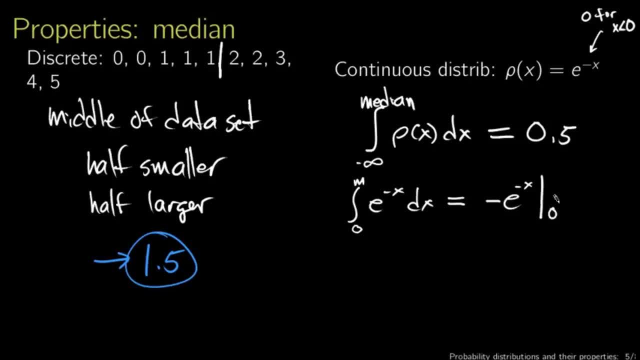 There will be a lot of integrals like this in quantum mechanics, Evaluated between 0 and m, and that has to be equal to 0.5.. Plugging in the limits here you get. well, I'll just simplify it and skip a step here. 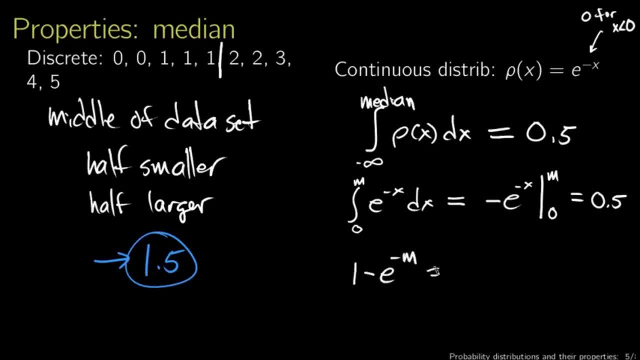 you get 1 minus e to the minus m equals 0.5, which, if you solve it for m, gives you that m equals the log of 2.. Now if I get sloppy and say log, here I really mean natural log. 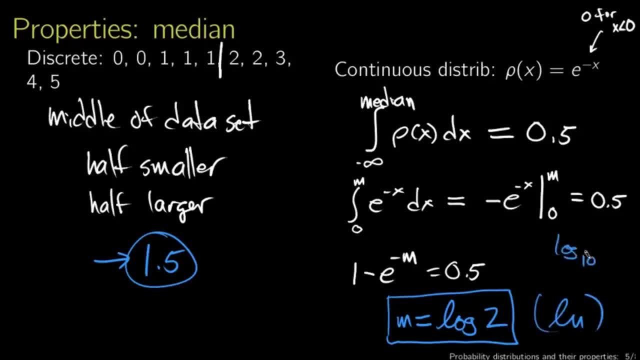 Log. if I ever need a log base 10, I'll write log base 10.. Most of the time, we'll be using natural logs in quantum mechanics. So that's the median. The next property, and this is one that will be very common. 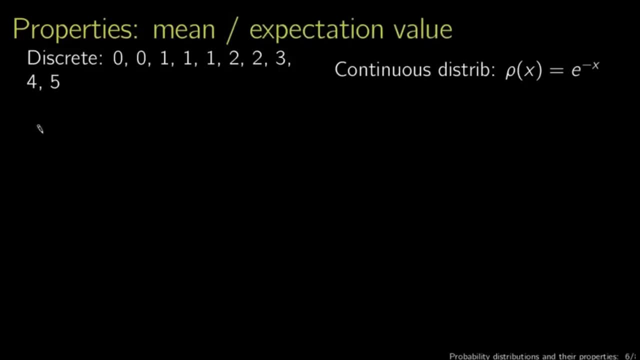 is the mean. The symbol that we use for the mean is mu and in the case of a discrete probability distribution, mu is the sum over all of your outcomes, of the outcome x sub i times the probability that, let's say, x is x sub i. 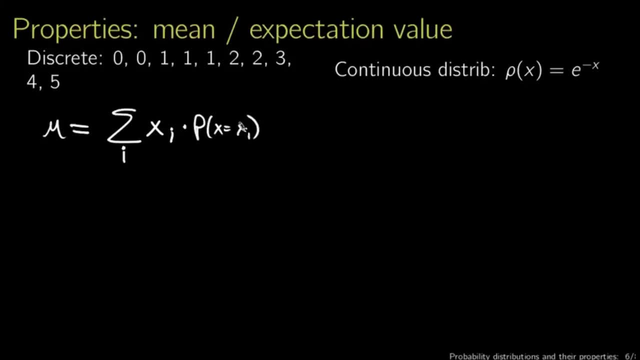 Sometimes this is just written as the probability of x sub i, which makes sense in the context of a discrete probability distribution. So what this looks like in the case of the discrete probability that I gave you earlier is: well, there's 0, that's x sub i. 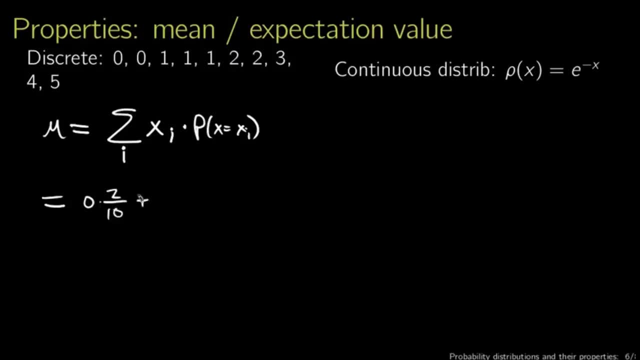 times the probability that x equals 0,, which was 2 tenths plus 1, that's x sub i times the probability that x equals 1,, which was 3 tenths plus 2,. x sub i times the probability that x is equal to 2,. 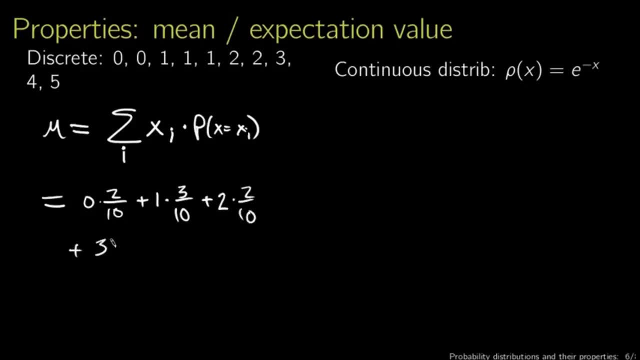 which is 2 tenths, And you can keep going plus 3 times 1 tenth, plus 4 times 1 tenth, plus 5 times 1 tenth, for 3,, 4, and 5,, all of which have probability 1 tenth. 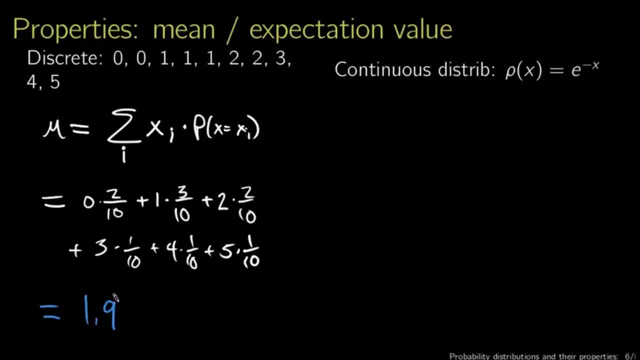 And if you run through the numbers you'll find this is equal to 1.9.. If you remember from an earlier class that the mean is the sum of the values divided by the total number of values that you added up, that's the same formula as this. 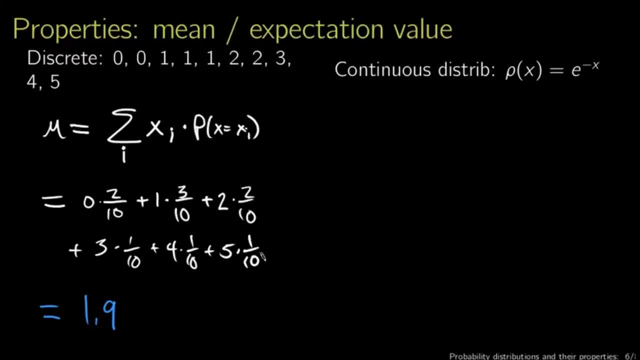 if you say, factor the 1 tenth out, All of these numbers have a 1 tenth and if we factor that out, we'll get 0 plus 0 plus 1 plus 1 plus 1 plus 2 plus 2 plus 3 plus 4 plus 5,. 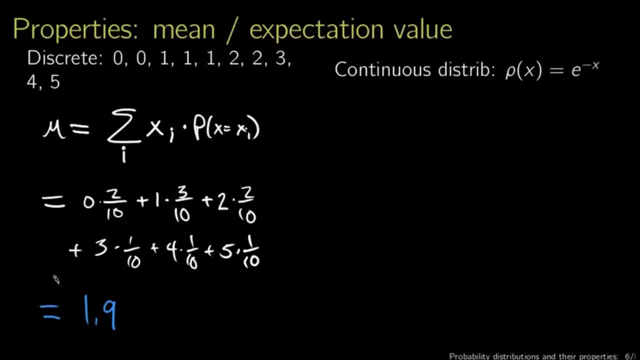 which is what you would get if you added all this up And you get the same answer. So there's no black magic there. The reason I'm writing this this way is this format here, where you have something times the probability of that something is something that shows up repeatedly. 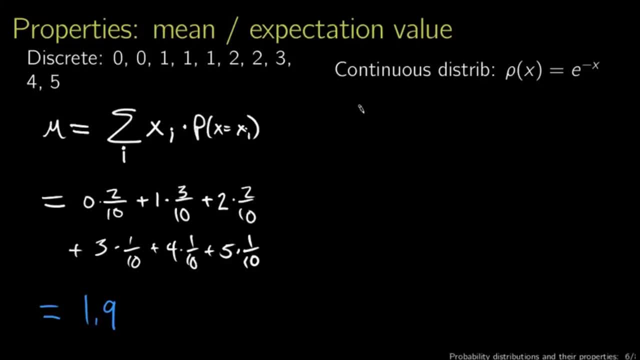 In the context of a continuous distribution, for example, the mean mu. now, instead of a sum, we have to have an integral. and instead of a sum over all possible values, we'll have an integral over all possible values, minus infinity to infinity. 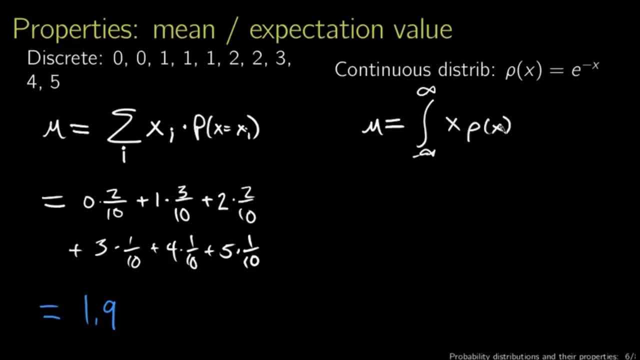 of x times the probability density rho of x, dx. Now if I plug in this example, we'd be integrating again from 0 to infinity, so that I don't have to worry about if I integrate from minus infinity to 0,. 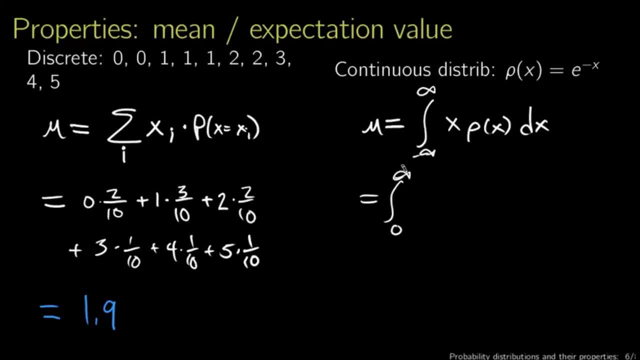 the probability density is going to be 0 for that entire range, So I can ignore that and just start my integral at 0, and then I would have x e to the minus x dx. Now, whenever you see an integral like this, hopefully you think integration by parts. 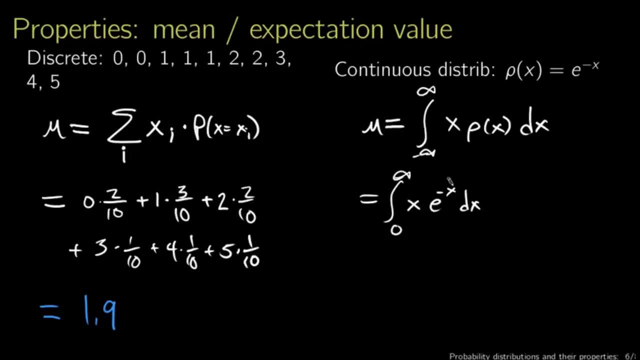 The way I like to do integration by parts is to try and figure out, probably just by trial and error, which pieces of this equation are going to become which of the parts that I'm going to use In this case. let's say u equals x. 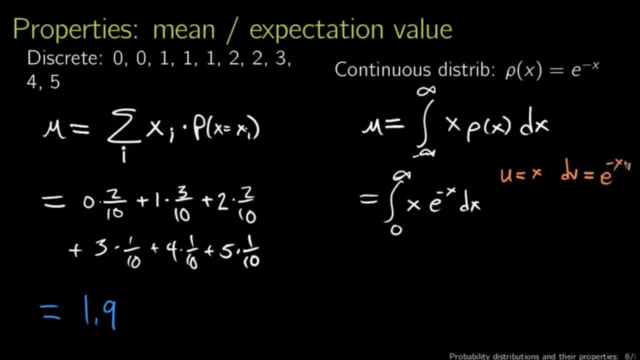 and dv equals e to the minus x dx. Now you differentiate this: du equals dx. and you integrate this: v equals minus e to the minus x. Now, in integration by parts, the forms that don't have any differentials in them. 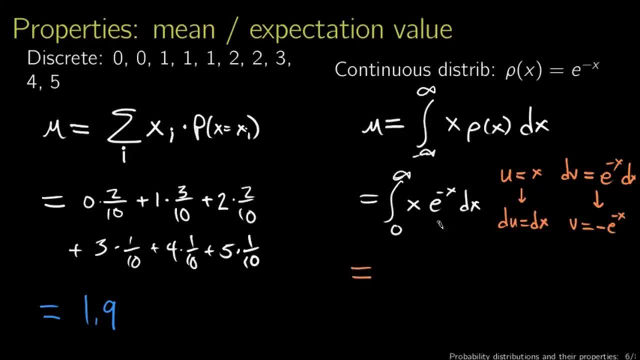 that's your leading term. so we would have this: integral is equal to x, e to the minus x, with a minus sign evaluated at the limits 0 and infinity. Then we have a minus sign and the integral part of the integration by parts. result: 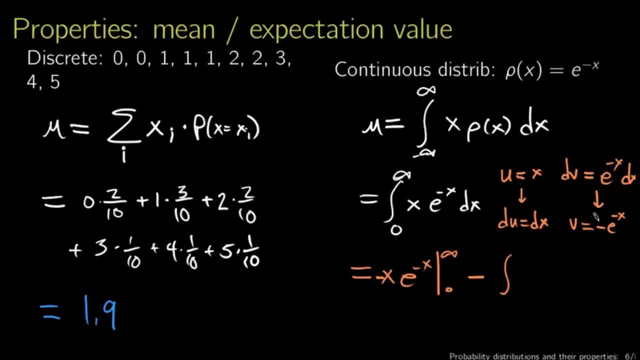 which are these bottom pieces? So the integral now of e to the minus x with a minus sign. so I'm going to change this minus out front into a plus and then this part just dx, from 0 to infinity. Now, what do we do with the endpoints on this? 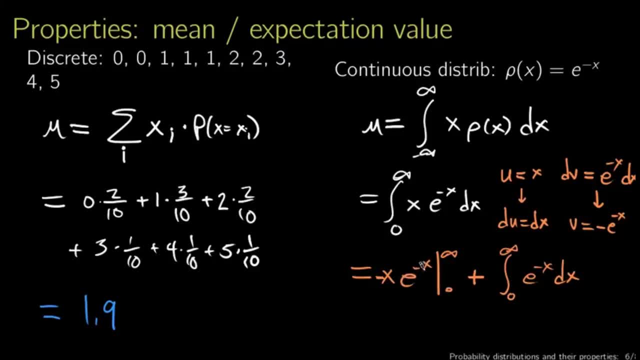 Well, at infinity, e to the minus infinity, that's 1, over e to the infinity, that's 0, and that's a really emphatic 0 if you think about it in the context of a limit, The limit as x, e to the minus x of. 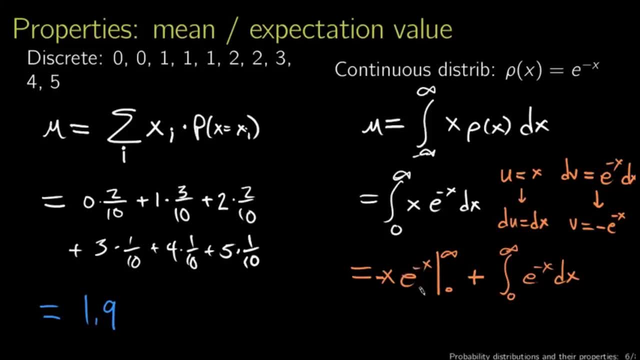 the limit of x, e to the minus x, as x goes to infinity, is 0. So our upper limit here is 0, and then we subtract what we get if we plug in 0 for this. Now, e to the minus 0 is just 1,. 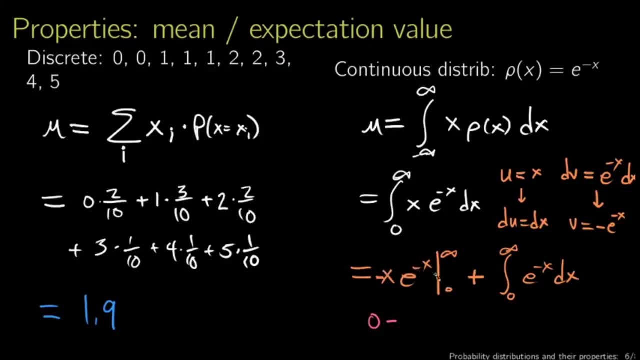 and x. well, x is 0, so we have effectively 0 minus a negative 0,, 0 plus 0,. whatever, it's still 0.. This term vanishes, And what we're left with here is the integral of e to the minus x dx. 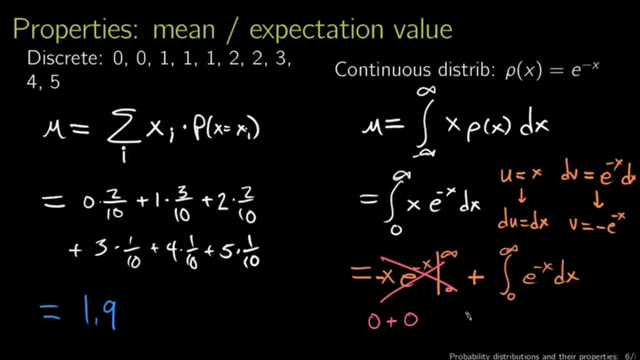 from 0 to infinity, And hopefully you know how to do that- That just in the end is going to equal 1.. So that's our mean Mean is also called expectation value, especially in quantum mechanics. It's not necessarily the value. 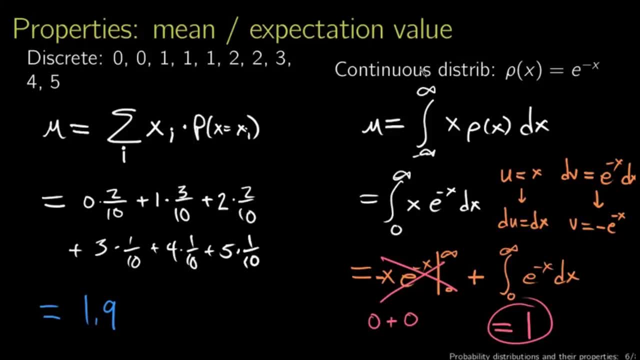 that you expect to get it is the well. it's this mathematical expression that tells you the value that is sort of in the middle of your distribution of possible values. The reason: expectation value is perhaps a better term than mean, especially in quantum mechanics. 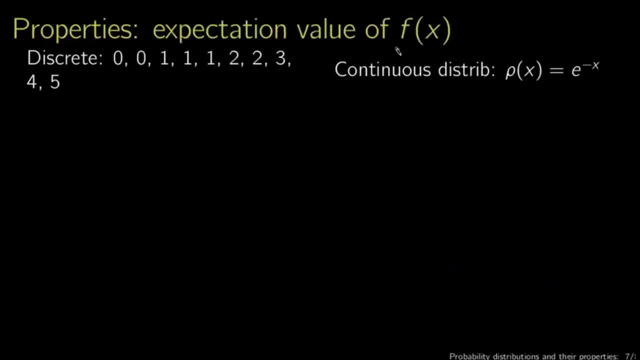 is that we can apply it more easily to functions, For instance f of x. The notation we use for the expectation value or the mean value of some function is to put that in brackets, So this is read as the expected value or the expectation value of x. 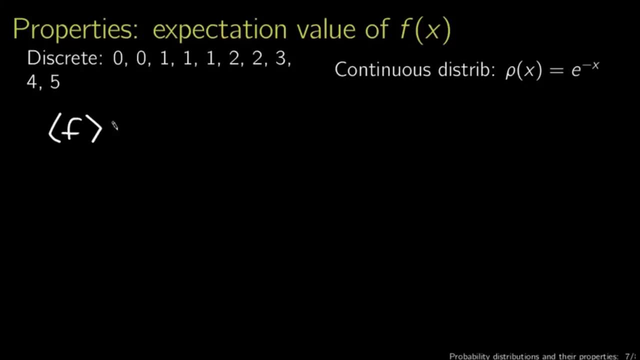 or perhaps just the expectation of f- Excuse me, f, not x- And this, in the context of a discrete probability distribution, looks a lot like the formula for the mean, except instead of x sub i in the sum we have f of x sub i. 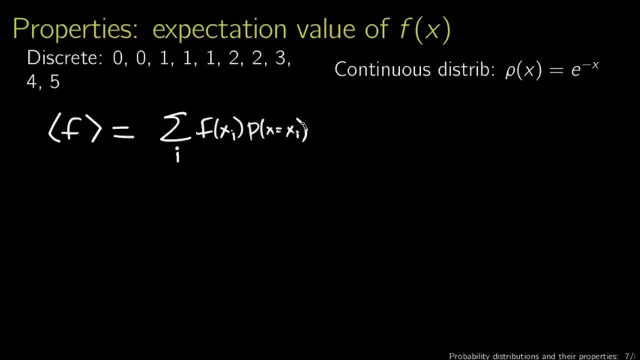 times the probability that x is x sub i. So suppose the function I wanted to work with was f of x equals x squared. What's the probability of x squared? Well, just applying this formula, you would have zero squared from f of x with x sub i. 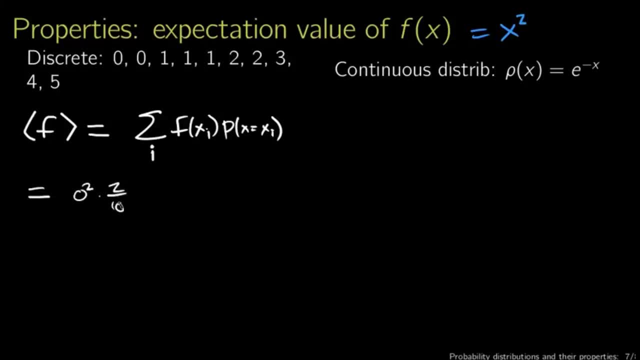 being zero times the probability of zero, which was two tenths plus one squared times three tenths. Now, this is one squared times the probability of one plus two squared times two tenths plus three squared times one tenth plus four squared times one tenth. 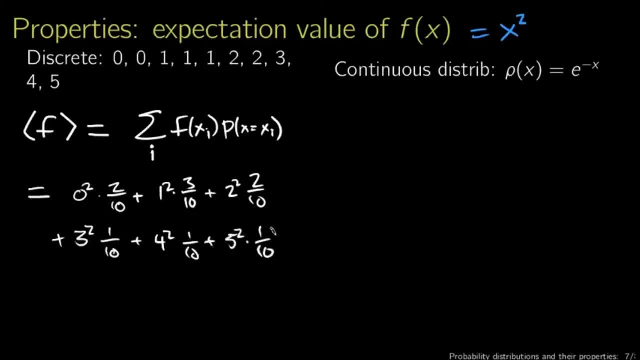 plus five squared times one tenth, And if you plug all the numbers in here, this is a fairly simple thing to do. Hopefully you can get the right answer on your calculator. It comes out to 6.1.. To keep with my format from earlier, 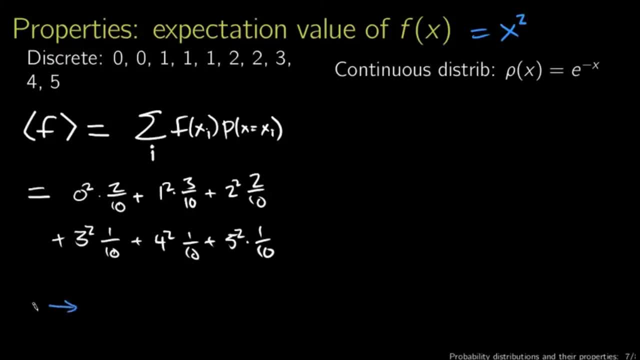 I should do this in color. The expected value of f is 6.1.. You might also see this written as the expected value of x squared, just compacting the notation a little bit and ignoring the definition of x, Ignoring the definition of f. 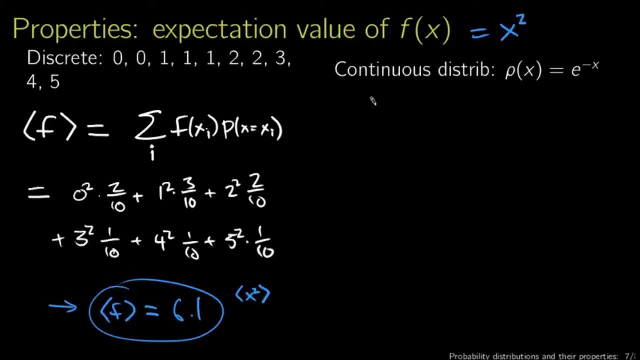 Same thing For the case of a continuous distribution. the pattern by now is hopefully reasonably clear. The expected value of f in the continuous distribution case is equal to the integral, from minus infinity to infinity, of f of x times rho of x dx. 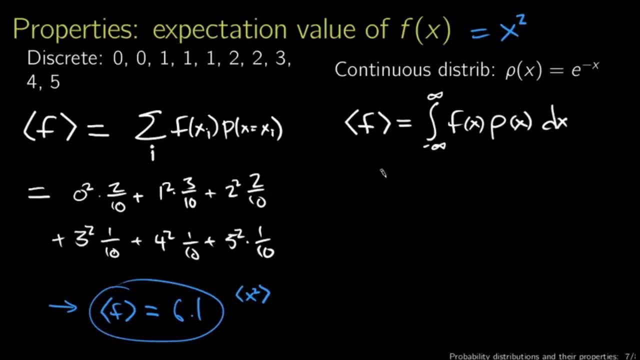 And the integral in this case, for the example function here is going to be equal to integral, from zero to infinity again, because rho of x is zero for x less than zero. f of x is x squared rho of x, e to the minus x. 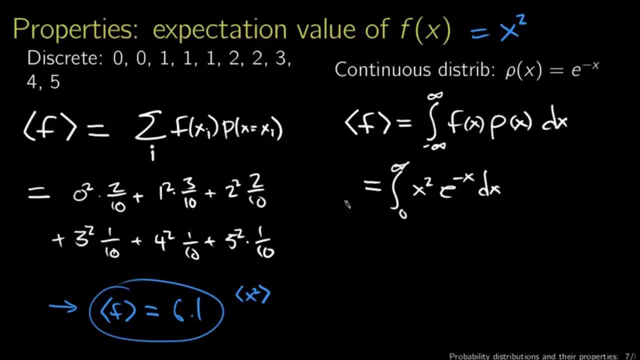 dx. Now again you see an integral like this. I want you to think integration by parts. Alternatively, I want you to think, oh, I should go plug this integral into Wolfram Alpha, or I should go look this up in a table of integrals. 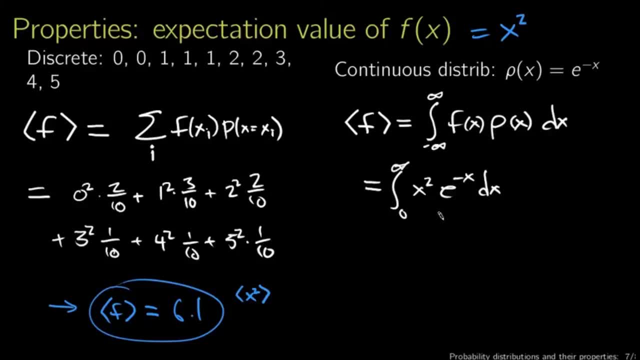 or whatever tool. if you have like a TI-89, or a TI-92,, they can do integrals like this. Whatever technique you want to use to solve integrals is okay with me, But in this case integration by parts will work. 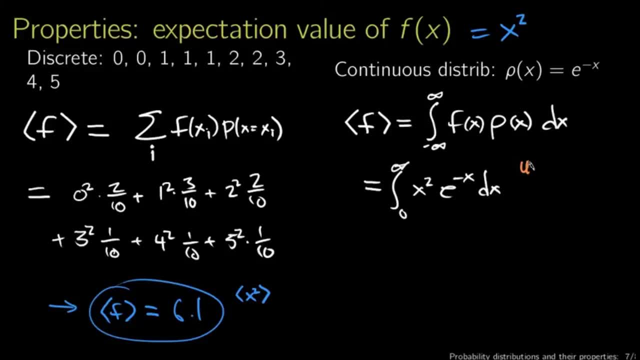 and it's not terribly difficult. So again u is going to be x squared and dv is. here's my eraser: dv equal to e to the minus x dx. Sorry, I'm running out of space there. So 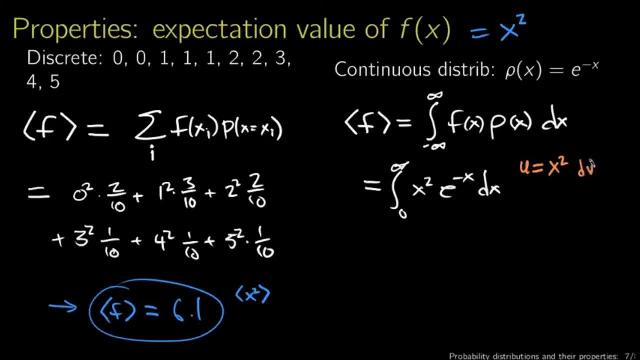 let me do this slightly more legibly: dv equals e to the minus x dx. Now differentiate this: du equals 2x dx and v equals minus e to the minus x In our integration by parts. then the term out front: 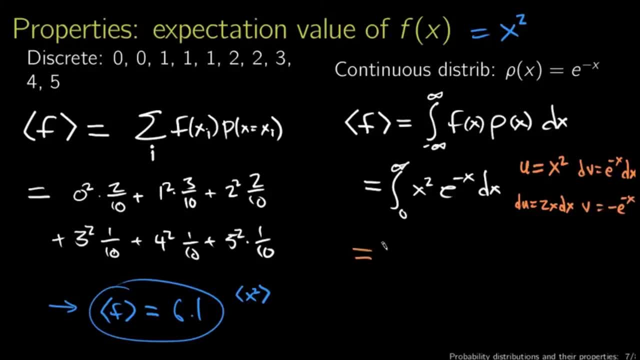 without the integral is going to be x squared times minus e to the minus x evaluated at the limits zero and infinity. And for the same reasons this term vanished In the last case, it's going to vanish here as well. 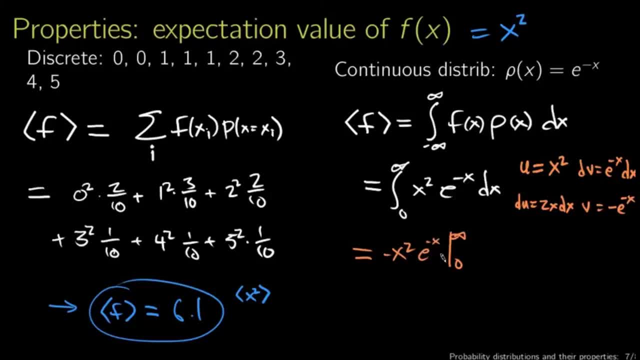 If I evaluate this at infinity, this is going to be zero. If I evaluate this at zero, this is going to be zero, So this term will vanish. The second part of our integration by parts is minus the integral from zero to infinity of. 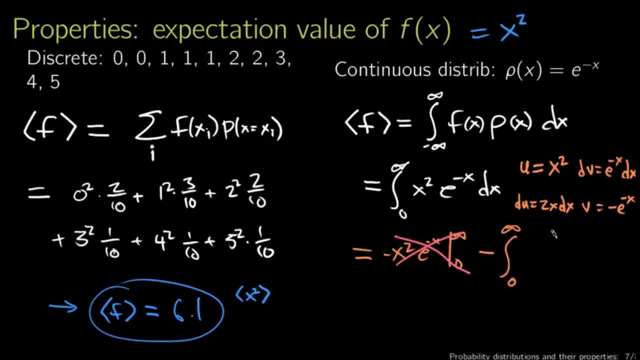 just for the sake of neatness: zero to infinity. The parts here with the differentials in them, 2x, dx, e to the minus x with a minus sign. so I'm going to change this minus sign to a plus sign. 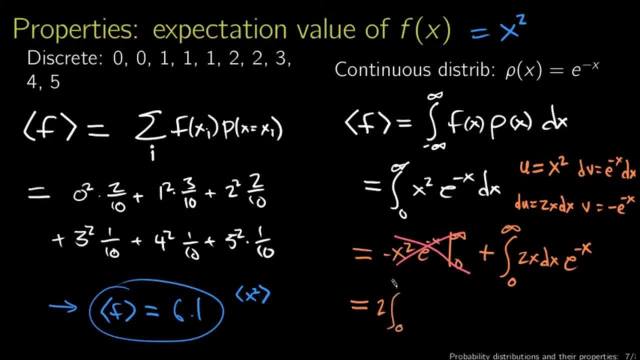 This integral. I'm going to pull the two out front, two times the integral, from zero to infinity, of x e to the minus x dx, And this integral you hopefully remember because we just did it- This integral was equal to one. 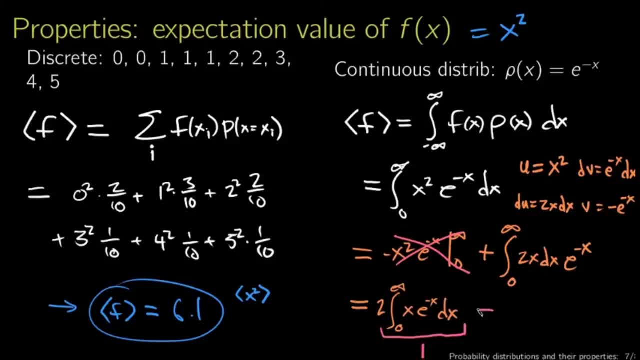 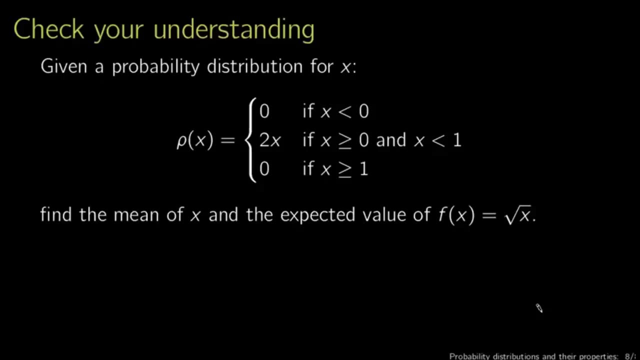 That was what we did on the last page. So this overall is going to equal two. So the expected value of x squared under this continuous probability distribution is two. To check your understanding, here's a sample problem: The probability density function in this case. 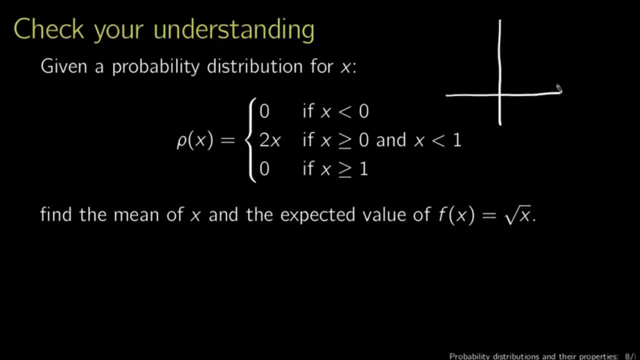 I'll plot it just to make things a little more intuitive. If this is zero and this is one, one and two, the probability density is zero. if x is less than zero, It's also zero if x is greater than one, And for x between zero and one. 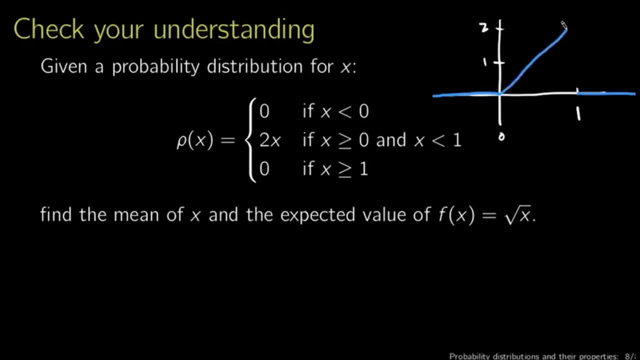 it's equal to 2x. So our probability density function looks something like this, and your task is to find the mean of x under this probability distribution. and the expected value of f of x equals the square root of x. So two tasks here. 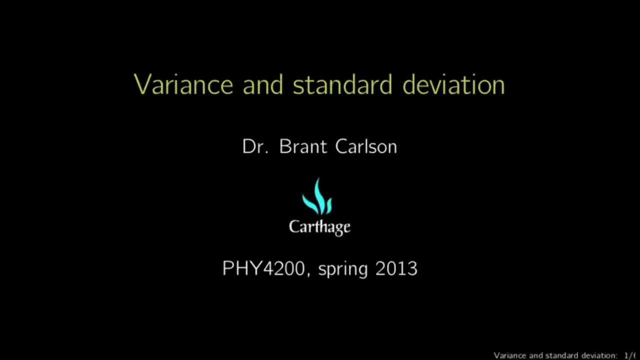 to accomplish with this sample. probability Variance and standard deviation are properties of a probability distribution that are related to the uncertainty. Since uncertainty is such an important concept in quantum mechanics, we need to know how to quantify how uncertainty results from probability distribution. So let's talk about the variance. 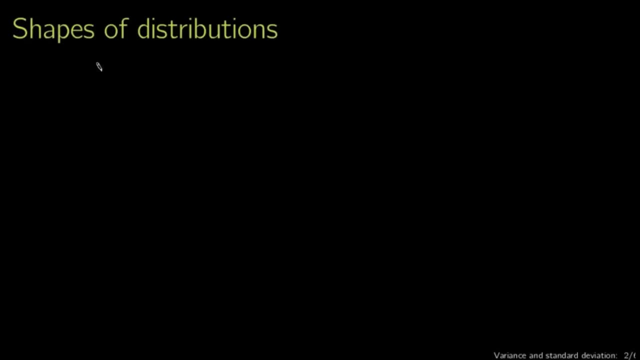 and the standard deviation. These questions are related to the shape. So if I have a set of coordinates- let's say this is the x-axis and I'm going to be plotting- then the probability density function, as a function of x, probability distributions come in lots of shapes and sizes. 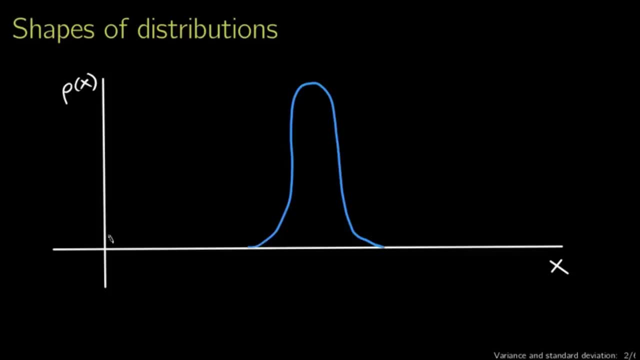 You can have probability distributions that look like this, probability distributions that look like this. You can even have probability distributions that look like this, or probability distributions that look like this, or probability distributions that look like this, And these are all different. The narrow peak here. 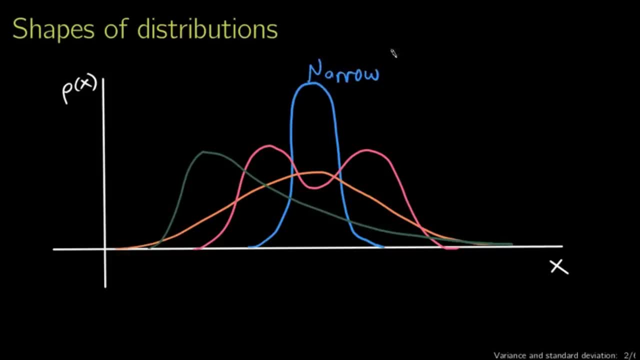 The narrow peak here versus the broad distribution here, versus the broad distribution here versus the broad distribution here, the distribution with multiple peaks or multiple modes. in this case it has two modes, so we call this distribution bimodal or multimodal, And then this distribution. 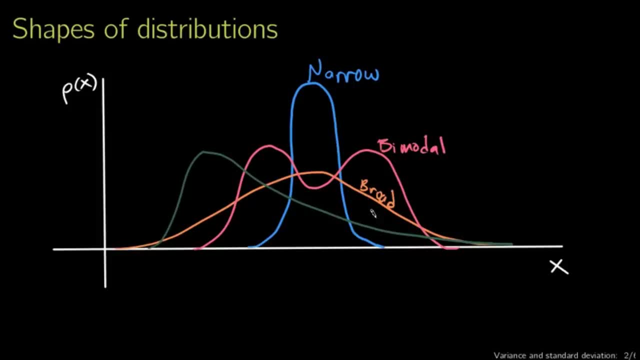 which is asymmetric, has a long tail in the positive direction and a short tail in the negative direction. We would say this distribution is skewed is skewed. So distributions have lots of different shapes, and if what we're interested in is the uncertainty, 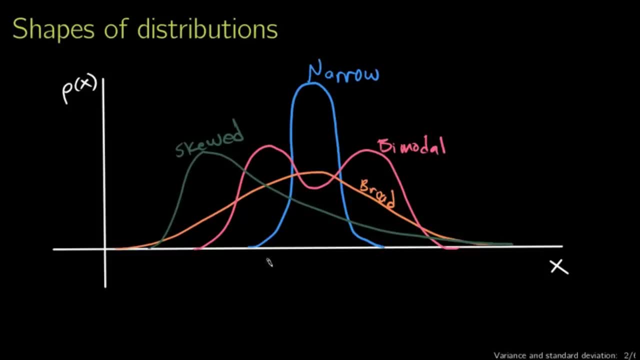 you can think about that roughly as the width of the distribution. you can think about that roughly as the width of the distribution. For instance, if I'm drawing random numbers from the orange distribution, the narrow one here, they'll come over roughly this range. 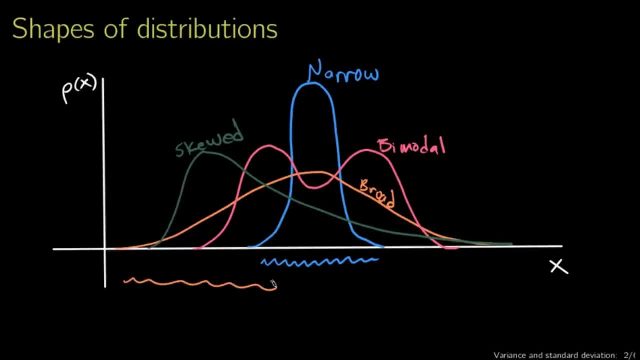 Whereas if I'm drawing from the blue distribution, they'll come over roughly this range. they'll come over roughly this range. So if this were, say probability density for position, say this is the squared magnitude of the wave function for a particle, I know where the particle represented by the 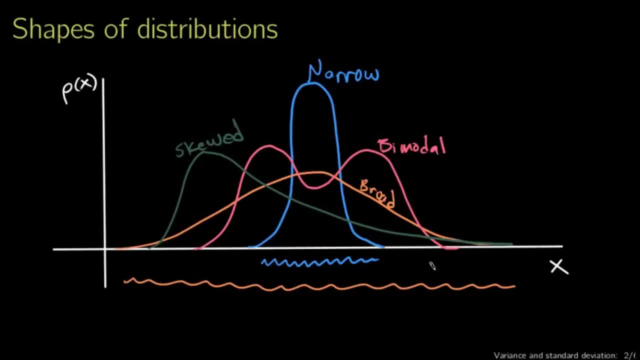 orange distribution is much more accurately than the particle represented by the blue distribution. So this concept of width of a distribution and the uncertainty in the position, for instance, are closely related. The broadness is related to the uncertainty. This is fundamental to quantum mechanics. so how do we quantify it In statistics? 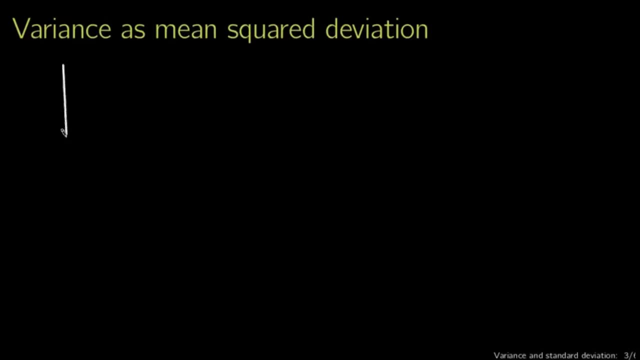 the broadness of a distribution is called the variance. Variance is a way of measuring the broadness of distribution, for example. So suppose this is my distribution. The mean of my distribution is going to fall roughly in the middle here. Let's say that's the expected value of x. if this is the x, 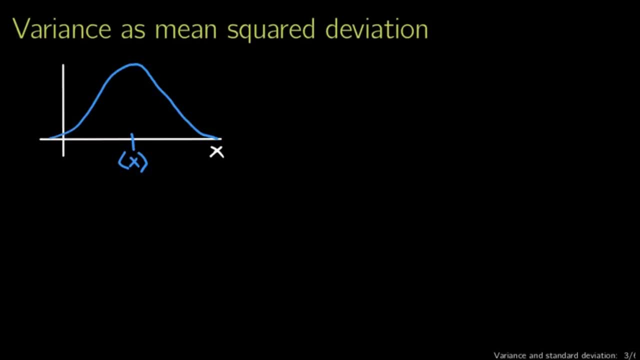 axis. Now, if I draw a random number from this distribution, I won't always get the expected value. Suppose I get a value here. If I'm interested in the typical deviation of this value from the mean, that will tell me something about how broad this distribution is. So let's define this displacement here to be. 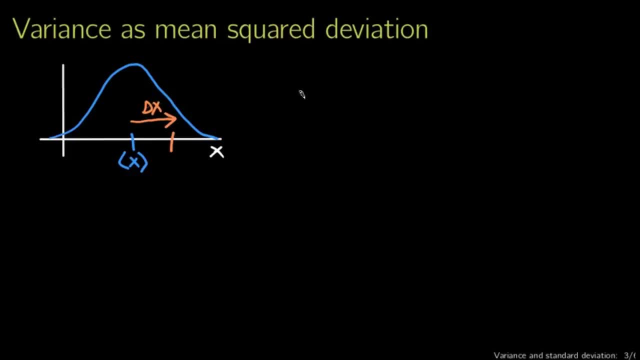 delta x. Delta x is going to be equal to x minus the expected value of x. And first of all, you might think: well, if I'm looking for the typical values of delta x, let's just try the expected value of delta x. Well, what is that? Unfortunately, the expected. 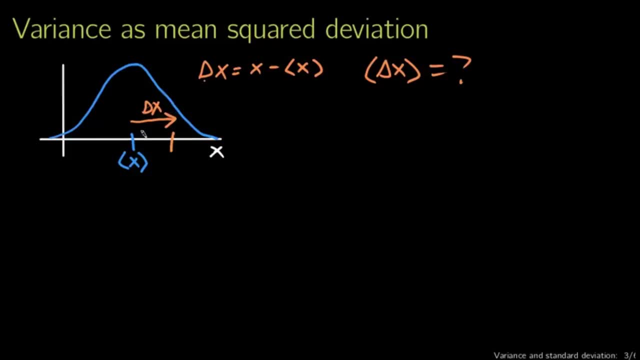 value of x doesn't really work for this purpose, because delta x is positive if you're on this side of the mean and negative if you're on this side of the mean. So the expected value of delta x is zero. Sometimes it's positive, sometimes it's negative, and they end up. 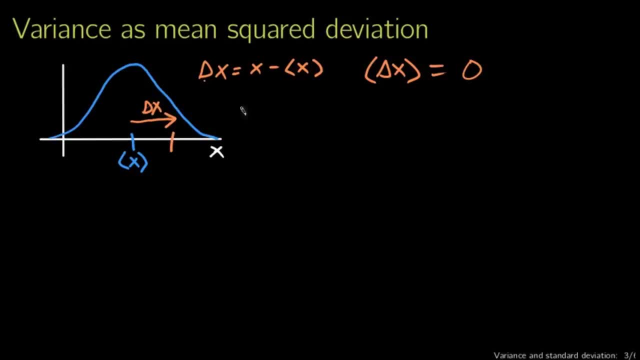 canceling out. Now, if you're interested in only positive numbers, the next guess you might come up with is: let's use not delta x, but let's use the absolute value of delta x. What is that? Well, absolute values are difficult to work with, since 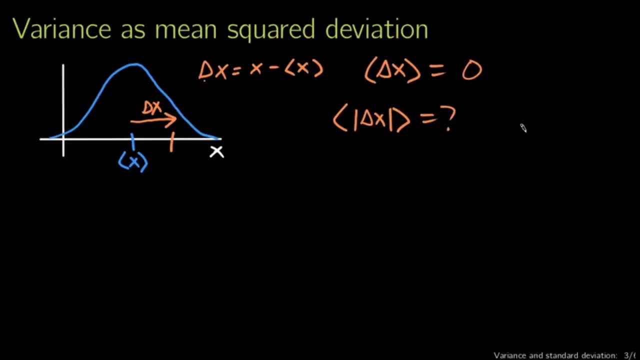 you have to keep track of whether a number is positive or negative and keep flipping signs if it's negative. So this turns out to just be kind of painful. What statisticians and physicists do in the end, then, is, instead of taking the absolute value of a number just to make it positive, we square it, So you. 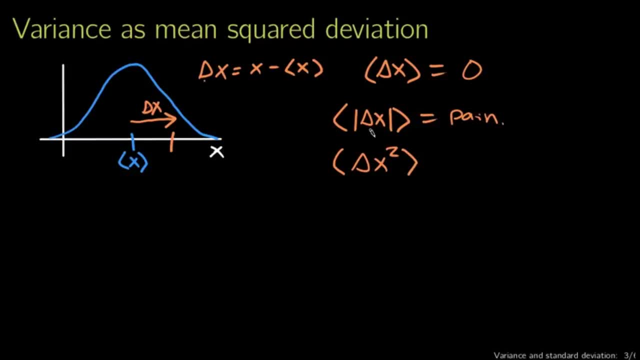 calculate the expected value of the squared deviation, sort of the mean squared deviation. This has a name in statistics. it's written as sigma squared and it's called the variance. To do an example, let's do a discrete example. Suppose I have two probability distributions, all with equally likely. 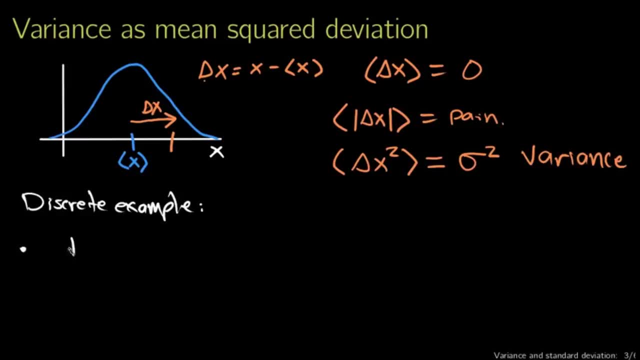 outcomes. Say, the outcomes of one distribution are 1,, 2, and 3, while the outcomes for the second distribution are 0,, 2, and 4.. Put it graphically, these numbers are more closely spaced than these numbers, So I would expect the 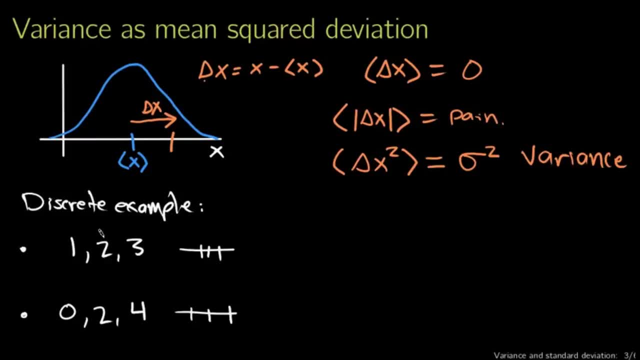 broadness of this distribution to be near the mean squared deviation and that's to be larger than the broadness of this distribution. You can calculate this out by calculating the mean squared deviation. So first of all we need to know the mean. the expected value of x is 2 in this case and also in this case. 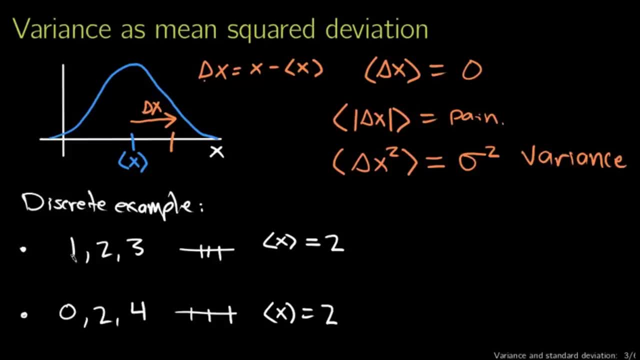 knowing the expected value of x, you can calculate the deviations. So let's say delta x here is going to be minus 1, 0, and 1 are the possible deviations from the mean for this probability distribution, whereas in this case it's. 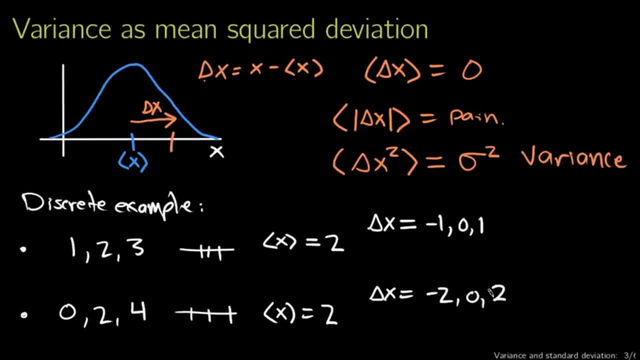 minus 2, 0, and 2.. Then we can calculate the delta x squareds that are possible and you get 1, 0, and 1 for this distribution and 4, 0, and 4 for this. 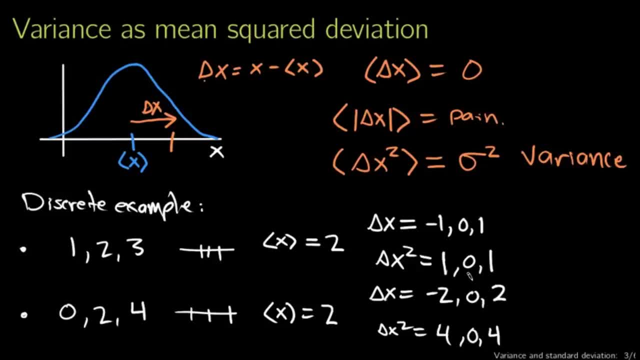 distribution. Now, when you calculate the mean of these squared deviations, in this case the expected value of the squared deviation is 2 thirds, whereas in this case the expected value of the squared deviation is 8 thirds. So indeed we did get a larger number for the variance in. 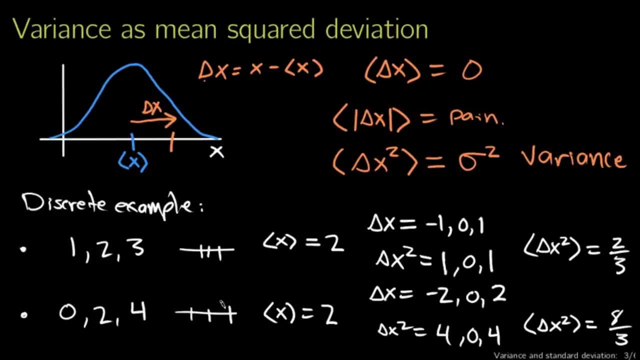 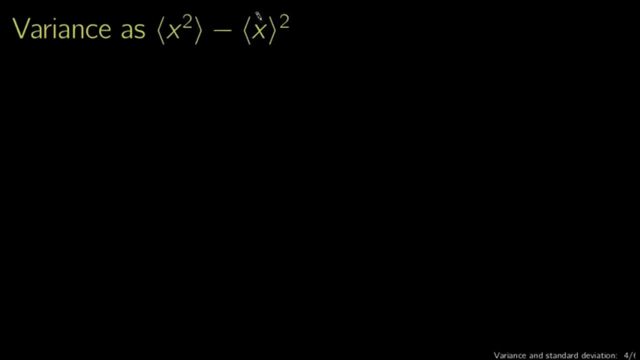 this distribution, So you can think of that as the definition. This is not the easiest way of calculating the variance, though It's actually much easier to calculate the variance as an expected value of a squared quantity and minus the square of the expected value of. 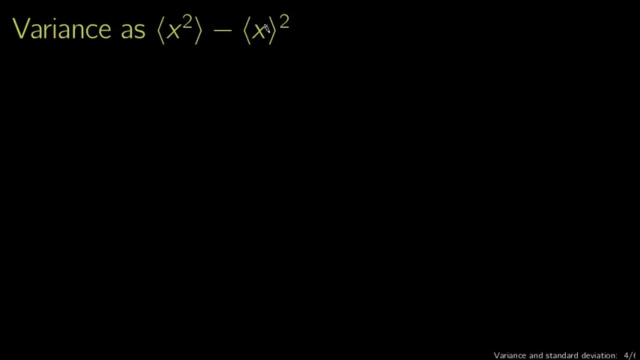 the quantity itself, so the mean of the square minus the square of the mean. If that helps you to remember it, You can see how this results fairly easily by plugging through some basic algebra. So, given our definition, the expected value of x squared, we're calculating an expected value. So suppose we have a continuous. 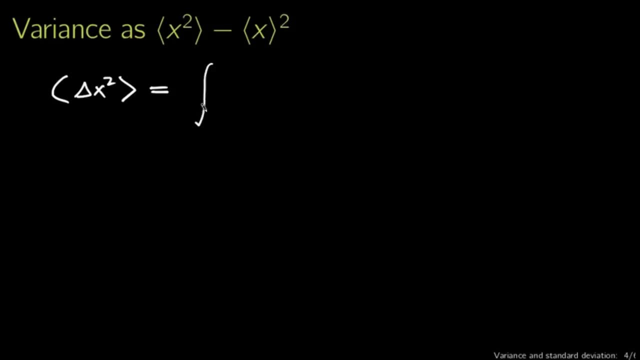 distribution. now The continuous distribution expected value has an integral in it. so we're going to have the integral of delta x squared times rho of x, dx, Now delta x squared. we know what delta x is. Delta x is x minus the expected value of x, so we can plug that in here and we're going to get the. 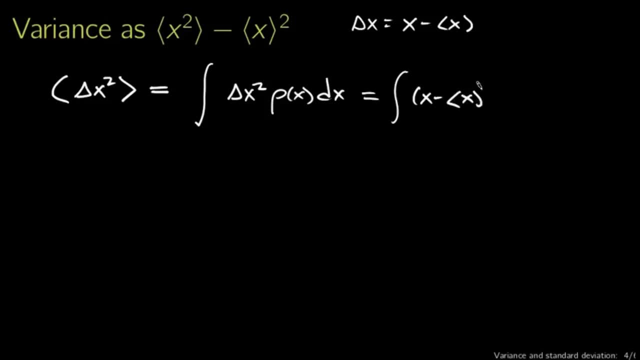 integral of x minus expected value of x, squared times rho of x- dx. I can expand this out and I'll get integral of x squared minus 2x expected value of x plus expected value of x, quantity squared rho of x- dx. Now I'm going to split this integral up into three separate pieces. First piece: 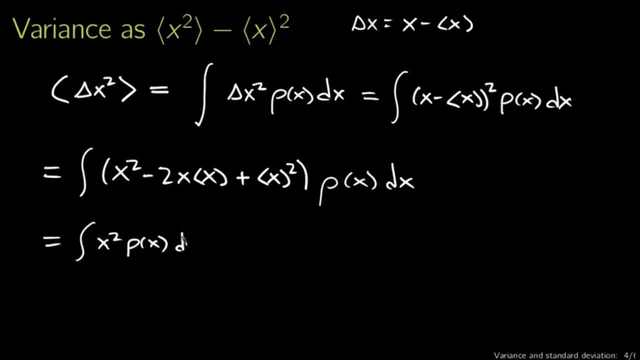 integral of x squared rho of x dx. Second piece: integral of 2x expected value of x rho of x dx. And the third piece: integral of expected value of x squared rho of x dx. Now this integral. 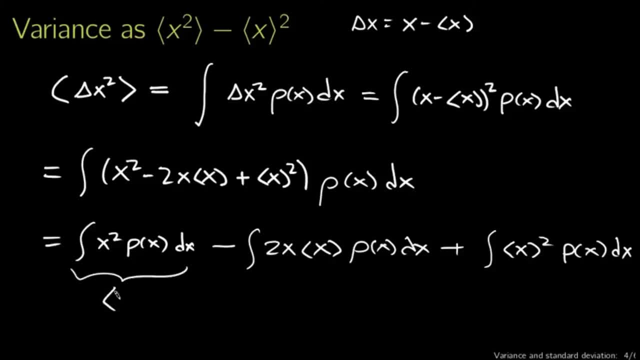 you recognize right away, this is the expected value of x squared, This integral. I can pull this out front, since this is a constant, this is just a number. this is the expected value. So this integral is going to become 2, I can pull the 2 out, of course, as well. 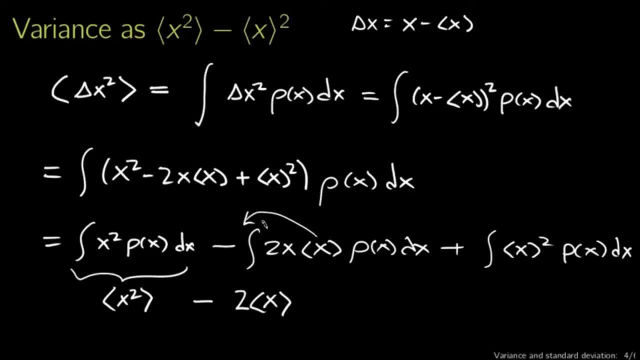 2 times the expected value of x, and then what's left is the integral of x, rho of x, dx, which is just the expected value of x. This integral again, this is a constant, so I can pull it out front, and when I do that I end up with just the integral of rho of x, dx. 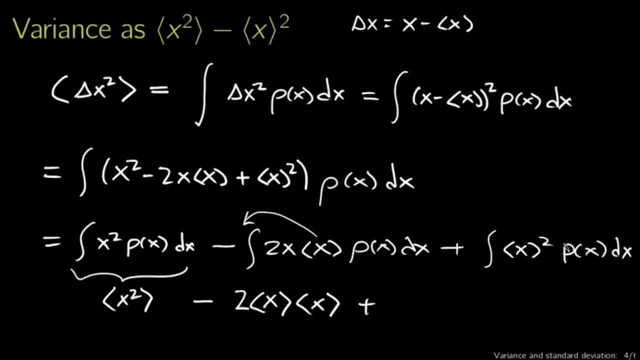 And we know the integral of rho of x dx over the entire domain. I should specify that this is the integral from minus infinity to infinity. now, All of these are integrals from minus infinity to infinity. The integral of minus infinity to infinity of rho of x dx is 1.. 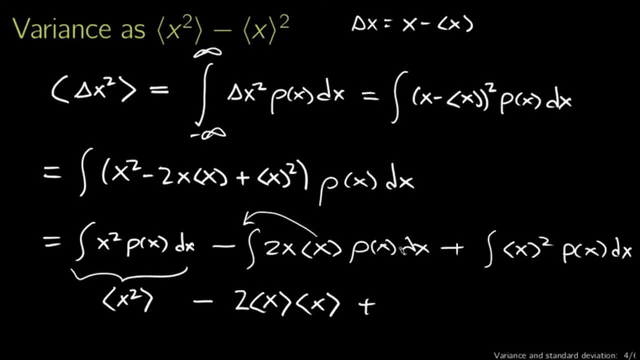 So this, after I pull the expected value of x quantity squared out, is just going to be the expected value of x quantity squared. So this is expected value of x squared. This is well. I can simplify this as well. this is the expected value of x quantity squared as well. 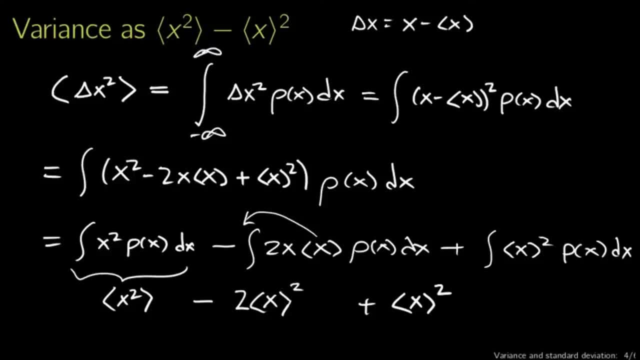 so I'm going to erase that and say squared there. So I have this minus twice this plus this And in the end that gives you expected value of x squared minus the expected value of x squared. So mean of the square minus the square of the mean. 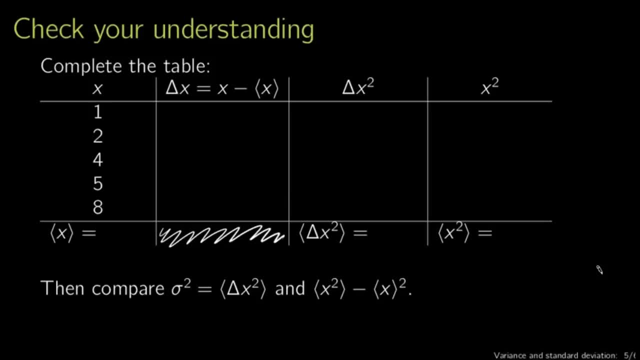 To check your understanding of how to use this formula, I'd like you to complete the following table Now. I'll give you a head start on this. If your probability distribution is given by 1,, 2,, 4,, 5, and 8,, 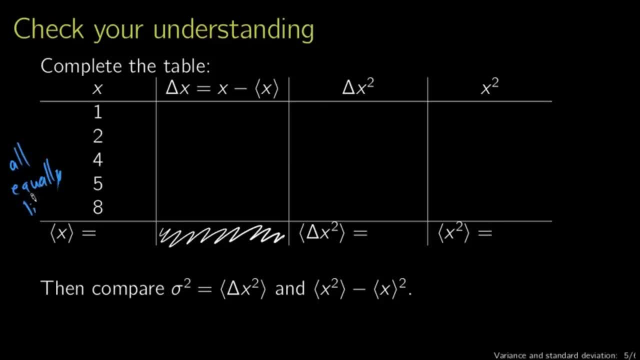 all equally likely. you can calculate the mean. Now, once you know the mean, you can calculate the deviations x minus the mean, which I'd like you to fill in here. Then square that quantity and fill it in here and take the mean of that squared deviation. 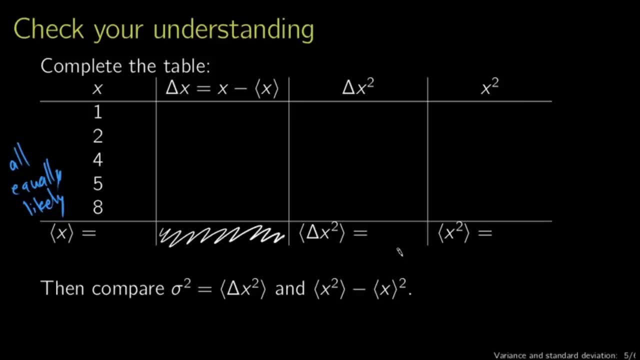 Same as what we did when we talked about the variance as the mean squared deviation. Then, taking the other approach, I'd like you to calculate the the squares of all of the x's and calculate the mean squared. You know the mean, you know the mean squared. 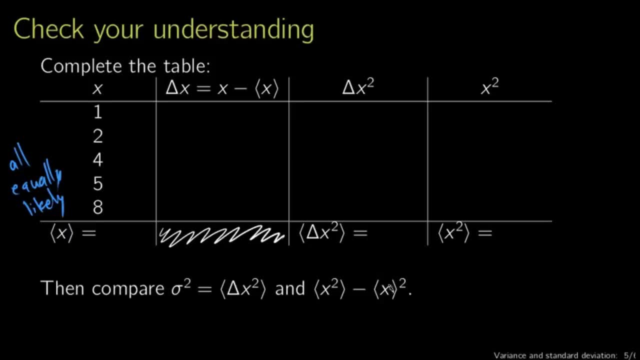 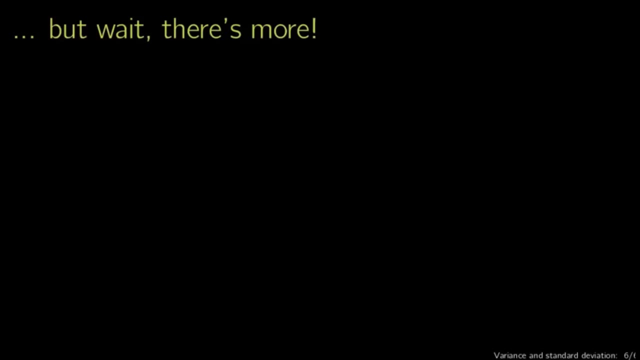 You can calculate this quantity Mean of the square minus the square of the mean, And you should get something that equals the mean squared deviation. That's about it for variance. But just to say a little bit more about this, Variance is not the end of the story. 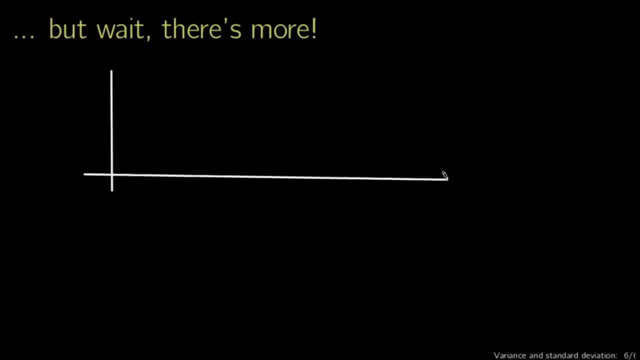 It turns out there's well, there's more. I mentioned the distributions that we were talking about earlier on the on the first slide. here I keep forgetting to turn my ruler off: The distributions that look like this versus distributions that look like this. 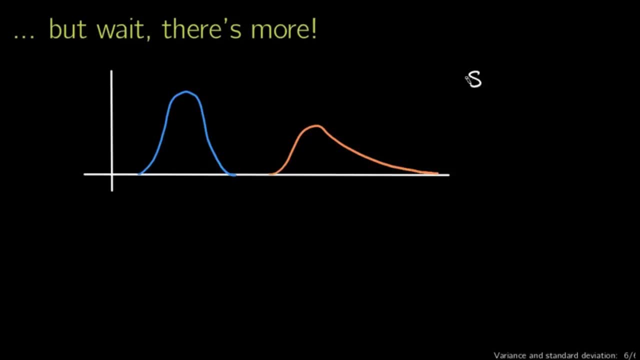 This is a question of symmetry, and the mathematical name for this is skew or skewness. There's also distributions that look like this Versus distributions that look like this, And this is what they're. mathematically, This is called kurtosis. 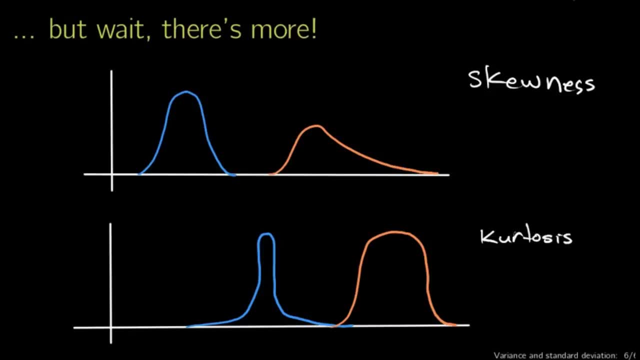 which kind of sounds like a disease or perhaps a villain from a comic book. Kurtosis has to do with the relative weights of things near the peak versus things in the tails. Now, mathematically speaking, you know the variance. sorry. 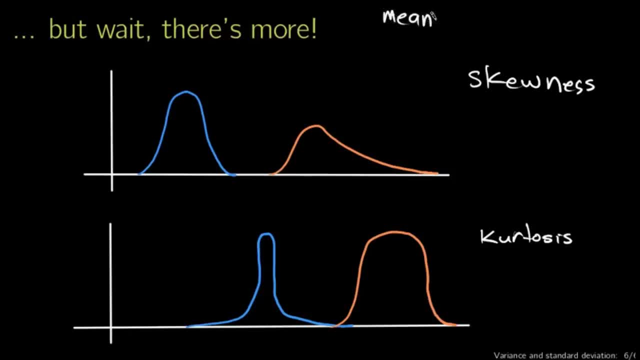 Let me go back a little further. You know the mean That was related to the integral of x- row of x dx. We also just learned about the variance Which was related to the integral of x squared Row of x dx. 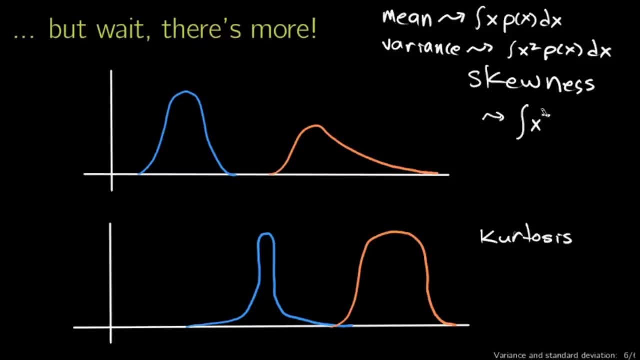 It turns out, the skewness is related to the integral of x cubed row of x- dx And the kurtosis is related to the integral of x to the fourth row of x- dx. At least those are common ways of measuring skewness and kurtosis. 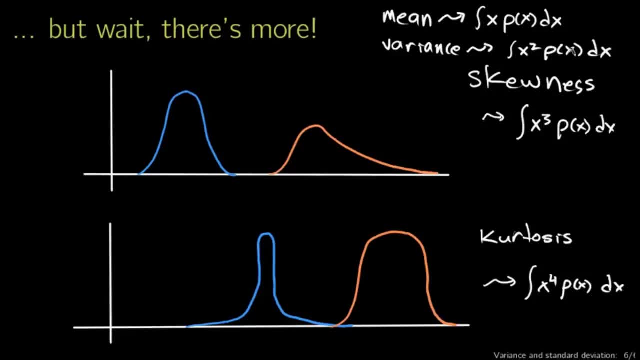 These are not exact formulas for skewness and kurtosis, nor is this an exact formula for the variance of course. So I'm taking some liberties with the math. But you can imagine well what happens if you take the integral of x to the fourth. 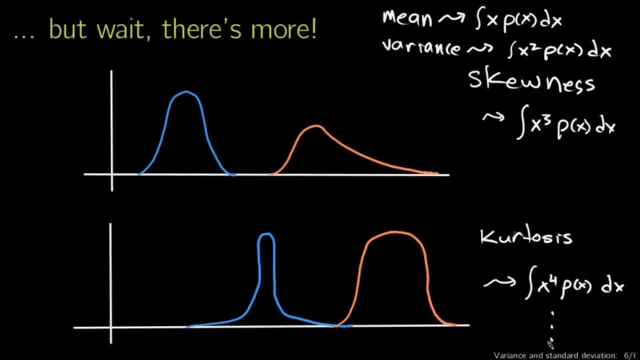 and you take the integral of x to the fifth, and you take the integral of x to the sixth, and you take the integral of x to the fifth row of x dx. You could keep going and you would keep getting properties of the probability distribution. 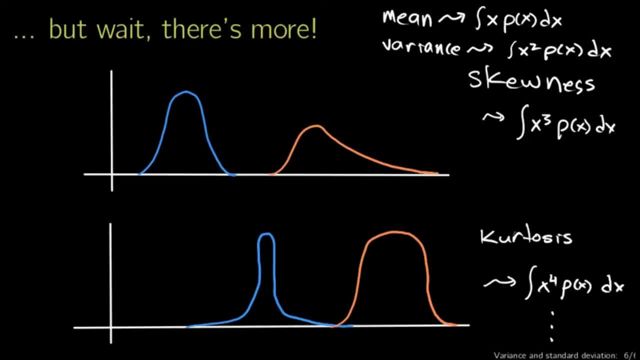 that are relevant to its shape. Now you won't hear very much about skewness and kurtosis in physics, but I thought you should know that this field does sort of continue on For the purposes of quantum mechanics. what you need to know is that variance is related to the uncertainty. 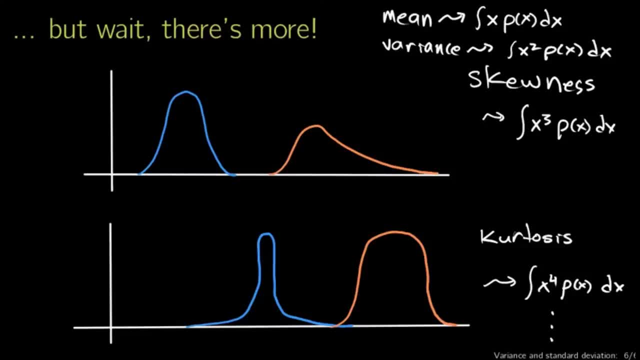 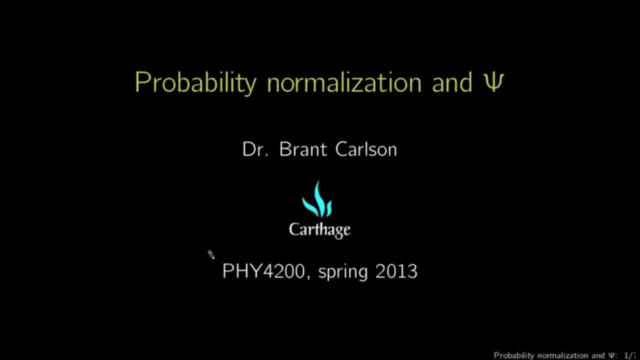 and we will be doing lots of calculations of variance on the basis of probability distributions derived from wave functions in this class. We talked a little bit about the probabilistic interpretation of the wave function, psi. That's one of the really remarkable aspects of quantum mechanics. 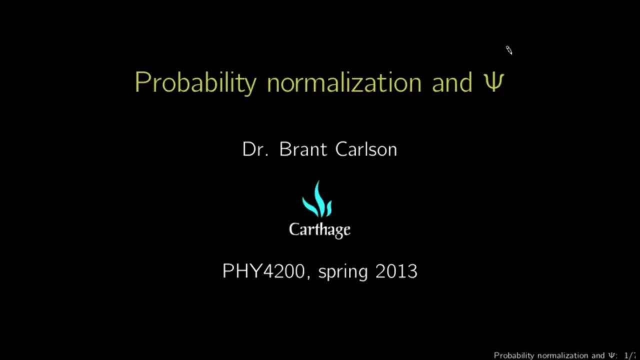 that there are probabilities rolled up in your description of the physical state. We also talked a fair amount about probability itself, and one of the things we learned was that probabilities had to be normalized, meaning the total sum of all of the probable outcomes, the probabilities of all of the outcomes in a probability distribution has to equal one. 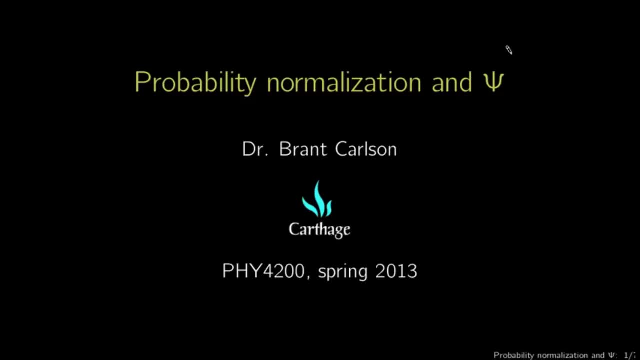 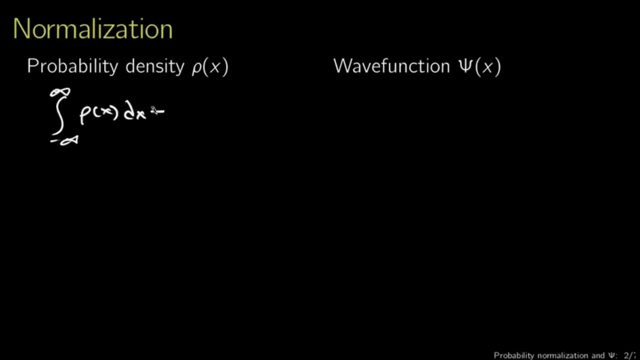 That has some implications for the wave function, especially in the context of the Schrodinger equation. So let's talk about that in a little more detail. Normalization in the context of a probability distribution just means that the integral from minus infinity to infinity of rho, of x, dx, is equal to 1.. 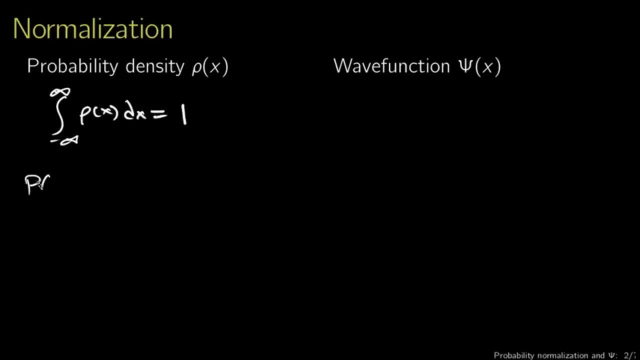 You can think about that as the sort of extreme case of the probability that say x is between a and b being given by the integral from a to b of rho, of x, dx. In the context of the wave function, that statement becomes the probability that the 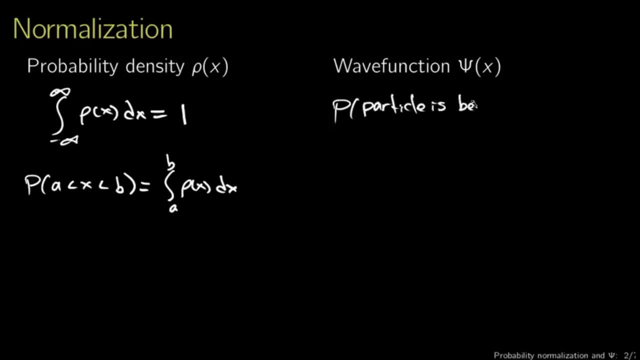 particle is between a and b is given by the integral from a to b of the squared magnitude of psi of x integrated between a and b. So this is the same sort of statement, but you're integrating from a to b and in the case of the probability, density. 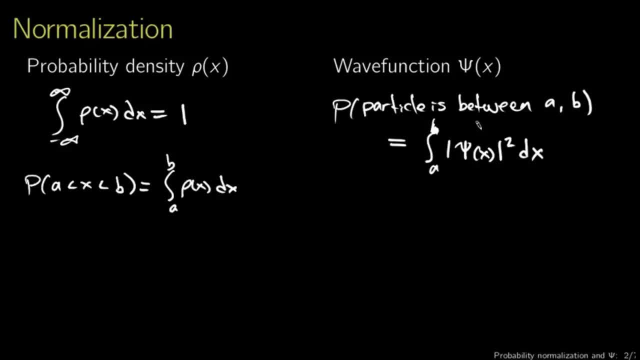 you have just the probability density. In the case of the wave function, you have the squared absolute magnitude of the wave function. This is our probabilistic interpretation. We're sort of making an analogy between psi- the squared magnitude- and a probability density. 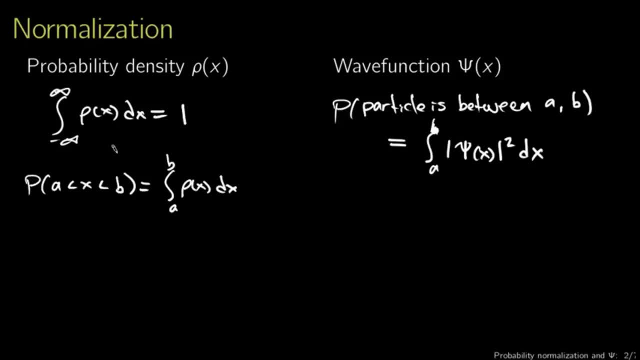 This normalization condition then has to also hold for psi. if the squared magnitude of psi is going to be treated as a probability density, So integral from minus infinity to infinity of squared absolute magnitude of psi, dx has to equal 1.. This is necessary for our statistical interpretation of the wave function. 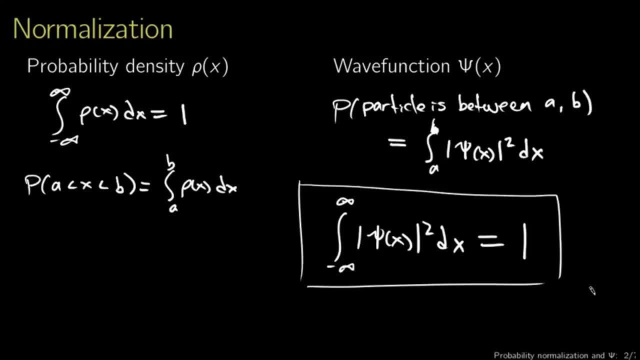 This brings up an interesting question, though, because not just any function can be a probability distribution. Therefore, this normalization condition- treating psi as a probability density- has to be treated as a probability density. This means there are some conditions on what sorts of functions are allowed to be wave functions. 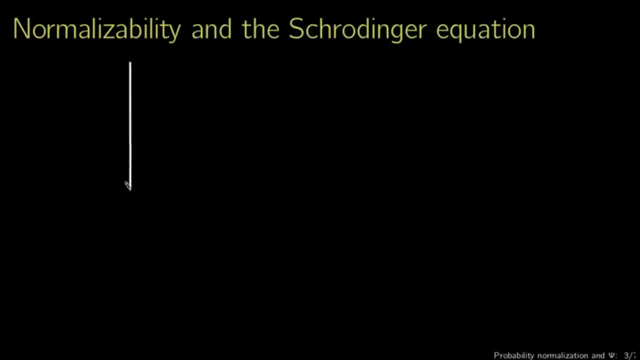 This is a question of normalizability. Suppose, for instance, I had a couple of functions that I was interested in. Say, one of those functions looks sort of like this and keeps on rising as it goes to infinity. If I wanted to consider the squared magnitude of this function, 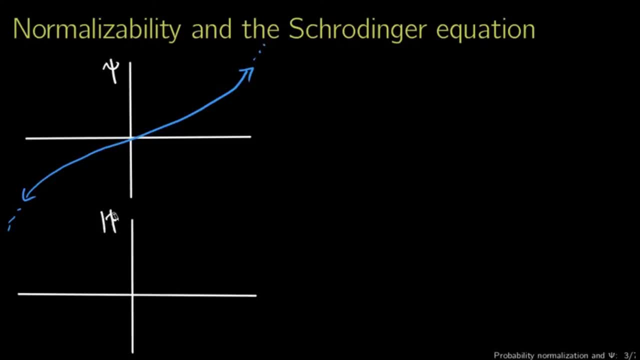 this is our possible psi, this is our possible psi-squared. sorry about the messy there. This function, since it's going to, you know, it's continuing to increase as x increases, both in the negative direction and in the positive direction, its squared magnitude. 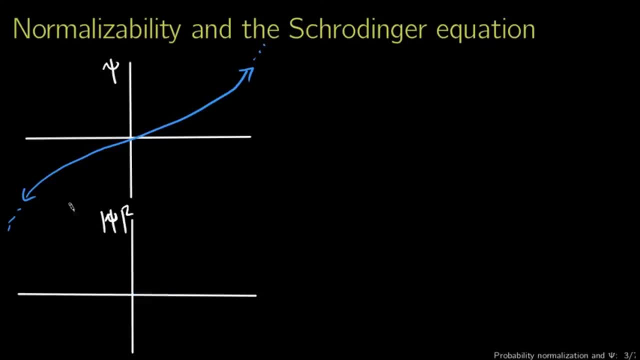 is going to look something like this. I can do a little better there. sorry, If I tried to say calculate the squared magnitude of this function, if I tried to say calculate the integral from minus infinity to infinity of this function. 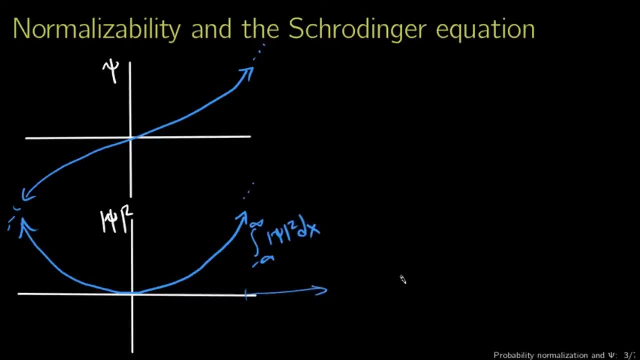 I've got a lot of area out here, from, say, 3 to infinity, where the wave function is positive. This would go to infinity. therefore, What that means is that this function is not normalizable. Not all functions can be normalized. 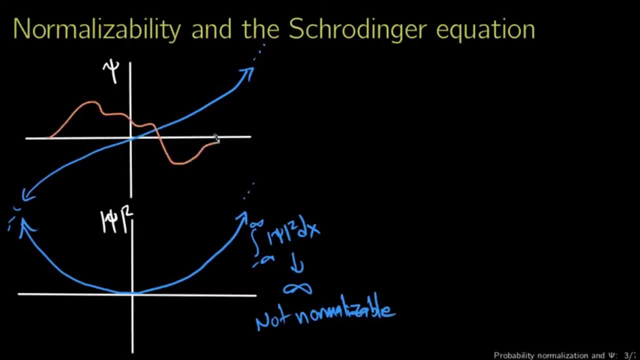 If I drew a different function, for example something that looked maybe something like this: its squared magnitude might look something like this: There is a finite amount of area here, so if I integrated the squared magnitude of the blue curve, I would get something finite. 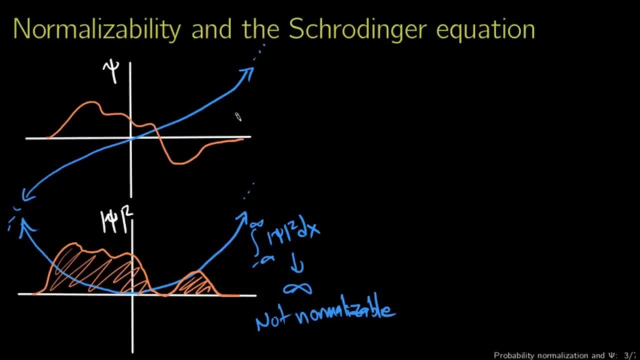 What that means is that, whatever this function is, I could de-multiply over it, I could de-multiply over it, I could de-multiply over it or divide it by a constant such that this area was equal to 1.. I could take this function and convert it into something such that: 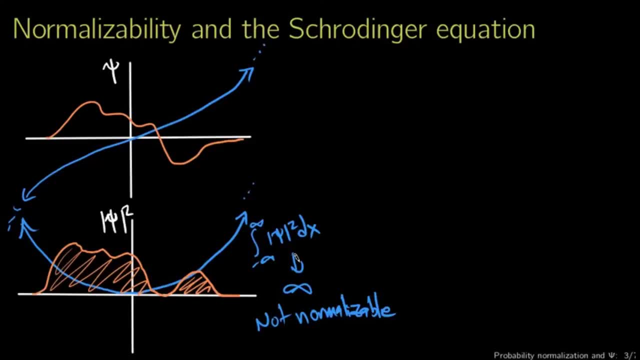 the integral, from minus infinity to infinity, of the squared magnitude of psi equaled 1, and it obeyed our sort of statistical constraint on the probability distribution. In order for this to be possible, psi has to have this property, and the mathematical way of stating it is that psi must be. 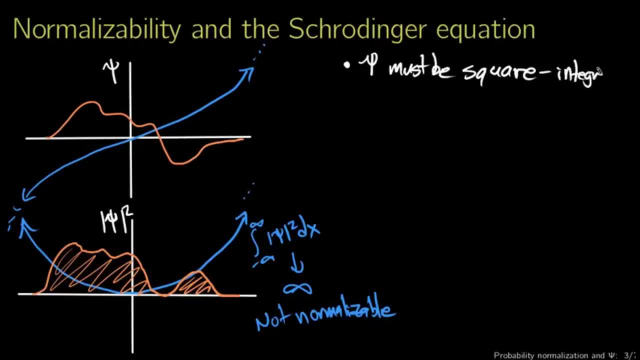 square integrable, And all this means is that the integral, from minus infinity to infinity, of the squared magnitude of psi is finite. You don't get 0, you don't get infinity. In order for this square integrability to hold, for example, though, 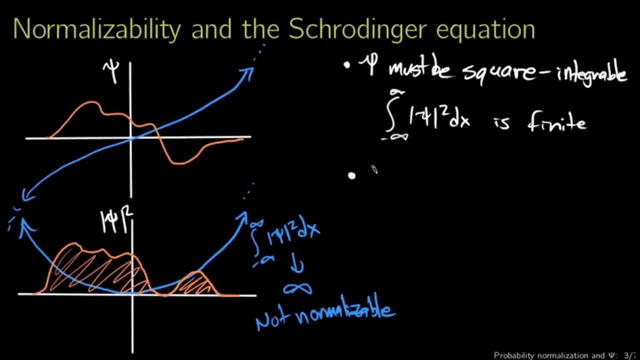 you need a slightly weaker condition: that psi goes to 0 as x goes to either plus or minus infinity. It's not possible to have a function that stays non-zero or goes to infinity itself as x goes to infinity, and still have things be integrable. 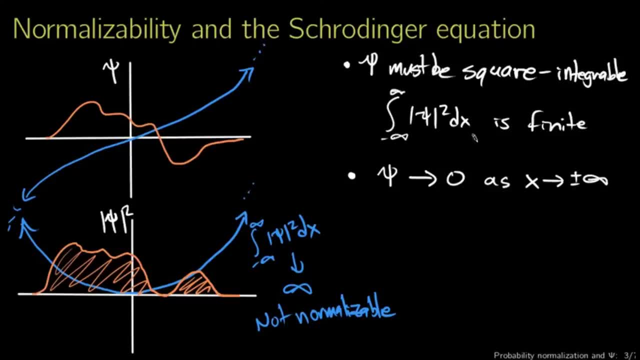 Like I said, if this holds, if this integral here is finite, you can convert any function into something that is normalized by just multiplying or dividing by a constant. Is that possible, though? In the Schrodinger equation? does multiplying or dividing 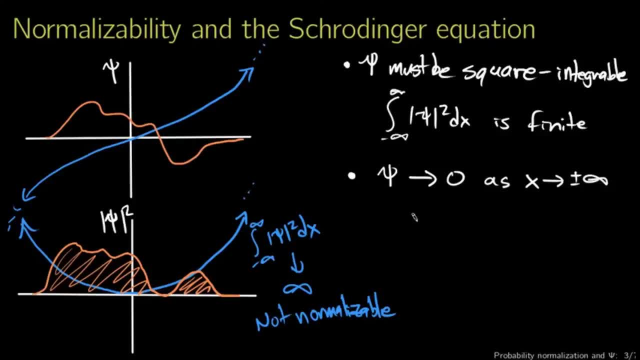 by a constant do anything. Well, the Schrodinger equation here. you can just glance at it and see that multiplying and dividing by a constant doesn't do anything. The Schrodinger equation is: i h-bar partial derivative with respect to time of psi equals minus h-bar squared over 2m. 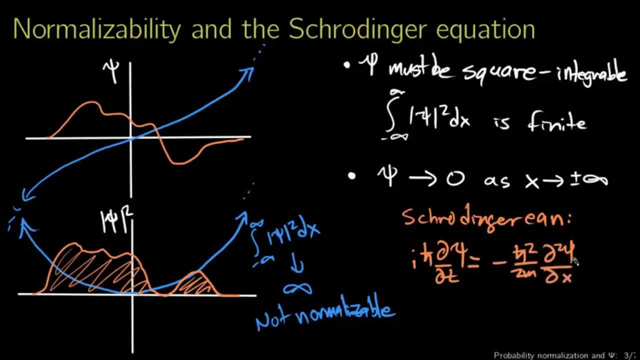 second derivative of psi with respect to position plus the potential times psi. Now if I made the substitution psi went to some multiple or some constant a multiplied by psi, you can see what would happen Here. I would have psi times a. 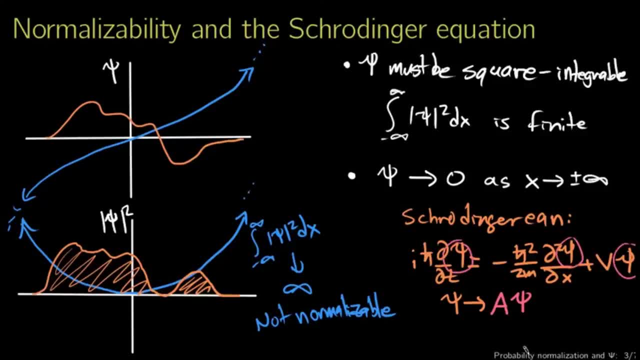 And here I would have psi times a, So I would have an a here, an a here and an a here, So I could divide through this entire equation by a and all of those a's would disappear and I would just get the original Schrodinger equation back. 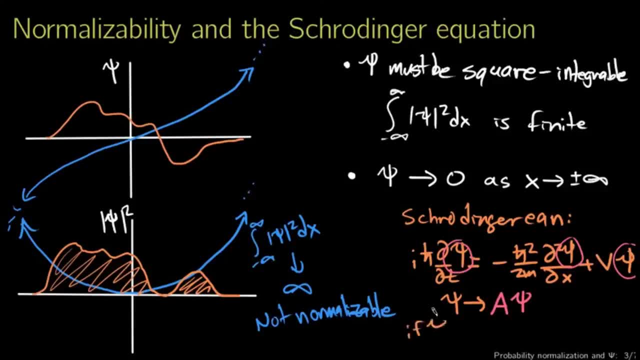 What that means is that if psi solves the Schrodinger equation, a psi does too. And I'll just say: a psi works. Now, this is only if a is a constant, Does not depend on time, does not depend on space. 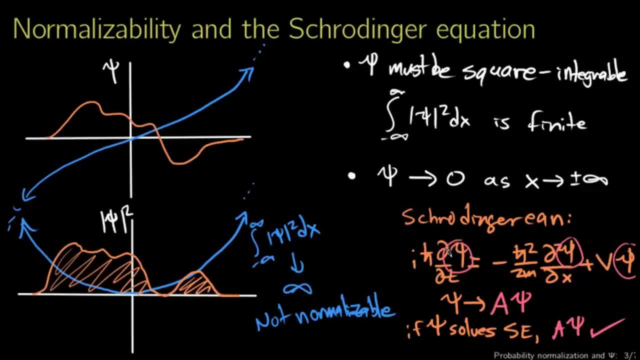 If a depended on time, I would not be able to divide it out of this partial derivative, because the partial derivative would act on that a Same goes for if a was a function of space. If a was a function of space, I wouldn't be able to divide it out. 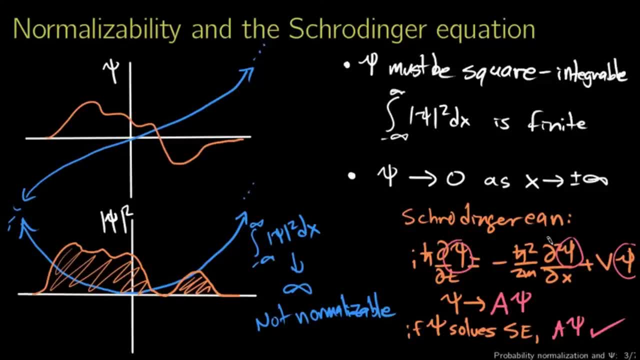 of this partial derivative with respect to x. So this only holds if a is a constant. That means that I might run into some problems with time evolution. I can choose a constant and I can multiply psi by that constant such that psi is properly normalized. at say time t equals 0,. 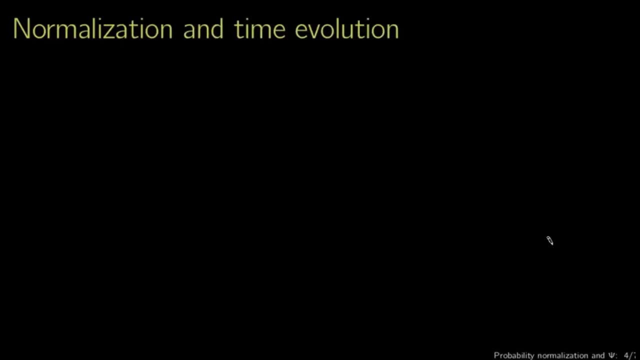 but will that hold for future times? It's a question of normalization and time evolution. What we're really interested in here is the integral from minus infinity to infinity of psi, of x and time squared dx, If this is going to always be equal to 1,. 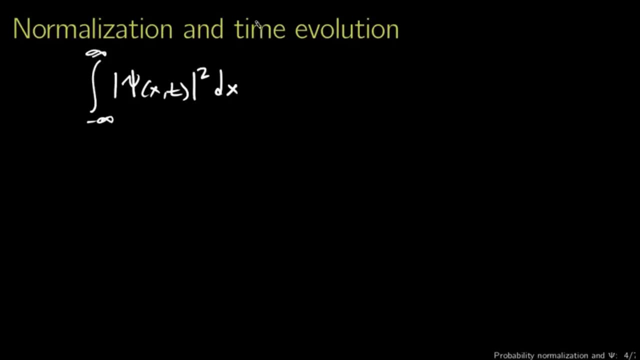 supposing it's equal to 1 at some initial time. what we really want to know is what the time derivative of this is. If the time derivative of this is equal to 0, then we'll know that, whatever the normalization of this is. 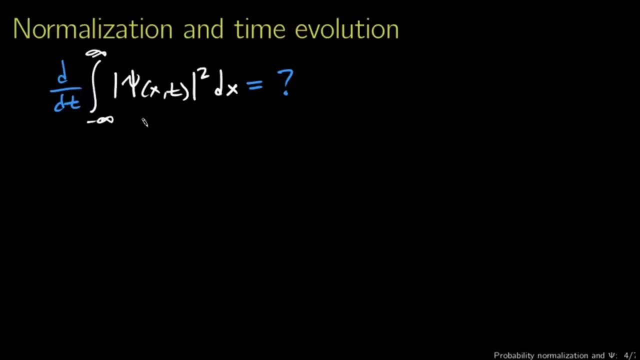 it will hold throughout the evolution of the- well, throughout the evolution of this, along with the wave function. Now I'm going to make a little bit of simplifying notation here and I'm going to drop the integral limits, since it takes a while to write. 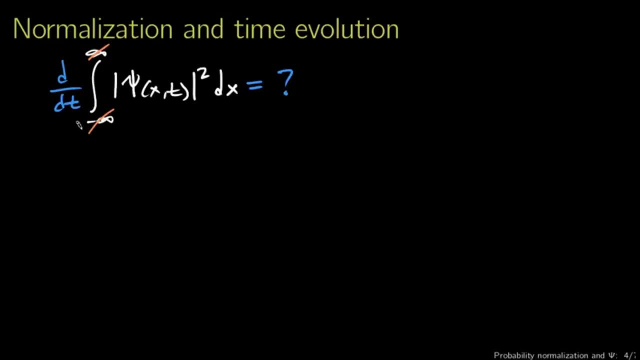 And we're going to manipulate this expression a little bit. We're going to use the Schrodinger equation, we're going to use the rules of complex numbers, we're going to use the rules of differential calculus and we're going to get something that will show that indeed, 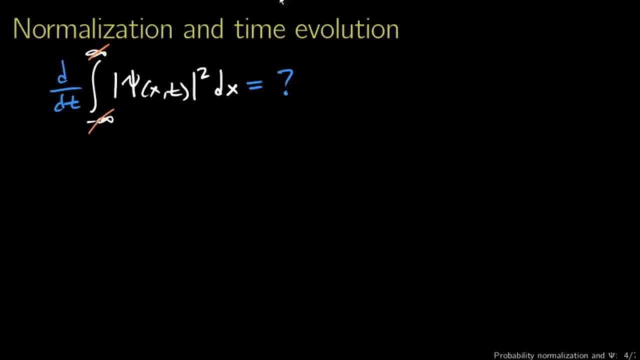 it's going to hold, So let's step through that. Manipulations of the Schrodinger equation like this are a little tricky to follow, so I'm going to go slowly, and if it seems like I'm being extra pedantic, please bear with me. 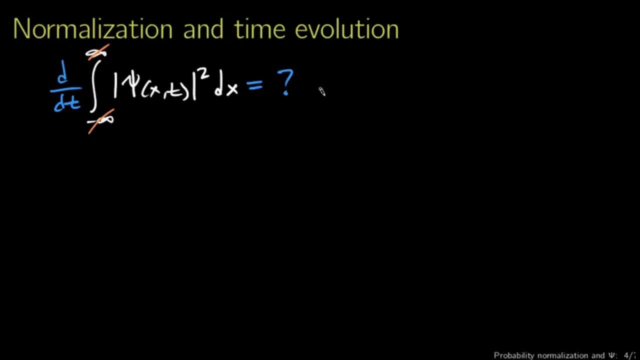 Some of the details are important. So the first thing that we're going to do- pretty much the only thing that we can do with this equation- is we're going to exchange the order of integration and differentiation Instead of differentiating with respect to time. 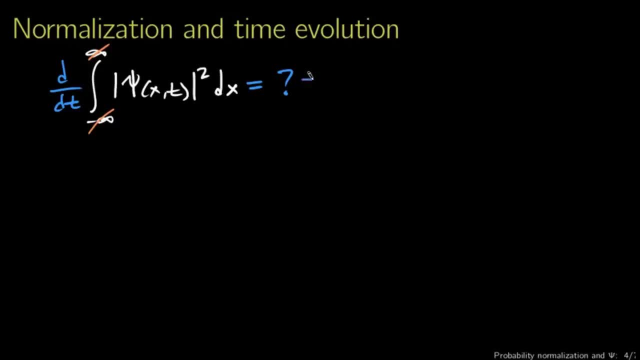 the integral with respect to x, we're going to integrate, with respect to x of the time, derivative of this psi of x and t quantity squared. Basically, I've just pushed the derivative inside the integral Now, notationally speaking, and I'm going to move some stuff around here. 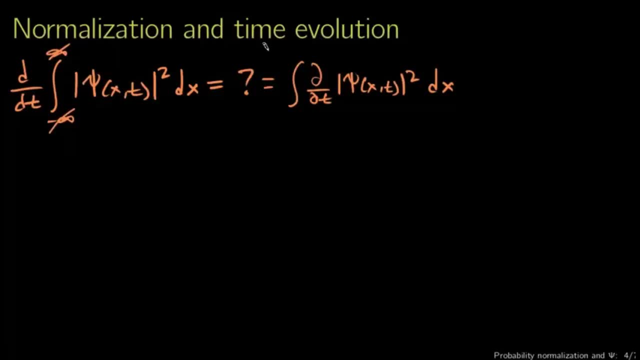 give myself a little more room. Notationally- oops didn't mean to change the colors. Notationally speaking, here the d- dt became a partial derivative. with respect to time. The total derivative d by dt is now a partial. 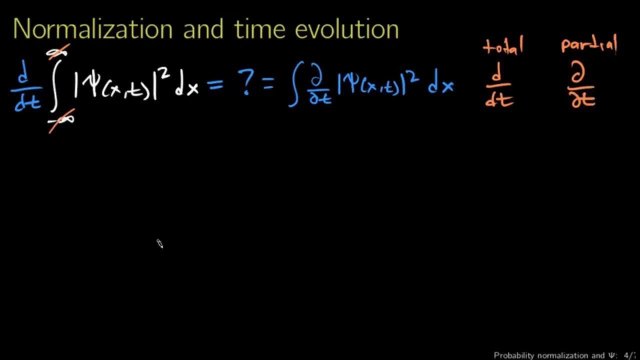 What the notation is keeping track of here is just the fact that this is a function only of time, since you've integrated over x and you've substituted in limits, Whereas this is a function of both space and time. So, whereas this derivative is acting on something, 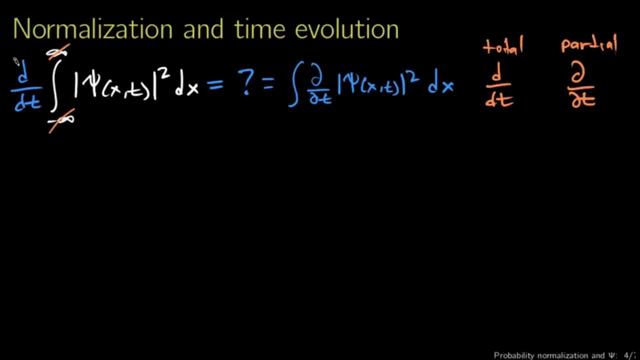 that's only a function of time. I can write it as a simple d by dt, the total derivative In this case. since what the derivative is acting on is a function of both position and time, I have to treat this as a partial derivative. now, 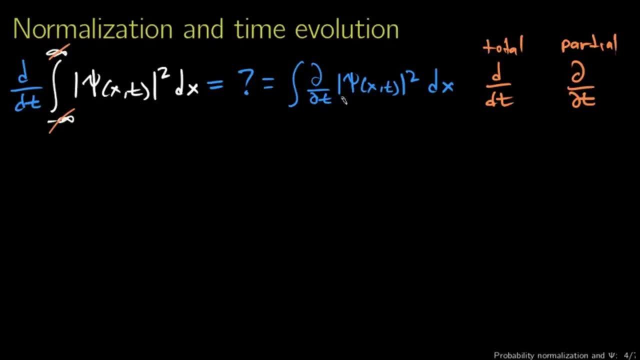 So the next thing that we're going to do, aside from after pushing this derivative inside and converting it to a partial derivative, is rewrite this squared absolute magnitude of psi as psi star times psi. Now, the squared absolute magnitude of a complex number is equal to the complex number times its complex conjugate. 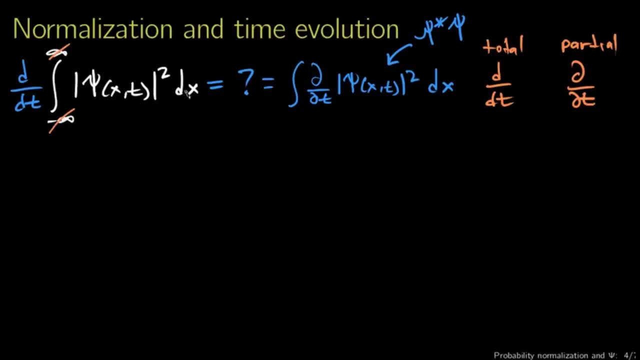 It's just simple, complex analysis rules there. So what we've got is the integral of the partial derivative with respect to time of psi, star times, psi integral of the x. Now we have a time derivative applied to a product. We can apply the product rule. 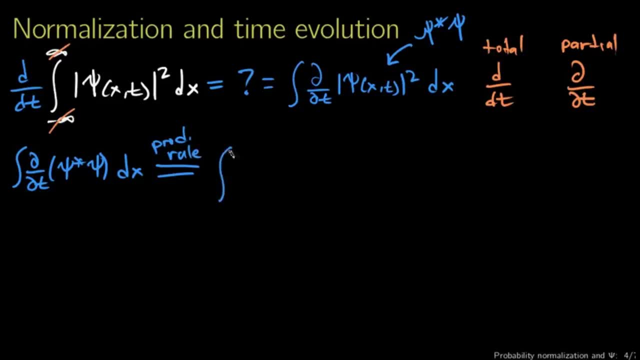 from differential calculus And what we end up with is the integral of the partial derivative, with respect to time, of psi, star times, psi plus psi. star. partial derivative of psi with respect to time, That's integrated dx. Now what I'm going to do is I'm going to notice. 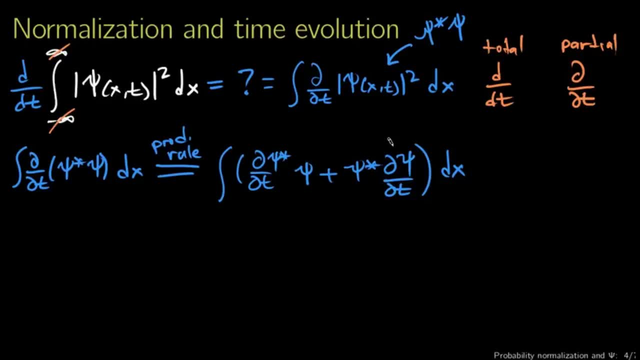 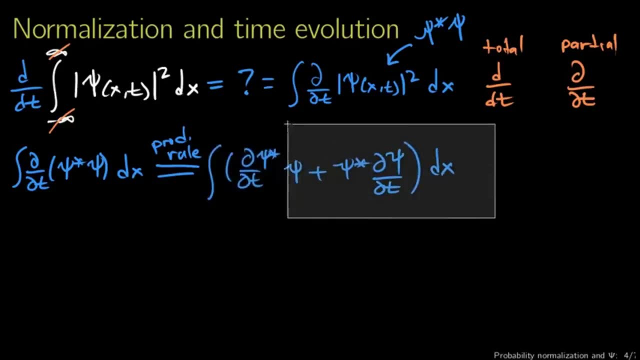 these partial derivatives with respect to time And I'm going to ask you to bear with me for a minute while I make a little more space. It's probably a bad sign if I'm running out of space on a computer where I have effectively infinite space. 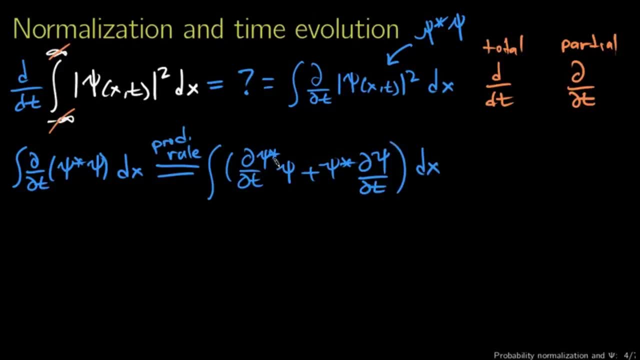 But bear with me. The partial derivatives with respect to time appear in the Schrodinger equation i: h bar d by dt of psi equals minus h bar squared over 2m. partial derivative. second partial derivative of psi with respect to position plus potential times: psi. 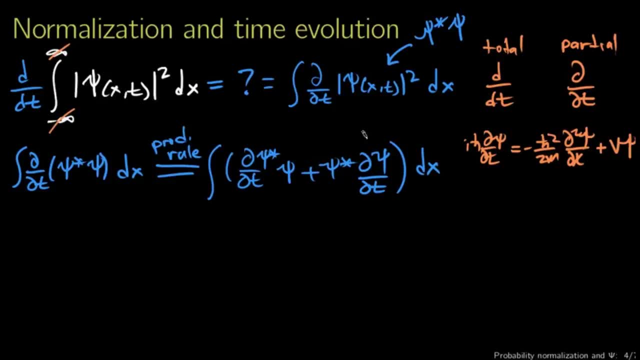 These are the time derivatives that I'm interested in. I can use the Schrodinger equation to substitute in, say, the right hand side for these time derivatives, both for psi star and for psi. So first I'm going to manipulate this by dividing through by i h bar. 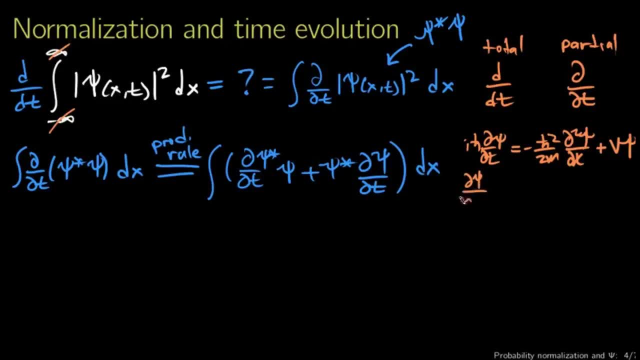 which gives me partial psi. partial time equals i, h bar over 2m. second partial of psi with respect to x minus. where did it go? i v over h bar psi, So that can be substituted in here. I also need to know something for the complex conjugate of psi. 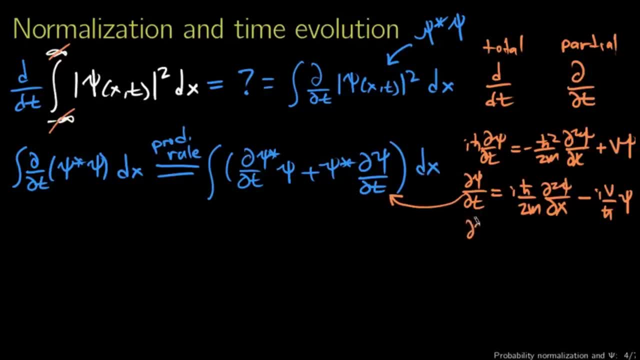 so I'm going to take the complex conjugate of this entire equation. What that looks like is partial derivative of psi star with respect to time. Now I'm taking the complex conjugate of this, so I have a complex part here. the sine of that needs to be flipped. 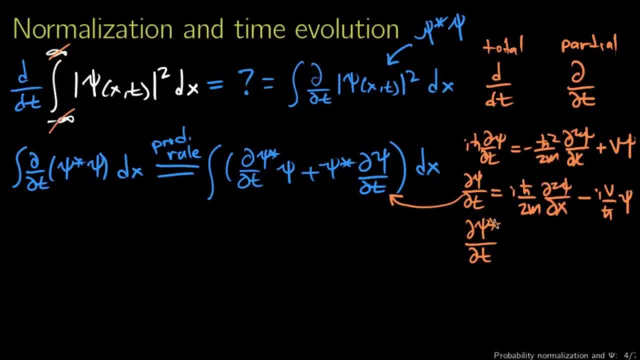 and I have a complex number here that needs to be complex conjugated, since the complex conjugate of a product is the product of the complex conjugates. What that means is this is going to become: i h bar over 2m d squared psi star. 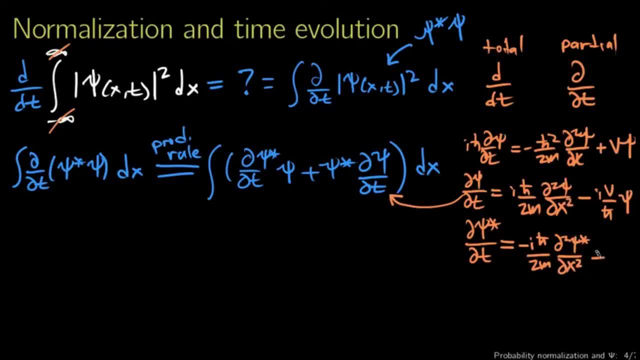 dx squared- sorry, I forgot the squared there- plus i, v over h bar psi. So I've just gone through and changed the signs on all of the imaginary parts of all these numbers: Psi became psi star, i became minus, i minus. i became i. This can be substituted in for that. 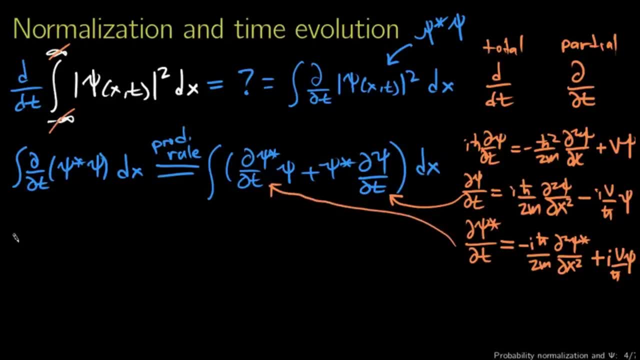 What you get when you make that substitution. this equation isn't really getting simpler, is it? It's getting longer. What you get is the integral of something. I'll put an open square bracket at the beginning. here I've got this equation minus i h bar. 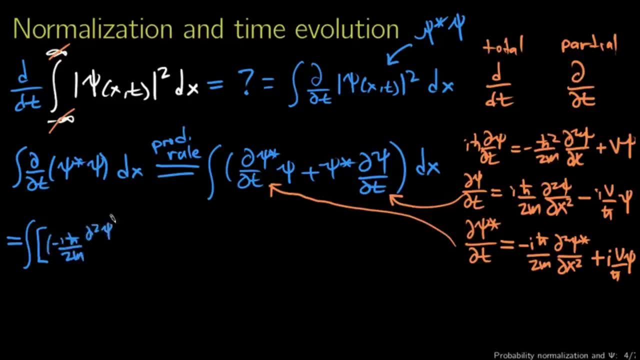 over 2m. the second partial derivative of psi star, partial x squared plus i, v over h bar psi star. that's multiplied by psi from here. So I've just substituted in this expression for this. Now the next part: I have plus psi star and 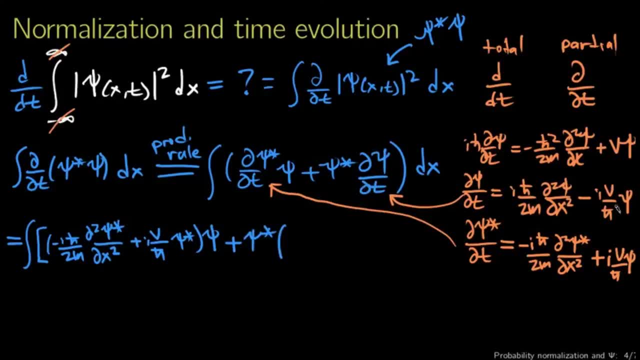 whatever I'm going to substitute in from this, which is what I get from this version of the Schrodinger equation here: i h bar over 2m. second partial derivative of psi with respect to x minus i v over h bar psi. close parentheses, close square brackets. 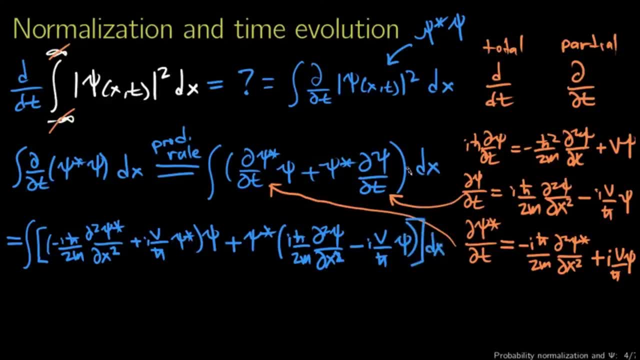 and I'm integrating dx Now. this doesn't look particularly simple, but if you notice what we've got here this term, if I distributed this psi in would have i v over h bar psi star times: psi. this term. if I distributed this psi star in would have an i. 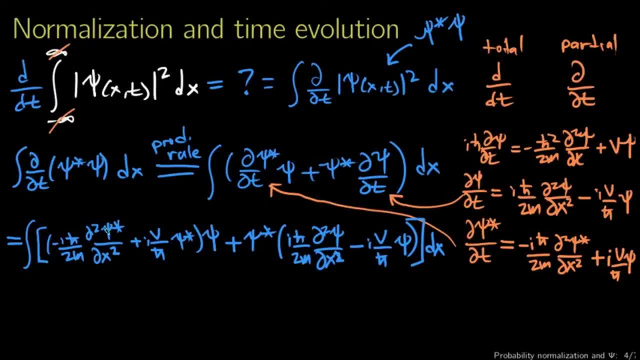 v over h bar. psi, star and psi. this term has a plus sign, this term has a minus sign, so these terms actually cancel out what we're left with then to rewrite things. both of the terms that remain have this minus. i h bar over 2m. 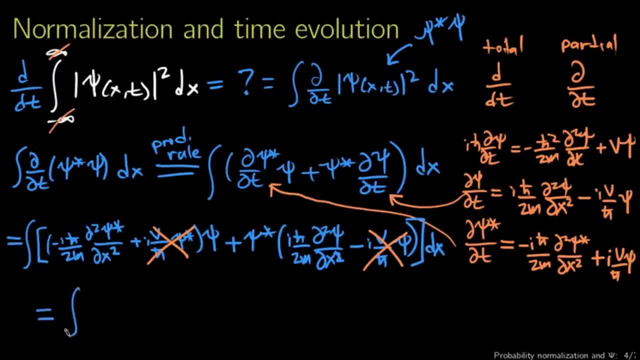 out front. so we're going to have equals to i h bar over 2m. and here I have a minus second partial derivative of psi star with respect to x times psi, and here I have plus psi star times the corresponding second partial of psi with respect to x. 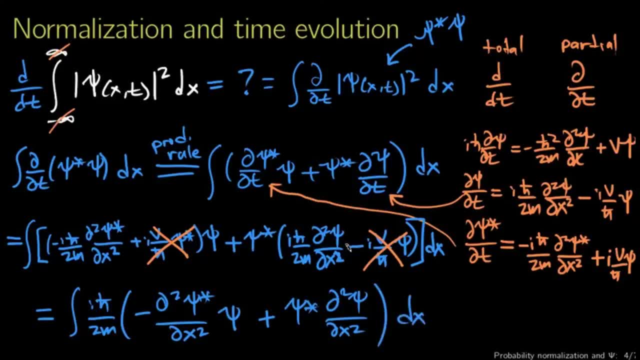 and this is integrated dx. is that all right? yes, Now what I'd like you to notice here is that we've got d by dx and we've got an integral dx. we don't have any time anymore, so we're making progress and we're actually almost done. 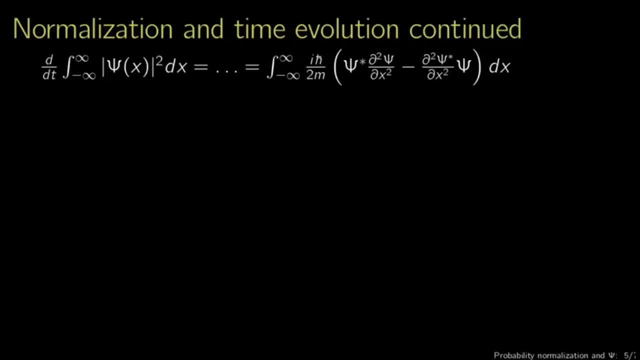 where did we get so far? we started with the time derivative of this effective total probability, which should have been equal to one, which would be equal to one if this were a proper probability distribution. but we're just considered with the time evolution, since we know that. 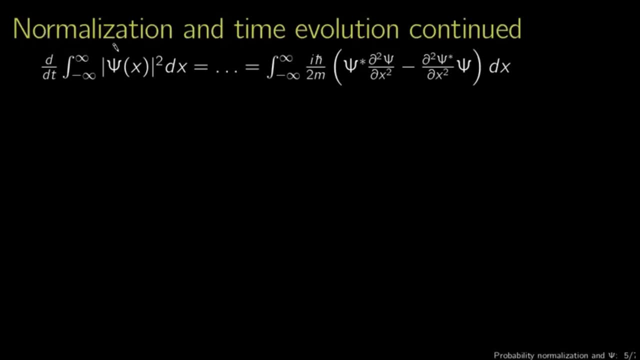 whatever psi is, we can multiply it by some constant to make it properly normalized at a particular time. now we're interested in the time evolution, we're looking at the time derivative of this and we've gone to this expression which has complex conjugates of psi and second partial derivatives. 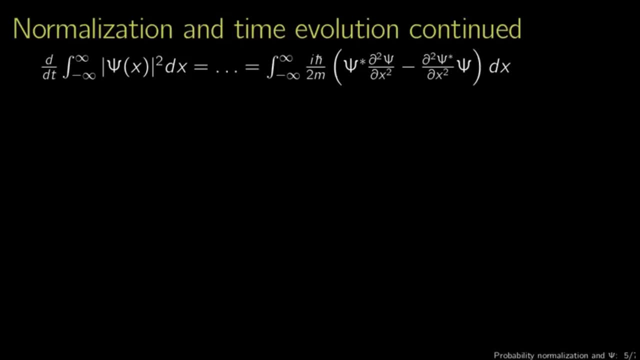 with respect to x. now, what I'd like you to do- and this is a check your understanding question- is: think about why this statement is true. this is the partial derivative, with respect to x, of psi star d, psi dx minus d, psi star dx. sorry, I'm saying d, I should be saying partial. 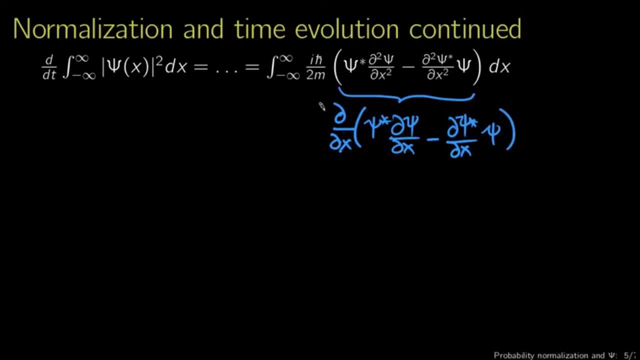 these are partial derivatives. this is true and it's up to you to figure out why. but since this is true, the derivative is: we have our i h bar over 2 m, an integral over minus infinity, to infinity of this expression, partial with respect to x of. 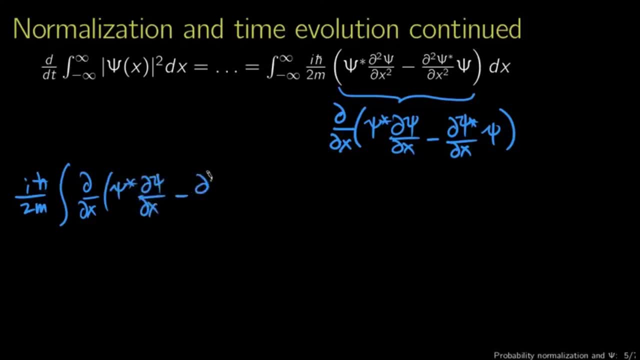 psi. star partial psi. partial x minus. partial psi. star partial x psi. we're integrating dx now, and this is nice because we're integrating dx of a derivative of something with respect to x. so that's easy. fundamental theorem of calculus. we end up with i h bar over 2 m. 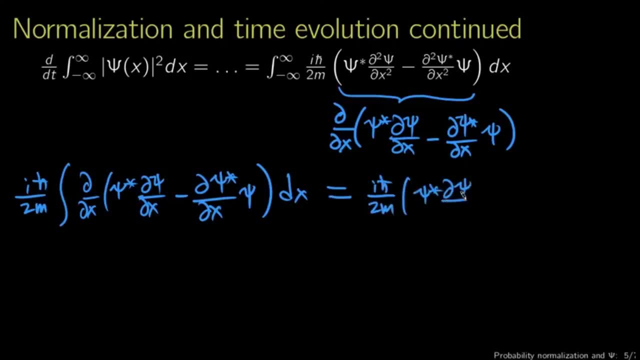 psi. star partial psi partial x. minus partial psi. star partial x. psi evaluated at the limits of our integral, which are minus infinity to infinity. now, if psi is going to be normalizable, we know something about the value of psi at negative and positive infinity. if psi is normalizable, 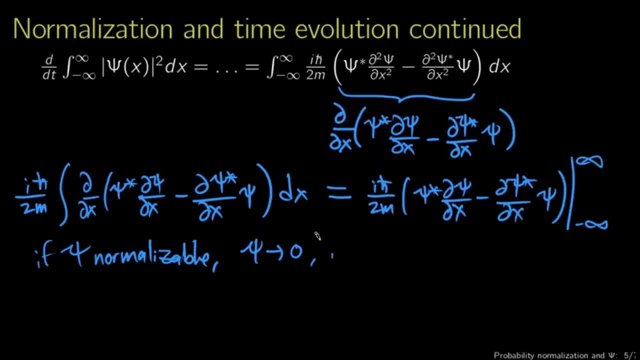 psi has to go to zero, as x goes to negative and positive infinity. what that means is that when I plug in the infinity here, I'm just going to get zero and zero. so the bottom line here, after all of this manipulation, is that this is equal to zero. 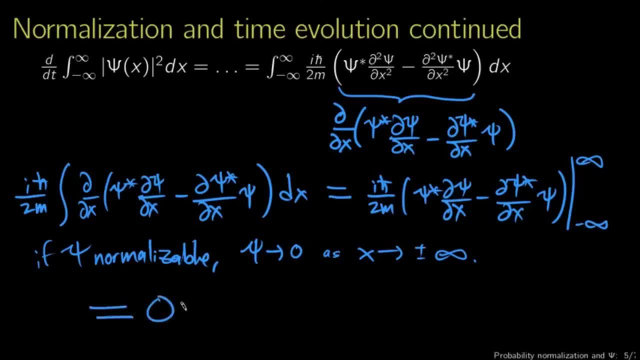 what that means is that the integral from negative infinity to infinity of the square, to absolute magnitude of psi, has a function of both x and time is equal to zero. so if psi is equal to a constant, put another way, time evolution does not affect normalization. what that means is that: 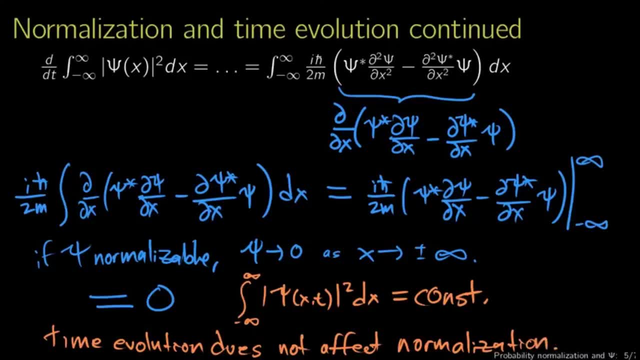 I can take my candidate wave function not normalized, integrate it, find out what I would have to multiply or divide it by to make it normalized and if I'm successful, I have my normalized wave function. I don't need to worry about how the system evolves in time. 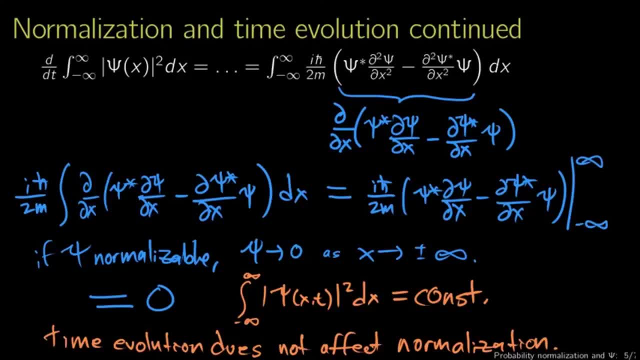 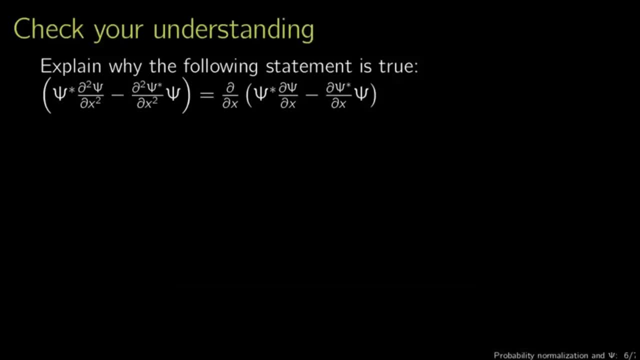 the Schrodinger equation does not affect the normalization. so this is that. check your understanding question. I mentioned the following statement: was that crucial step in the derivation and I want you to show that this is true. explain why in your own words. now to do an example here: 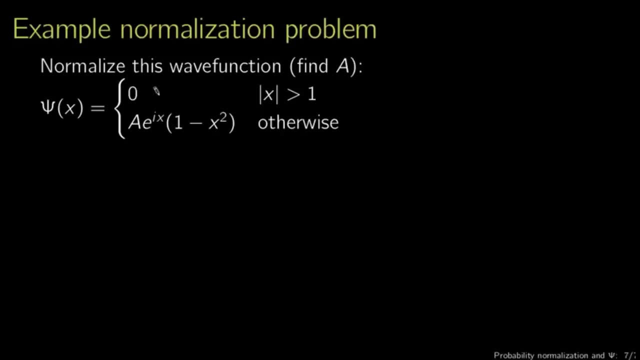 normalize this wave function. what that means is that we're going to have to find a constant- and I've already put the constant in the wave function- a such that the integral from minus infinity to infinity of the squared absolute magnitude of psi, of x in this case. 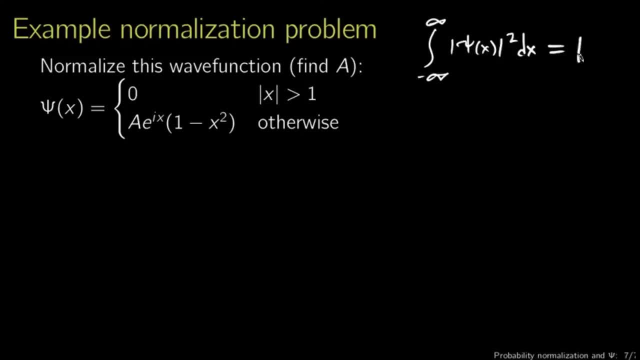 I've left the time dependence out is equal to one and same. as in the last problem, the first thing we're going to do is substitute the squared absolute magnitude of psi for psi, star times psi- the other thing I'm going to do before I get started. 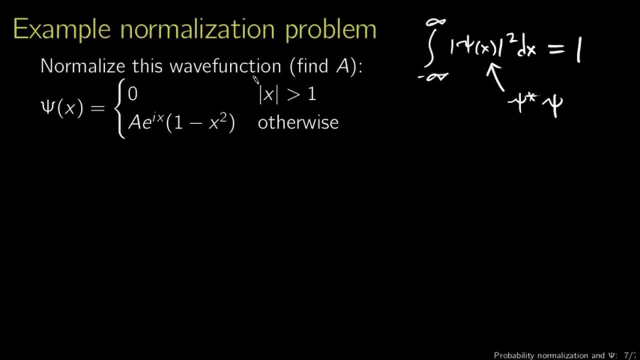 is. notice that my wave function is zero. if the absolute value of x is greater than one or less than one, I'm going to substitute the squared absolute magnitude of psi above one or below negative one. so instead of integrating from minus infinity to infinity here, I'm just going to focus on 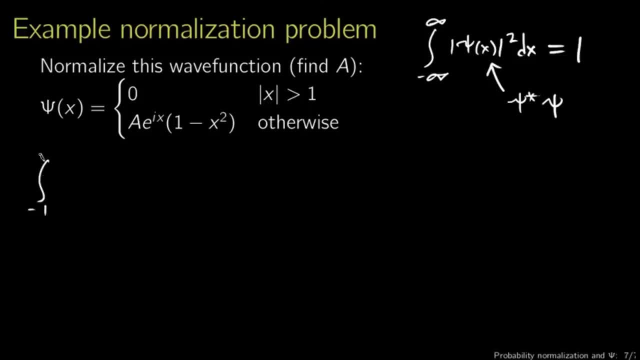 the part where psi is non-zero and integrate from minus one to one integral, from minus one to one of psi star, which is going to be a e to the i x, is going to become e to the minus i x and one minus x squared is still going to be. 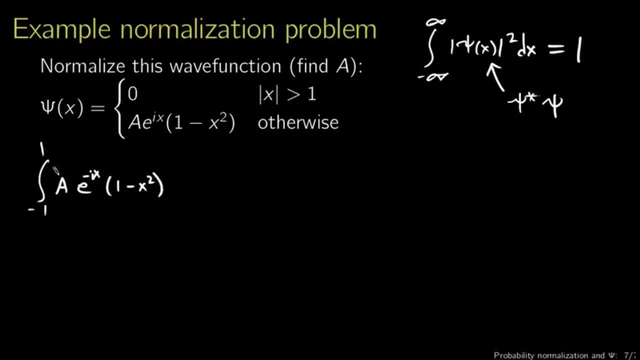 one minus x squared. now I haven't complex conjugated a, because part of the assumption about normalization constants like this is usually that you can choose them to be purely real. so I'm not going to worry about taking the complex conjugate of a, just to make my life a little easier. 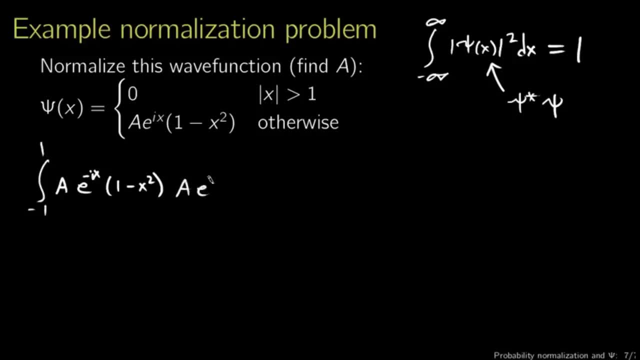 psi. well, that's just right here. a e to the i, x, one minus x squared and I'm integrating dx. this is psi star. this is psi integral dx. from minus one to one equal to one. so let's do this. we end up with a squared times the integral from. 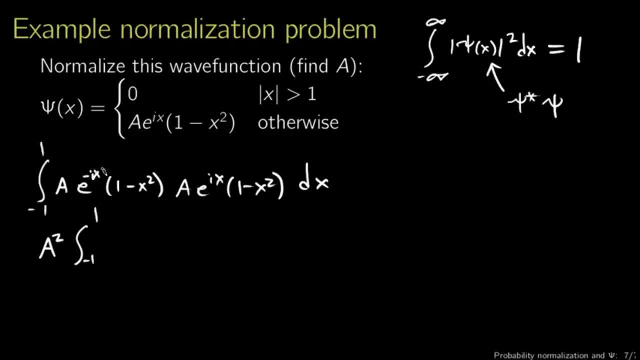 minus one to one, of e to the minus i x and e to the i x. what's e to the minus i x times e to the i x? well, thinking about this in terms of the geometric interpretation, we have e to the i x, which is cosine theta plus i sine theta. 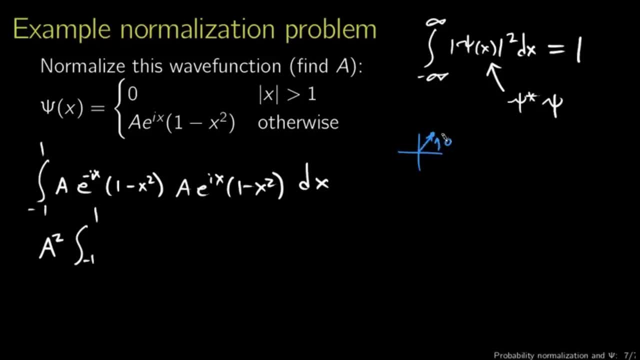 you can think about that as being somewhere on the unit circle at an angle. theta minus i. theta would just be in the exact opposite direction. so when I multiply them together, I'm going to get something that has the product of the magnitudes. the magnitudes are both one. 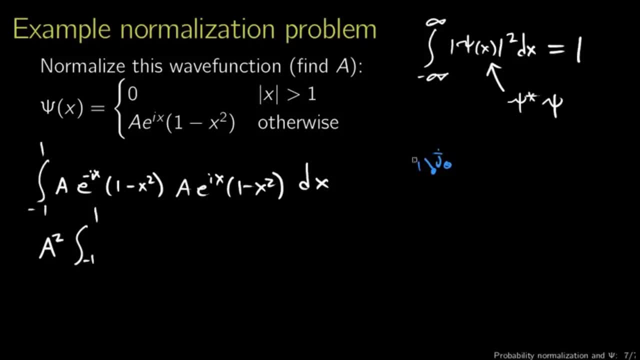 and it's purely real. you can see that also by looking at just the rules for multiplying exponentials like this: e to the minus, i x times e to the plus i x is e to the minus, i x plus i x, or e to the zero, which is one. 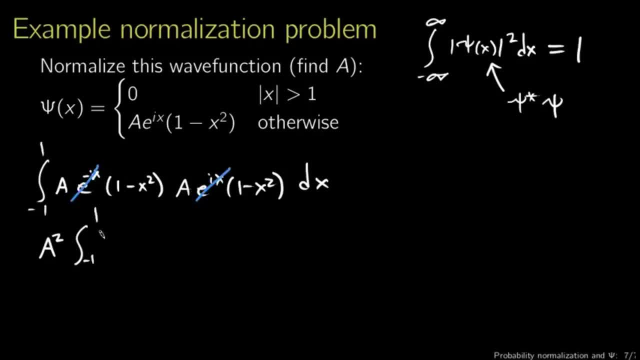 and cancel these out and what I'm left with is one minus x squared quantity squared dx. plugging through the algebra a little further, a squared integral minus one to one of one, minus two, x squared plus x to the fourth dx, you can do this. integral equals a squared. 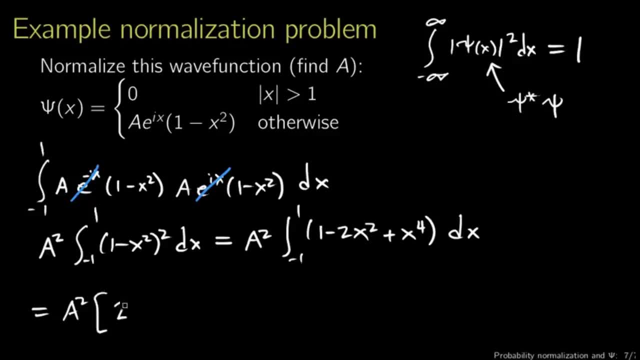 two x minus two, thirds x cubed plus x to the fifth, over five, between minus one and one, which, when you substitute in the limits, becomes a squared. this x part is going to be one minus the other limit minus one, which is one, minus minus one, which is two. 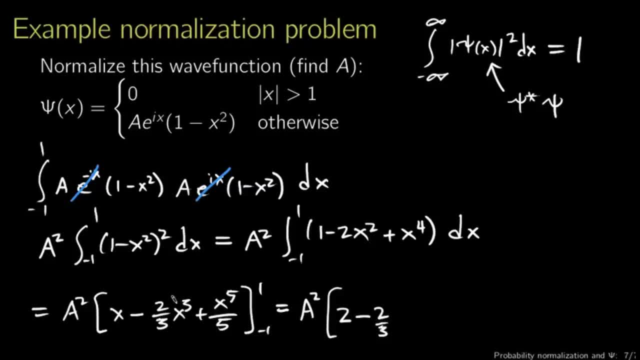 minus two thirds of whatever I get from the x cubed, which is again going to be one minus a minus one or two plus one fifth of x to the fifth, one minus one to the fifth and one to the fifth again. this is all basic algebra. hopefully this is not too confusing. 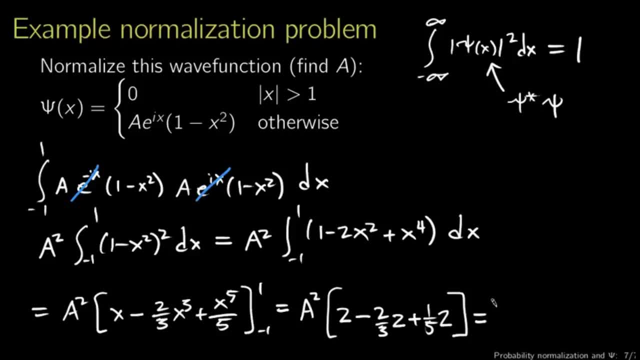 by this point, this ends up being a squared times sixteen over fifteen. now going up here: if a squared sixteen over fifteen is going to be equal to one, a has to be equal to the square root of fifteen over sixteen. that's what it means to normalize a wave function. 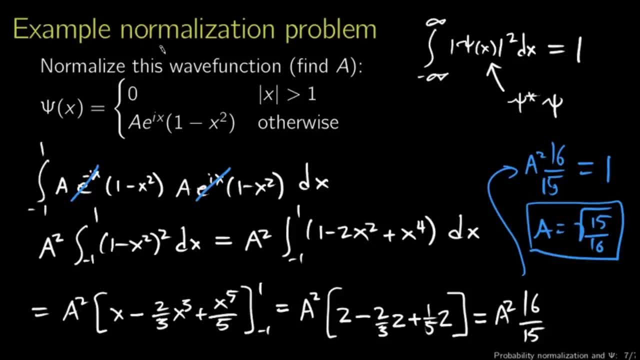 you have something that you think might be your wave function, but it's not properly normalized yet. so you guess that there's going to be some constant multiplied in and you write down the normalization condition integrating your wave function- absolute magnitude squared- which usually you will write as: 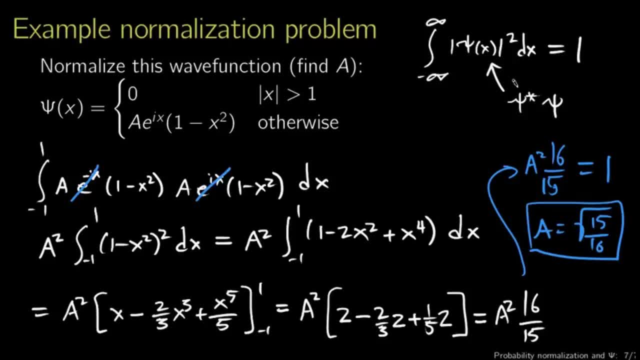 the wave function times its complex conjugate. typically, the complex parts of the wave function will drop out and you'll end up with just something that you can integrate. proceeding through the integral, you'll end up with some expression that tells you what that constant is. so that's the wave function. 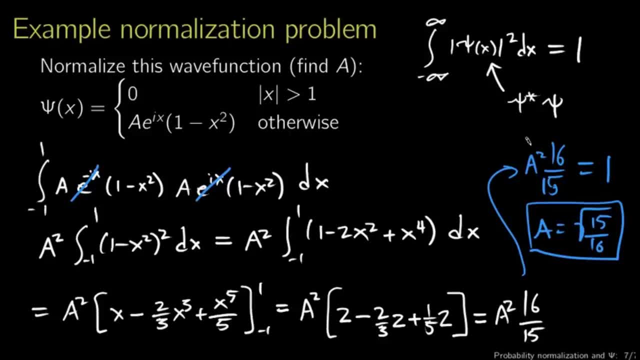 and how it's normalized. the time evolution of the normalization and the fact that it's not affected by the Schrodinger equation is really a nice feature of quantum mechanics. otherwise quantum mechanics would be completely unworkable. a lot of what we've talked about in this lecture has just been 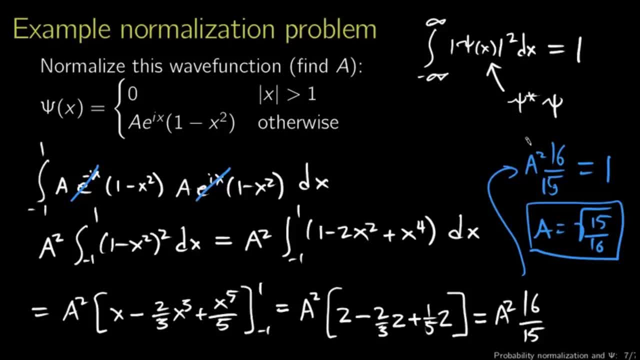 how to manipulate the Schrodinger equation or how to use the Schrodinger equation in manipulations of the wave function. and this is the sort of math that quantum mechanics is all about. there's calculus, there's partial derivatives, total derivatives, integrals. keeping track of everything is tricky. 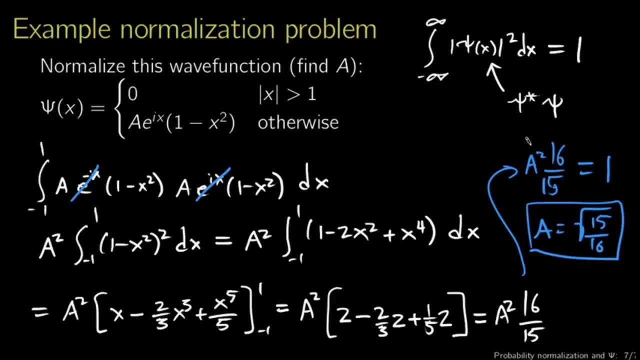 well, the result that we've got for normalization here helps- I'm rambling, though. at any rate, that's about it- for wave functions and normalization, and this is nice because all of the pieces that we've described today all fit together and support this statistical interpretation. 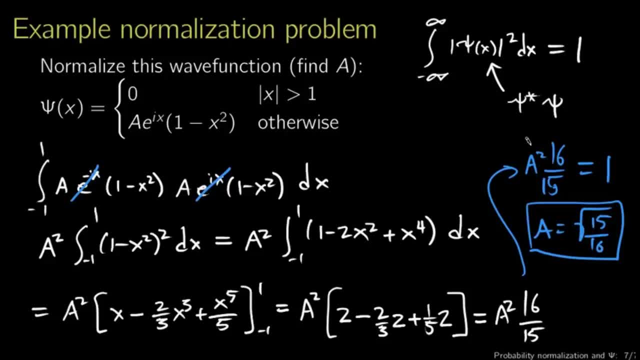 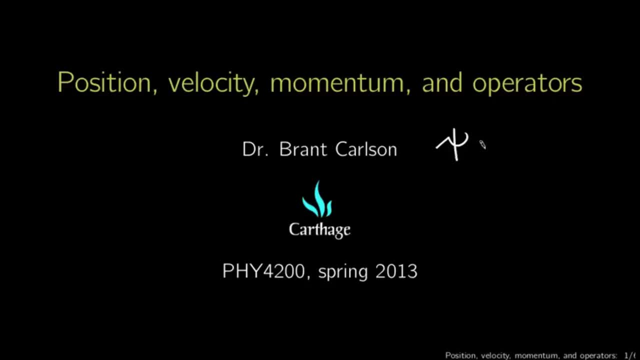 of the wave function as being related to a probability distribution. we know in quantum mechanics that all of the information about the physical system is encapsulated in the wave function psi. psi, then, ought to be related to physical quantities, for example position, velocity and momentum of the particle. 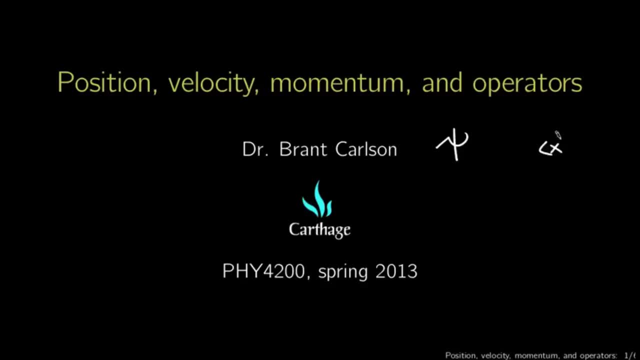 we know a little bit about the position. we know how to calculate things like the expected value of the position and we know how to calculate the probability that the particle is within a particular range of positions. but what about other dynamical variables like velocity or momentum? the connection with velocity and momentum? 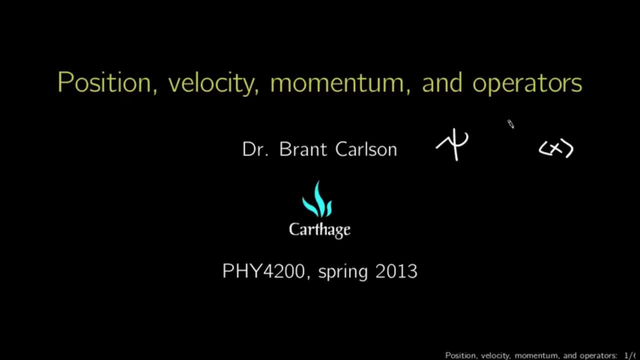 brings us to the point where we really have to talk about operators. operators are one of our fundamental concepts in quantum mechanics, and they connect the wave function with physical quantities. but let's take a step back first and think about what it means for a quantum system to move. 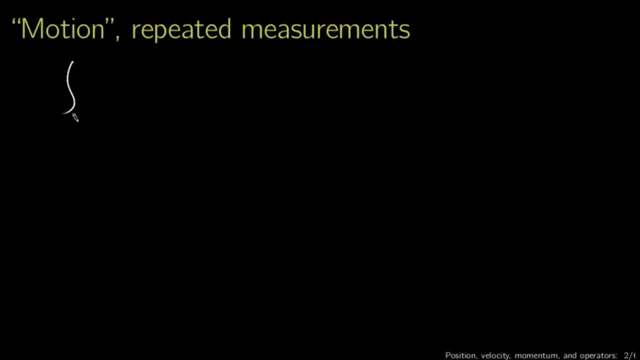 the position of the particle. we know, say, the integral from a to b of the squared magnitude of the wave function. dx gives us the probability that the particle is between a and b, and we know that the expected position is given by a similar expression, the integral from minus infinity to infinity. 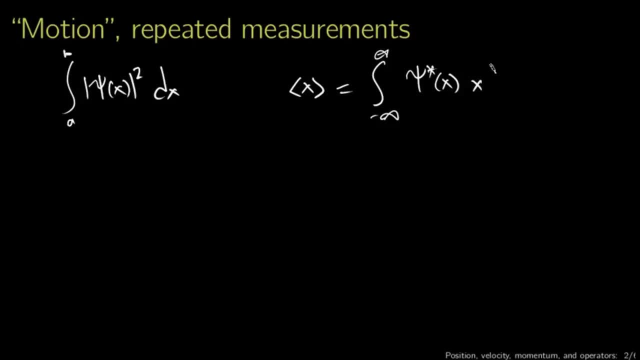 of psi star, of x times x times psi, of x dx. now, these expressions are related by the fact that the squared magnitude of psi is the probability density function describing position, and this is really just the calculation of the expected value of x, given that probability density function. 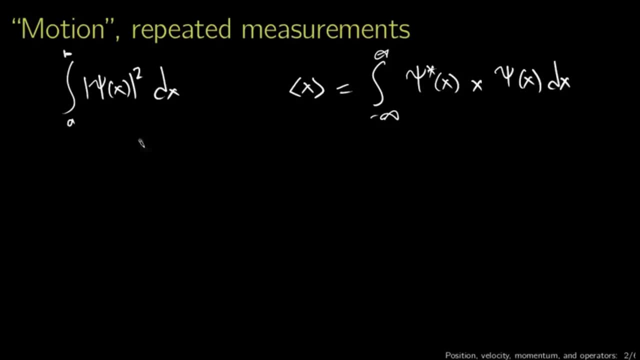 now what if I want to know what the motion of the particle is? one way to consider this is suppose I have a box and if I know the particle is, say here, at time t equals zero. what can quantum mechanics tell me about where the particle is later? 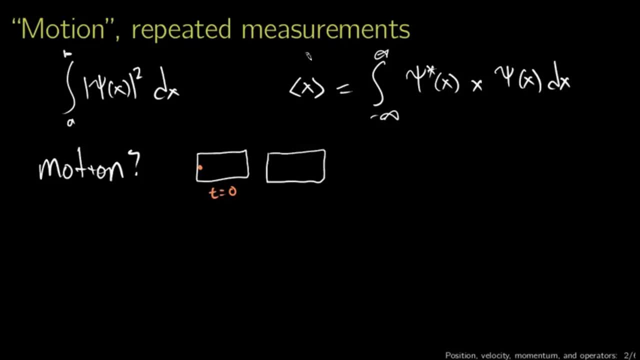 physically speaking. you could wait until say t equals one second and then measure the position of the particle. maybe it would be here. you could then wait a little longer and measure the particle again. maybe at that point it would be here at say t equals two seconds, or if I wait a little bit longer. 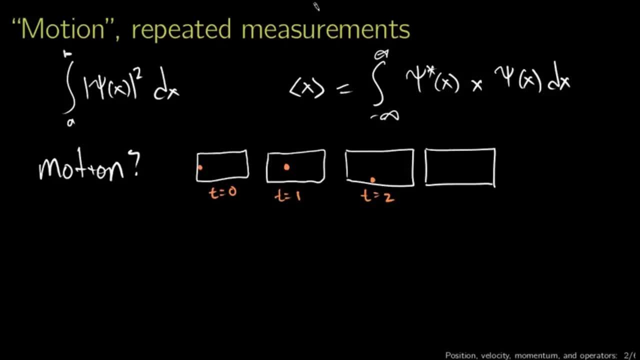 and measure the particle yet again. at, say, t equals three seconds, maybe the particle would be up here now. does that mean that the particle followed a path that looked something like this? no, we know that the position of the particle is not something that we can observe at any given time with impunity. 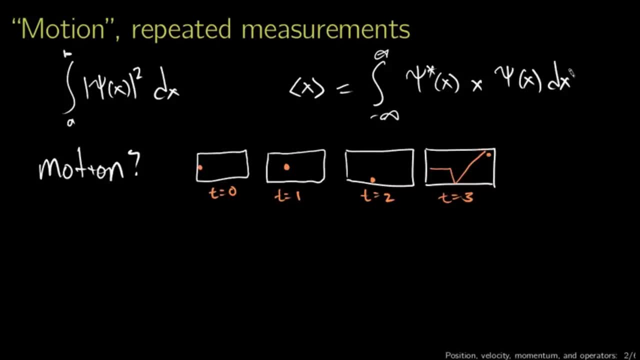 because of the way the observation process affects the wave function. back when we talked about measurement, we talked about having a wave function that looks something like this, a probability density that looks something like that, and then, after we measure the position of the particle, the probability density has changed. 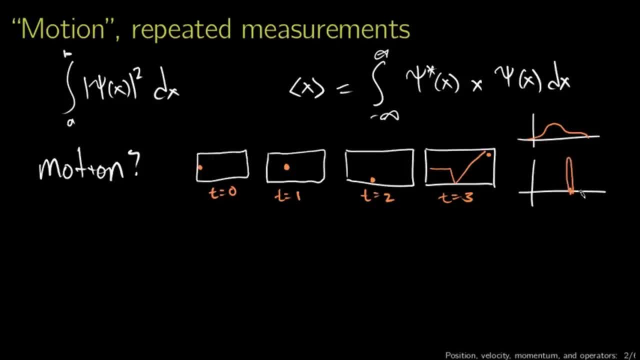 if we say measure the particle to be here, the wave function has to accommodate that new probability density function. the fact that measurement affects the system like this means that we really can't imagine repeatedly measuring the position of a particle in the same system. what we really need 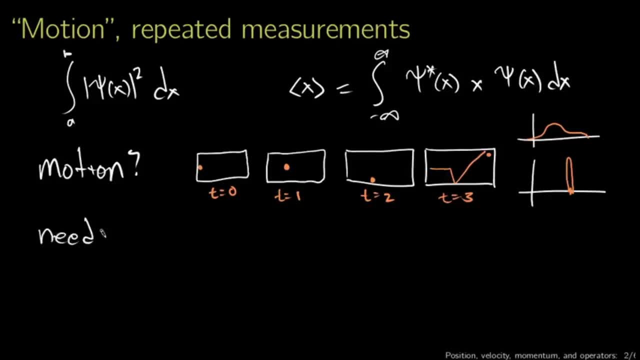 is an ensemble. that's the technical term for what we need. what an ensemble means in this context is that you have many identically prepared systems. now, if I had many identically prepared systems, I could measure the position over and over and over and over again, once per system. 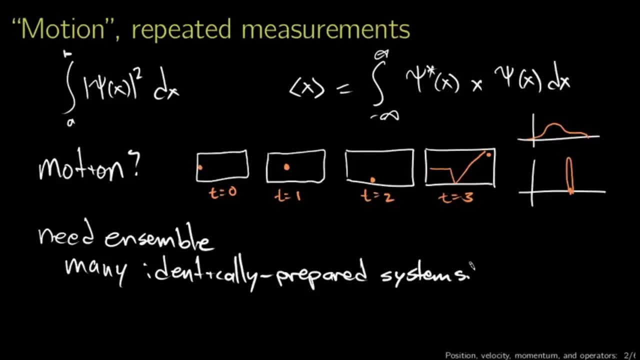 if I have 100 systems, I could measure the position 100 times, and that would give me a pretty good feel for what the probability density for position measurements is. if I wanted to know about the motion of the particle, I could do that again, except instead of taking my 100 measurements. 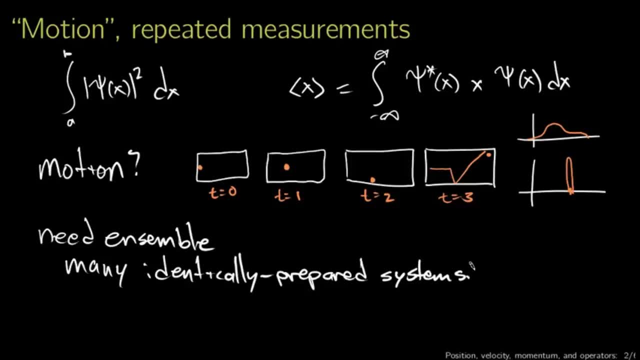 all at the same time. I would take them at slightly different times, so, instead of this being the same system, these would all be different systems that have been allowed to evolve for different amounts of time and, as such, the motion of the particle isn't going to end up looking something like that. 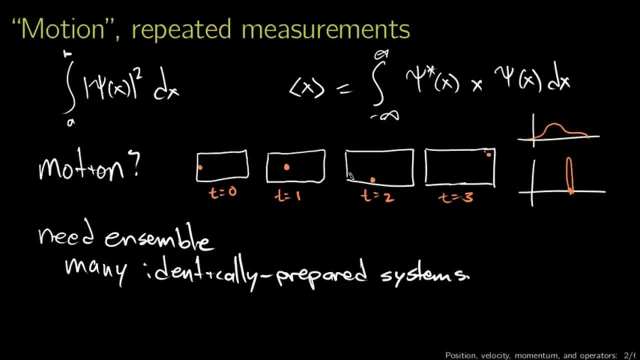 it's going to end up looking like some sort of probabilistic motion of the wave function in space. what we're really interested in here? oh, sorry, I should make a note of that many, oops, sorry. single measurement per system, this notion of averaging over many identically prepared systems. 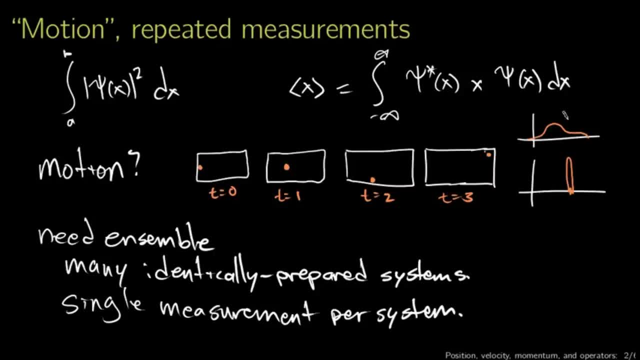 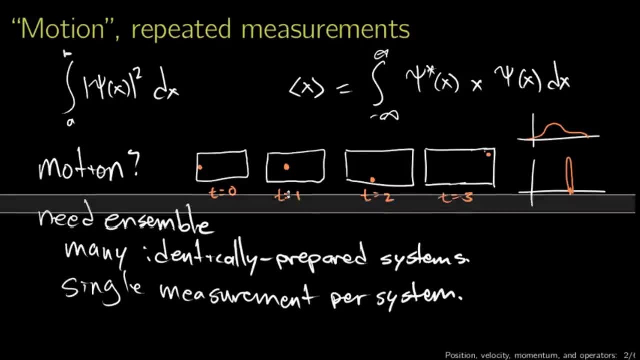 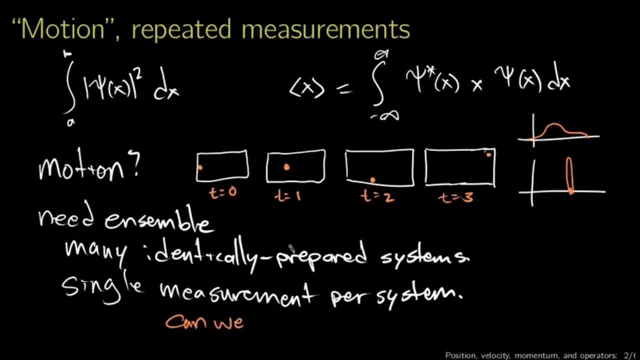 is important in quantum mechanics because of this effect that measurement has on the system. so what we're interested in now in the context of something like motion is: well, can we predict this? can we predict where the particle is likely to be as a function of time? and yes, we can. 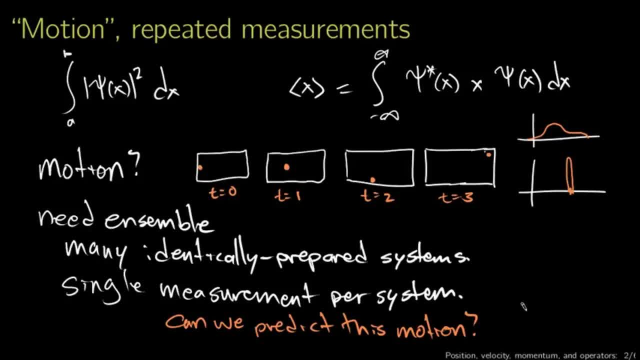 and what I'd like to do, to talk about that is to consider a quantum mechanical calculation that we can actually do: the time derivative of the expected value of position. this time derivative tells us how the center of the probability distribution, if you want to think about it that way. 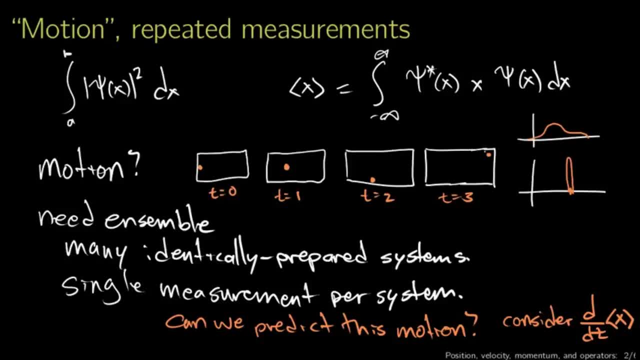 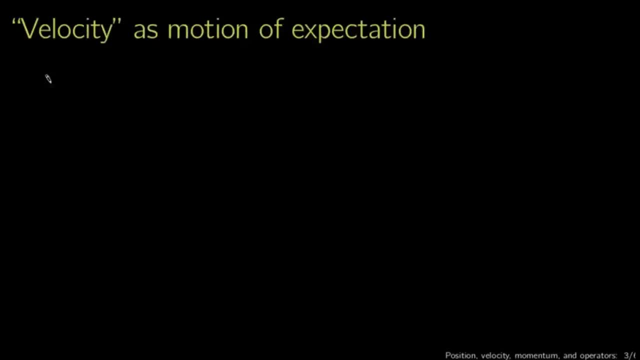 how the center of the wave function moves with time. so this time derivative d by dt of the expected value of x, that's d by dt of. let's just write out the expected value of x integral from minus infinity to infinity of x times psi, star of x. 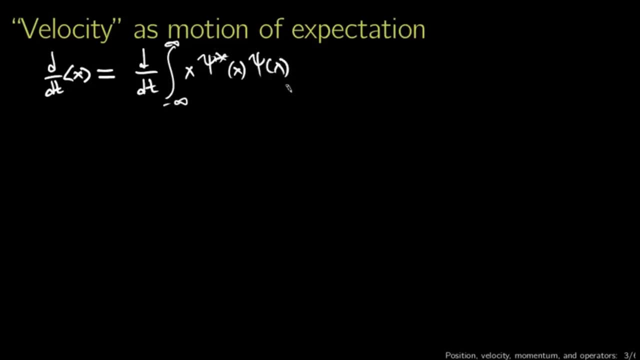 psi of x, where this is the probability density function given by the wave function and this is x. we're integrating dx now. if you remember when we talked about normalization, whether the normalization of the wave function changed as the wave function evolved in time, we're going to do the same sort of 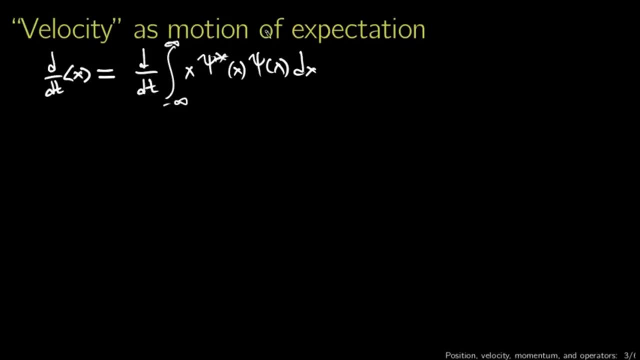 calculation with this. we're going to do some calculus with this expression. we're going to apply the Schrodinger equation but, as before, the first thing we're going to do is move this derivative inside the equation. this is a total time derivative of something that's a function of. in principle, 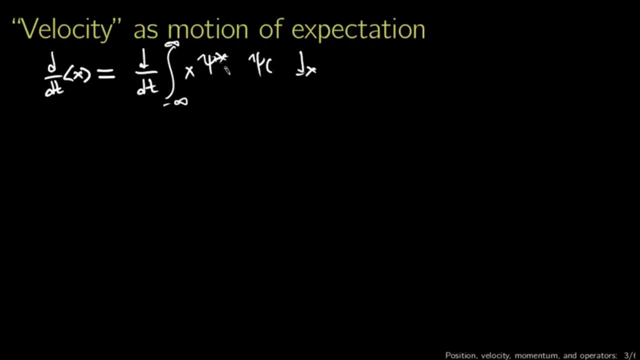 position and time. I should write these as functions of x and t, and what you get when you push that in is as before: the integral or the total derivative becomes a partial derivative, since x is just the coordinate x. in this context of functions of both space and time. 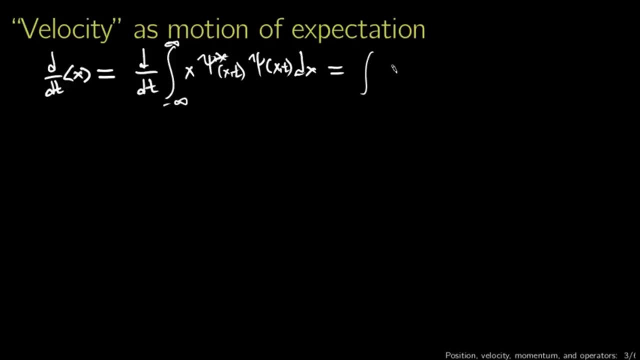 the total time derivative will not affect the coordinate x, even if it becomes a partial derivative. so what we'll end up with is x times the partial time derivative of psi, star, psi integral dx. I'm not going to write the integral from minus infinity to infinity here, just to save myself. 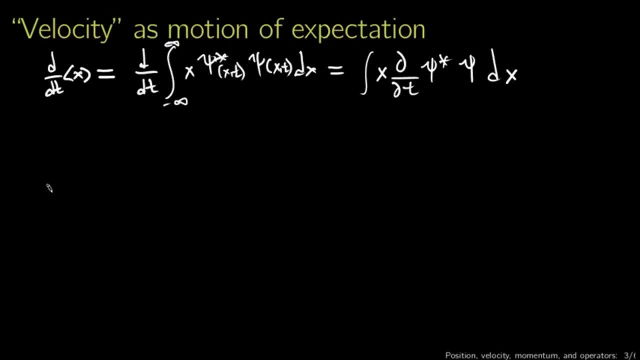 some time now, if you remember this expression, the integral- or sorry, not the full integral, just the partial time derivative of psi, star psi. that was what we worked with in the lecture on normalization. so if we apply the result from the lecture on normalization and it's equation 126, 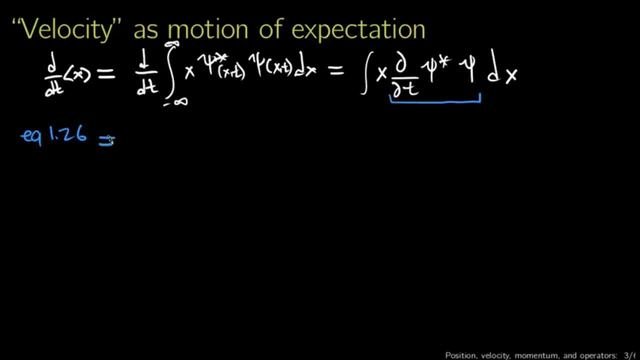 yes in the book. um, if we apply that, you can simplify this down a lot right off the bat and what you end up with is i, h bar over 2m times this integral x, and then what we substitute in equation 126 gives an expression for this highlighted part here. 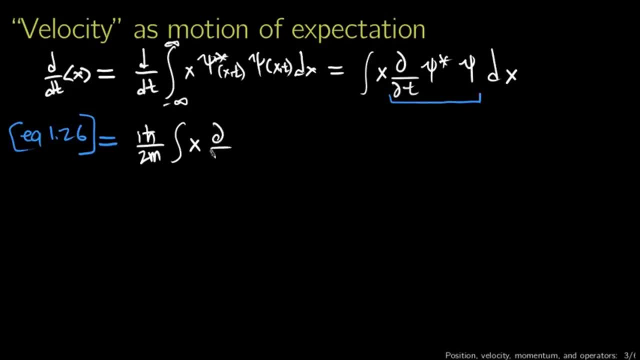 in orange, and what you get is the partial derivative, with respect to x, of psi star, partial of psi with respect to x minus. partial of psi star with respect to x times psi integral, still with respect to dx, of course. now, if we look at this equation, we're making the same sort of progress we made. 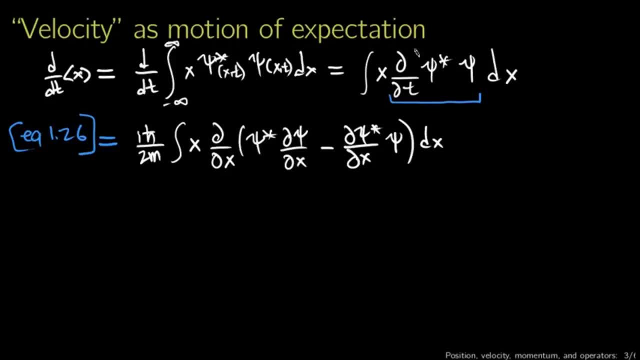 when we did the normalization derivation, um, we had time derivatives here, now we have only space derivatives, and we have only space derivatives in an integral over space. so this is definitely progress. now we can start thinking about what we can do with integration by parts. the first integration by parts i'm 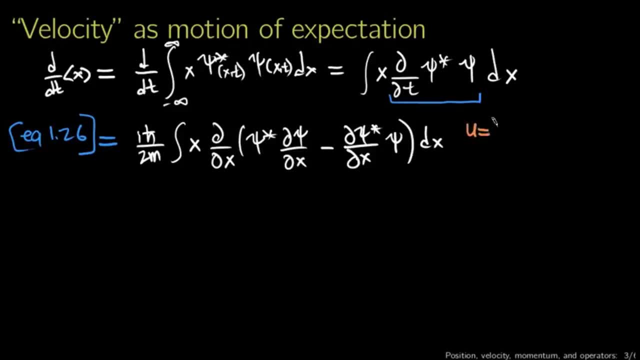 going to do has the non-differential part just being x and the differential part being dv is equal to. you know, i'm not going to have space to write this here, i'm going to move stuff around a little bit. so the differential part is dv is the partial derivative. 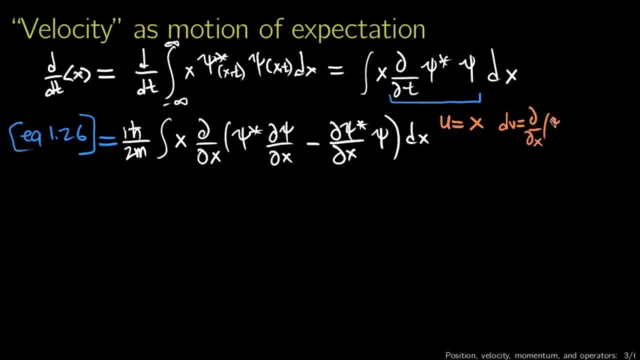 well, what's left of this equation? the partial derivative, with respect to x, of psi, star d, psi, dx, minus d psi, dx, psi. oh sorry, d psi, star, dx, psi. and then there's the dx from the integral. sorry, i'm running out of space. this um differential. 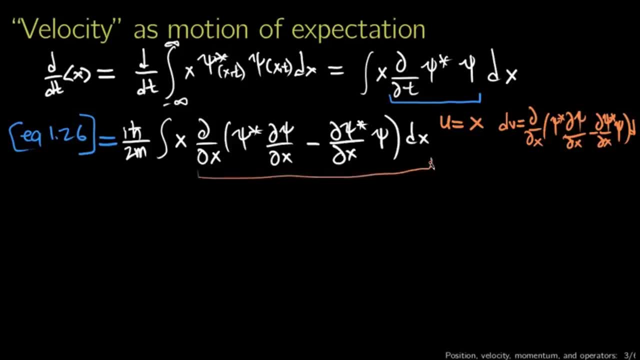 part. here is just this part of the equation. so now i can take this derivative du- dx in my integration by parts procedure. du equals dx and dv here is easy to integrate because this is a derivative. so when i integrate the derivative there i'll just end up with v equals. 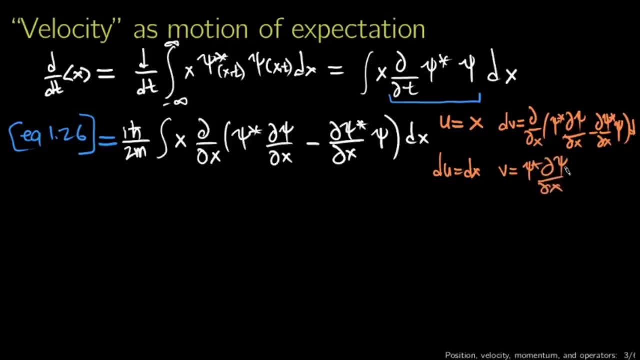 psi star d psi dx. minus d psi star, dx psi. now when i actually apply those, that integration by parts- the boundary term here without the integral in it- is going to involve these two. so i'm going to have x times psi star, partial psi. partial x. minus partial psi star. 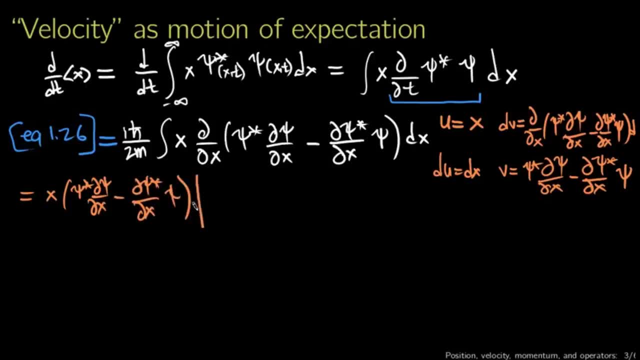 partial x psi, and that's going to be evaluated between minus infinity and infinity, the limits on my integral, the integral part which comes in with the minus sign, is going to be composed of these bottom two terms: integral of psi, star. partial psi, partial x minus. partial psi, star. 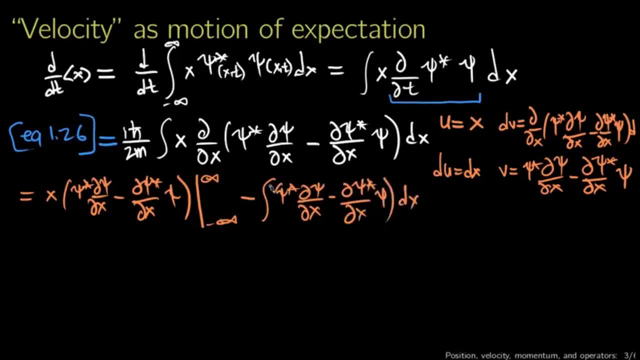 partial x, psi and its integral dx from minus infinity to infinity. now what's nice? oh, you know, i forgot something here. what did i forget my leading constants? i still have this ih bar over 2m out there. ih bar over 2m is multiplied by this entire expression. 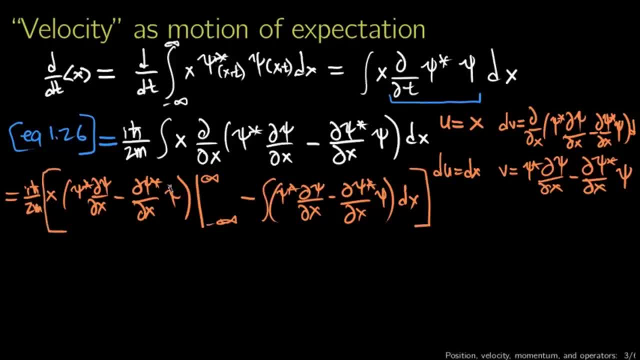 now the boundary terms here vanish. the boundary terms in integration by parts in quantum mechanics will often vanish, because if you're evaluating something at, say, infinity, psi has to go to zero at infinity. so this term is going to vanish. psi star has to go to zero at infinity. 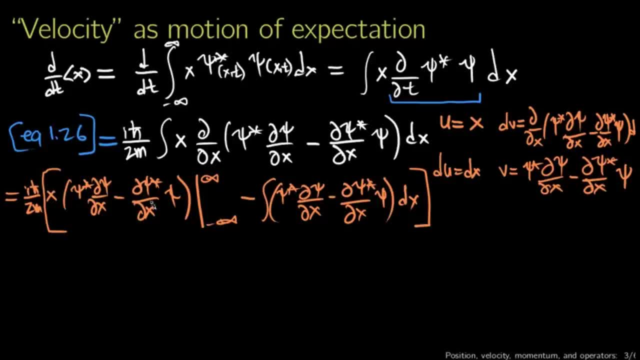 so this is going to vanish. so even though x is going to infinity, psi is going to zero, and if you dig into the mathematics of quantum mechanics, you can show convincingly that x times psi goes to infinity is going to be zero. so this boundary term vanishes. 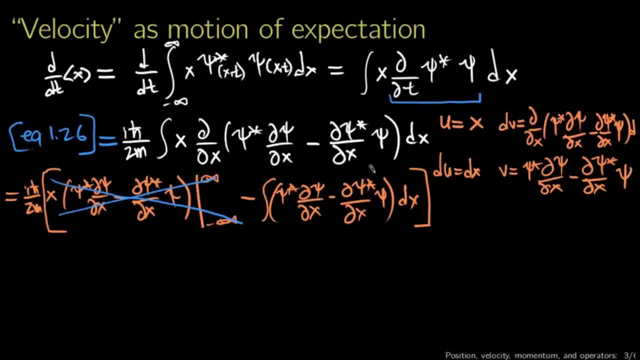 both at infinity and at minus infinity, and all we're left with is this: yes, all you're left with is that. so i'll write that over ih bar, over 2m times the integral of psi star partial psi partial x. minus partial psi star partial x. 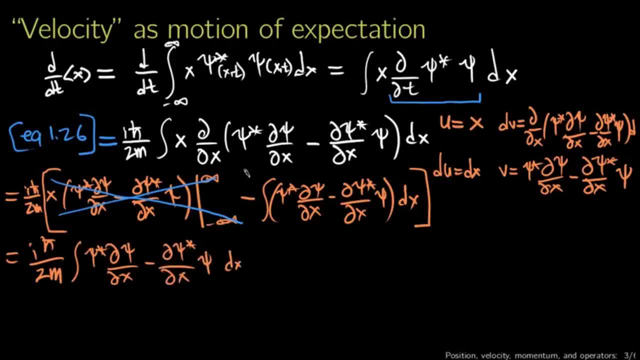 psi integral dx. i'm actually going to split that up into two separate integrals. so i'll stick another integral sign in here and i'll put a dx there and i'll put parentheses around everything so my leading constant gets multiplied in properly. and now i'm going to apply integration by parts again. 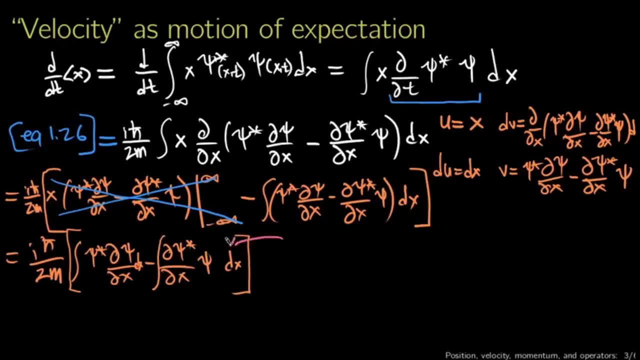 but this time just to the second integral here. so here we're going to say u is equal to psi and dv is equal to, again using the fact that when we do this integral, if we can integrate a derivative, that potentially simplifies things. so this is going to be partial psi. 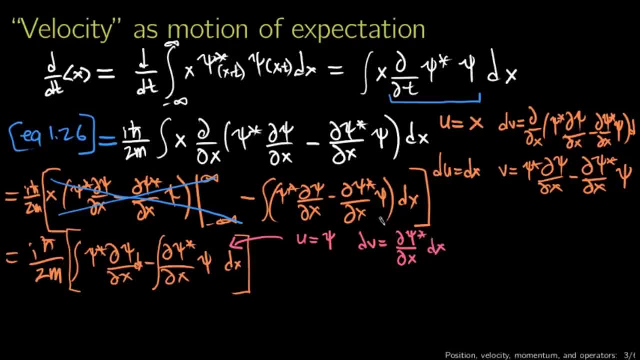 star, partial x, dx. so when we take the derivative of this, we're going to get: du is equal to partial psi, partial x, and when we integrate this, we're going to get v equals psi star. now, when we do the integration, when we write down the answer, 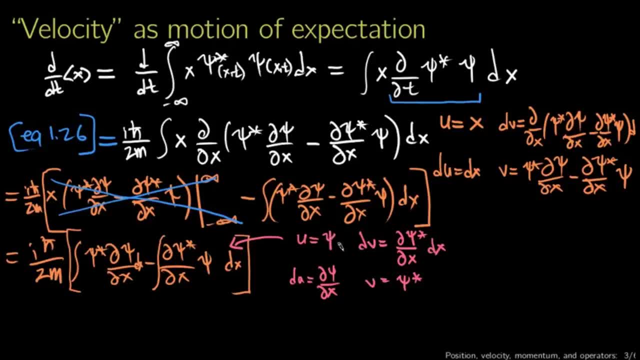 from this integration by parts, the boundary term here, psi star times, psi- is going to vanish again because we're evaluating it at a region where both psi star and psi well vanish. so the boundary term vanishes and you notice i have a minus sign here. when we do the integration by parts, 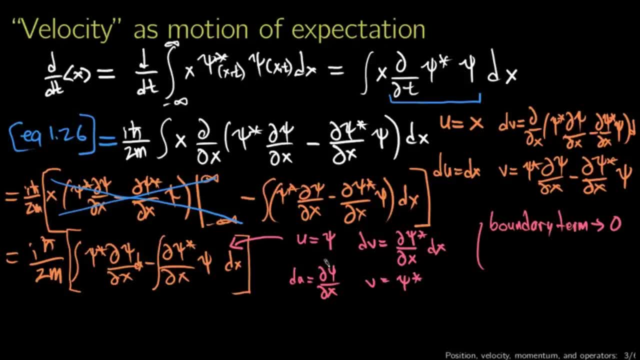 the integral term has a minus sign in it here. so we're going to have the partial psi with respect to x and psi star, with a minus sign coming from the integration by parts and a minus sign coming from the leading term here. so we're going to 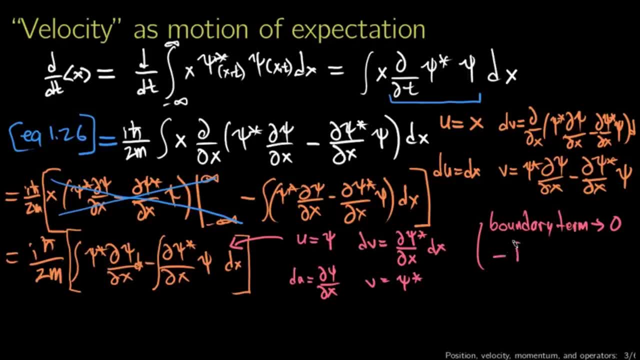 end up with a plus sign there, so we get a minus from the integral part. what that means, though, is that i have psi star and partial psi, partial x. in my integration by parts, i end up with partial psi, partial x and psi star. it's the same. 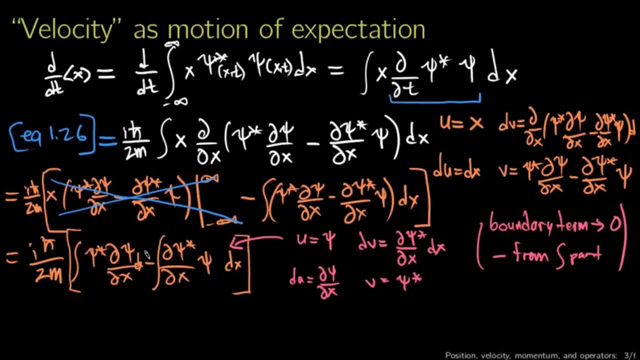 and the fact that i had a minus and another minus means i get a plus, so i have two identical terms here. the result of this, then, is i h bar over m. i'm adding a half and a half and getting one. basically times the integral of psi star partial psi. 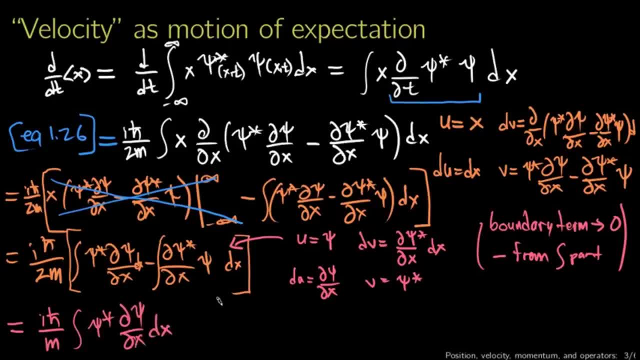 partial x, dx, and this is going to be something that i'm going to call now the expectation of the velocity vector, velocity operator. this is the sort of thing that you get out of operators in quantum mechanics. you end up with expressions like this and this i'm sort of equating. 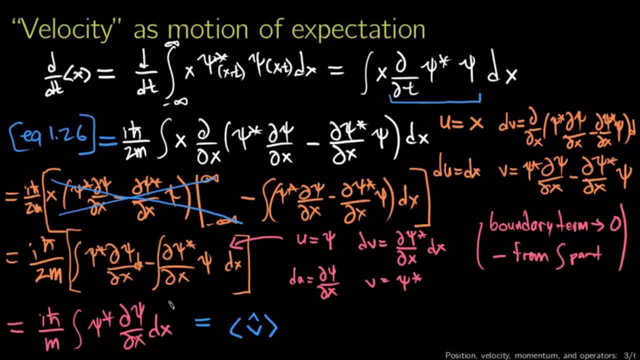 just by analogy with the expectation of a velocity operator. this is not really a probability distribution anymore, at least not obviously. we started with the probability distribution due to psi, the absolute magnitude of psi squared, and we end up with the partial derivative on one of the psi's. 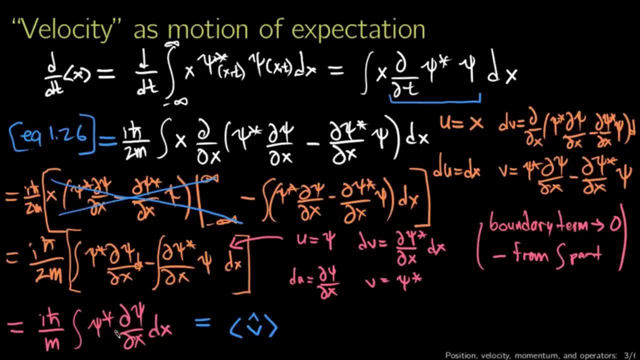 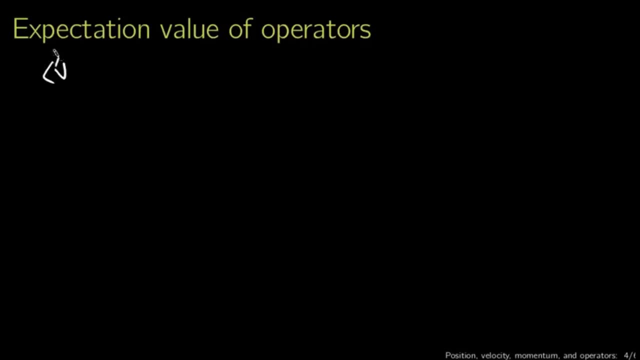 so it's not obvious that this is a probability distribution anymore. and well, it's the probability distribution in velocity and it's giving you the expected velocity in some sense in a quantum mechanical sense. so this is really a more general sort of thing. we have the velocity operator. 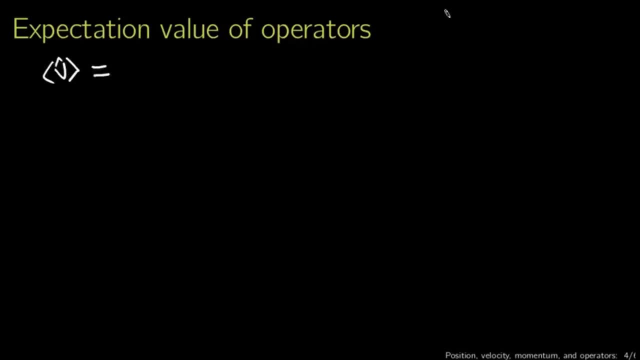 the expectation of the velocity operator. operator wise. i will try to put hats on things i will probably forget. i don't have that much attention to detail when i'm making lectures like this. the hat notation means operator. if you see something that you really as an operator but it doesn't have a hat, that's probably. 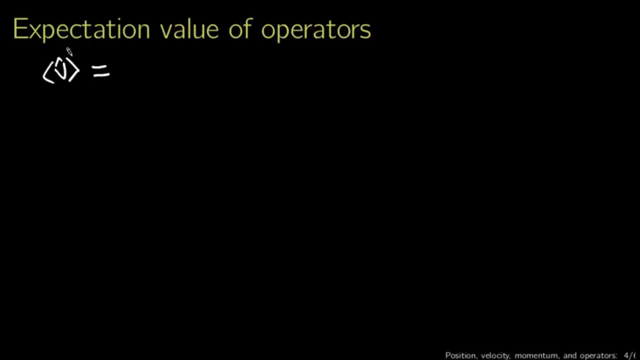 just because i made a mistake, but this expression for the expectation of the velocity operator is the one we just derived, minus i h, bar over m times the integral of psi star partial derivative of psi with respect to x. now it's customary to talk about momentum instead of velocity. 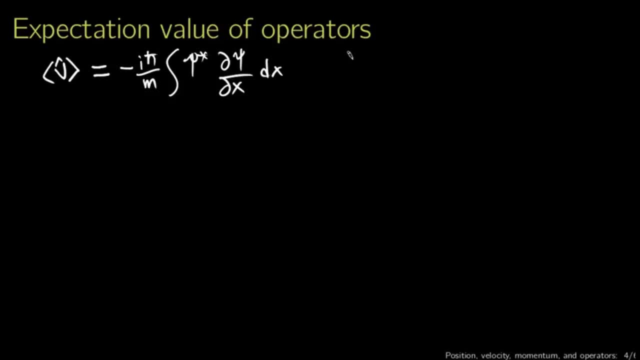 momentum has more meaning because it's a conserved quantity under most physics. so we can talk about the momentum operator, the expectation of the momentum operator, and i'm going to write this momentum operator expression in a slightly more suggestive way. the integral of psi star times something in parentheses. 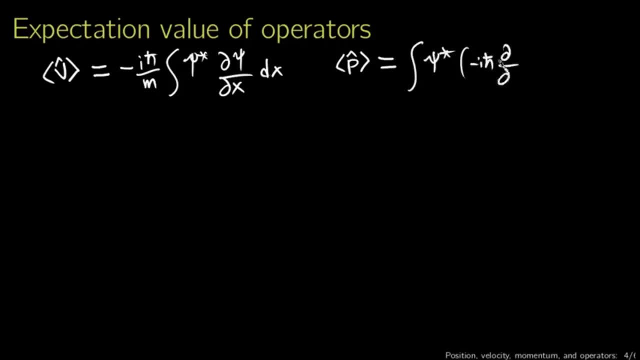 here, which is minus i h, bar partial derivative with respect to x, and i'm going to close the parentheses there- put a psi after it and a dx for the integral. you have the same sort of expression for the position operator. we were just writing that as the expected value of position. 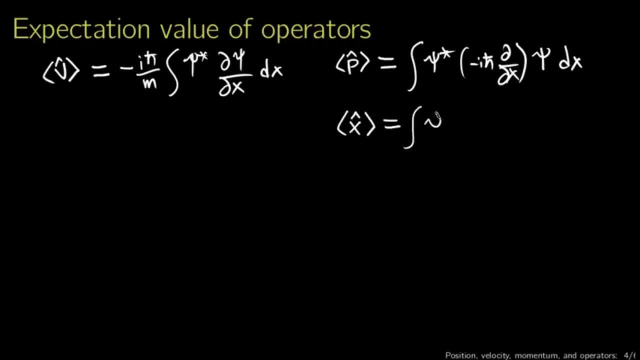 without the hat earlier. but that's going to be the integral of psi star. what goes in the parentheses now is just x, psi dx. so this recognizes the expectation of the variable x subject to the probability distribution given by psi star times psi. this is slightly more subtle. 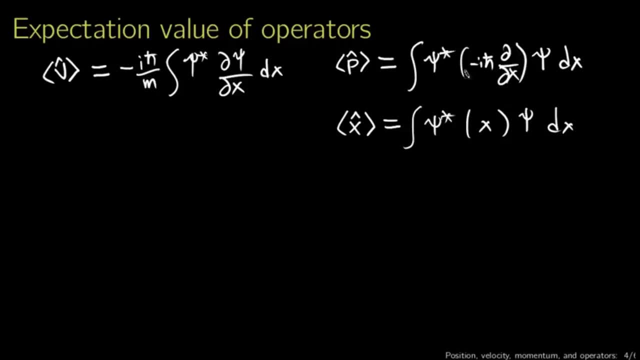 you have psi star and psi, which looks like a probability distribution, but what you have in the parentheses now is very obviously an operator that does something. it does more than just multiply by x. it multiplies by minus i, h, bar and takes the derivative of psi operators in general. 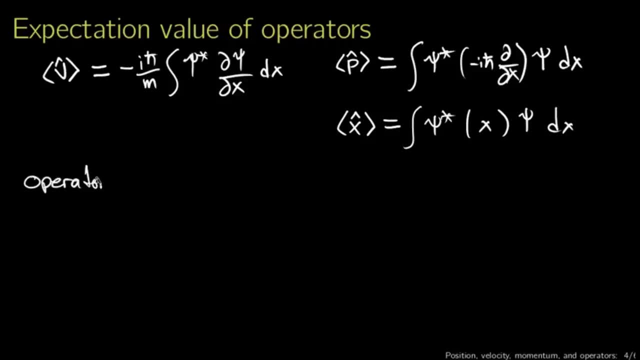 do that. we can write them as, say: x hat equals x times, where there's very obviously something that has to go after the x in order for it to be considered an operator. or we can say the same for v hat: it's minus. i h bar over m times. 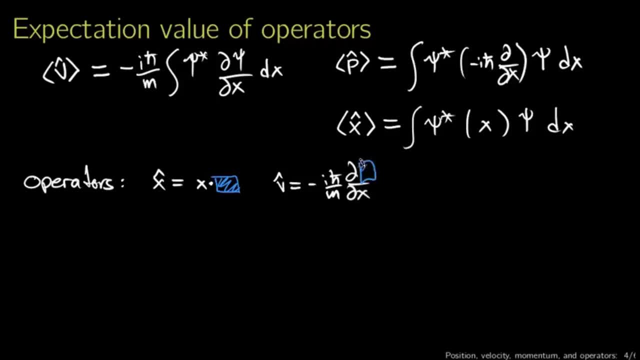 the partial derivative with respect to x, where there obviously has to be something that goes here. likewise for momentum minus i, h, bar partial derivative with respect to x. something has to go there. another example of an operator is the kinetic energy operator, and that's minus h, bar, squared over 2m. 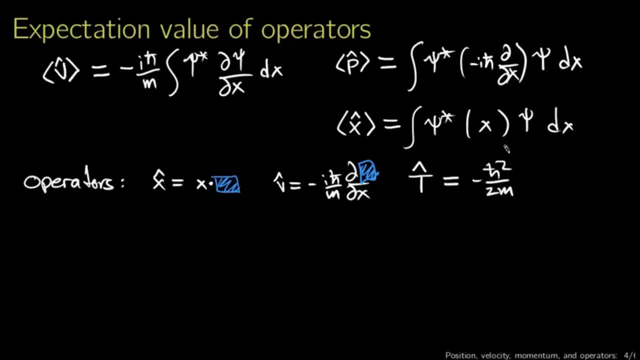 you can think of it as the momentum operator squared. it's got a second derivative with respect to x, and again there very obviously has to be something that goes there. the operator acts on the wave function. that's what I said back when I talked about the fundamental concepts. 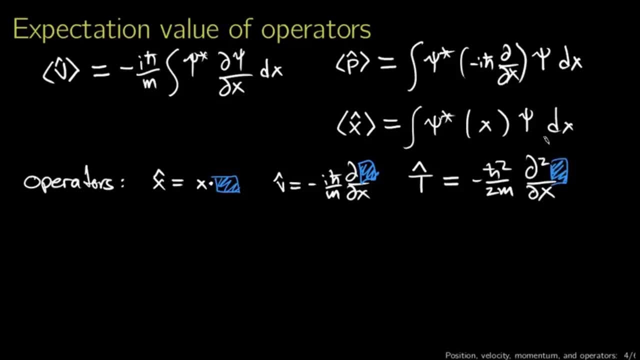 of quantum mechanics, and this is what it means for the operator to act on the wave function. the operator itself is not meaningful. it's only meaningful in the context, when it's acting on a wave function in general, wrong color, in general, the expectation value of some operator. 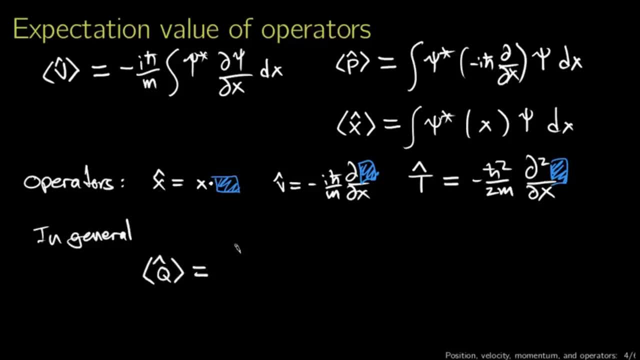 which I'll just call q, is going to be the integral of psi, star q, psi dx, where q acts on the psi and this is what allows us to say: predict the expected value of really any physical quantity. you need to know how to write that physical quantity. 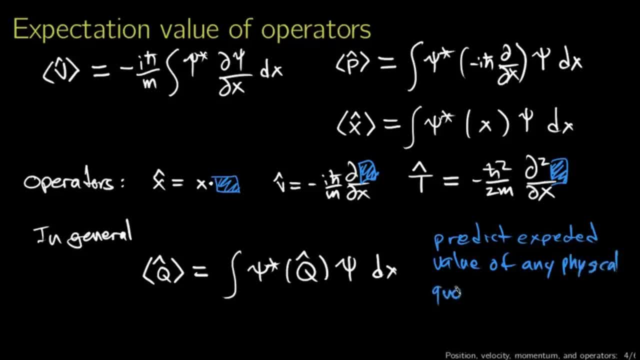 in terms of operators and typically this q hat- here will be written, as you know, something with x hat, the position operator and the value of psi, star q and p hat, the momentum operator. so the operators can in principle be quite complicated, but they're generally expressed in terms of simpler operators. 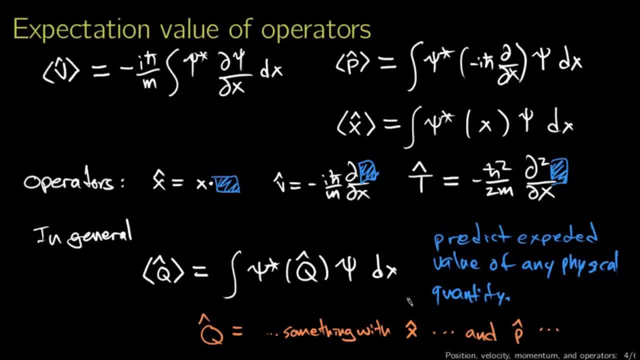 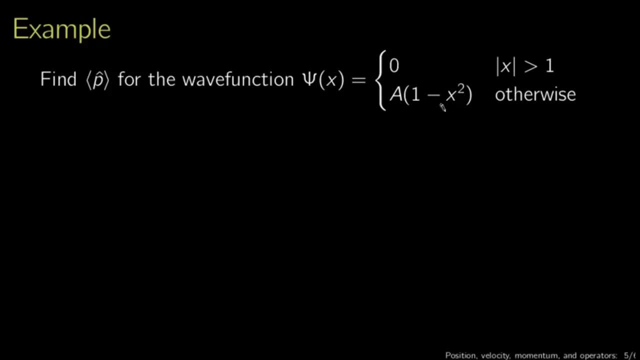 like position and momentum. to give an example of how this is actually used, suppose I want to find the expected value of the momentum for the wave function given by psi. psi here is that wave function that I talked about back in the normalization example, where I found what the value. 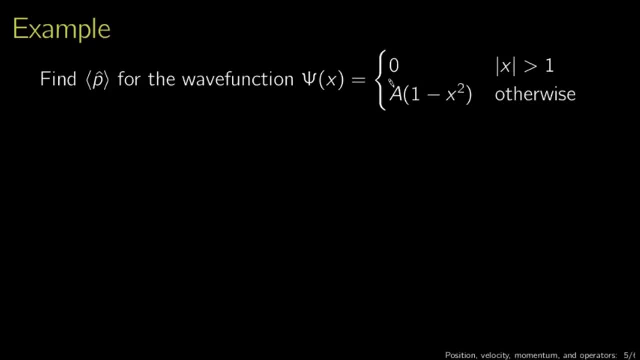 of a was to normalize this wave function properly. I'm just going to leave it as a for now and deal with the wave function part. it's also important to note that this wave function has no time dependence and it has no complex part, so I'm simplifying things a lot. 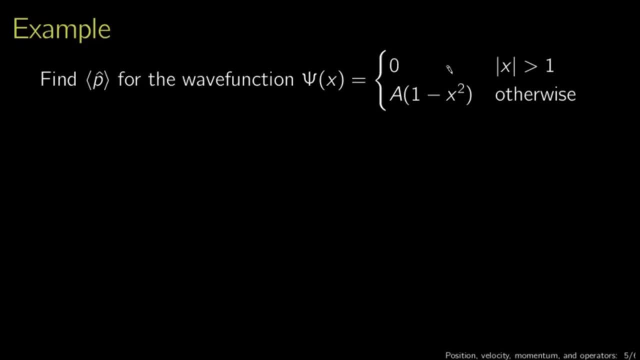 you will work with wave functions that look a lot like this under specific conditions, but know that this isn't a general wave function. this isn't a solution to any particular Schrodinger equation. this is just something that I'm cooking up as an example. it is a valid wave function. 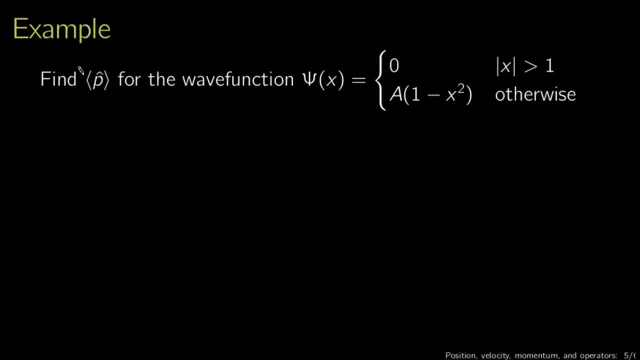 at least if you consider it at say, t equals zero. the goal is to find p hat expected value and the expected value of something you know, expected value of p? hat is given by the integral of psi star, p hat, psi dx, which is the integral, and this integral will be from minus infinity to infinity. 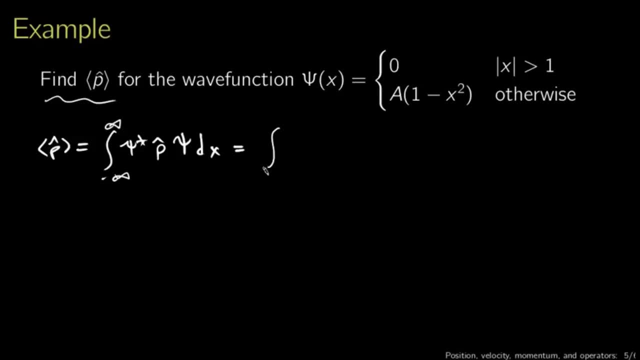 but since my wave function is zero for absolute value of x greater than one, I'm going to drop the condition here and make my integral only go from minus one to one. and for psi star I have a complex conjugate of a- assuming it's real- one minus x squared. 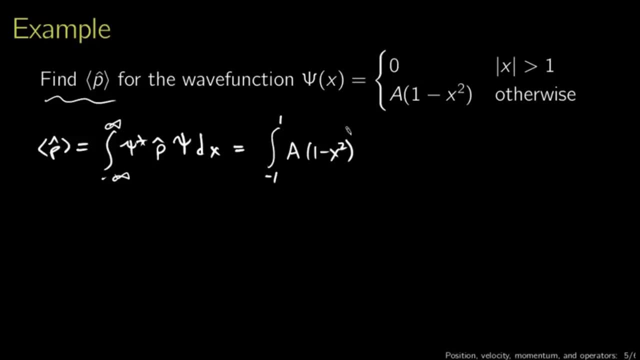 complex conjugate of one minus x. squared x is real. no complex conjugate, or complex conjugate has no effect here. times the momentum operator, which is going to be i h bar minus i h, bar, partial derivative with respect to x of psi, without the complex conjugate. 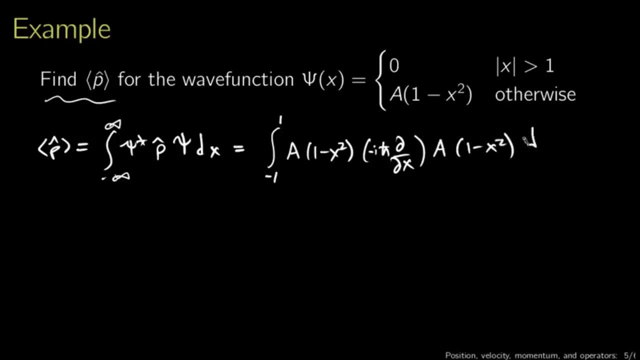 a one minus x squared, all integrated dx. now I can simplify this a little bit. you end up with the integral from minus one to one. oops, sorry, let me pull my i h bar out front minus i h bar integral from minus one to one of. I can pull out the a squared as well. 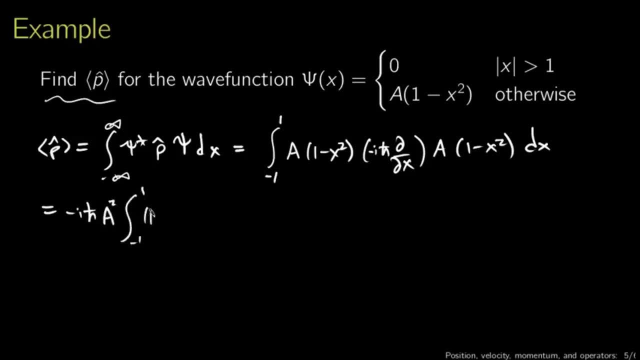 integral from minus one to one, of one minus x squared times the second. sorry, the derivative now of one minus x squared. well, the derivative of one. so I can push the derivative in. so the derivative of one is zero and the derivative of minus x squared is minus two x. 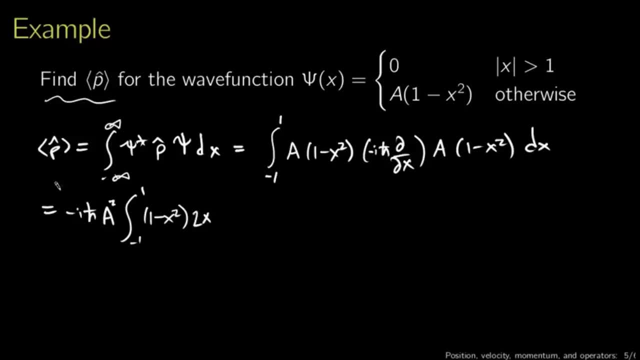 so I'm going to have a minus two x here and just write two x, and I'll put a plus sign out front to compensate for the minus sign, and this is integrated dx. this then is i h bar, let's say two i h bar. I can pull the two out as well. 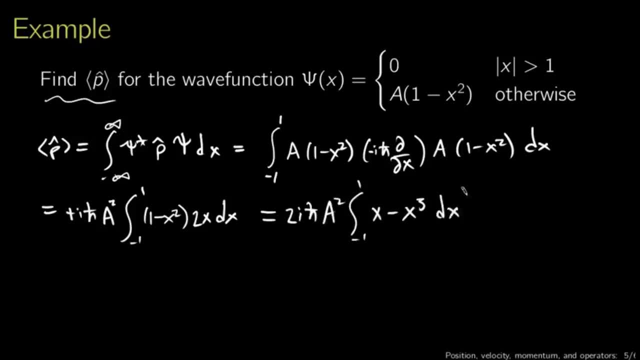 a squared integral from minus one to one of x minus x cubed dx. now, right away, hopefully you can look at this and say x minus x cubed. this is an odd function, meaning if I actually plotted this it would look something like this: this is my coordinate system. 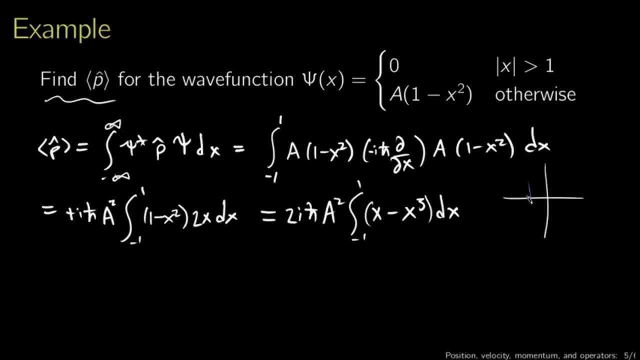 x minus x- cubed, it's going to look something like this: where f of x equals minus f of minus x. what that means is when I integrate this from minus one to one over an interval that starts equally far into the negative side as it goes into the positive side. 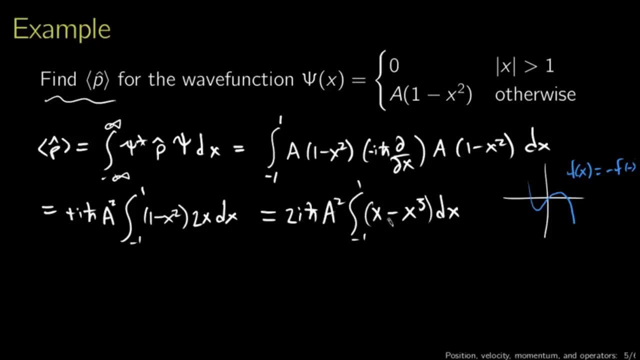 I'm going to get zero, so you can just write down, just by looking at this, that the integral is going to be zero. you can also, of course, plug this in: you'll get x squared over two and x to the fourth over four for these integrals. 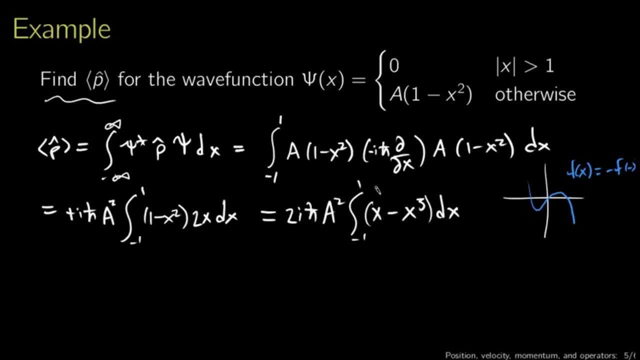 and then you'll plug in minus one and one and find out that minus and plus doesn't make any difference for x squared and x to the fourth, and you'll end up with zero that way as well. but the bottom line here is that the integral of the momentum 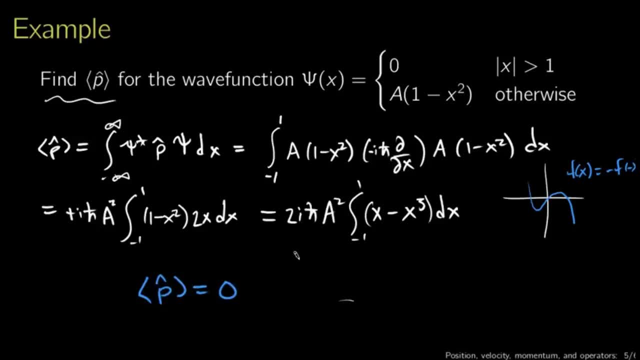 is equal to zero and this makes sense. the reason this makes sense is that my wave function is symmetric. if that's a coordinate system, we can say: this is the x axis. if this is going to be my wave function could look. don't want the ruler. my wave function would look something like this: 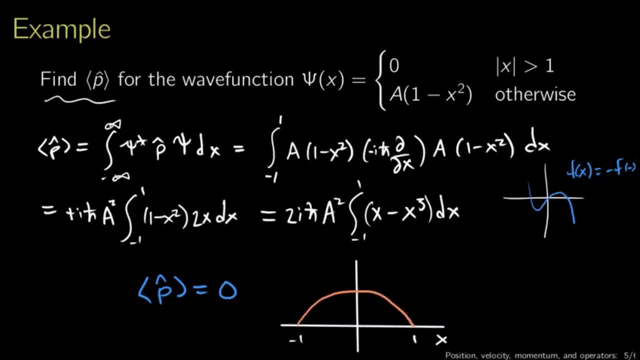 where it goes from minus one to one outside of that range. now if you had an expected value of momentum that was non-zero here, that would suggest the wave function was, on average, moving. and if you look at this wave function it doesn't really seem to be moving. 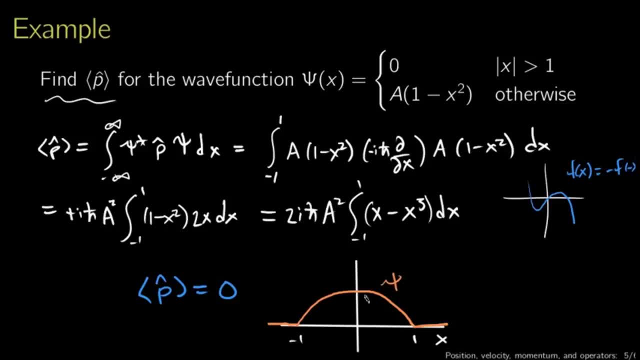 there's no preferred direction to this. if you showed me this and asked: is it moving to the left or to the right, I wouldn't be able to tell you, and it makes sense then- that the expected value of the momentum is zero. the wave function is effectively not moving. 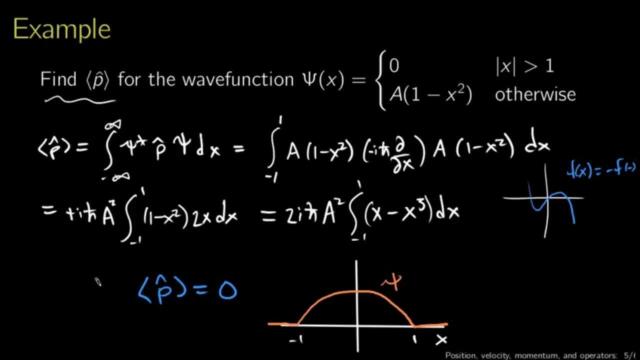 the particle represented by this wave function has no momentum on average. now, this doesn't mean that if you measure the momentum of the particle as described by this wave function, you would always get zero. it just means you would get zero on average. so that's a little bit about operators. 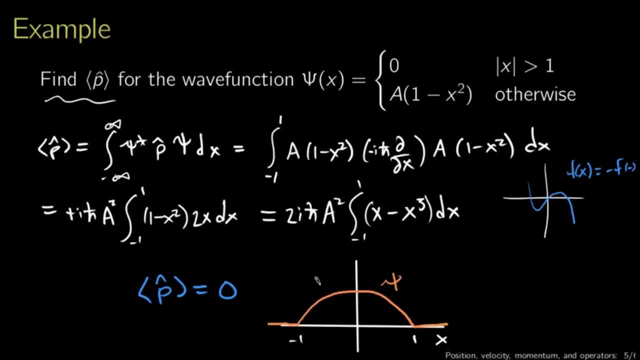 and we'll be working with operators much more in the future. the basic concepts that I want you guys to take away from this lecture is that the expected value of some general operator is what you get if you take psi, star and psi and sandwich your operator in between them. 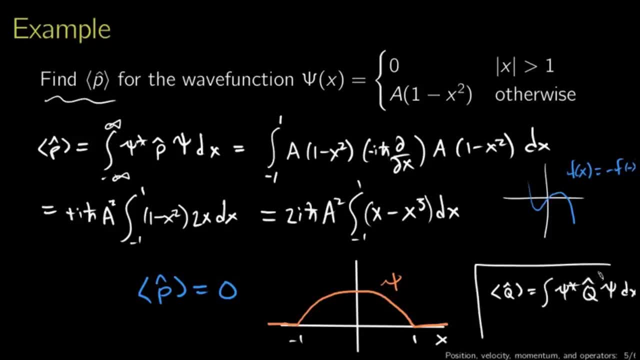 and integrate and then know that the operator may actually do something to psi. it's not just a multiplication. so I cannot say that this q hat is equal to the integral of q hat, psi, star, psi, dx. I can't just move the q around, I'm not allowed to do that. 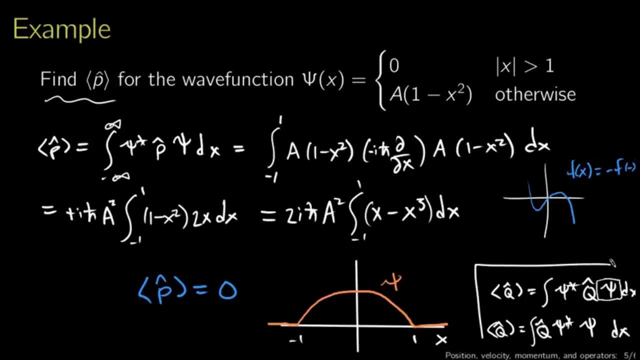 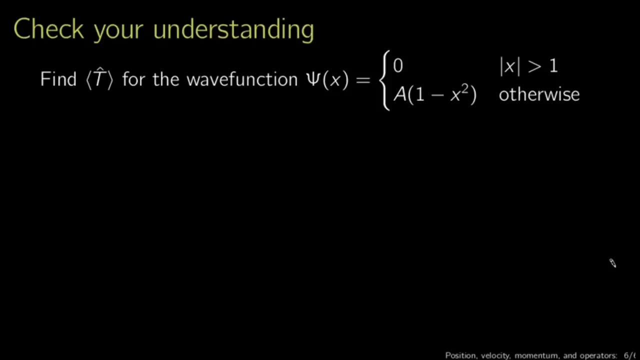 because q is acting on this psi. really, this is just reasoning by analogy. right now there is no rigorous formal proof. we'll come back to discuss the math of quantum mechanics quite a lot later on, but that's it for this lecture. as a check your understanding, I'd like you to find 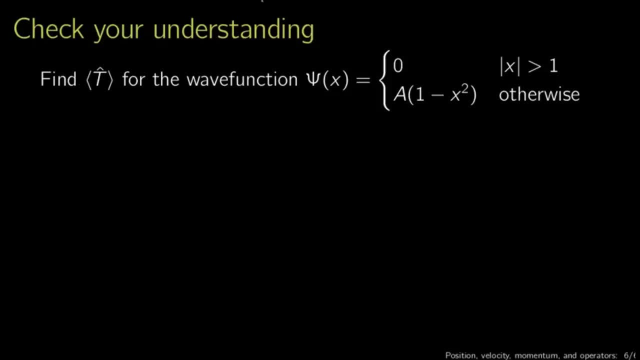 the expected value of the kinetic energy operator for this wave function. remember that the kinetic energy operator t hat is equal to minus h bar squared over 2m times the second derivative with respect to x, and I almost wrote a psi there. but I'm not supposed to write a psi. 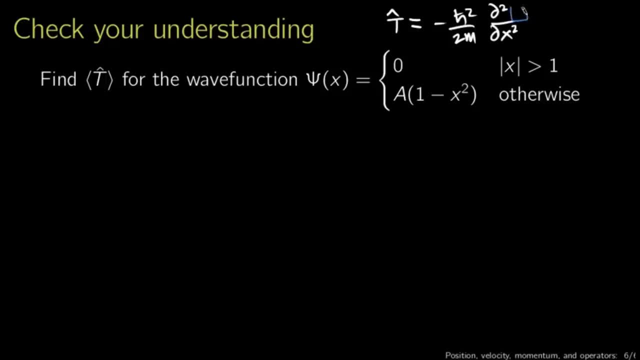 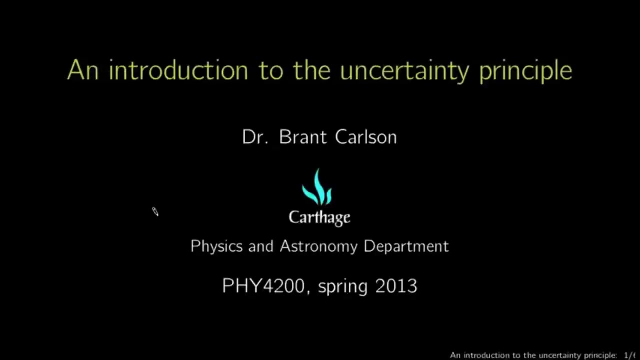 the operator has to act on psi, so there should be some space here for psi to go. so go back to that same formula for the expectation. use the kinetic energy operator instead and calculate the expected value of the kinetic energy for this wave function. as an introduction to the 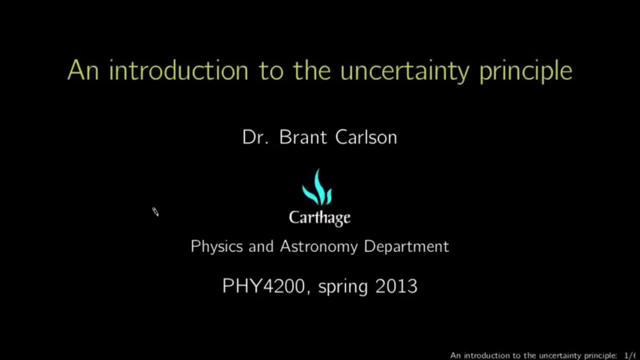 uncertainty principle. we're going to talk about waves and how waves are related to each other. we'll get into a little bit of the context of Fourier analysis, which is something we'll come back to later, but the overall context of this lecture is the uncertainty principle, and the uncertainty principle is one of the key. 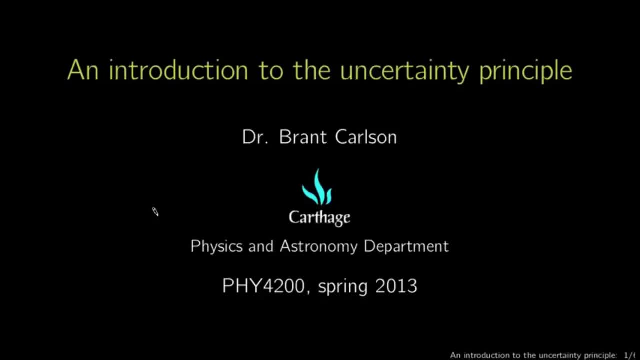 results from quantum mechanics and it's related to what we discussed earlier in the context of the boundary between classical physics and quantum physics. quantum mechanics has these inherent uncertainties that are built into the equations, built into the state, built into the nature of reality, that we really can't surmount. 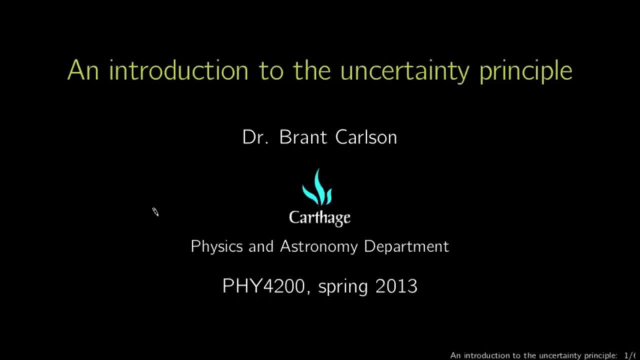 and the uncertainty principle is the mathematical description. it's those relationships that I gave you earlier. delta p, delta x is greater than about equal to h-bar over 2. I think I just said greater than about equal to h-bar earlier. we'll do things a little more mathematically here. 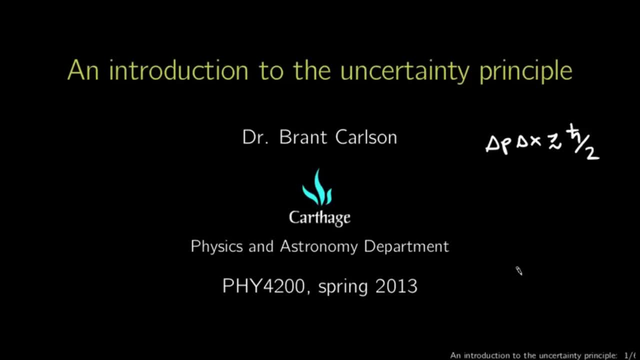 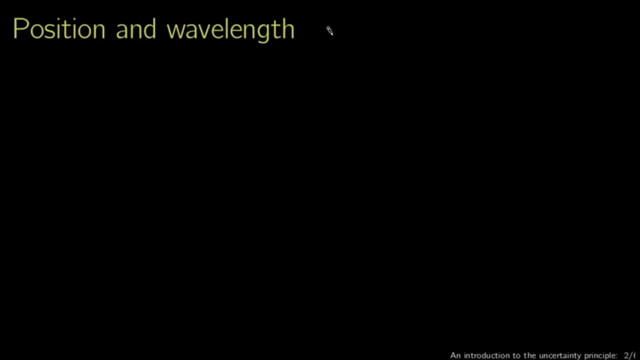 and it turns out there's a factor of 2 there. to start off, though, conceptually think about position and wavelength, and this really is now in the context of a wave. so, say, I had a coordinate system here, something like this, and if I had some wave? 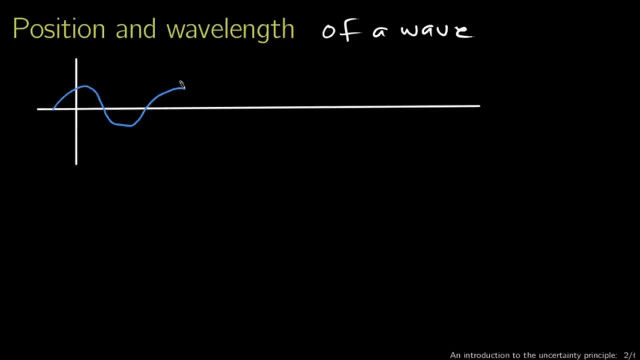 with a very specific wavelength. you can just think about it as a sinusoid. if I asked you to measure the wavelength of this wave, you could take a ruler and you could plop it down there and say: okay, well, how many inches are there from peak to peak? 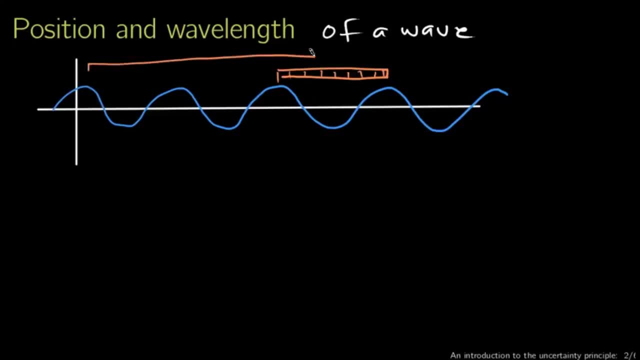 or from zero crossing to zero crossing. out of the two, you could get a tape measure and measure many wavelengths: one, two, three, four wavelengths. in this case, that would allow you to very accurately determine what the wavelength was. if, on the other hand, the wave 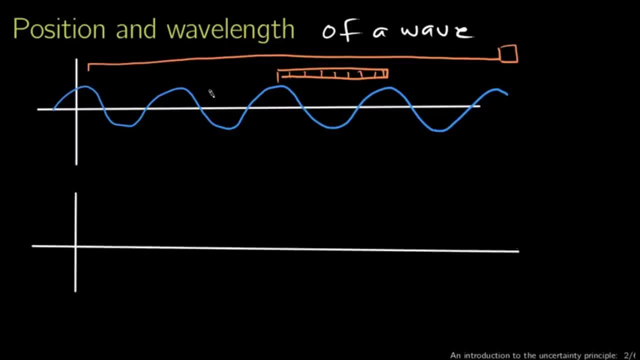 looked more like this. give you another coordinate system here. the wave looked something like this. you wouldn't be able to measure the wavelength very accurately. you could, as usual, put your ruler down on top of the wave, for instance, and count up the number of inches or centimeters. 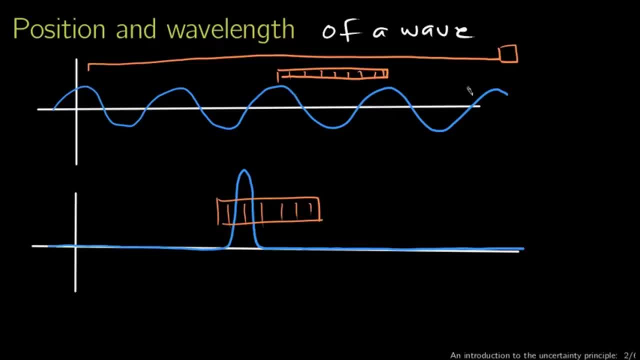 from one side to the other. but that's just one wavelength. it's not nearly as accurate as, say, measuring four wavelengths or ten wavelengths or a hundred wavelengths. you can think of some limiting cases. suppose you had a wave with many, many, many, many, many oscillations. it looks like I'm crossing out the wave. 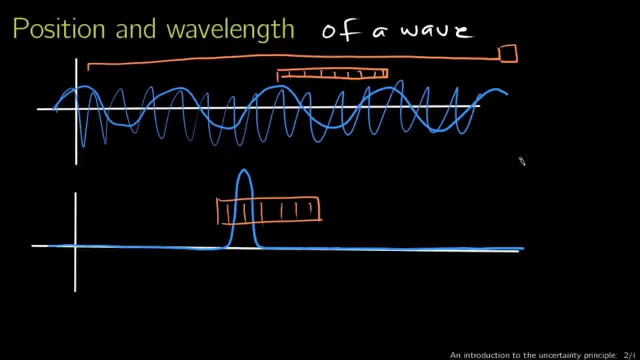 underneath there. so I'm going to erase this in a moment. if you had many wavelengths and you could measure the total length of many wavelengths, you would have a very precise measurement of the wavelength of the wave. the opposite is the case here. you only have one wavelength. 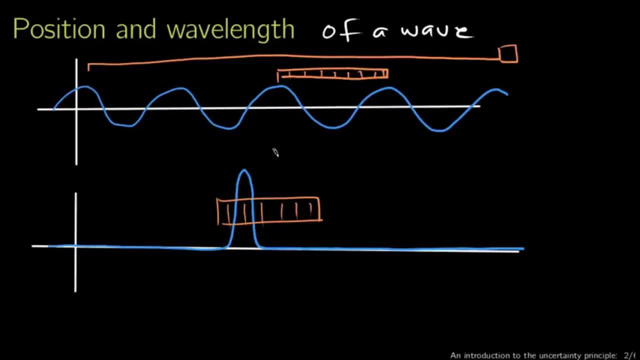 you can't really measure the wavelength very accurately. what you can do, however, is measure the position very accurately. here I can say pretty certainly the wave is there plus or minus a very short spread in position. the other hand, here I cannot measure the position of this wave. 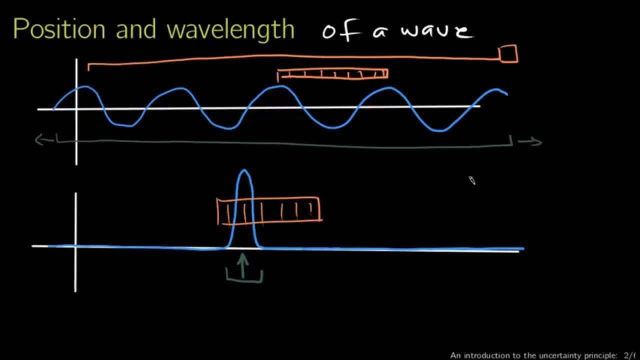 if this thing continues, I can't really say where the wave is. it's not really a sensical question to ask: where is this wave? this wave is everywhere. these are the sorts of built in uncertainties that you get out of quantum mechanics: where is the wave? the wave is everywhere. 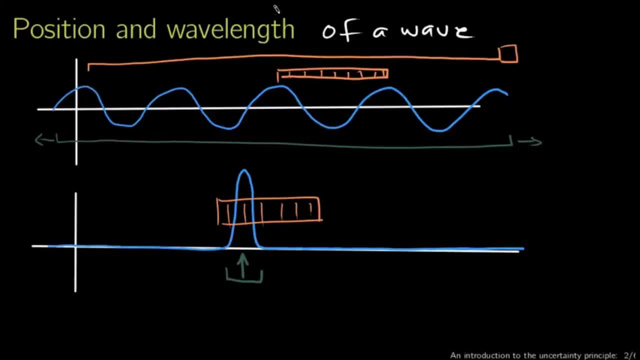 it's a wave, it doesn't have a local position. it turns out, if you get into the mathematics of Fourier analysis, that there is a relationship between the spread of wavelengths and the spread of positions. if you have a series of waves of all different wavelengths and they are added up, 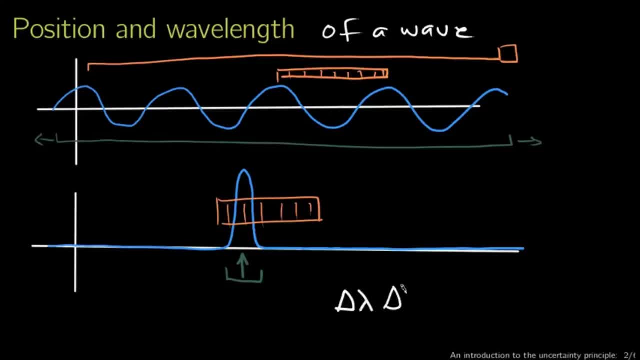 the spread in the wavelength is related to the spread in positions of the sum, and we'll talk more about Fourier analysis later, but for now just realize that this product is always going to be greater than or equal to about one wavelength is something with units of inverse length. 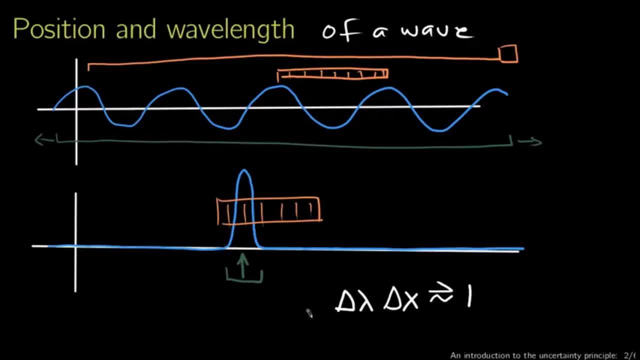 and the position, of course, is something with units of length. so the dimensions of this equation are sort of a guideline. wavelength and position have this sort of relationship, and this comes from Fourier analysis. so how do these waves come into quantum mechanics? well, waves in quantum mechanics really first got their start with. 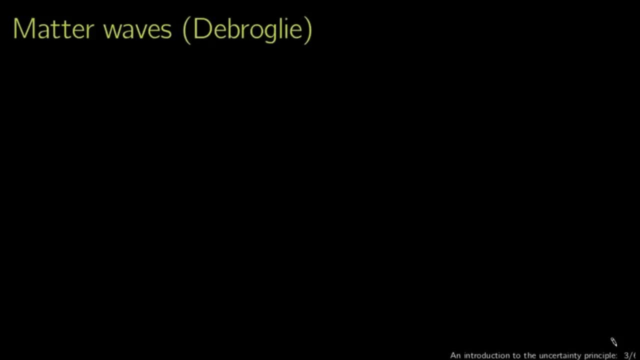 Louis de Broglie. I always thought his name was pronounced de Broglie, but well, he's French so there's all sorts of weird pronunciations in French. de Broglie is my best guess at how it would probably be pronounced. de Broglie proposed. 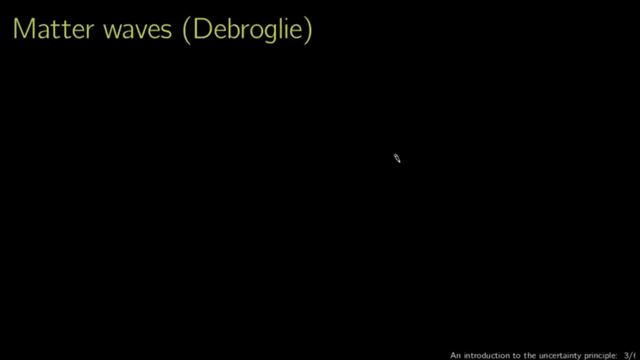 that matter, could travel in waves as well, and he did this, with an interesting argument, on the basis of three fundamental equations that had just recently been discovered when he was doing his analysis. this was in his PhD thesis, by the way. E equals MC squared. you all know that equation. 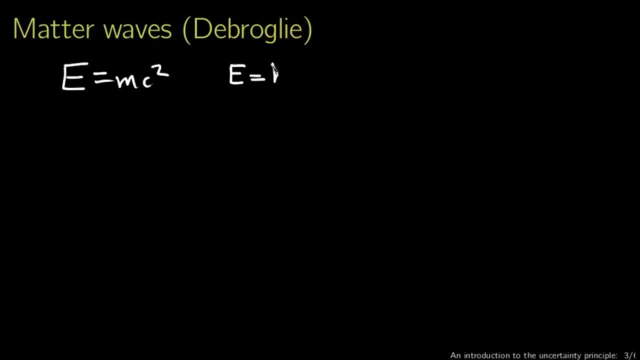 you all hopefully also know this equation: E equals HF constant times. the frequency of a beam of light is the energy associated with a quanta of light. this was another one of Einstein's contributions and it has to do with his explanation of the photoelectric effect. the final equation: 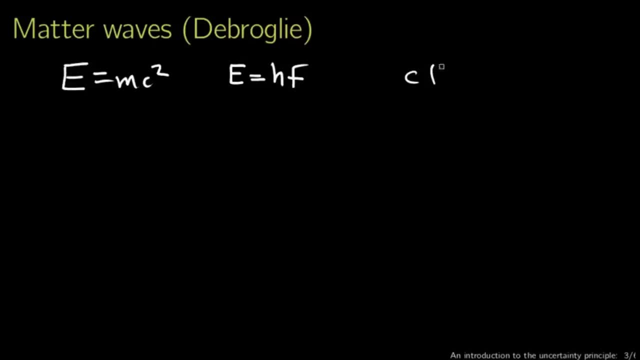 that de Broglie was working with was C equals F lambda. the speed of light is equal to the frequency of the light times, the wavelength of the light, and this is really not true just for light. this is true for any wave phenomenon where the frequency and the wavelength are related. 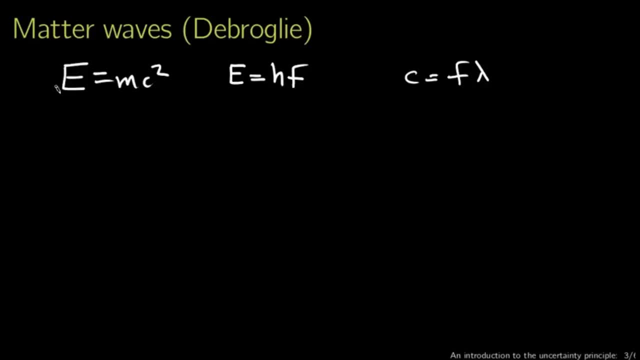 now, if these expressions are both equal to waves or are both equal to energy, then I ought to be able to say: MC squared equals HF, and this expression tells me something about F. it tells me that F equals C over lambda, so I can substitute this expression in here. 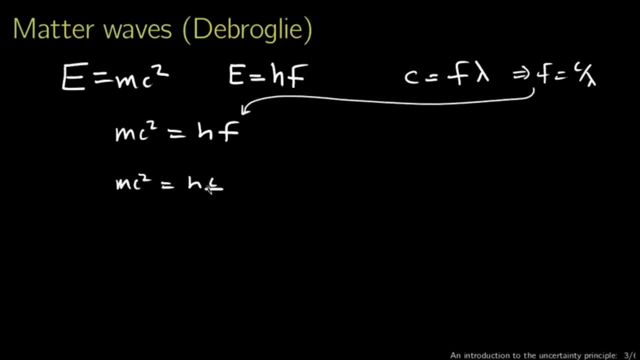 and get MC squared: equals H over lambda. now I can cancel out one of the C's and I'm left with MC: equals H over lambda. now what de Broglie said was this: this is like momentum, so I'm going to write this equation as: P equals H over lambda. 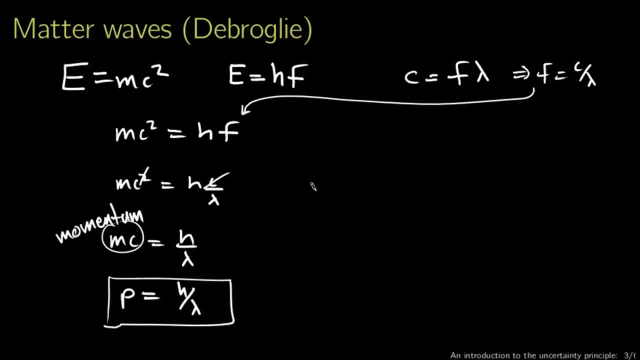 and then I'm going to wave my hands extraordinarily vigorously and say: while this equation is only true for light and this equation is only true for waves, this is also true for matter. how actually this happened in the context of quantum mechanics, in the early historical development of quantum mechanics. 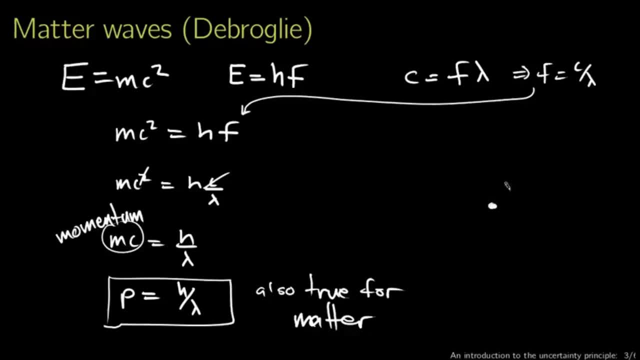 is de Broglie noticed that the spectrum of the hydrogen atom, this bright line spectra that we were talking about, where a hydrogen atom emits light of only very specific wavelengths- intensity as a function of wavelength looks something like this: but that could be explained if he assumed that the electrons 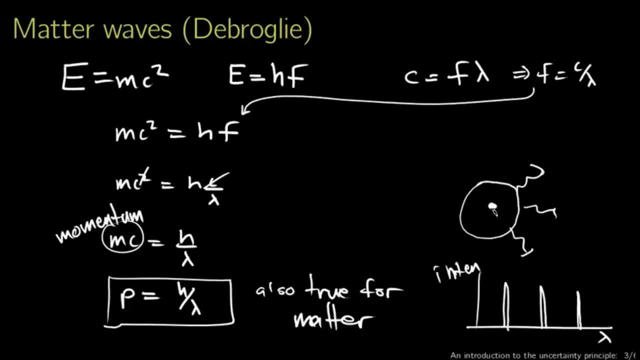 were traveling around the nucleus of the hydrogen atom as waves and that only an integer number of waves would fit. the one that I just drew here didn't end up back where it started, so that wouldn't work. if you had a wavelength that looked something like this: 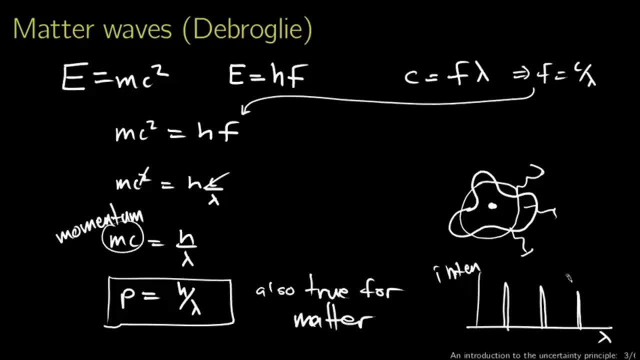 in a circle that would potentially account for these allowed emission energies. that was quite a deep insight, and it was one of the things that really kicked off quantum mechanics at the beginning. the bottom line here, for our purpose, is that we're talking about waves and we're talking about matter: waves. 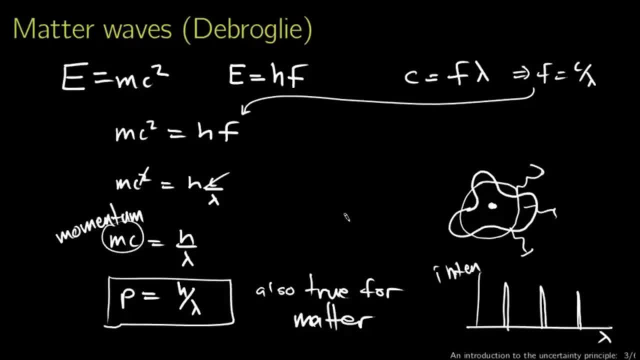 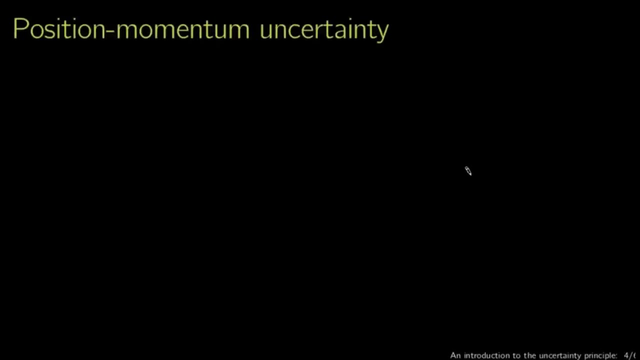 so that uncertainty relation or the relationship between the spreads of wavelengths and the spreads in positions in the context of Fourier analysis will also potentially hold for matter. and that gets us into the position momentum uncertainty relation. the wave momentum relationship we just derived on the last slide was: p equals h over. 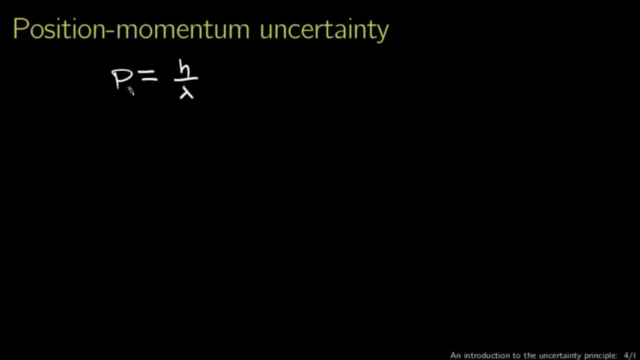 lambda. this tells you that the momentum and the wavelength are related. from two slides ago, when we were talking about waves and whether or not we should say exactly where a wave was, we had a relationship. that was something like delta lambda: the spread in wavelengths times the spread in positions of the wave. 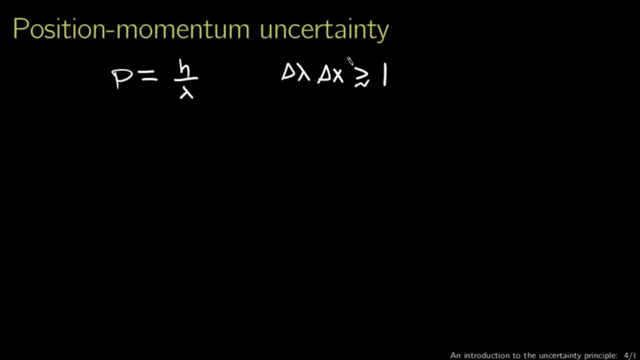 is always greater than about equal to one. combining these relationships together in quantum mechanics- and this is not something that I'm doing rigorously now, I'm just waving my hands- gives you delta p. delta x is always greater than about equal to h bar over two. 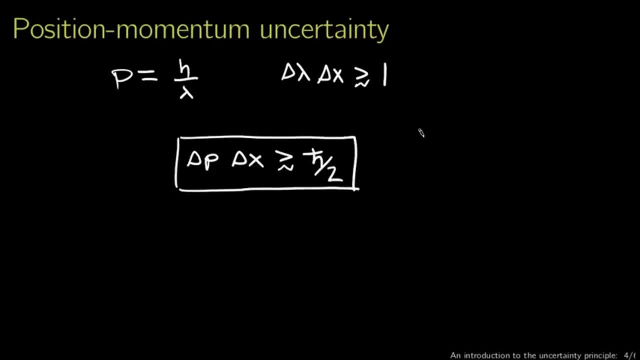 and this is the correct mathematical expression of the Heisenberg uncertainty principle that we'll talk more about and derive more formally in chapter three. but for now just realize that the position of a wave, the position of a particle are uncertain quantities and the uncertainties are related by this. 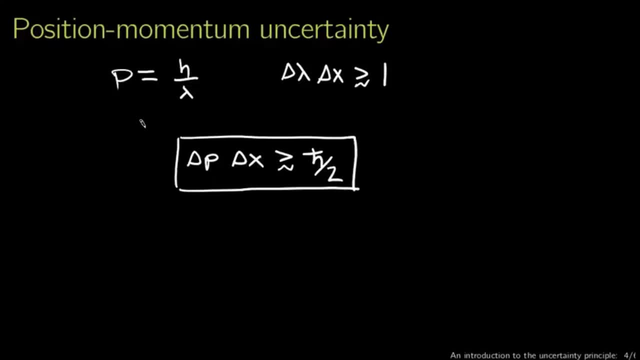 which, in one perspective, results from consideration of adding many waves together in the context of Fourier analysis, which is something we'll talk about later as well, extended through the use of or the interpretation of matter as also a wave phenomenon. to check your understanding, here are 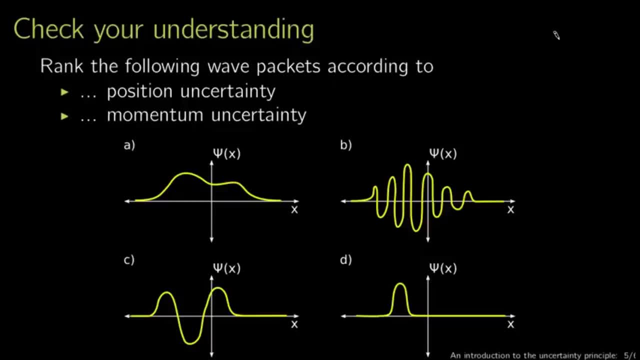 four possible wave packets and I would like you to rank them in two different ways: one according to the uncertainties in their positions and two according to the uncertainties in their momenta. so if you consider, say wave b to have a very certain position, you would rank that one highest. 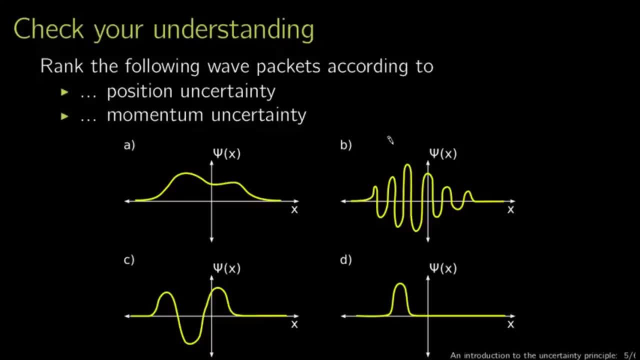 in terms of the certainty of its position. perhaps you think wave b has a very low uncertainty in position. you would put it on the other end of the scale. I'm looking for something like the uncertainty of b is greater than the uncertainty of a is greater than the uncertainty of d. 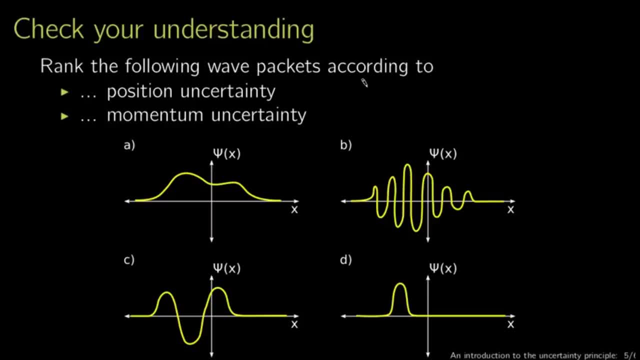 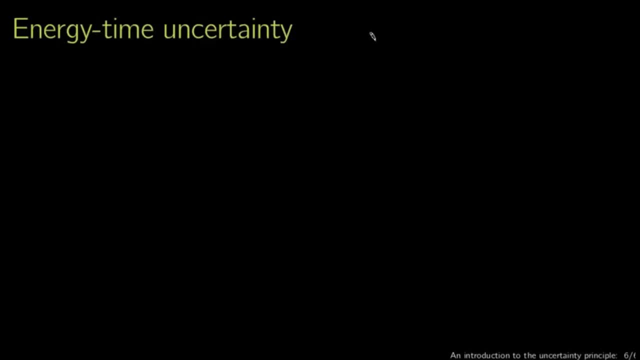 is greater than the uncertainty of c for both position and momentum. the last comment I want to make in this lecture is on energy-time uncertainty. this was the other equation I gave you when I was talking about the boundary between classical physics and quantum physics. we had delta p, delta x, 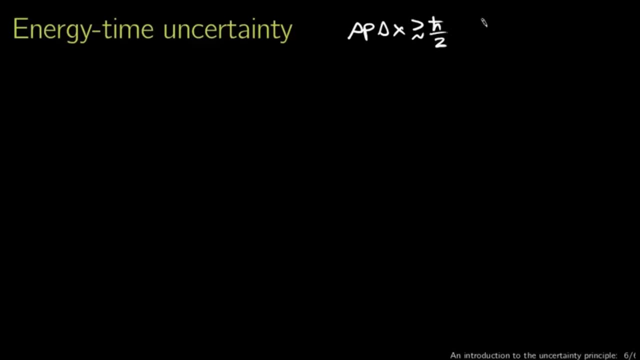 greater than or equal to h-bar over 2, and now we also had- excuse me for a moment here- delta e, delta t greater than or equal to h-bar over 2- same sort of uncertainty relation, except now we're talking about spreads in energy and spreads in time. 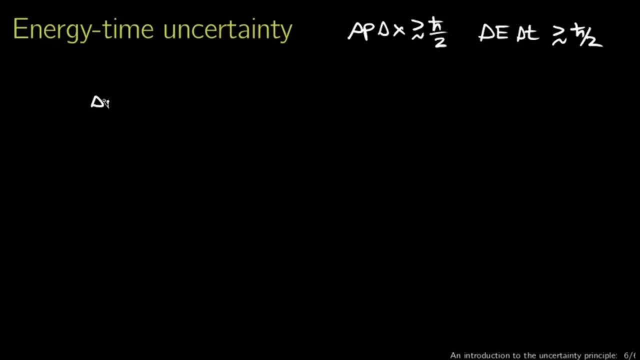 I'd like to make an analogy between these two equations, delta p and delta x. delta p, according to de Broglie, is related to the wavelength, which is sort of a spatial frequency. it's the frequency of the wave in space. delta x, of course, is just 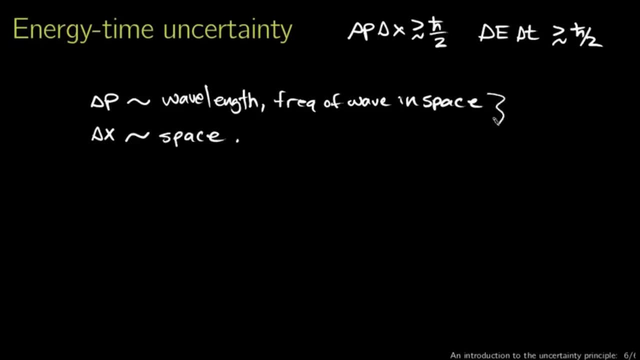 well, I'll just say that's space and these are related according to this equation. in the context of energy and time we have the same sort of thing. well, that's pretty clear. that's time and delta e. well, that then therefore, by analogy here, has to have something to do with. 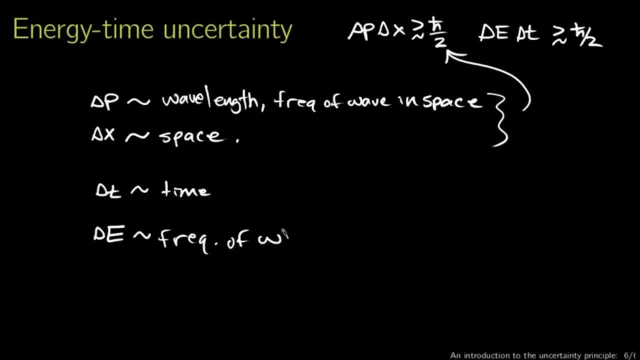 the frequency of the wave now in time, and that's simple. that's just the frequency. the fact that these are also related by an uncertainty principle tells you that there's something about energy and frequency in time, and this is something that we'll talk about in more detail in the next lecture. 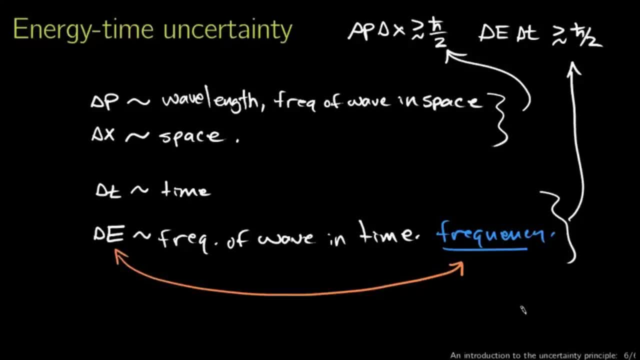 when we start digging into the Schrodinger equation, the time dependent Schrodinger equation, and deriving the time independent Schrodinger equation, which will give us the relationship exactly. but for now, position and momentum, energy and time we're all talking, are both talking about sort of wave. 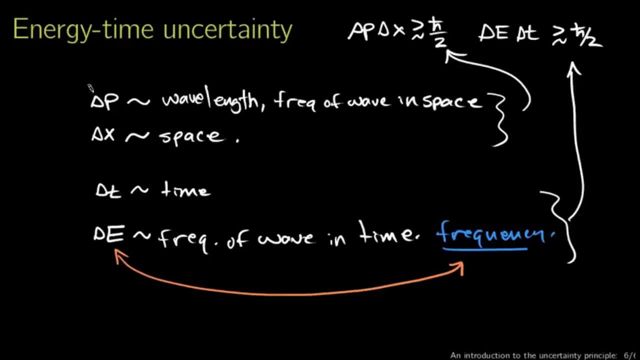 phenomenon, except in the context of position and momentum. you're talking about wavelength, frequency of the wave in space, whereas energy and time. you're talking about the frequency of the wave in time, how quickly it oscillates. that's about all the uncertainty principle, as I've said. 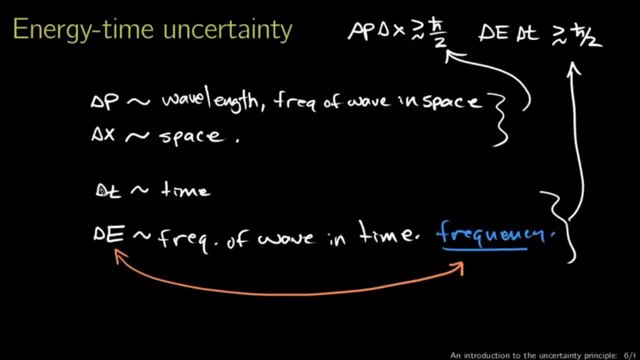 is something that we'll treat in much more detail in chapter 3, but for now, the uncertainty principle is important because you have these equations and these are fundamental properties of the universe. if you want to think of them that way, there's something that we're going to be. 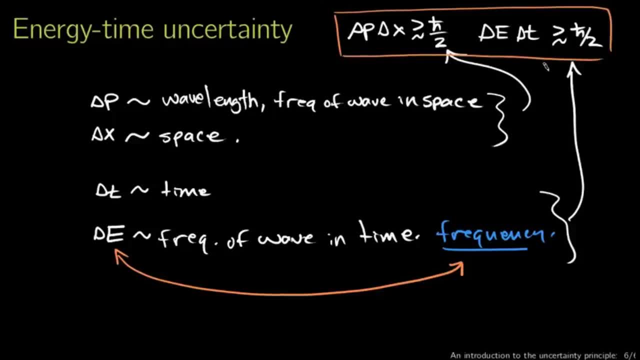 working with as a way of checking the validity of quantum mechanics throughout chapter 2. that's all for now. you just need to conceptually understand how these wavelengths and positions, or frequencies and times, are interrelated. the last few lectures have been all about the wave function. 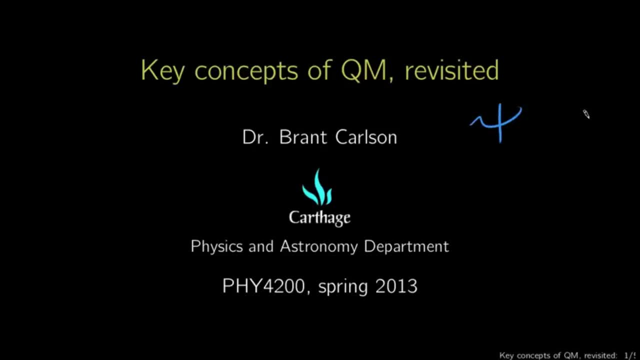 psi, and since psi is such an important concept in quantum mechanics- really the first entire chapter of the textbook is devoted to the wave function and all of its various properties. since we've reached the end of chapter 1 now, now is a good opportunity to go and review. 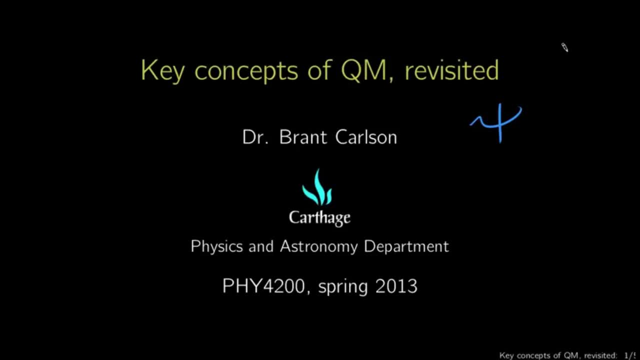 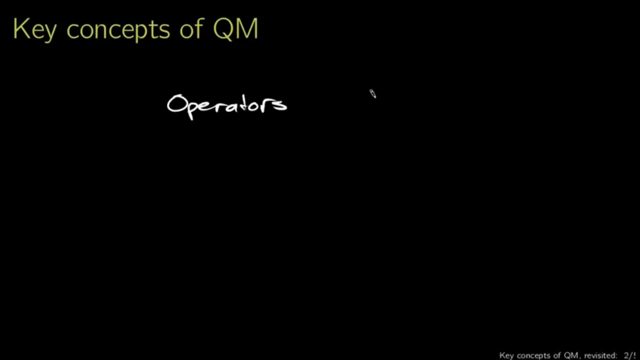 the key concepts of quantum mechanics, in particular the wave function and how it is related to the rest of quantum mechanics. the key concepts, as I stated them earlier, were operators, the Schrodinger equation and the wave function. operators are used in the Schrodinger equation. 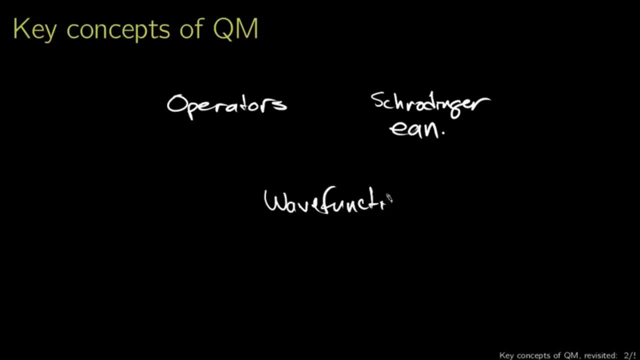 and act on the wave function. your friend and mine, psi. what we haven't really talked about a lot yet is how to determine the wave function, and the wave function is determined as solutions to the Schrodinger equation. that's what chapter 2 is all about. 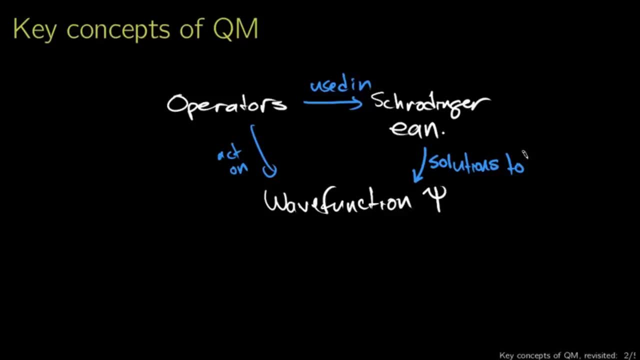 solving the Schrodinger equation. for various circumstances, the key concepts that we've talked about so far- operators and the wave function- conspire together to give you observable quantities, things like position or momentum, or say the kinetic energy of the wave function of a particle. they don't give us these properties. 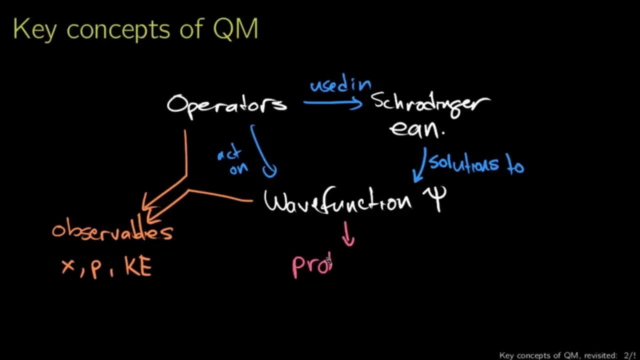 with certainty. in particular, the wave function really only gives us probabilities, and these probabilities don't give us really any certainty about what will happen. uncertainty is one of the key concepts that we have to work with in quantum mechanics, so let's take each of these concepts in turn. 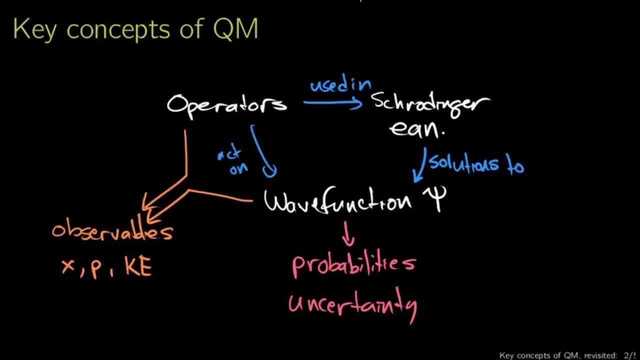 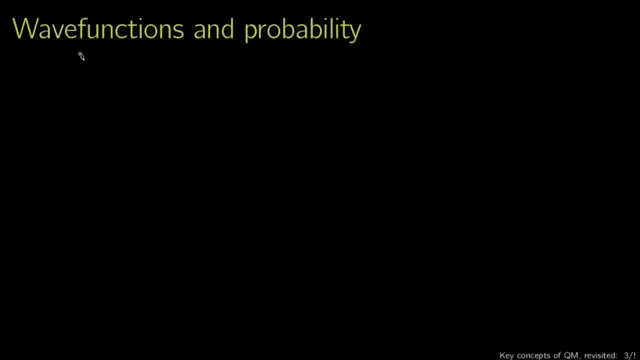 and talk about them in a little more detail. since now we have some actual results, that we can use, some mathematics, we can put more meat on this concept map than just simply the concept map. first, the wave function. the wave function psi does not tell us anything. 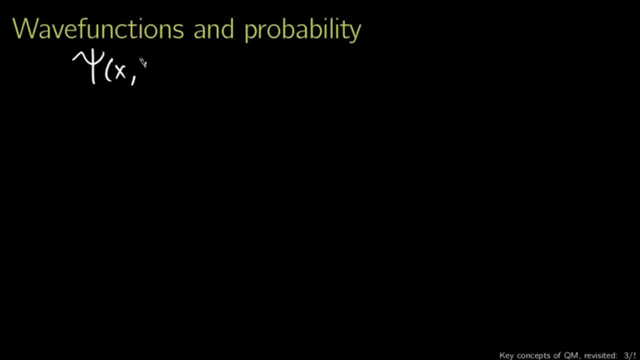 with certainty, and it's a good thing too, because psi as a function of position and time is complex. it's not a real number and it's hard to imagine what it would mean to actually observe a real number, so the wave function is already, on, somewhat suspect. 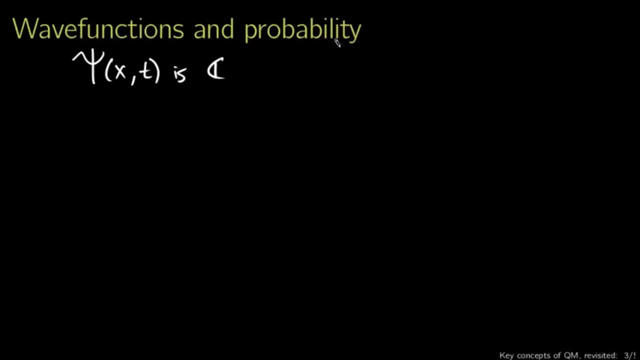 ground here, but it has a meaningful connection to probability distributions. if we more or less define the squared modulus, the absolute magnitude of the wave function, to be equal to a probability distribution, and this is the probability distribution for what? well, it's the probability distribution for outcomes of measurements of position. 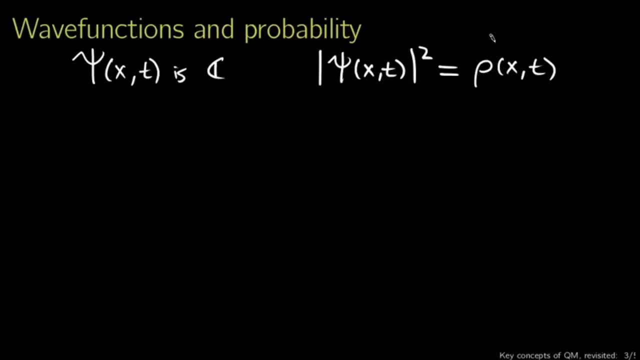 for instance, you can think about this as a probability distribution for where you're likely to find the particle should you go looking for it. this interpretation as a probability distribution requires the wave function to be normalized, namely that if I integrate the squared magnitude of the wave function, 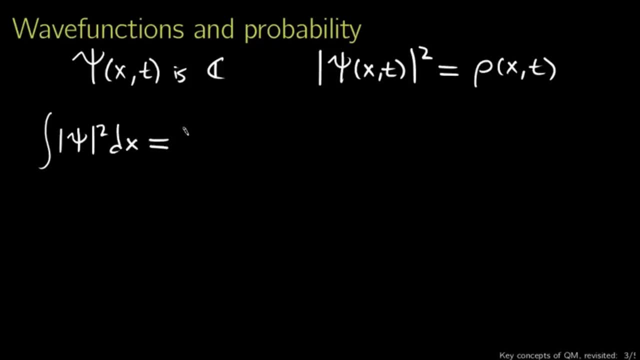 over the entire space that I'm interested in, I have to get one. this means that if I look hard enough for the particle everywhere, I have to find it somewhere. the probability distributions, as I mentioned earlier, don't tell you anything with certainty. in particular, there is a good deal of uncertainty. 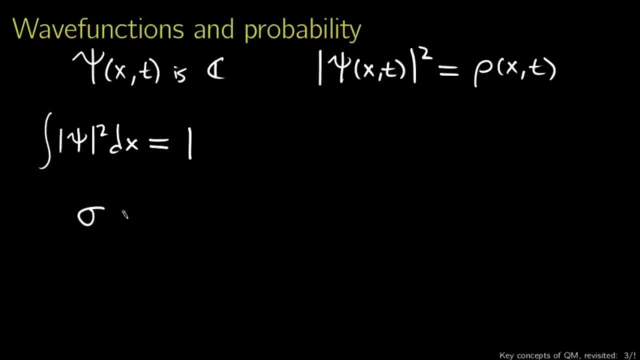 which we express as a standard deviation or a variance. for instance, if I'm interested in the standard deviation of the uncertainty or standard deviation of the position, excuse me, it's most easy to express as the variance which is the square of the standard deviation and the square of this standard deviation. 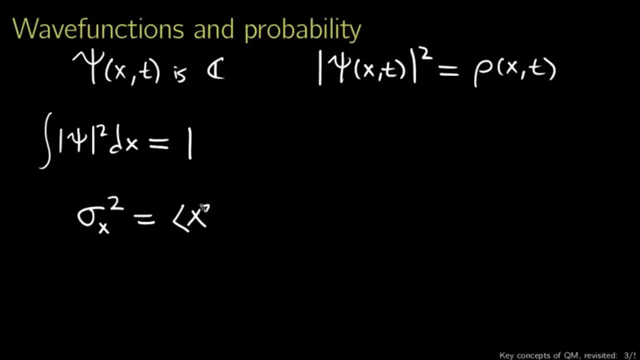 or the variance is equal to the expectation value of the square of the position minus the square of the expectation value of the position, and we'll talk about expectation values in a moment. expectation values are calculated using expressions with operators that look a lot like these sorts of integrals. 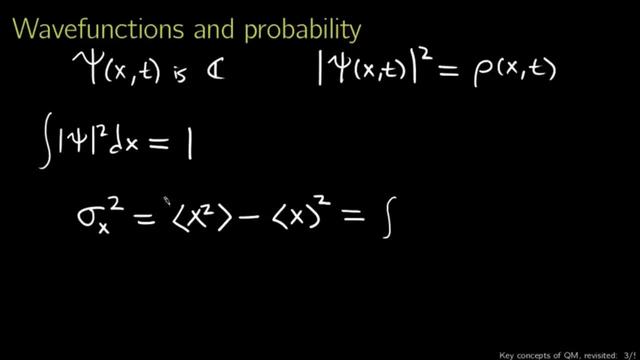 in fact I can re-express this as: the expectation of the square in terms of a probability distribution is just the x squared multiplied by the probability distribution with respect to x integrated over all space. this is the expectation of x squared. I can add to that or subtract from that. sorry. 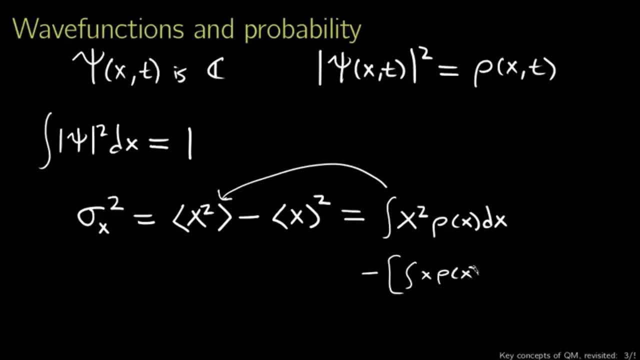 the square of the expectation of x, which has a very similar form, and that gives us our variance. so our wave function, which is complex, gives us probability distributions which can be used to calculate expectation values and uncertainties. so this probabilistic interpretation of quantum mechanics gets us into some trouble. 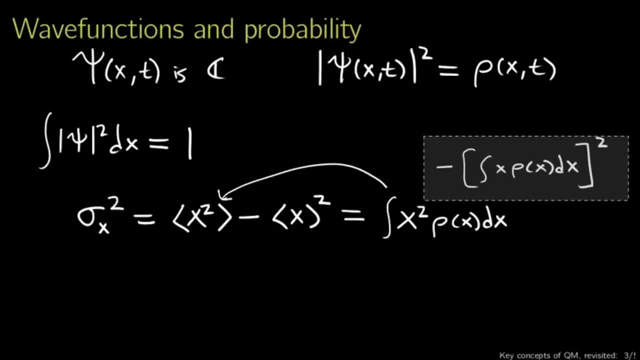 pretty quickly. I'm going to move this up now, give myself some more space, namely with the concept of wave function. collapse now collapse, bothers a lot of people, and it should. this is really a philosophical problem with quantum mechanics that we don't really have a good interpretation. 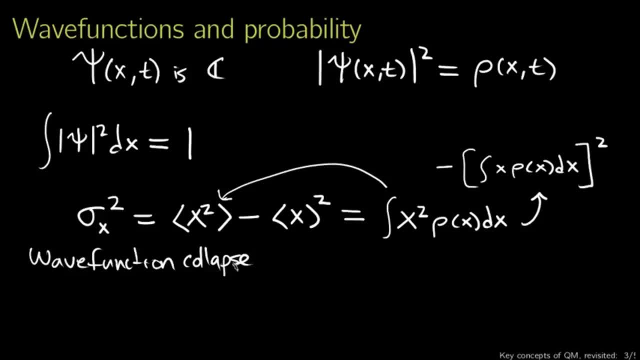 of what quantum mechanics really means for the nature of reality. but the collapse of the wave function is more or less a necessary consequence of the interpretation of the wave function as a probability distribution. if I have some space, some coordinate system, and I plot on this coordinate system, 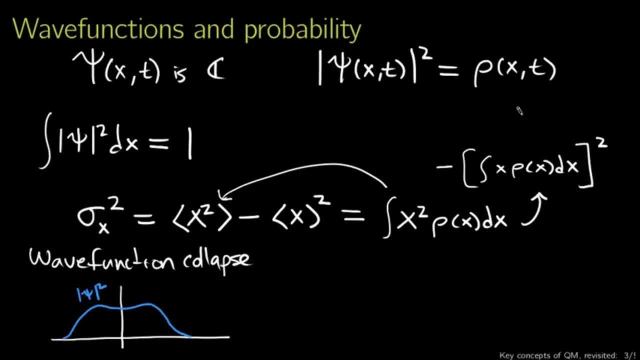 the squared magnitude of psi. this is related to our probability distribution with respect to position. if I then measure the position of the particle, what I'm going to get is, say, I measure the particle to be here now. if I measure the position of the particle, again immediately. 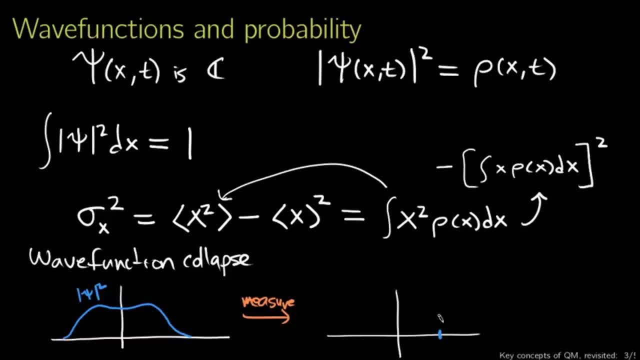 I should get a number that's not too different than the number that I just got. this is just sort of to make sure that if I repeat a measurement it's consistent with itself that I don't have particles jumping around truly randomly. if I know the position, I know the position. 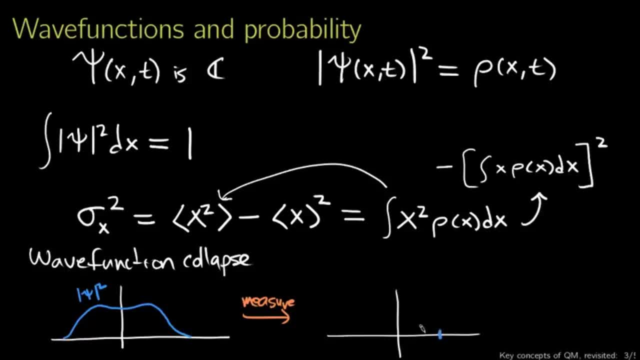 what that means is that the new probability distribution for the position of the particle after the measurement is very sharply peaked about the position of the measurement if this transition from a wave function, for instance, that has support here, to a wave function that has no support here. 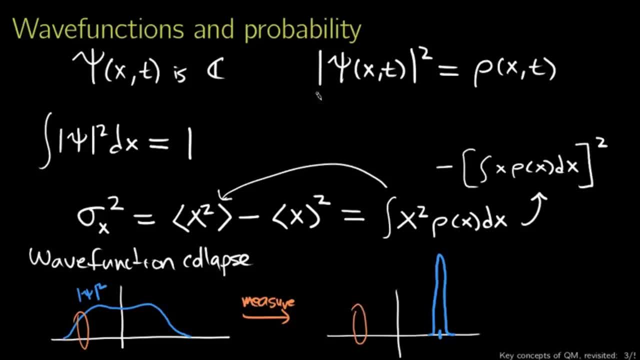 did not happen instantaneously. it's imaginable that if I tried to measure the particle's position twice, that I would have one particle measured here and another particle measured here. does that really mean I have one particle or do I have two particles? these particles could be separated. 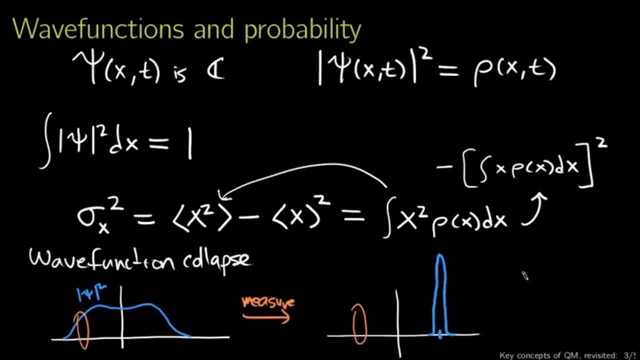 by quite a large distance in space and my measurements could not be separated by very much in time, so I might be getting into problems with special relativity and the speed of light. and these sorts of considerations are what leads to the Copenhagen interpretation of quantum mechanics, which centers on this idea of wave functions. 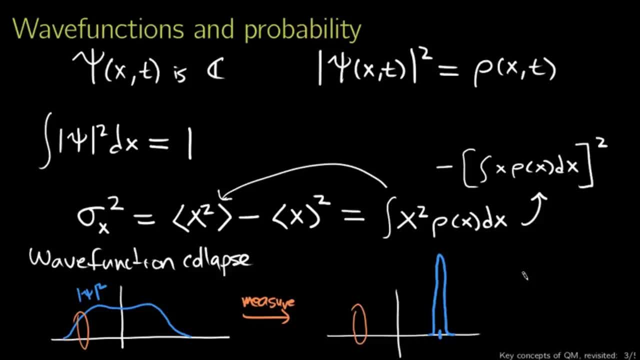 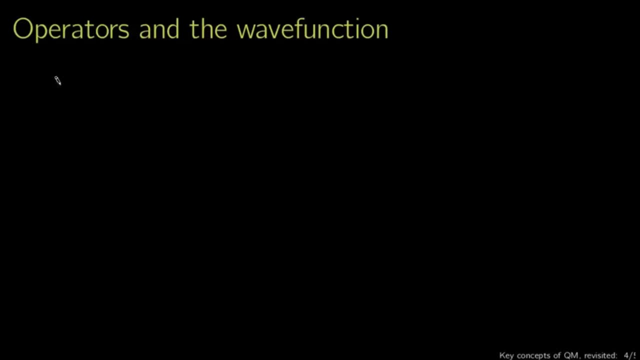 as probability distributions that can collapse as part of the measurement process. now I mentioned operators in the context of expectation values. operators are our second major concept in quantum mechanics. what about operators in the wave function? well, operators, let's just write a general operator as q hat. 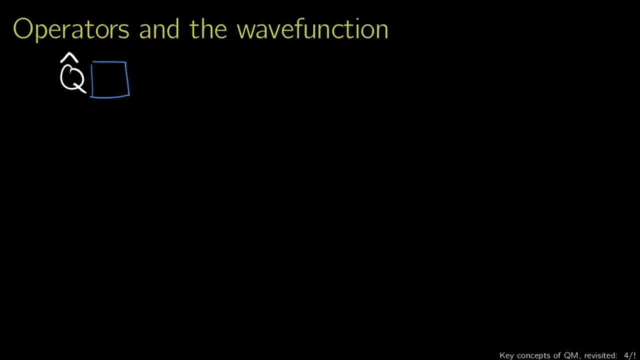 hats usually signify operators. operators always act on something. you can never really have an operator in isolation, and what the operators act on is a function. we have a couple of operators that we've encountered, namely the position operator x hat, which is defined as x times and what's it multiplied by. 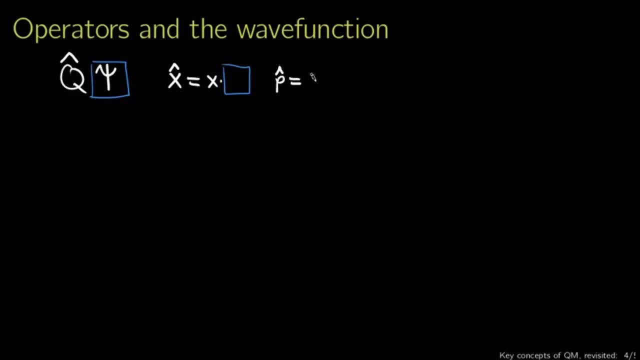 well, it's multiplied by the wave function. we also have the momentum operator, p hat, and that's equal to minus i h bar times the partial derivative with respect to x of the wave function. we also have the kinetic energy operator, t hat. you could also write it as t hat. 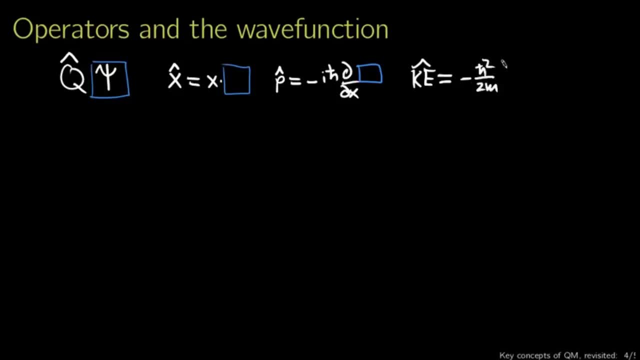 that operator is equal to minus h bar, squared over 2m times the second derivative with respect to position of what well? of the wave function. and finally, we have h hat, the Hamiltonian, which is an expression of the total energy in the wave function. it's a combination of the kinetic energy. 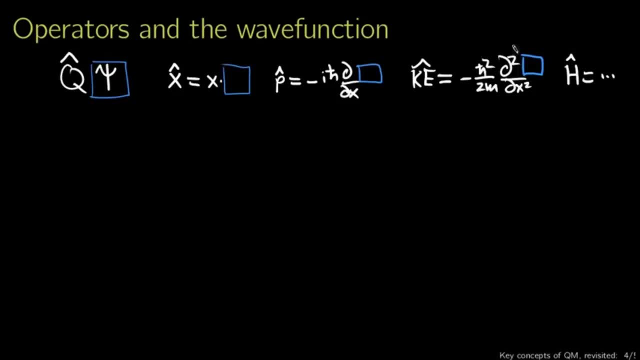 operator here, p squared. we have a second derivative with respect to position minus h, bar squared. this is just p squared divided by 2m. p squared over 2m is a classical kinetic energy. the analogy is reasonably clear there. you add a potential energy term in here. 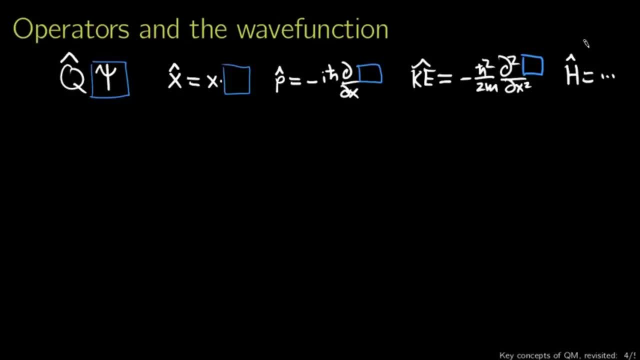 and you get the Hamiltonian. now, expectation values of operators like this are calculated as integrals. the expectation value of q, for instance, is the integral of psi star times q acting on psi over all space. this bears a striking resemblance to our expression, for instance, for the: 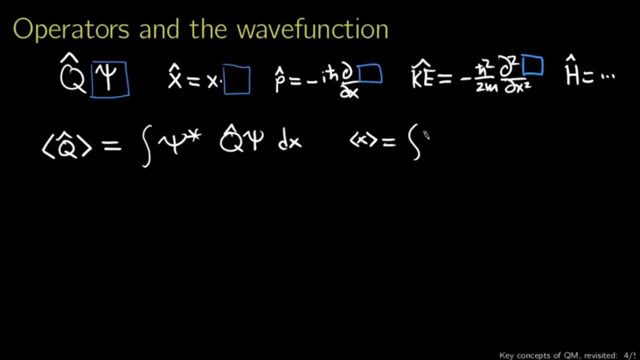 expectation of the position, which was the integral of just x times rho of x, where rho of x is now given by the absolute magnitude of psi squared, which is given by psi star times psi. now, basically, the pattern here is: you take your operator and you sandwich it. 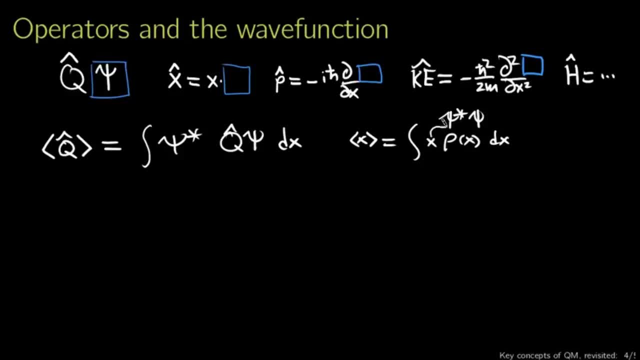 between psi, star and psi, and you can think about this position as being sandwiched between psi, star and psi as well, because we're just multiplying by it. it doesn't really matter where I put it in the expression. the sandwich between psi, star and psi of the operator is more. 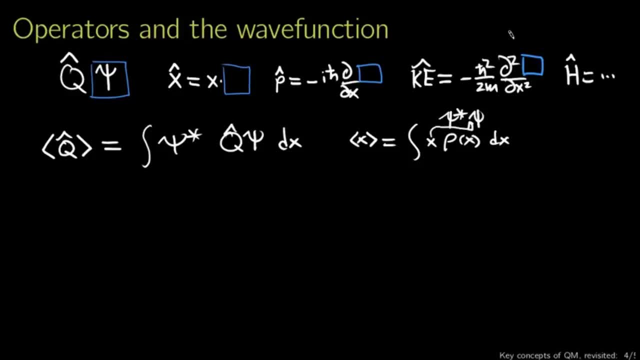 significant when you have operators with derivatives in them. but I'm getting a little long winded about this. perhaps suffice it to say that operators in the wave function allow us to calculate meaningful physical quantities like x, the expectation of position. this is more or less where we would expect. 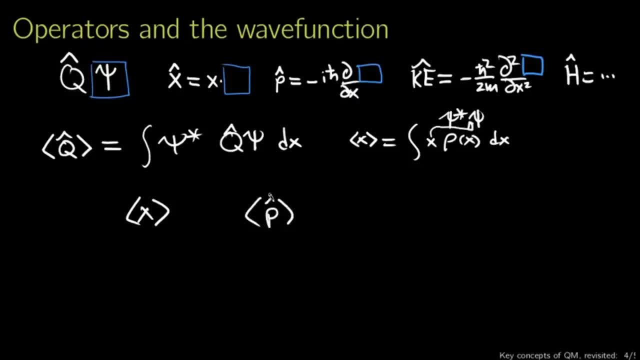 to find the particle or the expectation of p, and I should be putting hats on these since technically they're operators. the expectation of p is more or less the expected value of the momentum, the sorts of momentum momenta that the system can have, or the expectation value of h. 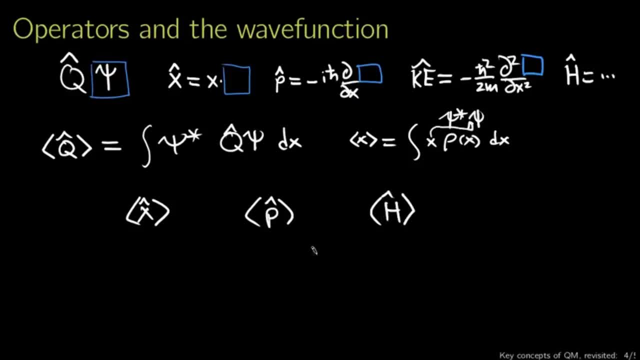 the typical energy the system has and all of these are tied together in the context of uncertainty. for instance, if I wanted to calculate the uncertainty in the momentum, I can do that with the same sort of machinery we used when we were talking about probability that I calculate.